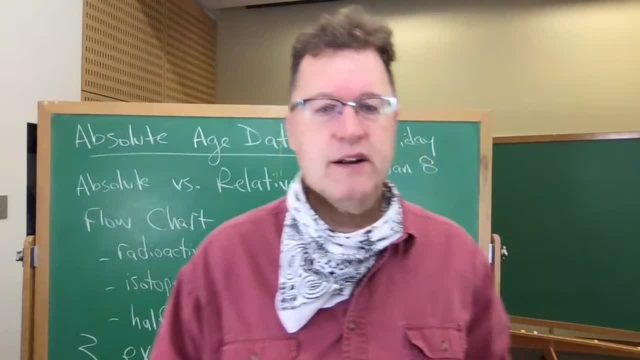 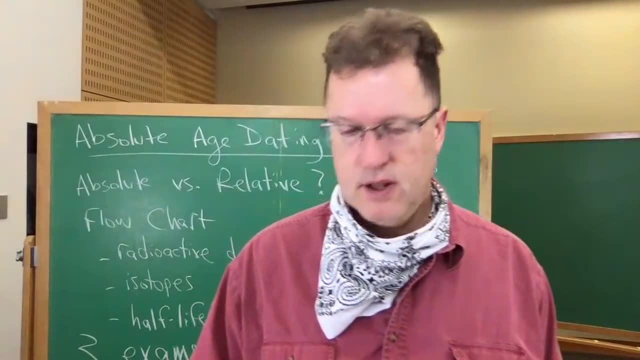 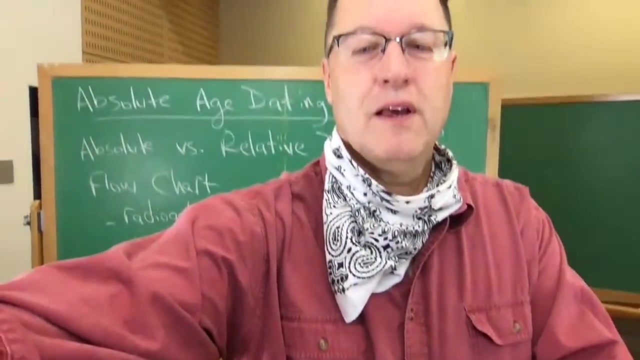 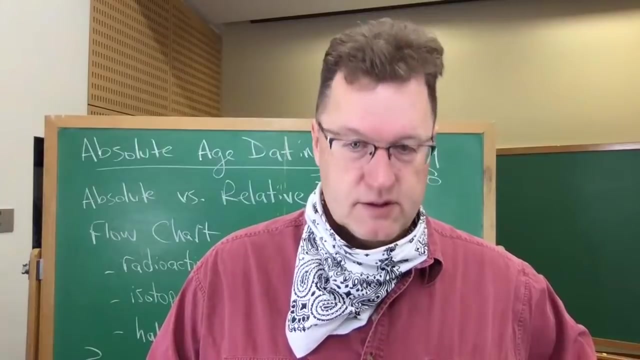 adjustments Got the light A little higher today- These two side lights a little further away from me, But let me give you a chance to copy down your outline today, students. Oh no, we'll say hi first. How about that? Just making sure that we are communicating properly. Good morning Friday. 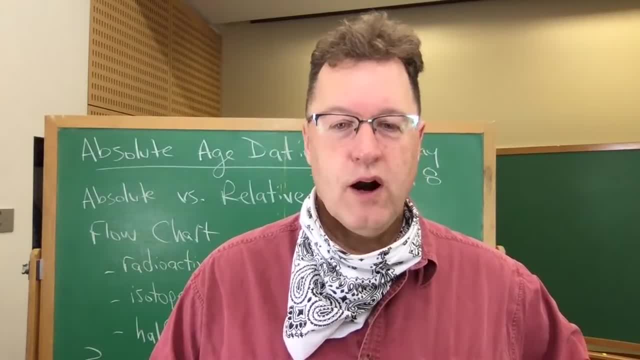 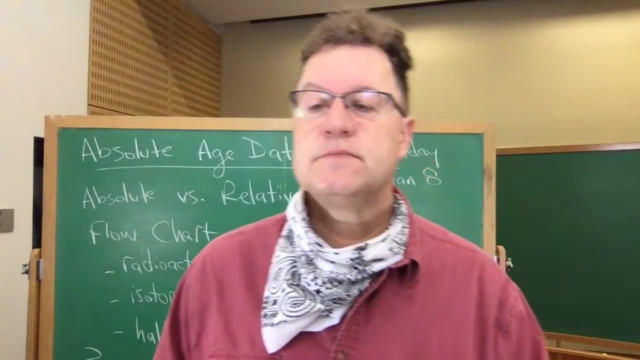 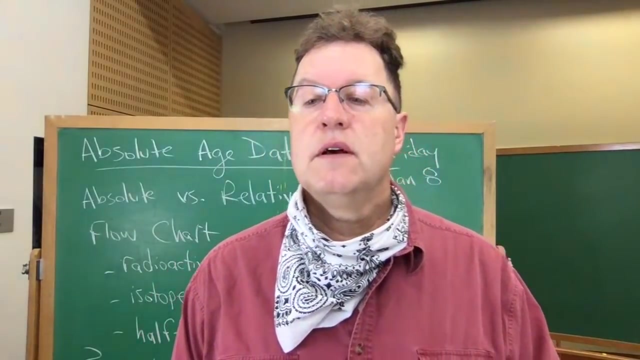 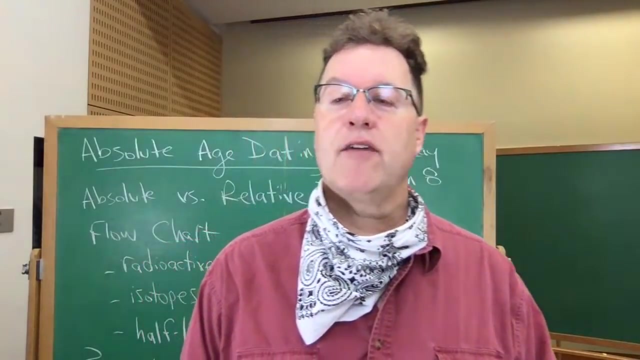 morning, It's Fri-yay And where are you viewing from? Matthews and Connections, Connecticut. Hello Elise in Devon, UK. Eric's in Marion, Virginia. Dennis is in Jurassic Coast, Dorset, UK. Temecula, California. Hello Cleveland, Ohio. Sharon's in Woodstock. 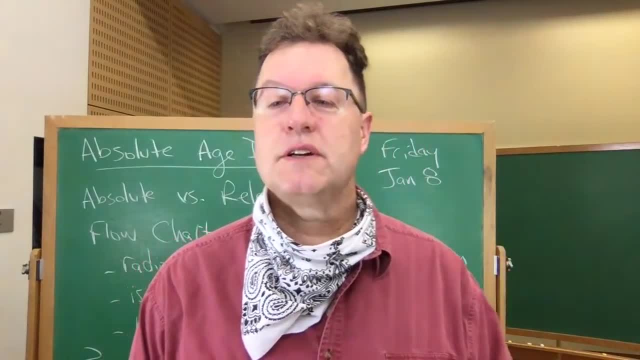 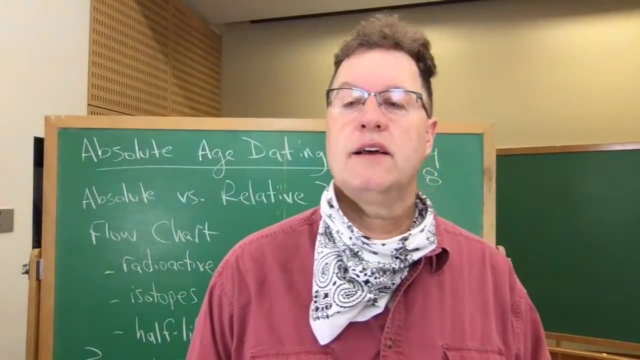 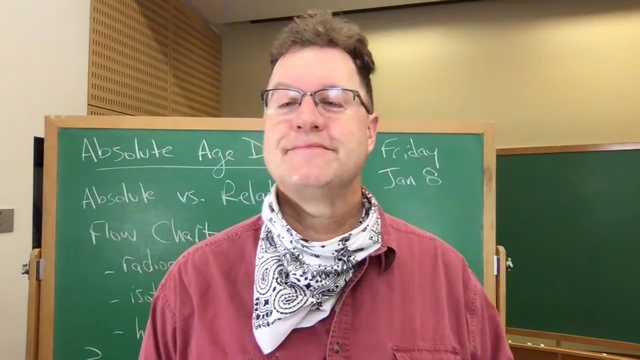 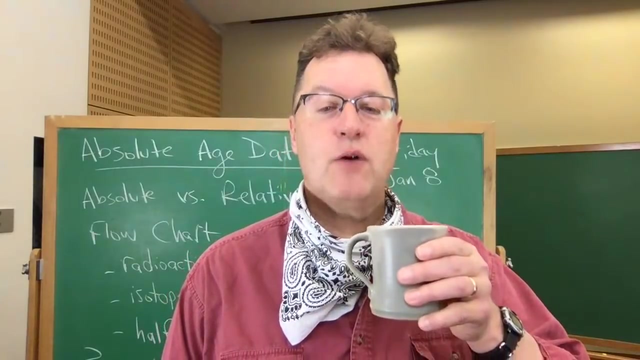 Georgia, Calarjo's in Switzerland, Karen is in Midland Ontario, Jay's in North Carolina, Lila is in Kansas City, Sid's in Cretaceous, Texas, Barbara's in Indiana. Oh man, the Badgers, Wisconsin Badgers, Indiana Hoosiers, That was a great game last night, That college. 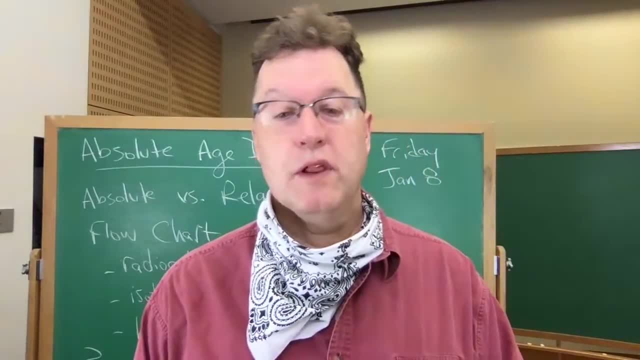 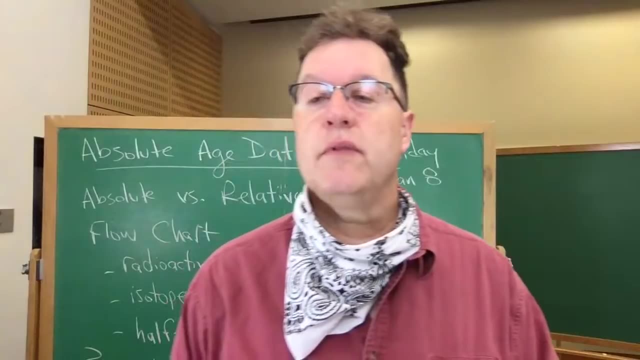 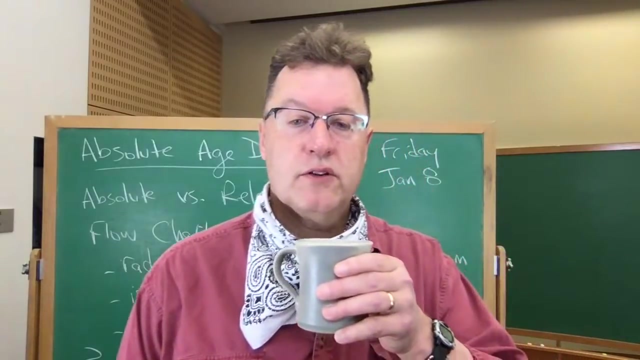 basketball. I'm talking about Boy really thoroughly enjoyed that. Linda Santa Cruz, California. That's from the UK. Mark from Kingman, Arizona. Custodians talking loudly in the hallway- Oh, maybe they're pissed at me. I got chalk dust all over the place. 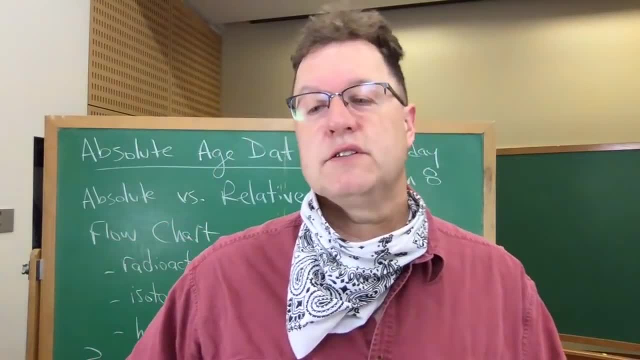 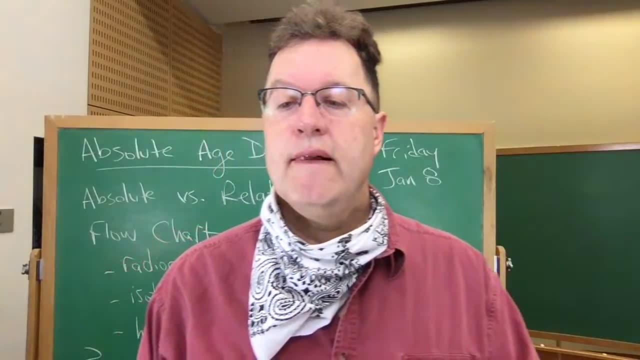 Aarhus, Denmark. Hello. A few more and then I'll give you a chance to look at our outline for today. Indy Cougar Craig is in the Metow Valley, Minneapolis, Minnesota. Hello, Terry, We're greeting our주opost accompaniment officials儿. 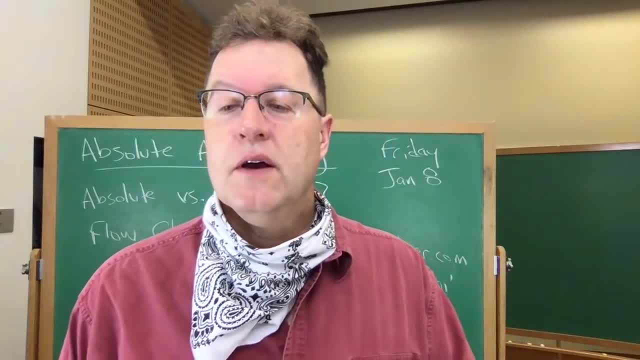 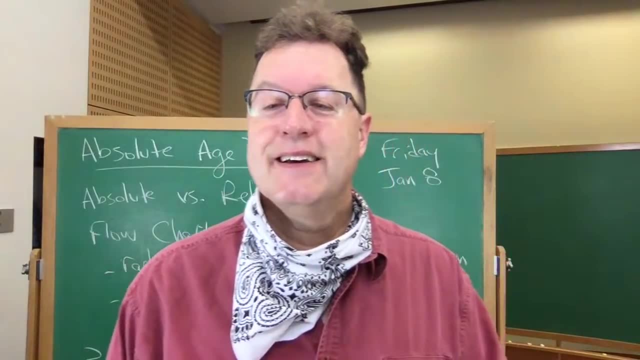 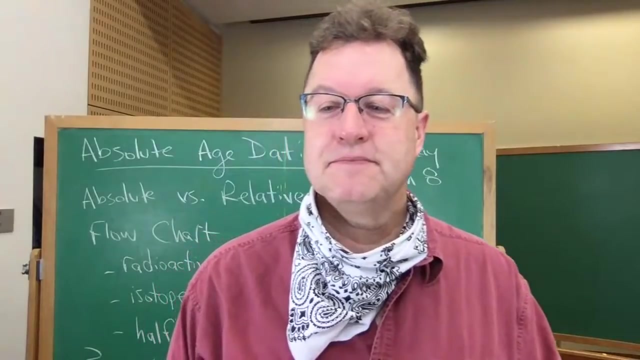 Mostly North Americans today. is that true? Valencia, Venezuela. Hello Clara, That's cool Freebird in Whidbey Island, Washington, Aurelio from Spain. Gillian is in Pasco, Rio de Janeiro. Good morning or good afternoon. 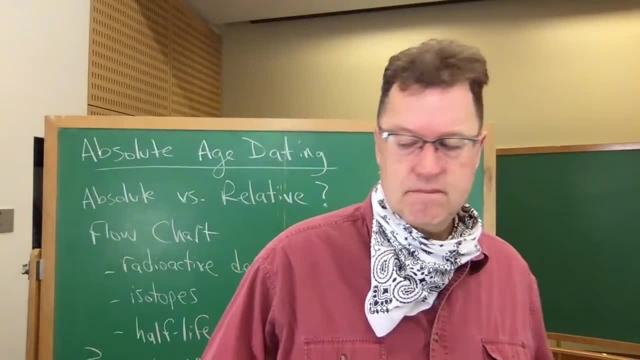 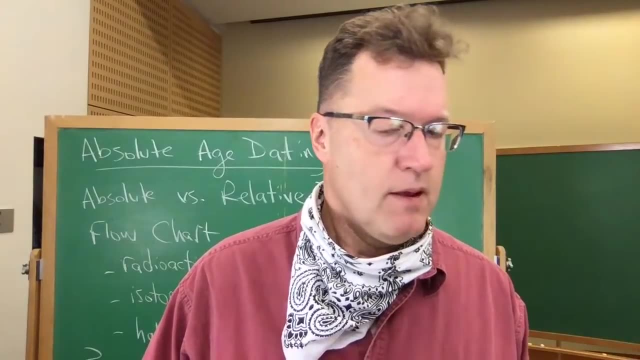 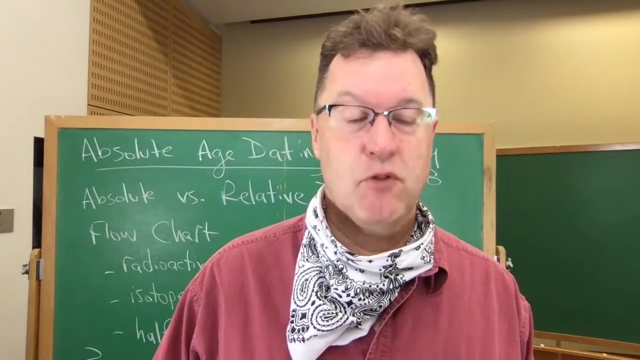 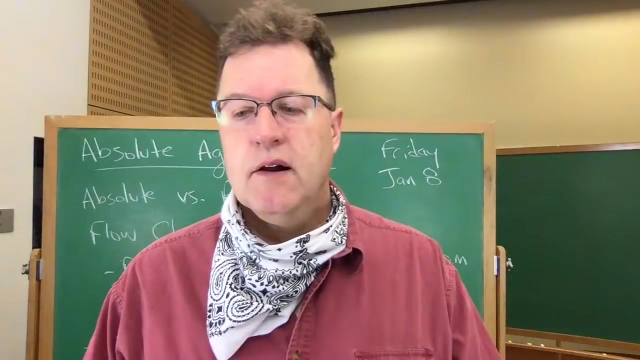 Wonderful, Okay, Uh, There's less and less to say ahead of time. I feel like we've got things going here a little bit. Today will be a challenge if you haven't heard this content before for some. I'll tell you what. 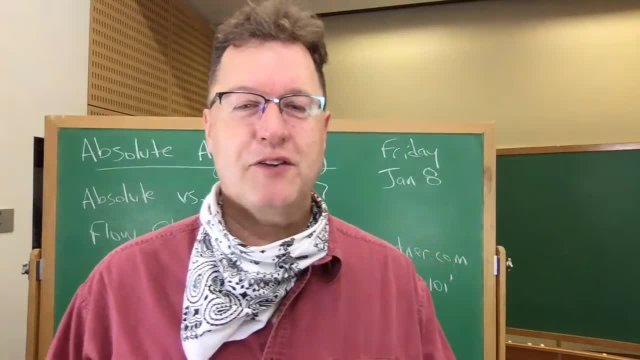 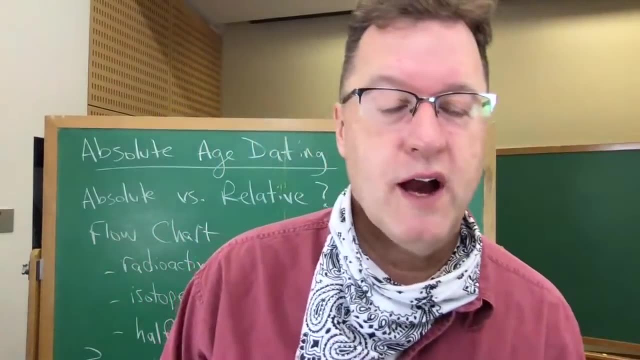 So there were a lot of suggestions on what to call you all, because you know the drill by now, I think. right, We're still early in the class, so I guess I'll say it one more time. I am paid to teach to CWU students. 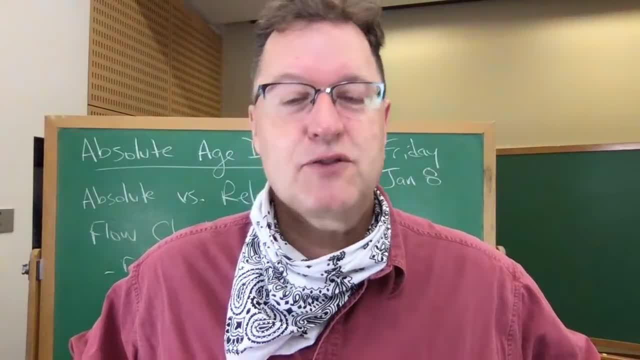 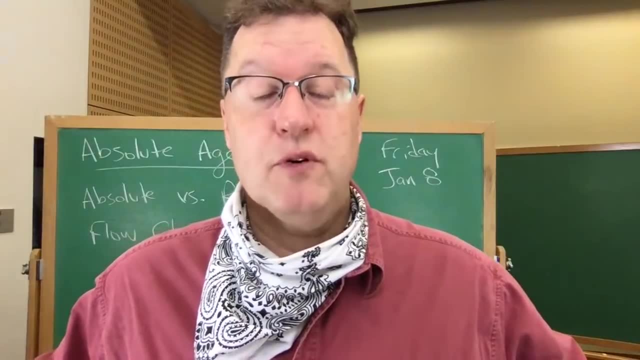 Makes sense, right? That's where I teach, That's where this classroom is right now- Central Washington University- And we are patiently waiting until Tuesday, January 19th for them to arrive in person, And there's about 20 of them. 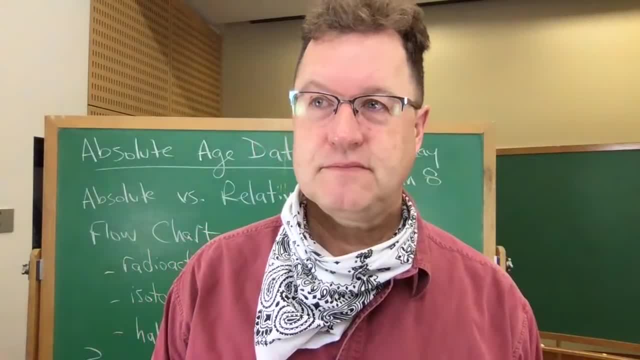 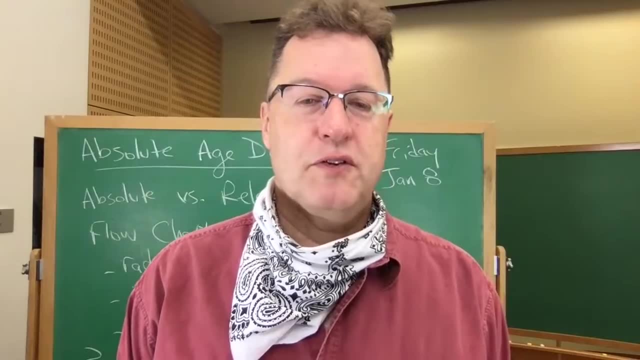 That will be spread out throughout this large auditorium And I will continue to live stream, even though I'll be talking to them. So those are the students, But I was kind of playing with what am I going to call you guys? 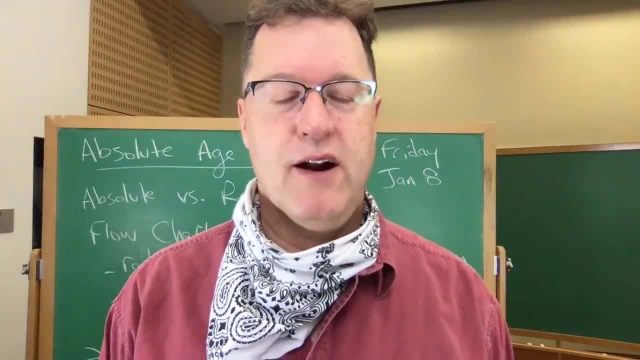 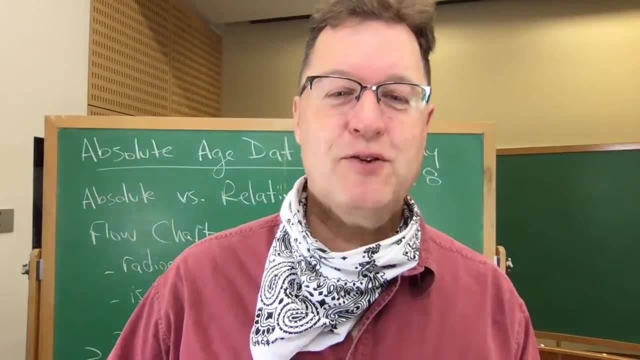 And again, as soon as I said it, I'm like: well, that doesn't even really matter because I'm not going to be referring to you. I'm talking to them. They're the paying customers, But I have used the term townies for folks from: 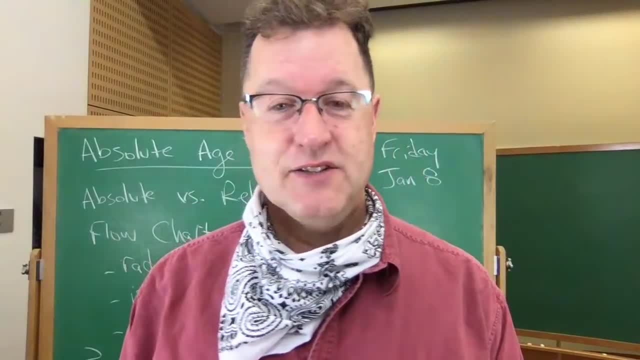 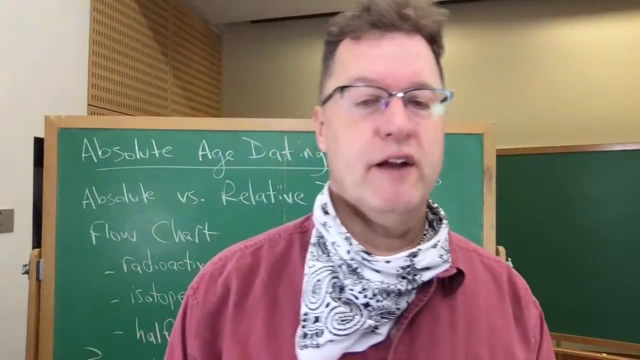 town who would come in and sit sit in on the class for free, And some townies. I started this about 10 years ago Now. we teach every fall and every winter And felt like I burned through most of the community. 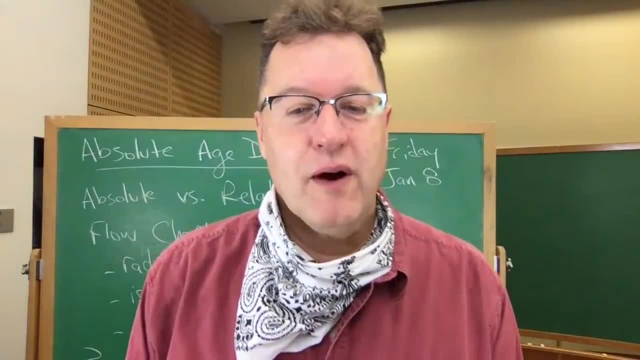 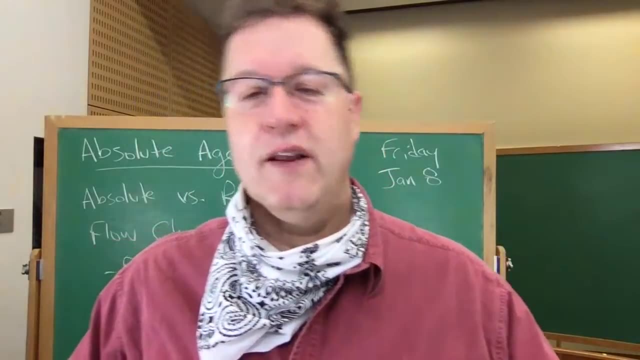 They'd, all you know, usually retired folks. you know they want to stay active, They want to get on campus, They want to get it back, you know, to learning a few things. Just go out for coffee in the morning and then walk over here and sit in with the class. 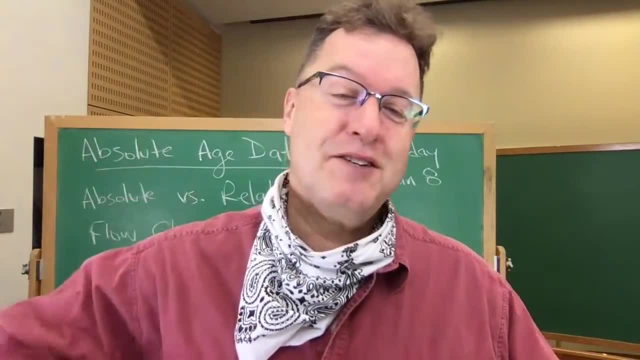 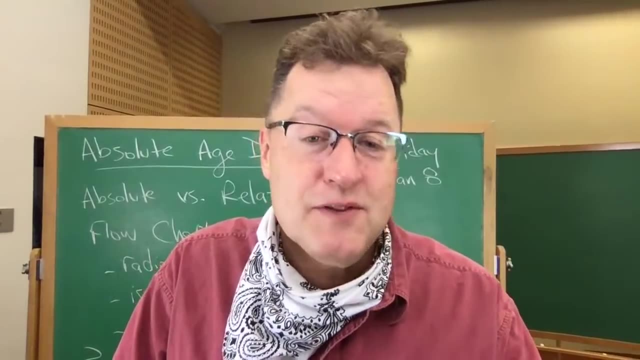 So I would call them townies And I think I'm going to call you guys townies. There were all sorts of interesting suggestions, Many of them I really liked, So thank you for the suggestions for the names of what to call you. 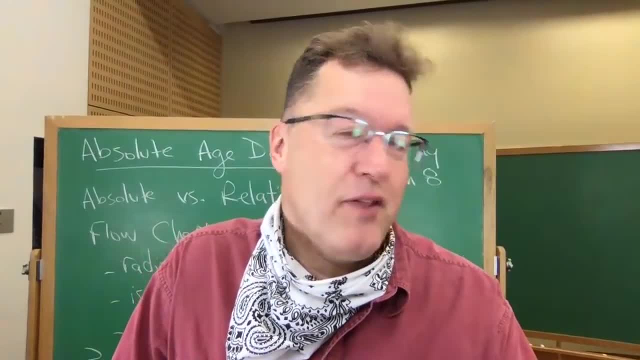 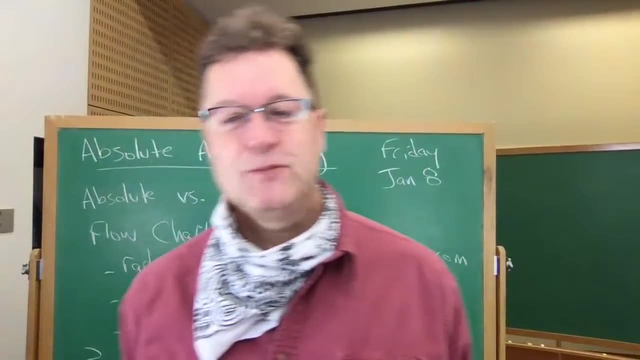 But it's going to be easiest And I think it's actually after thinking about it. a few of you suggested I just continue with townies. I kind of like it. This is a global town essentially, So you're sitting in on the class. 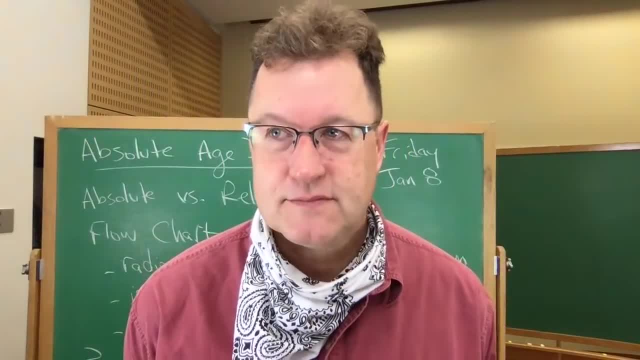 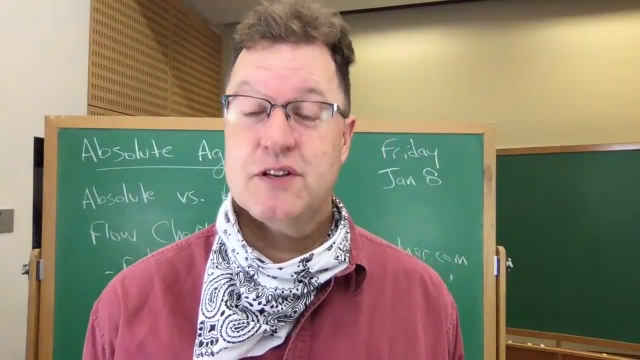 It's part of your routine, many of you, And that's what the townies were. I hope we can go back to that at some point, Maybe as soon as this fall. Wouldn't that be nice? It's dangerous to hope these days. 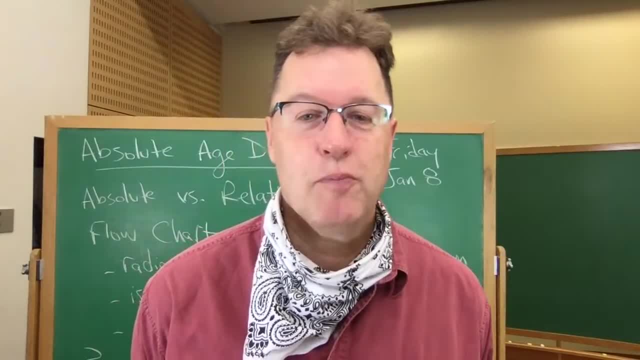 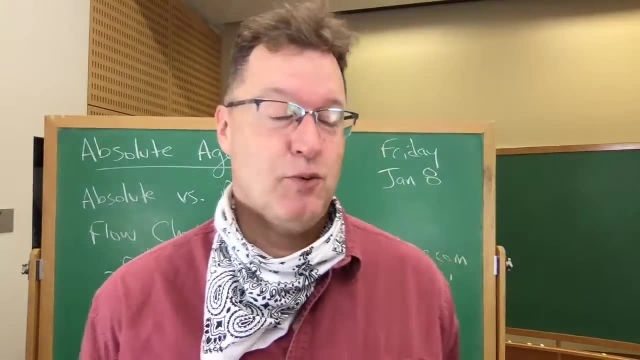 But I don't know. Doesn't hurt to hope, does it? So I think you guys are the townies, That's at least what I'll refer to you as. But if you still want to hold out and call yourself whatever, that's great. 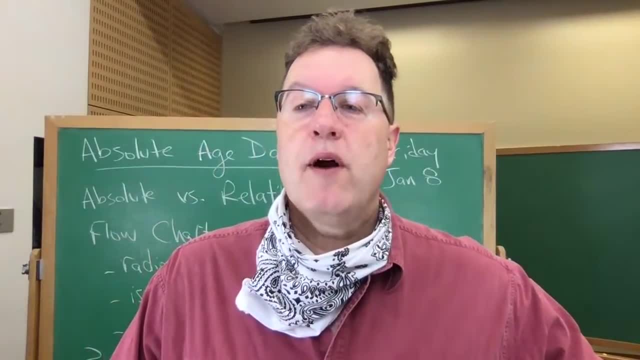 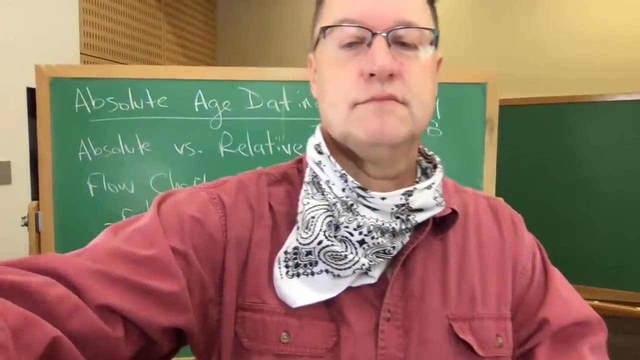 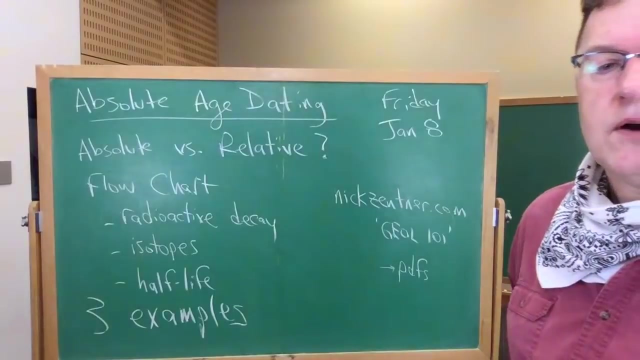 Adele, good morning. All right, A couple more hellos And then I'll start thinking about: oh no, I want to give you a chance to. I'll say one more thing. I'll stay out of your way. 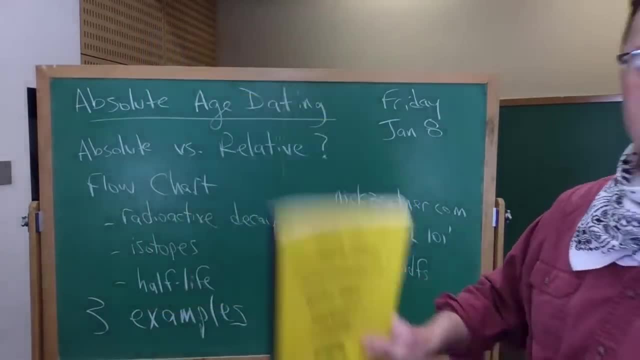 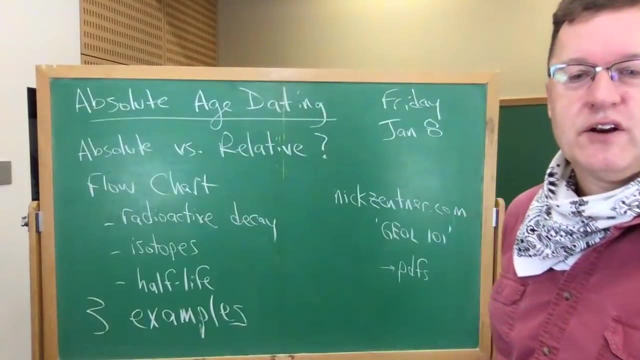 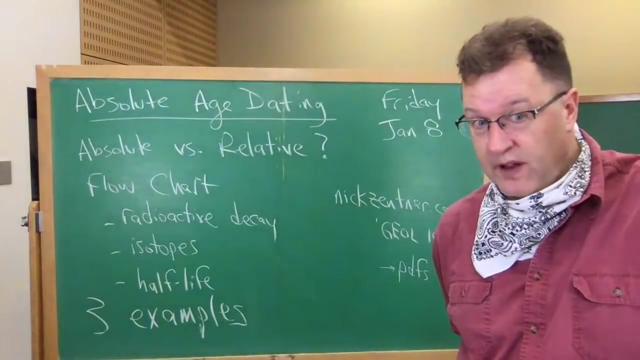 I mentioned that this is the course pack for the quarter And I'm talking to you townies now. I'm assuming the central students are not here yet. I want them to buy this thing. I want them to go to the next building over into the university bookstore. 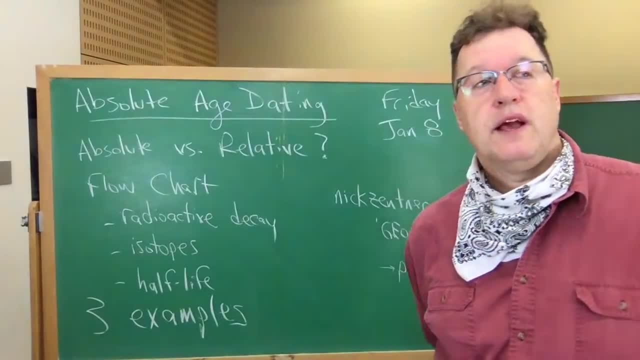 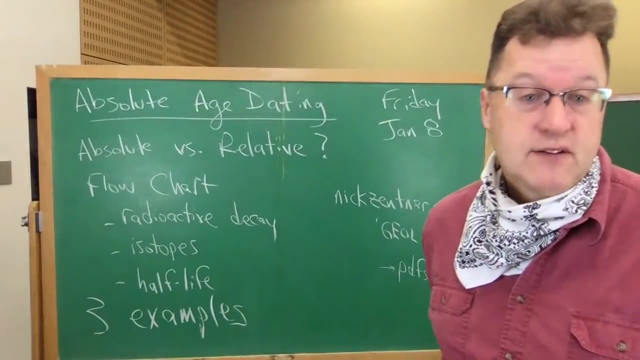 And I want them to buy this thing for $10.. I have a good relationship with those guys in custom publishing, Darren and Michelle. they've been great to me over the years And they take the time to print these out and publish them and that sort of thing. 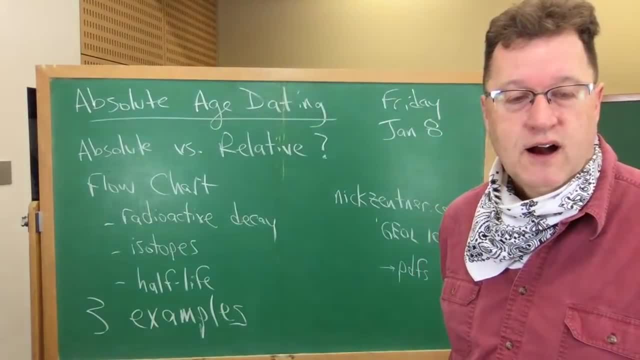 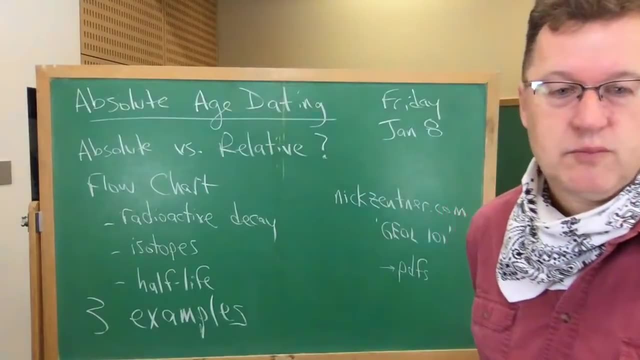 So I don't want to put the PDF of this on my website right now, Because these guys, I don't know what they'll do, but there's a chance they wouldn't go over and buy the book. They would. just I don't know. 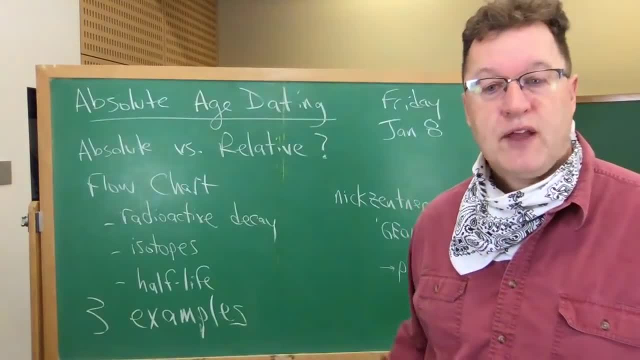 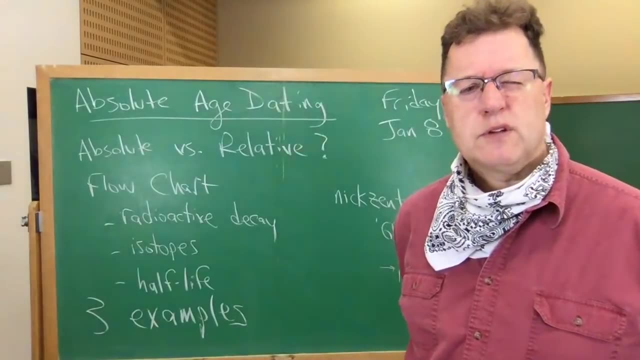 They wouldn't buy the book. I want them to buy the book. I think it's best for them to have this in paper form as they come in. But Darren was a little hesitant when I said, hey, can I just get the PDF for this thing? 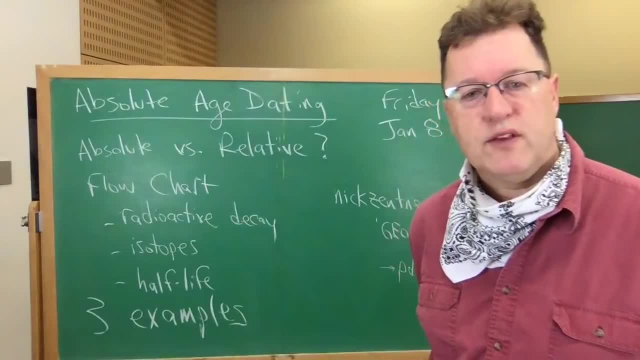 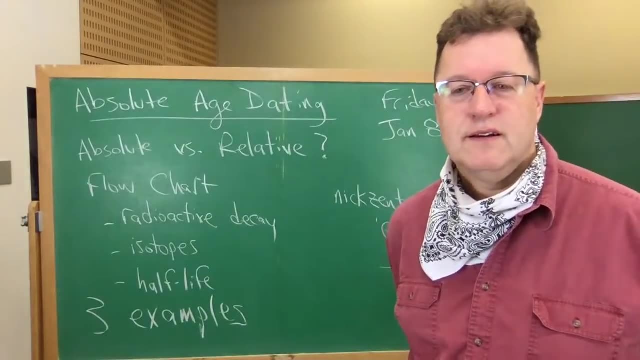 I think I'm going to have a distant audience that's going to want this book. He's like, well, yeah, I guess, so I can do that for you. But you know we want your students to. you know we need to exist over here. 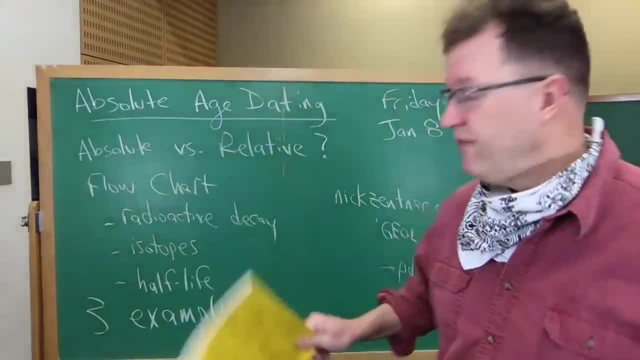 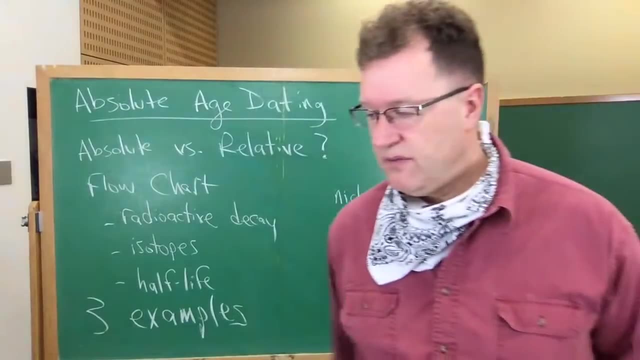 So my point is: I'm going to make this PDF available here, but not till next week. We're going to use it this morning, but I'm only going to use it for a few little pages. And I've heard from many of you and you want this thing and I get it. 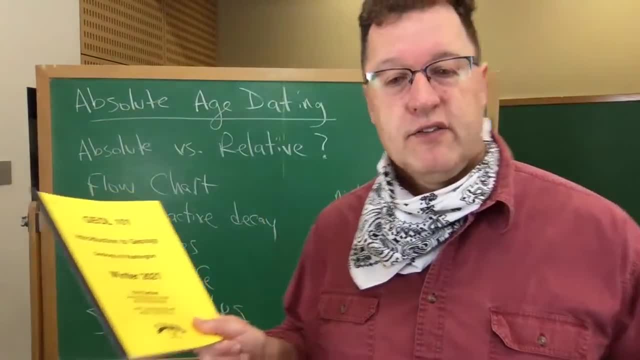 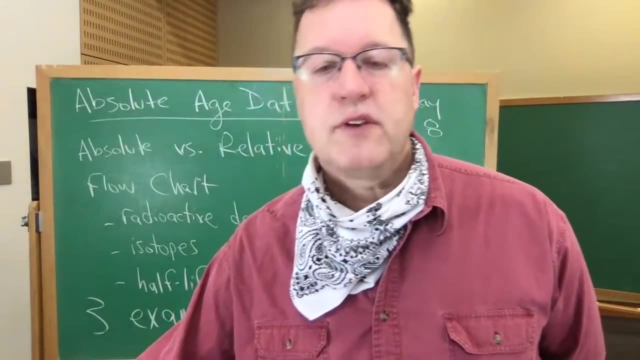 And I'll give it to you for free as a PDF that you can print out if you want. I guess, Or just you know refer to. But I want those central kids to pay their $8. It's not much, but 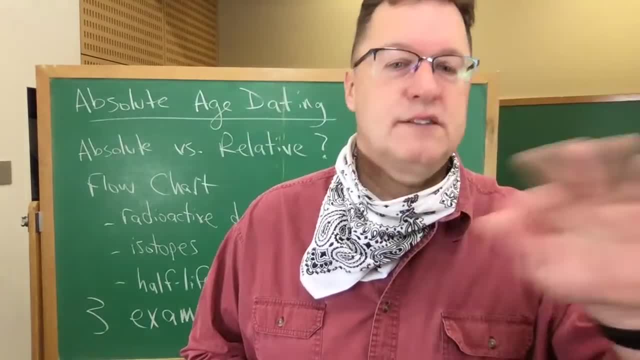 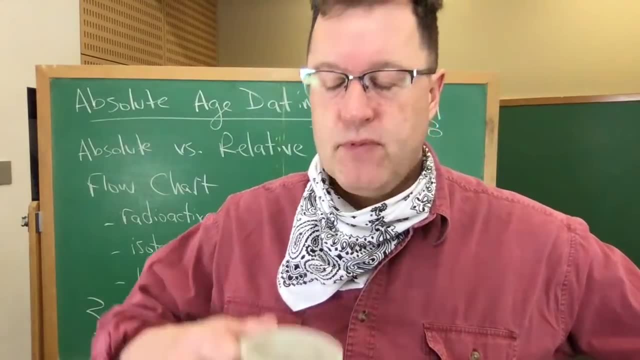 So that's my thinking there. And I know you'll pay for it, et cetera, et cetera. But it's just too messy that way. Let's just make it nice and easy. Okay, Thank you, All right. 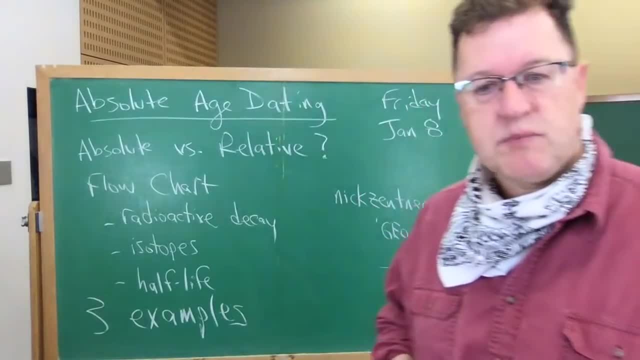 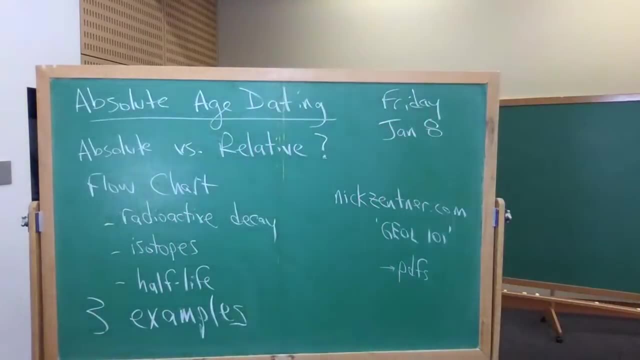 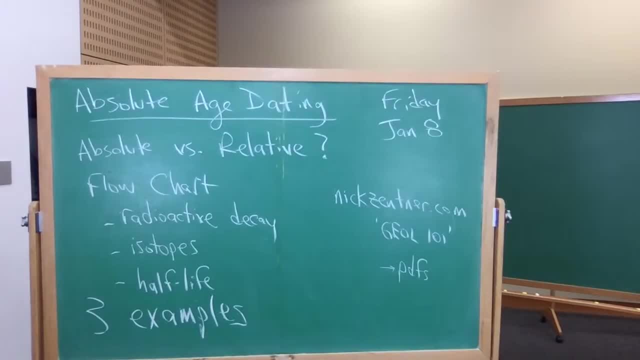 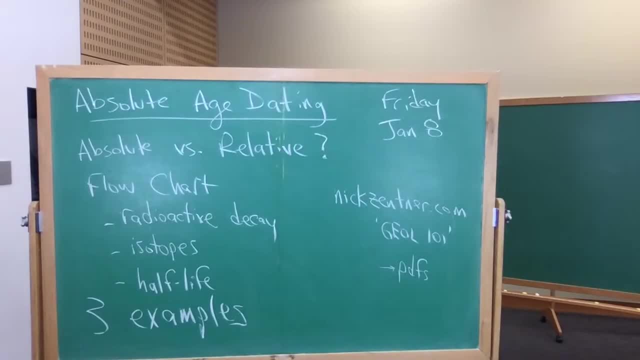 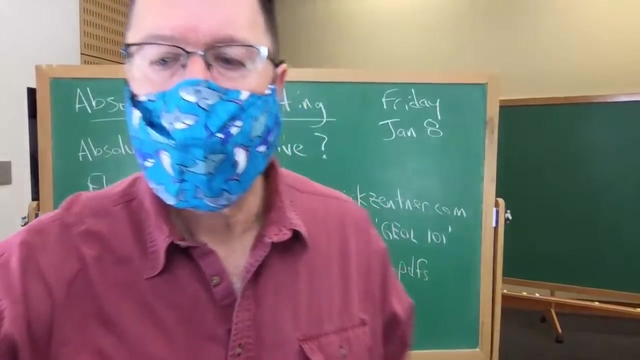 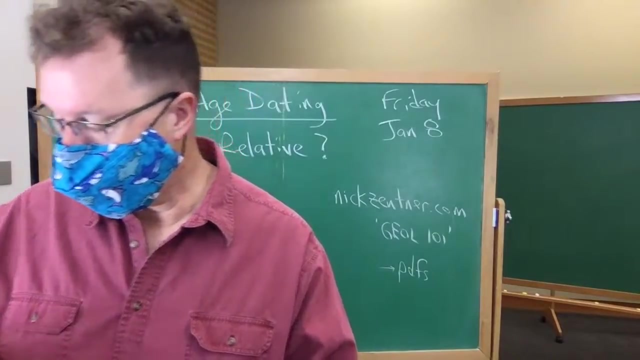 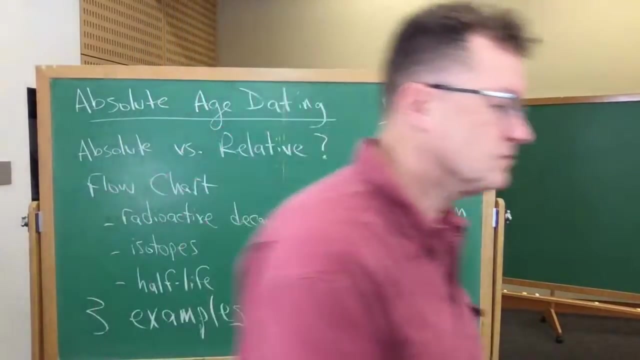 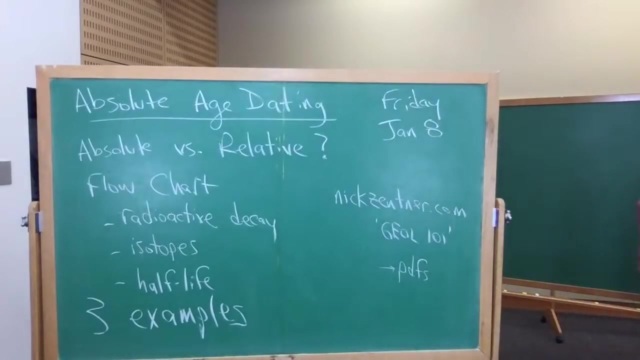 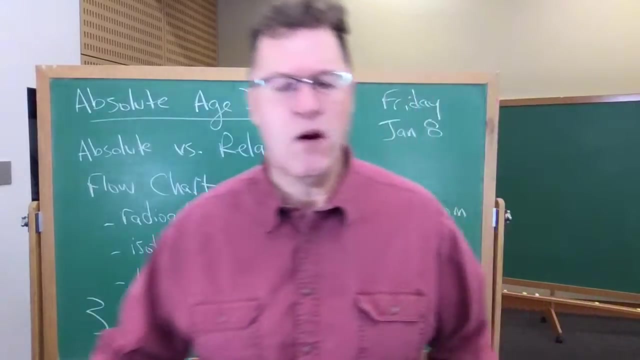 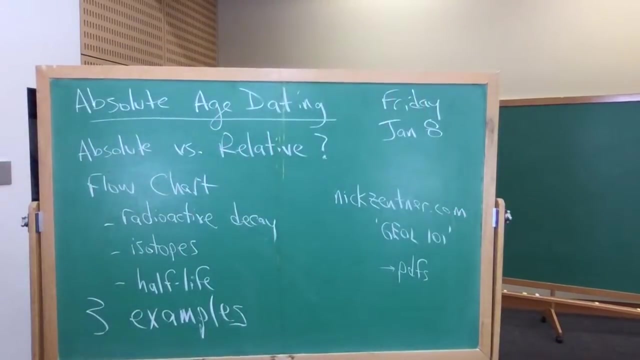 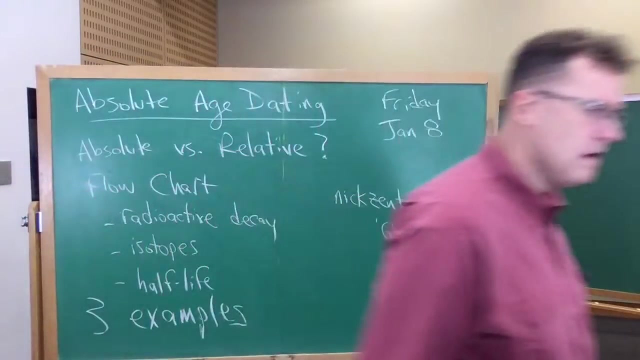 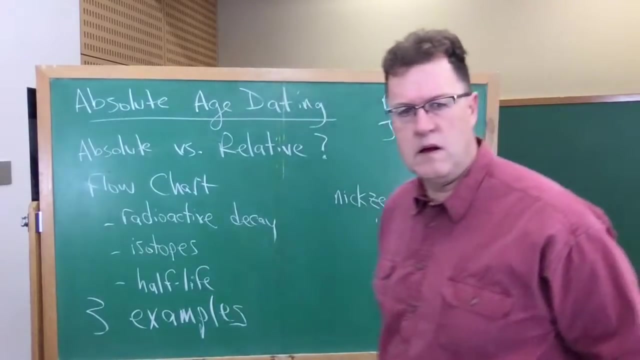 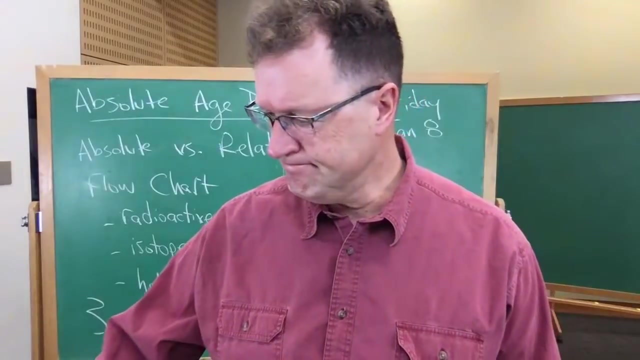 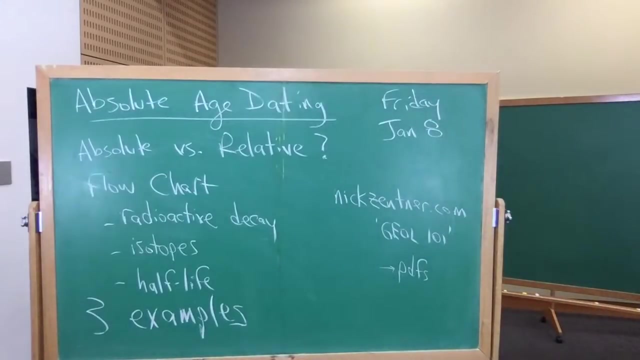 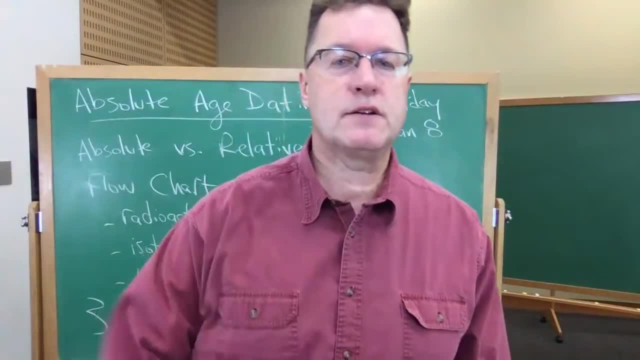 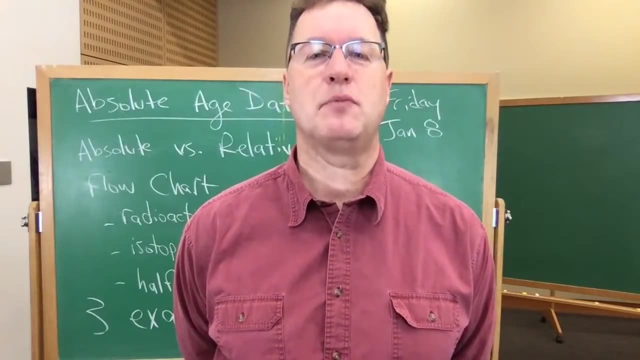 Well, good morning Central students. Thank you for joining us again live this morning. It's 10 o'clock in the morning, That is our class time and we meet every day except Wednesday, So I'll see you next Monday morning, of course, at 10 am. 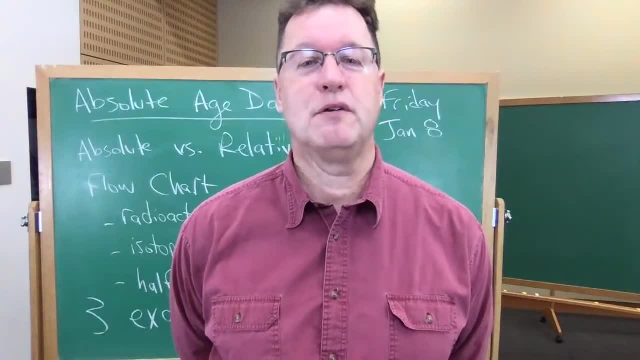 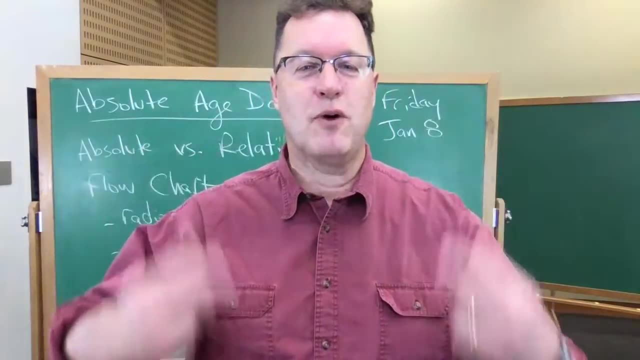 I've been hearing from many of you. You've been following through on watching these live with us and then, as soon as I sign off, you send an email to me The first day to confirm that you watched the live stream. you emailed me with the subject: word green. 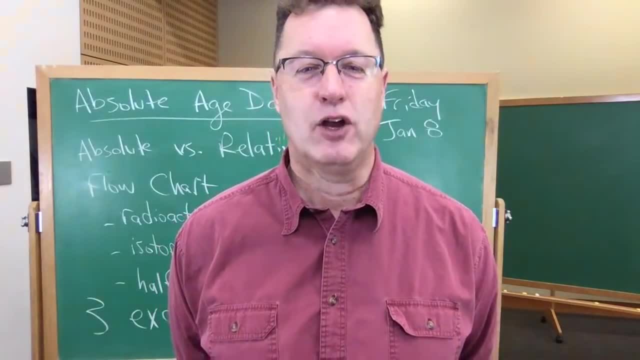 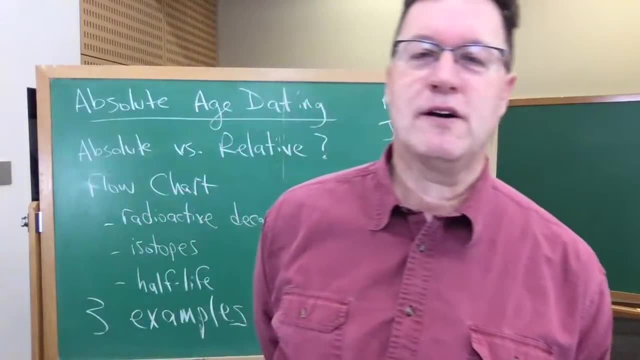 Many of you did that and I got a big kick out of it Yesterday. you suck about 15 of you. That's wonderful. Thank you Today. the secret word that you will email me, I guess now or in 50 minutes when we're done. 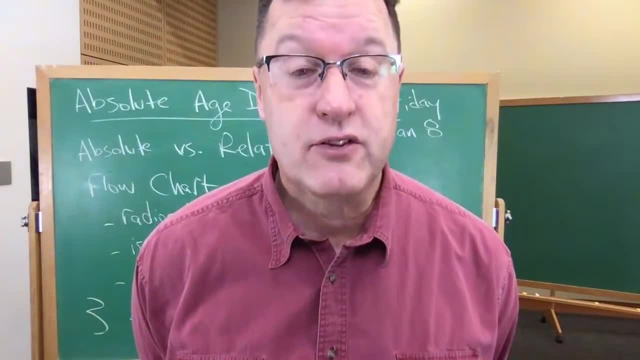 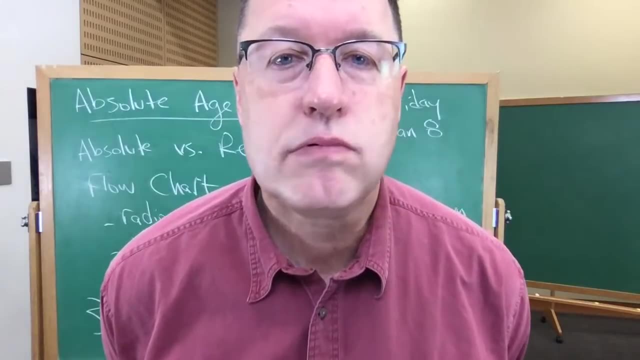 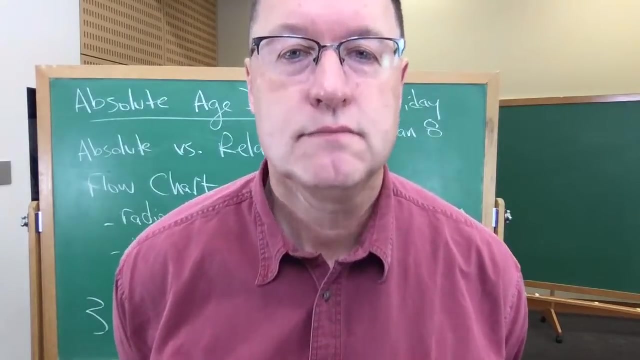 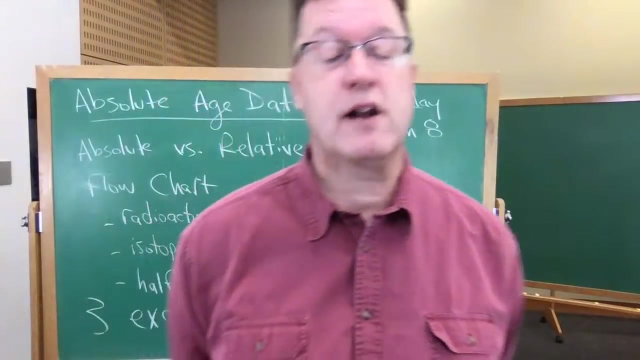 probably better to wait until the end is. can you please send me an email with the subject word Again, that is, type please in the subject of your email: Thank you, And that will let me know that you are alive, that you are part of the class. 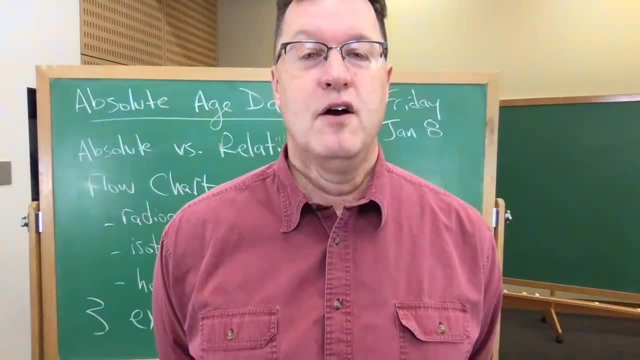 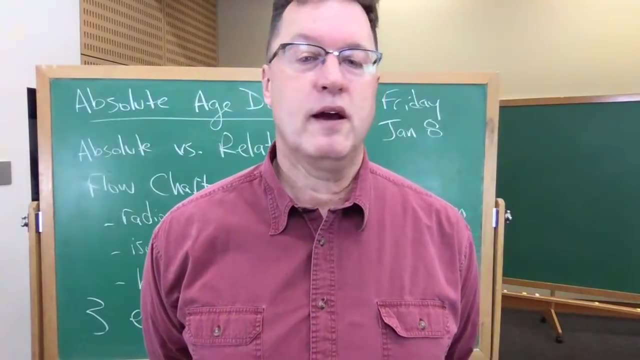 that you are taking notes, that you are preparing yourself for our first quiz, So that when we finally get to see each other a little more than a week from now, we won't be having to start from scratch. We'll already have a bunch of water under the bridge, as it were. as it was. 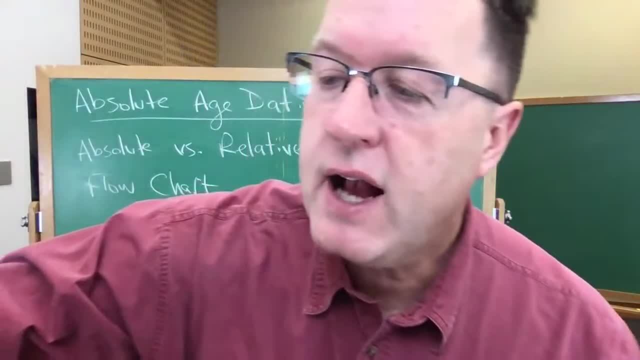 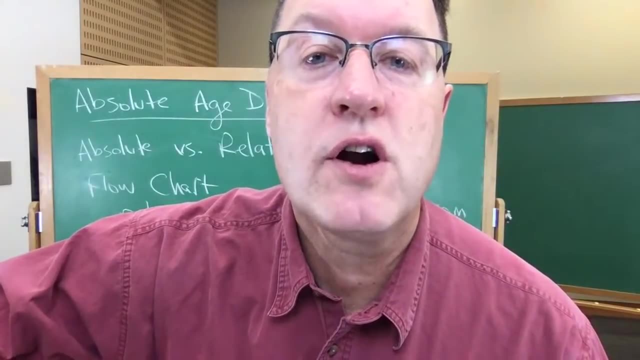 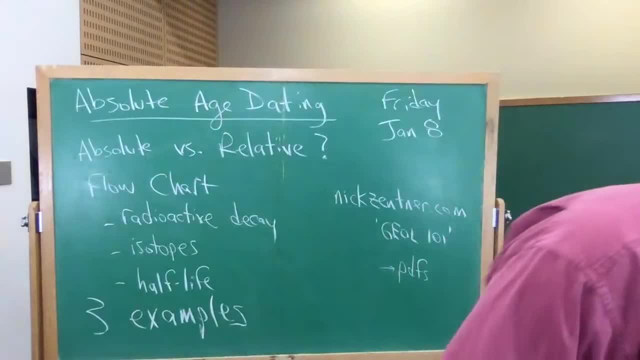 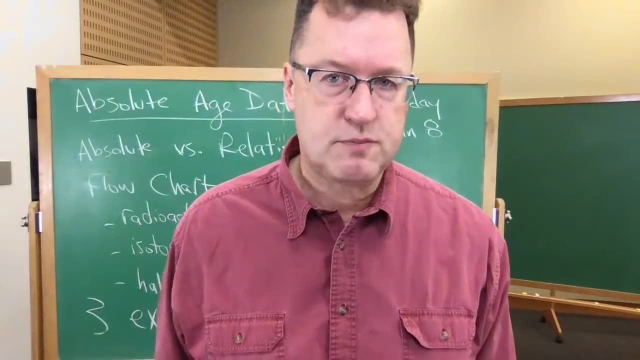 Okay, Okay, Let's go. You're better than this. Come on, You're missing out. Don't dig yourself a hole, especially after today's lecture. You want to make sure you're on top of this material and ready to go when we see each. 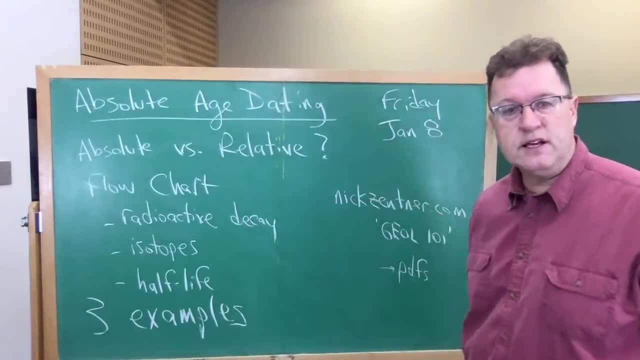 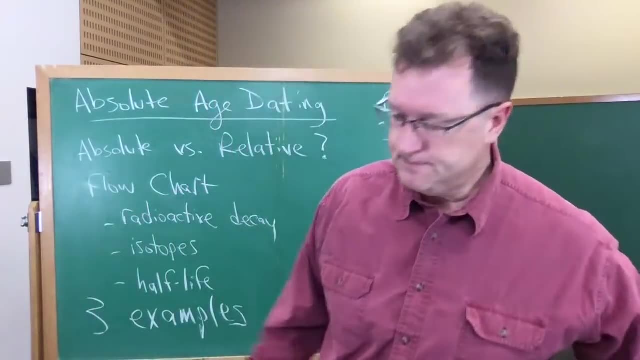 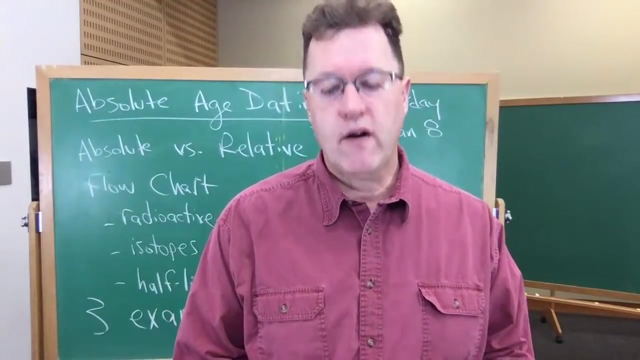 other. Okay, So today is absolute age dating, Yesterday was relative age dating. What's the difference? Well, well, well. well, yesterday we talked about James Hutton, uniformitarianism, kind of philosophical stuff, about modern geology, and then we ended with this: 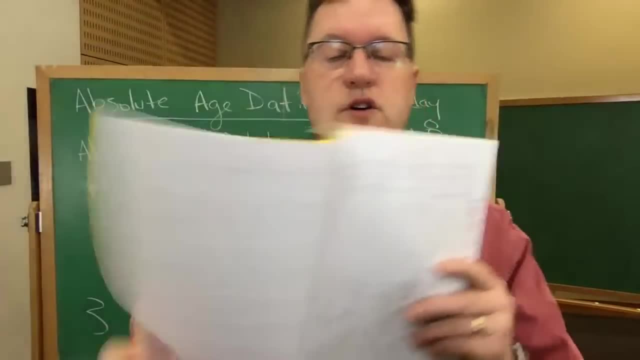 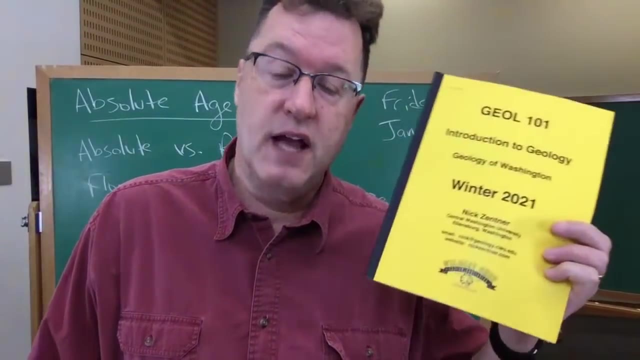 which is page two in your course pack. so i heard from darren over at the bookstore. he's got these now. they're on the shelf, they're ready to be purchased for i think it's eight dollars. so if you're in town i encourage you to go over today. grab this thing so that you're ready for. 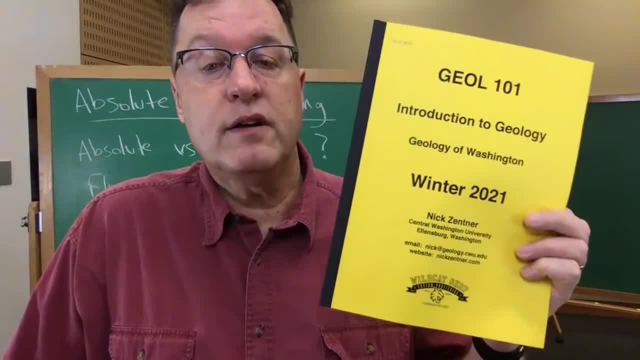 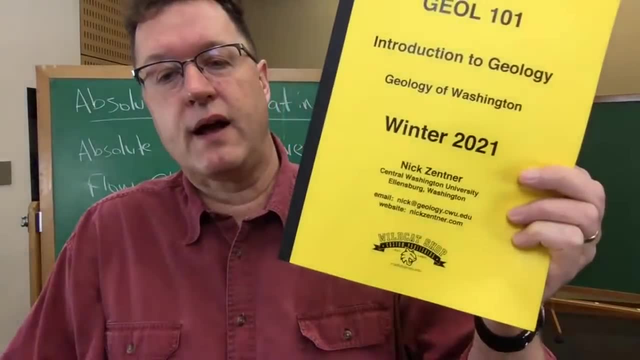 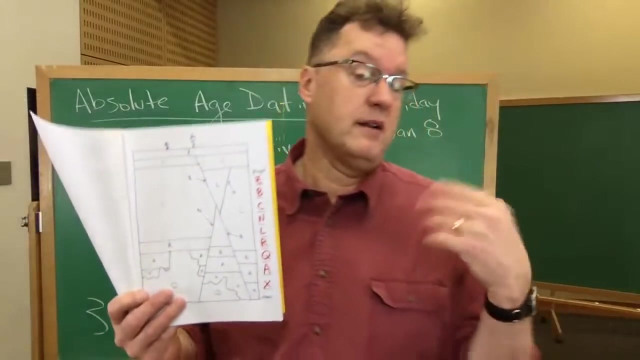 monday's class. if you are not in town, you can get to the wildcat shop- email, uh, web form page, whatever- order a course pack and i don't know how they'll get it to you, but whatever. so please get this thing as soon as you can- not urgent, but would be helpful to you and you'll want this in class. 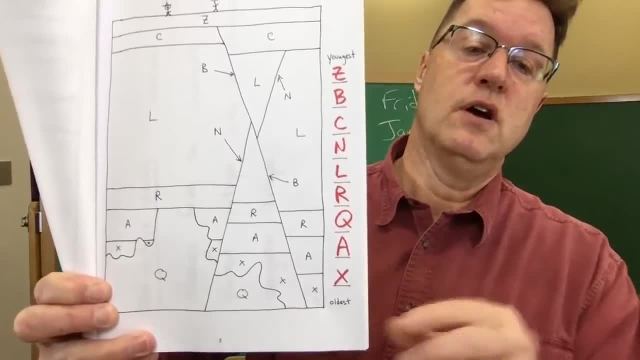 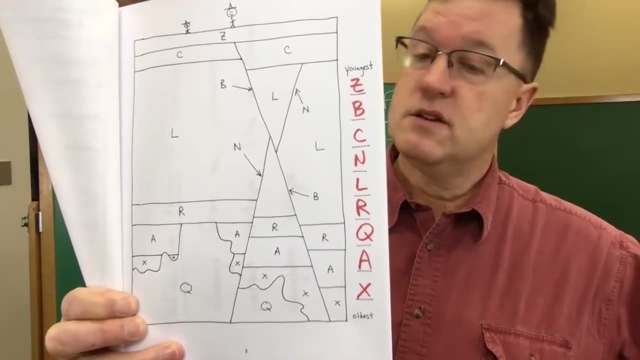 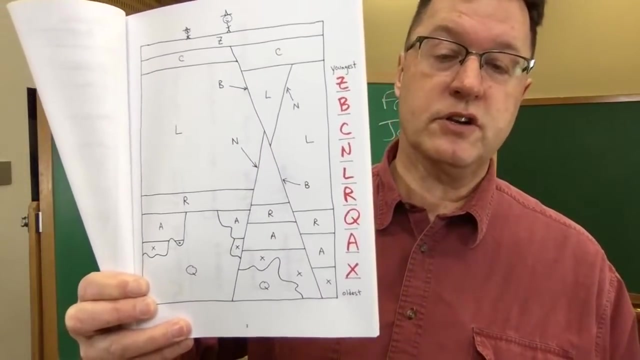 with you every day that you come in. and here's page two with the quote-unquote answers. and we talked about relative age dating last time. what was the game? simply putting things in order. we have no idea when this happened. this all could have happened a hundred million years ago, a billion years ago. this thing could be a billion. 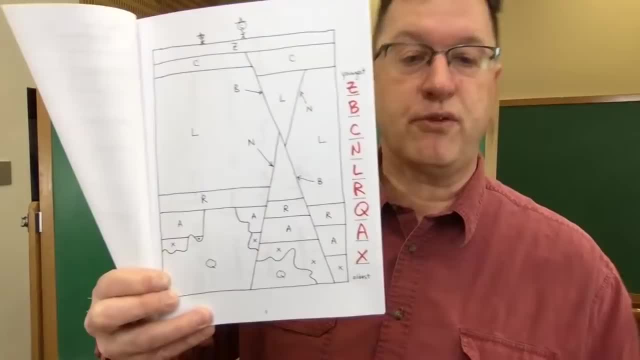 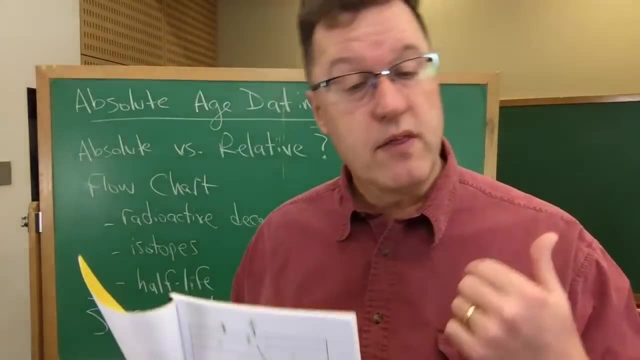 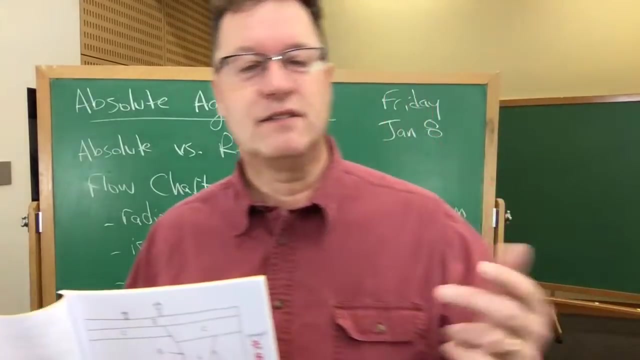 years old. this could be 700 million years ago. that fault could be 300 million years. we don't know. all we know from relative age dating using those three laws, remember them: superposition, original, horizontality, cross-cutting relations. i just got distracted because i noticed 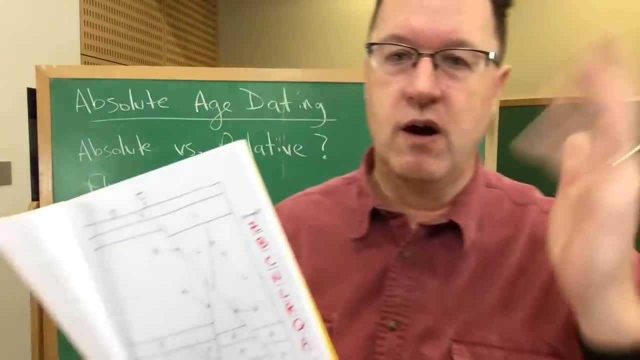 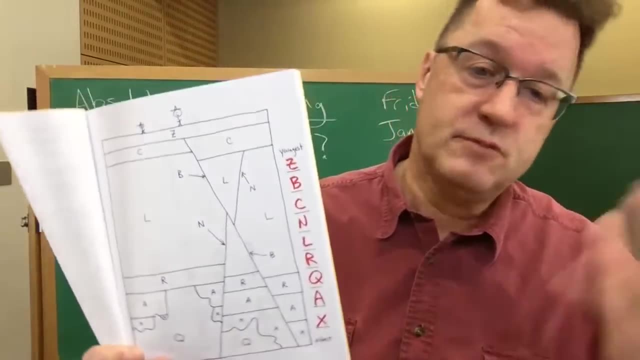 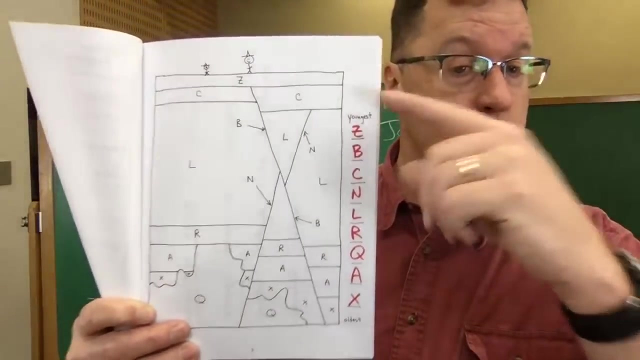 this weird lighting thing. again, i can't control this camera. many of you are bothered by that. i i can't control it. it's it's a camera built into this laptop. i don't know how to fix it, so we'll just have to run with it, so we know how to put things in order. that's what relative age dating is. that's. 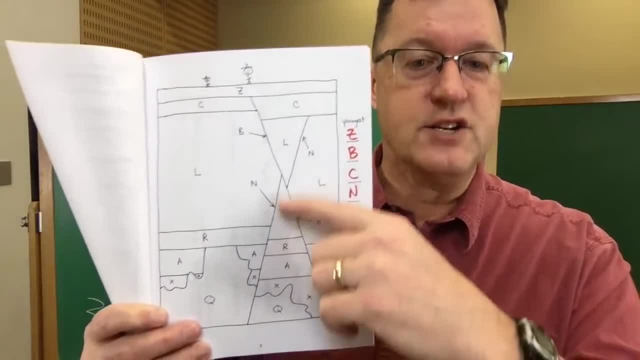 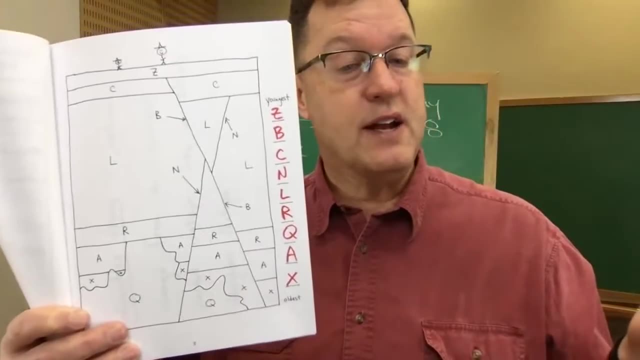 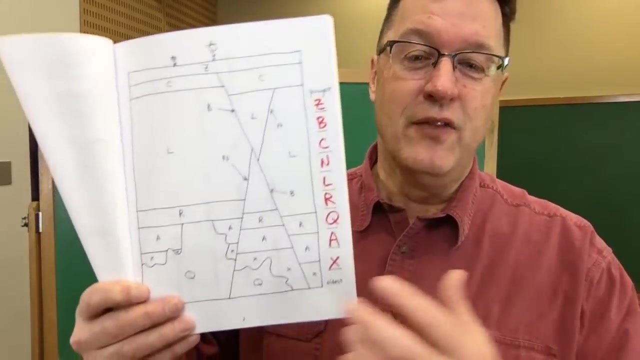 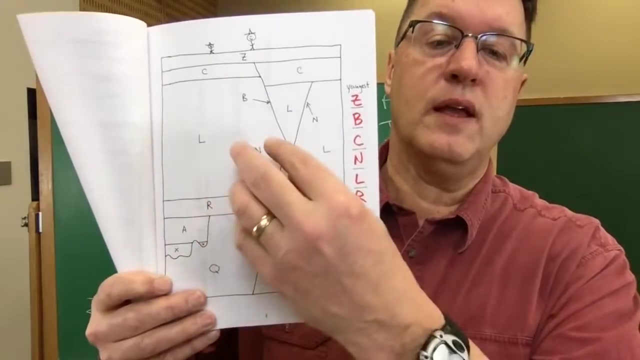 the only goal of relative age dating. what's the relative age of each of these things, each of these layers, each of these faults, this squirt of magma? they represent events, they represent stuff that went down long ago. they didn't all happen at the same time and, using those laws, we were able to put them in order chronologically, without knowing exactly. 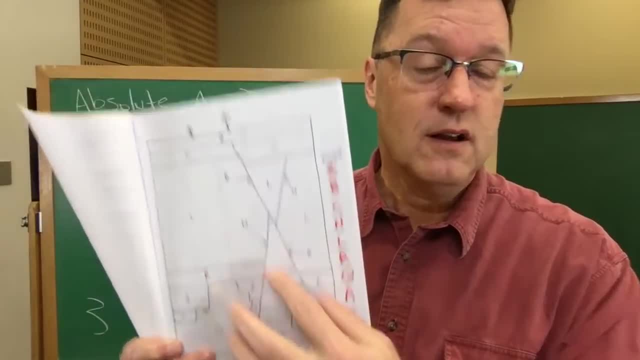 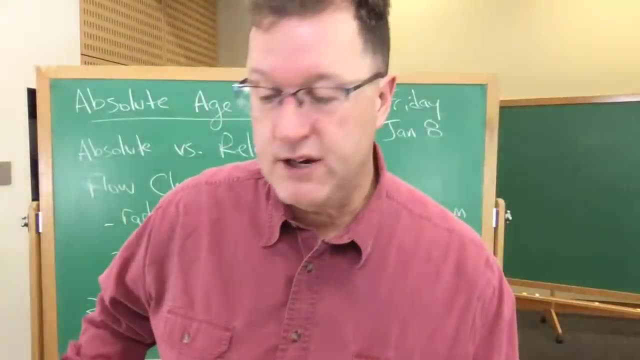 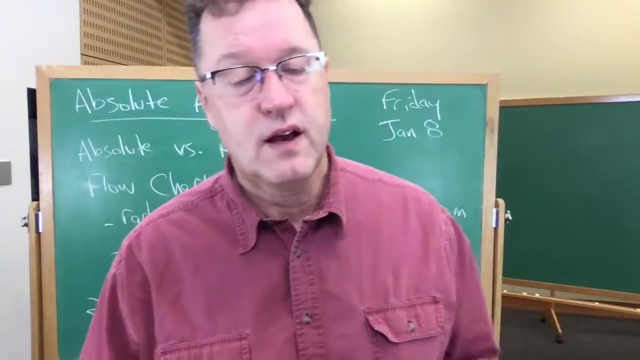 when it happened. so that's powerful. but we're going to do something different today. today, the only goal- and we are going to use the next three pages in the yellow book, the only goal today, it's one simple goal. it's one question: how do we know that this rock is 513 million years old? 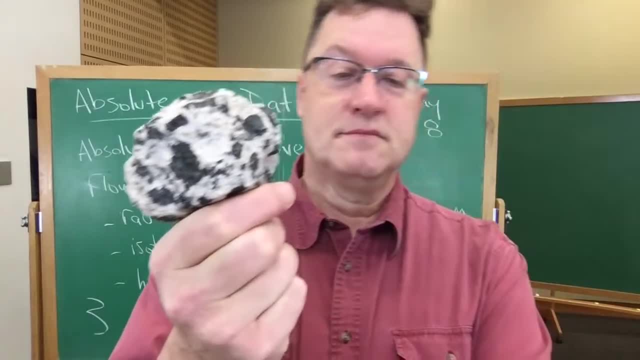 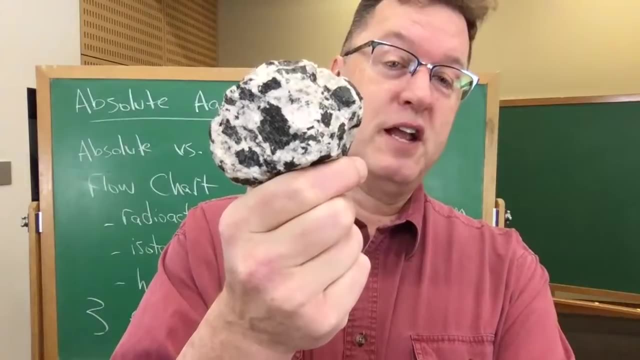 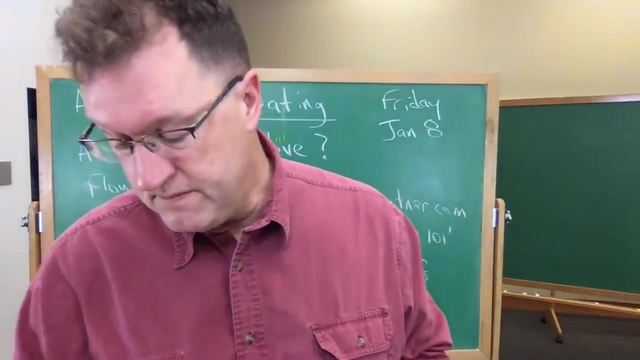 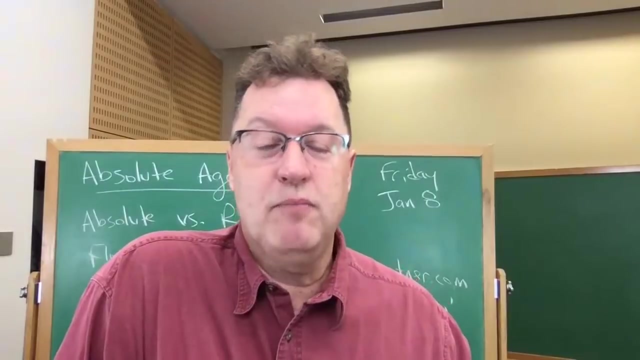 that's an absolute age. that's what we call an absolute age rock, 513 million years old. now, how do we come up with that? and obviously it's an important question and, as i've mentioned before, there's usually a bit of an attitude when you get question and answer after a public talk and 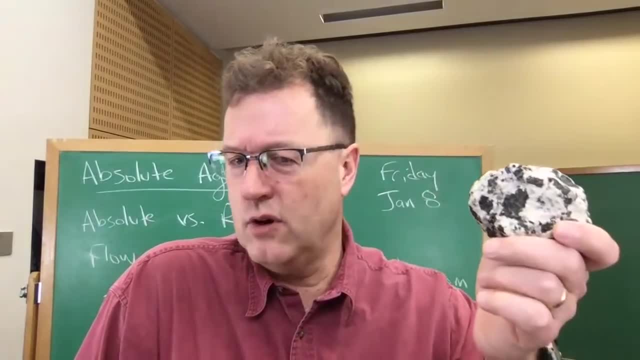 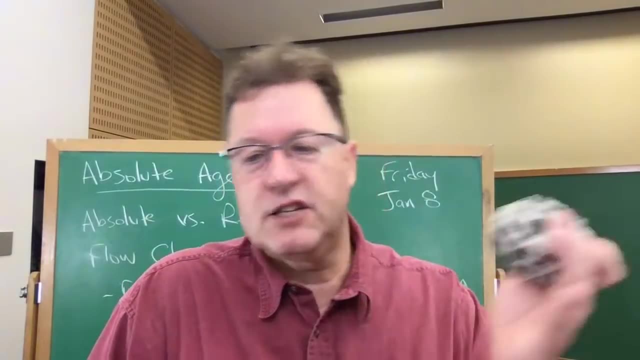 the attitude usually comes with this: how do we know those old ages subtext? i don't believe you. and then, of course, there's different ways to ask about climate change as well, and isn't that all a sham? so i'm experienced dealing with both of those topics and 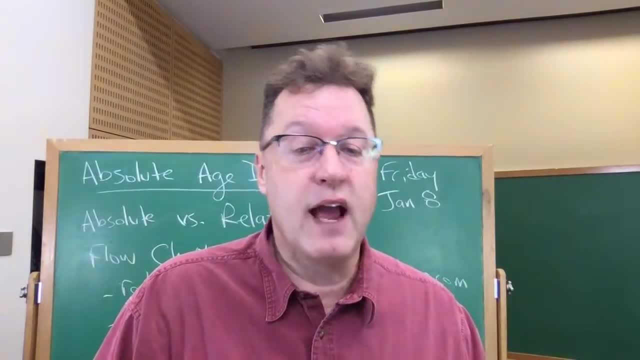 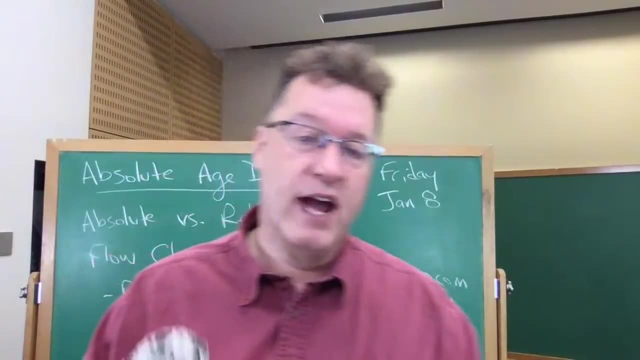 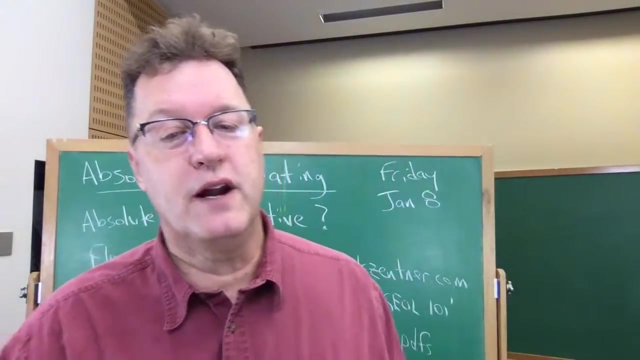 we'll try to you know in a measured way. talk about the data for both of those topics, and this is hot topic number one, of course. so in a public setting, i have kind of a two-minute answer to explain how we know the absolute age of this rock. well, you're not getting the two-minute answer. 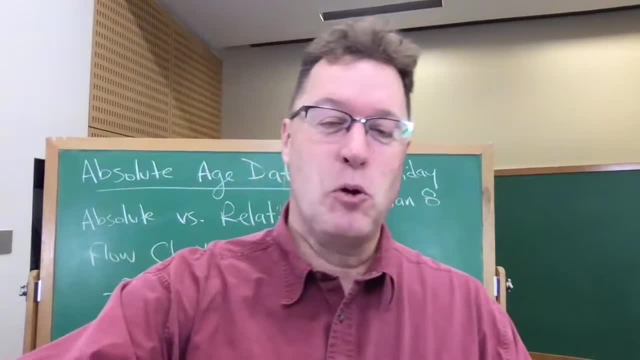 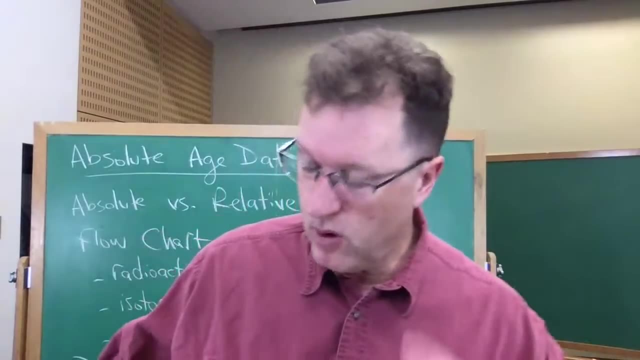 you're getting the 45-minute answer, okay. so it's one question and our game plan is on the board and i know you can't see the bottom of the board, but when i'm working with the board you'll see the bottom of it. you've already seen the bottom of it, okay. chalkboard police. okay, good. 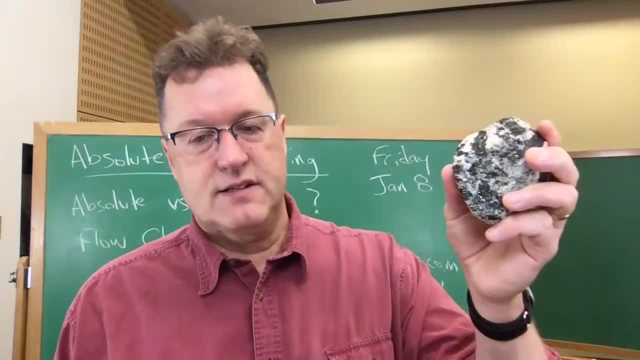 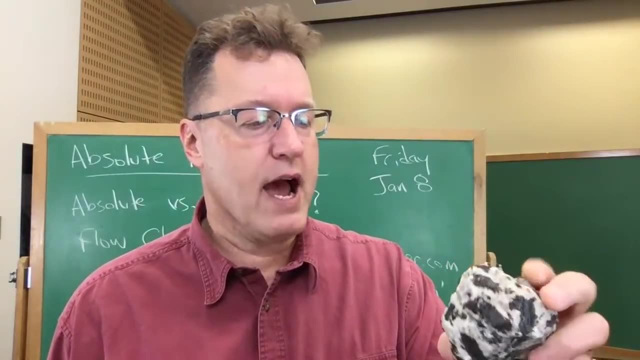 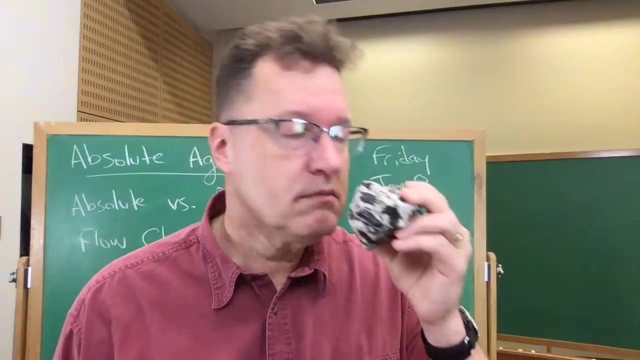 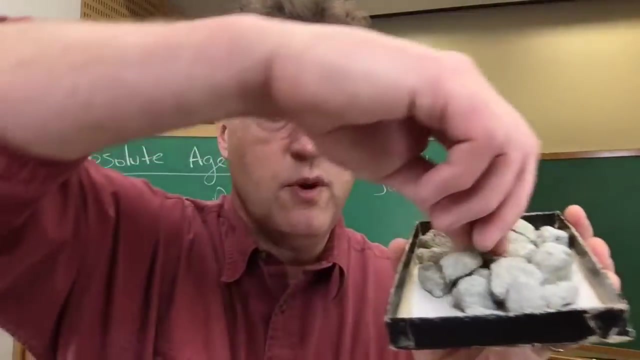 so what is the process? to come up with an absolute age like what you're supposed to like? look at it and go, i don't know. hmm, yeah, mesozoic or uh, you know, does does it work with, with all kinds of rocks? that's the first message. no, 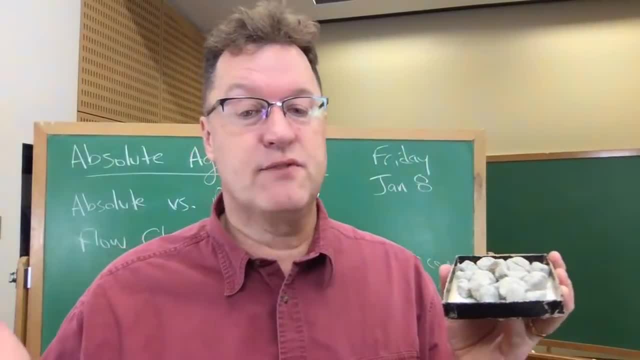 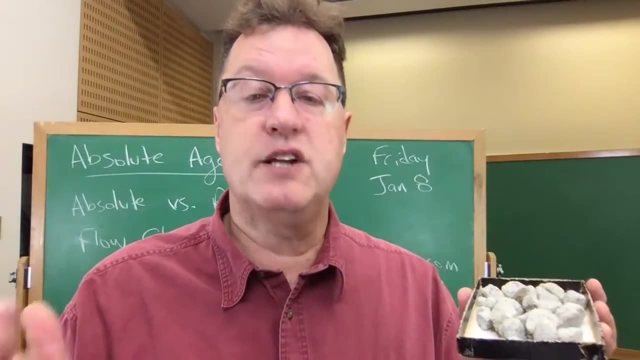 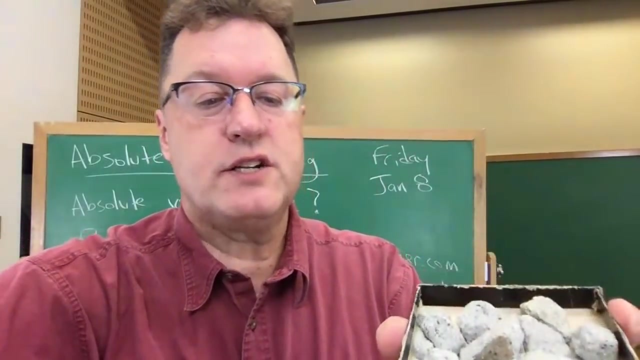 there are thousands of different kinds of rocks. there are many of those rocks that we cannot do this process. You cannot get an absolute age from every kind of rock. This is sedimentary rock. I don't want to make too much of a mess here because I'm on top of Craig's laptop, but this is sandstone, Can I? 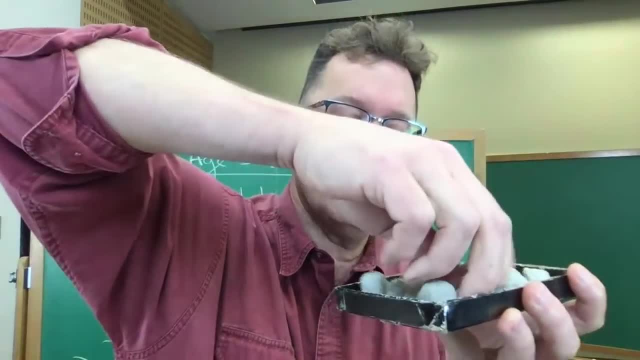 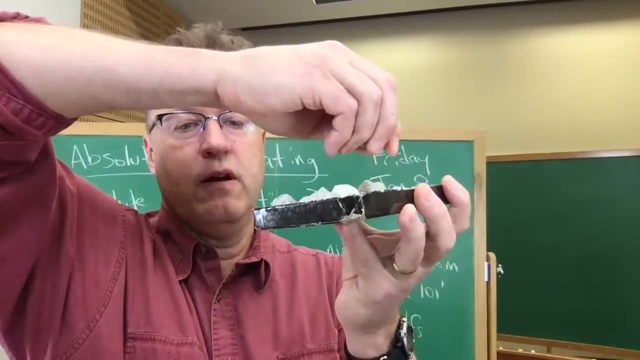 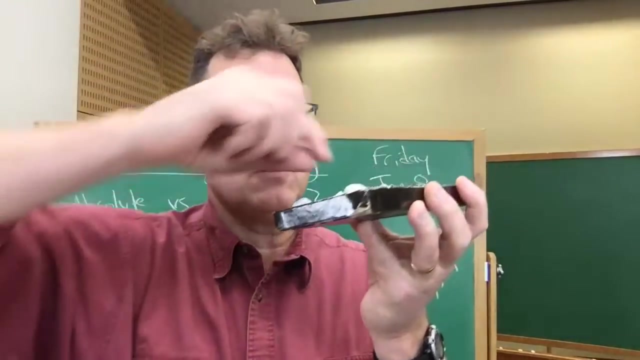 do this one-handed? Can I break an egg with one hand? Yeah, I can. Can you see that, Craig? I really don't want to screw up your computer. Hopefully you can see. I'm making a bunch of sawdust here. I'm breaking up grains of sand from these little clumps of sandstone. 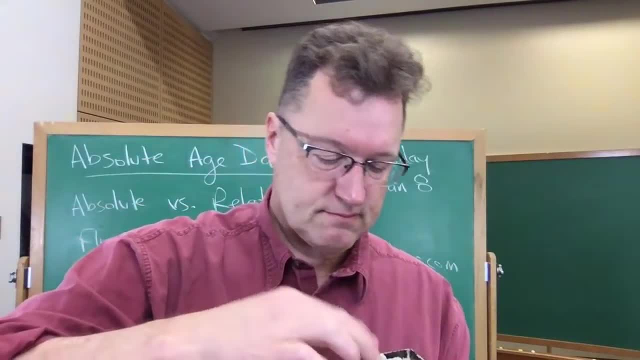 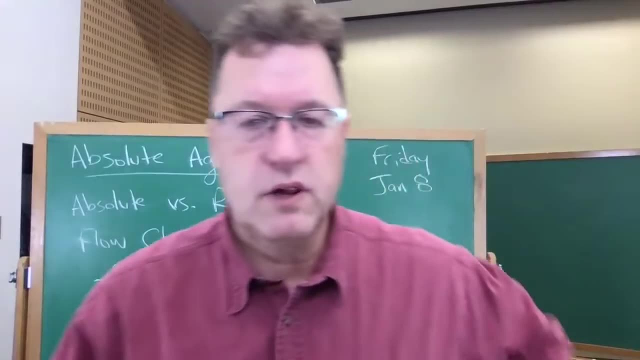 So every grain of sand? I really should have thought this through a little bit better. I can't show you that, I'll just give it to you verbally. You can't do this process today: absolute age dating with sandstone. You can't do this process today: absolute age dating with sandstone. 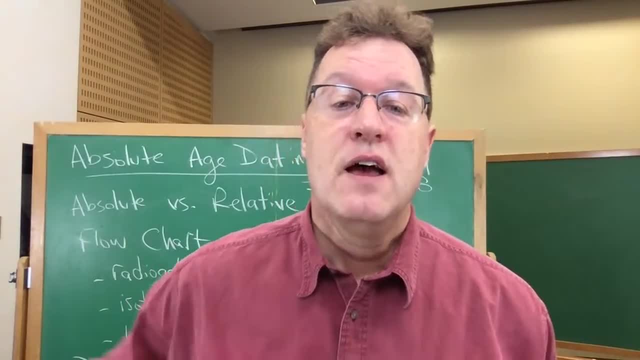 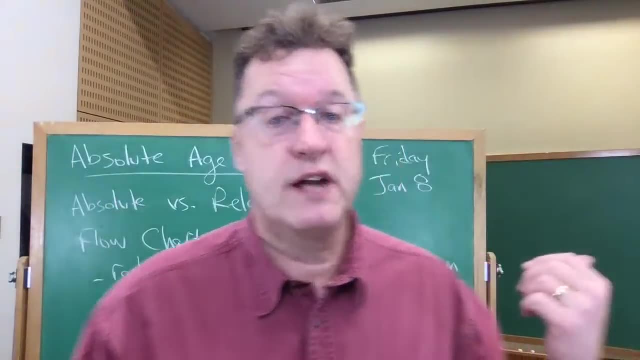 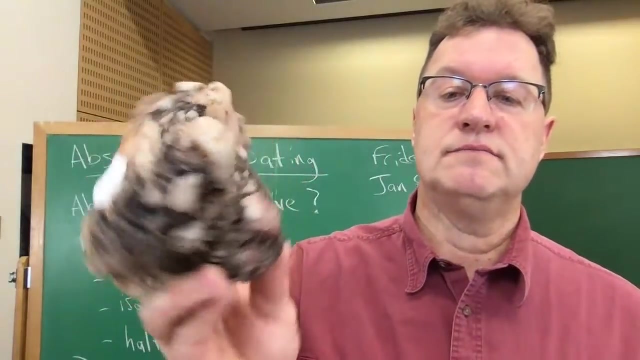 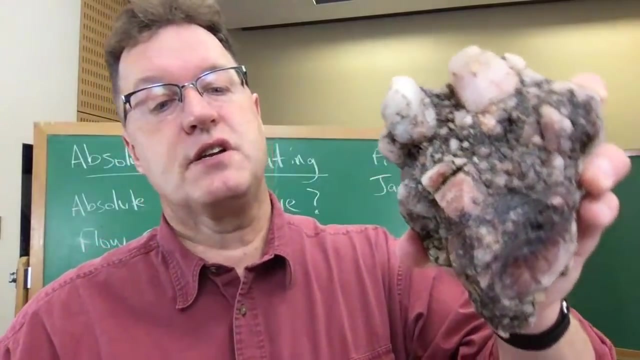 You just can't. A sedimentary rock is a bunch of fragments of other rocks that have been glued together- Sandstone, I just showed you. Let me show you another one. Here's a big old, beefy sedimentary rock. It's called a breccia, And each piece of material, each clast in this sedimentary rock is a. 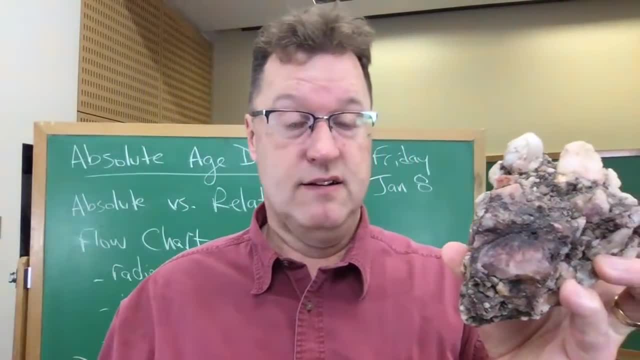 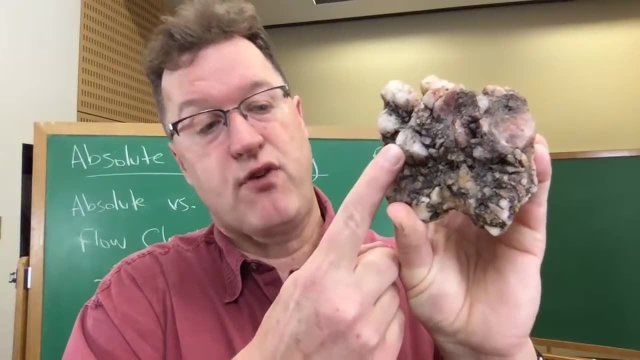 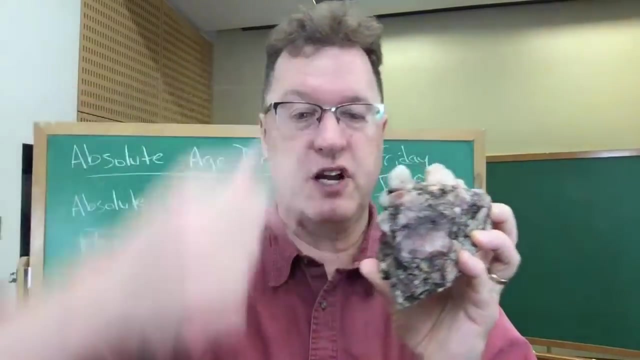 different fragment coming from a different area, And so if we analyze this clump right here, this clast, this piece, this fragment, and get an absolute age date for it, it's not going to be the age for the whole rock, because every piece is going to be different. This looks like it has. 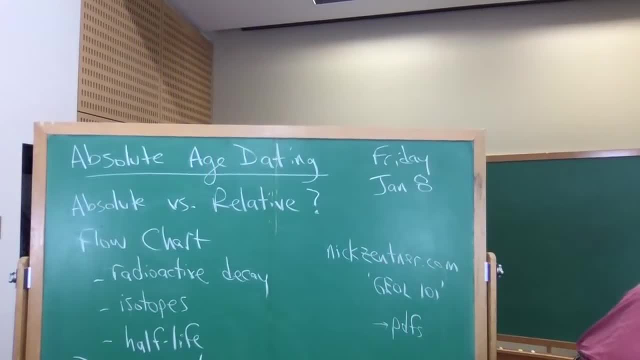 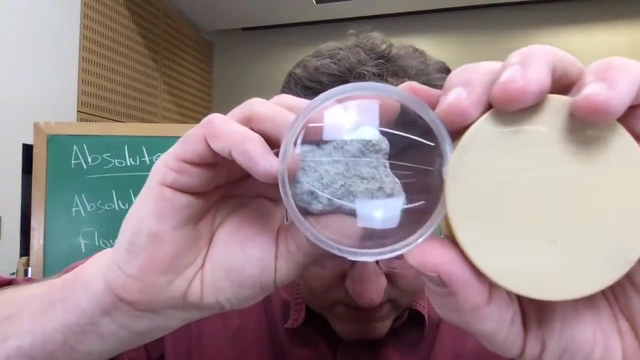 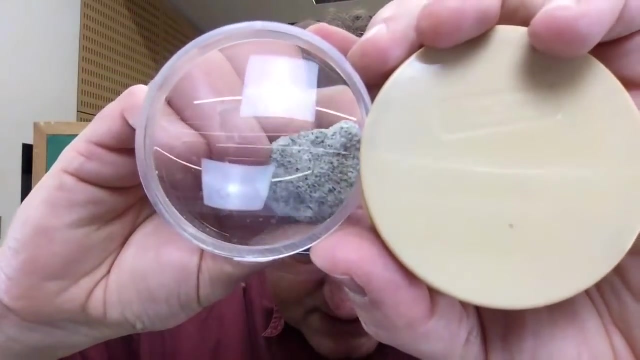 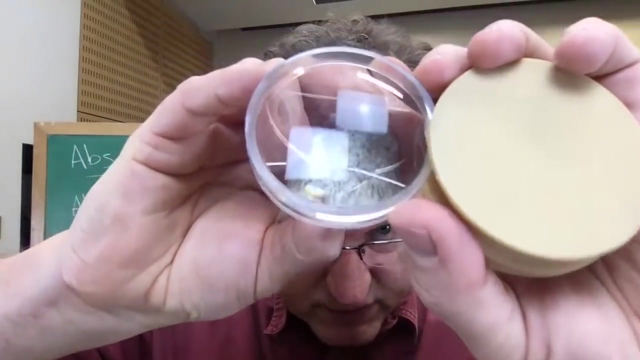 similar particles. I guess I'll just go back. This is sandstone again. Oh, this kind of works. So this is not a granite, This is a sandstone Again. I don't want to screw up the laptop, but I guess I've already showed you that I can get these into individual pieces. 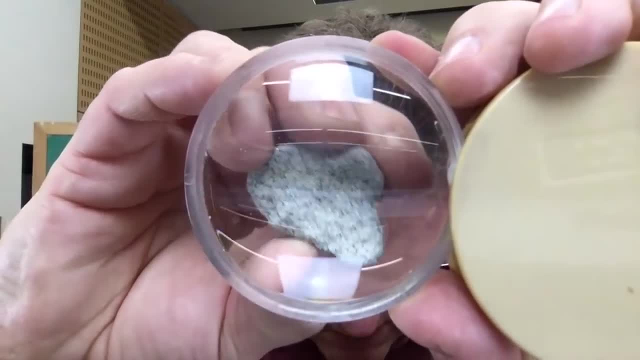 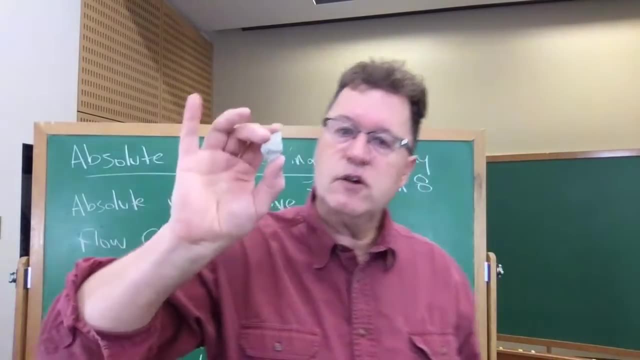 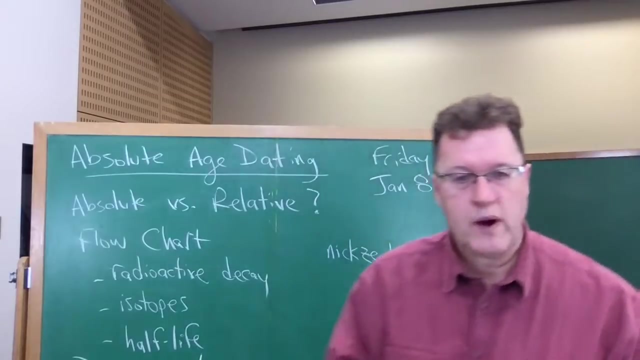 There. So there's a bunch of different fragments of clasts and each of those fragments is going to have a different age. So we can't do this absolute age dating with sedimentary rock. I think you're hearing me. So what is the process? Here's another collection of samples from the lab room. What is the process? 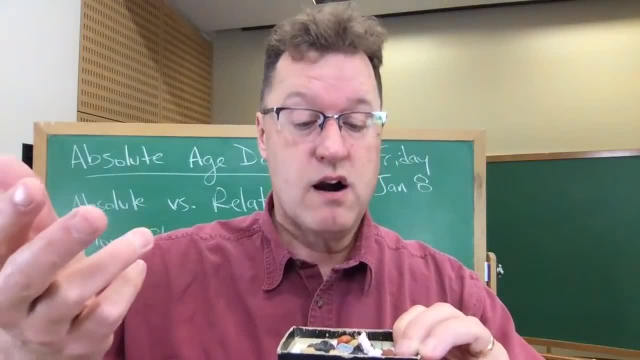 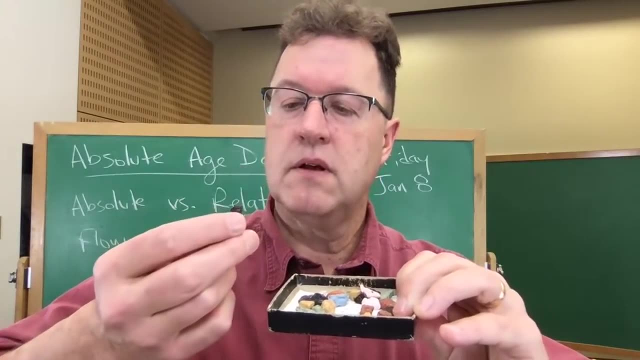 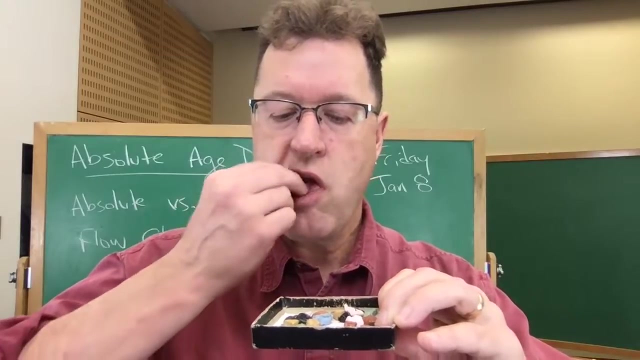 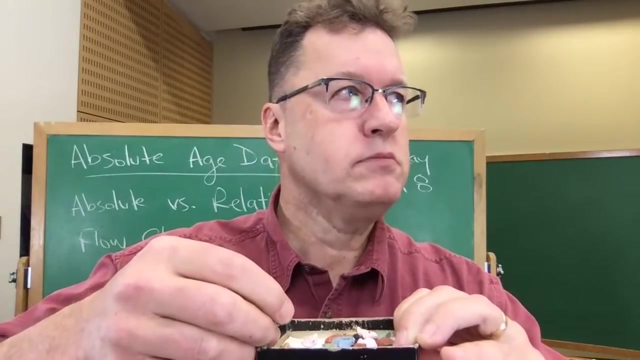 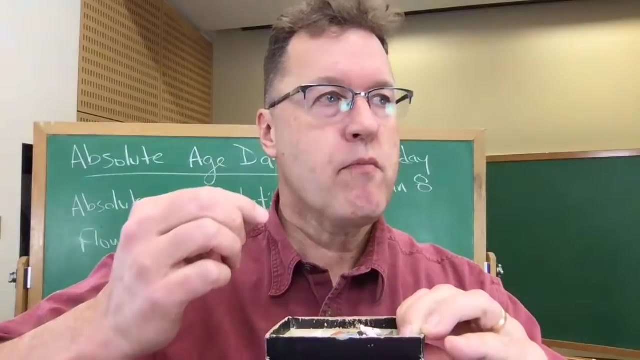 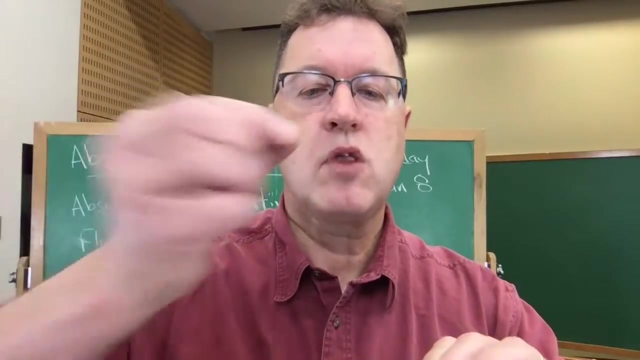 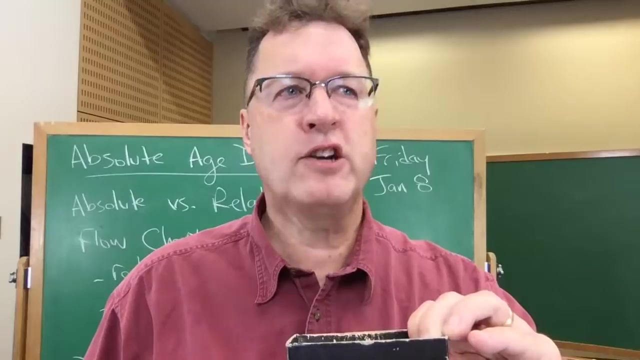 If this is igneous or metamorphic rocks, which are the kinds of rocks we need to do this process, what do we? 100 and absolute age Hold on? I can't do it. 112 million years, plus or minus 1.3 million years. 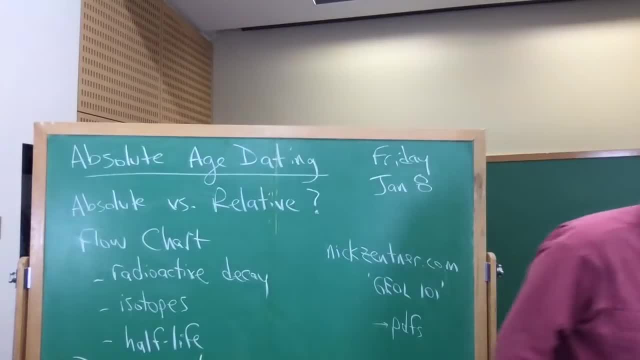 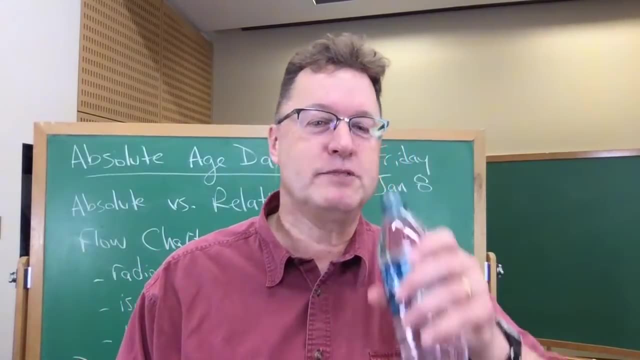 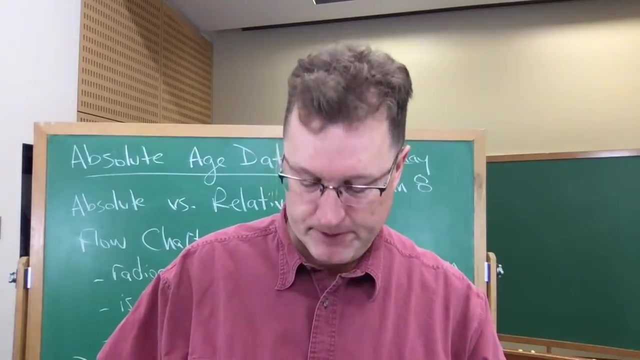 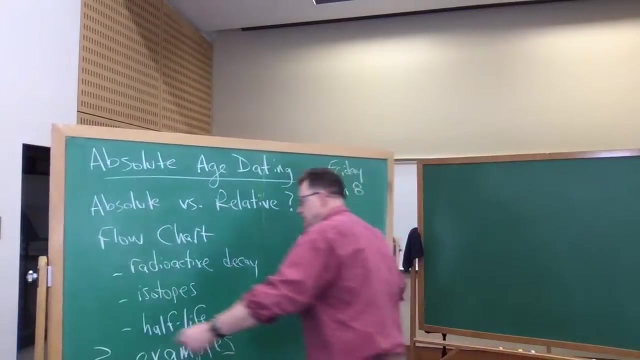 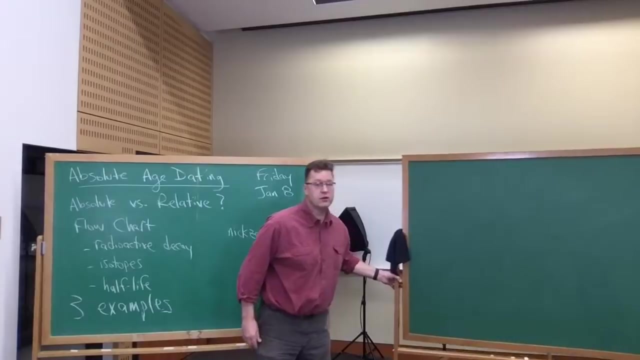 Okay, It's all showbiz. It's all showbiz, baby, Let's begin. Okay, Going away. Now, psych yourself up. This is going to be. I don't know How are you doing with this? I'm going to show you the tension span. 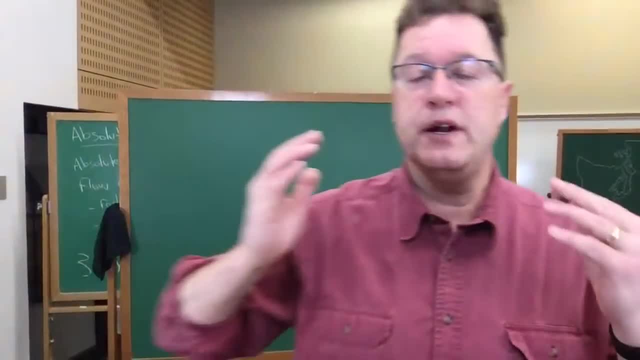 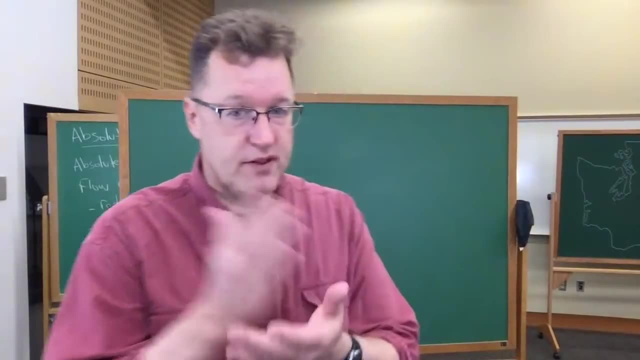 Because this is kind of one long answer to the question: how do we know the absolute age of certain igneous or metamorphic rocks? So try to stick with me this whole process. here We start with. I'm going to make a flow chart. 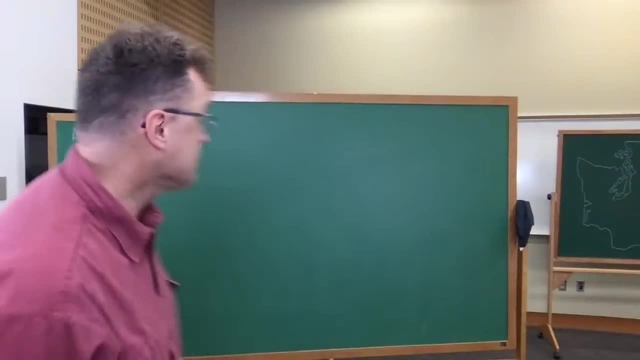 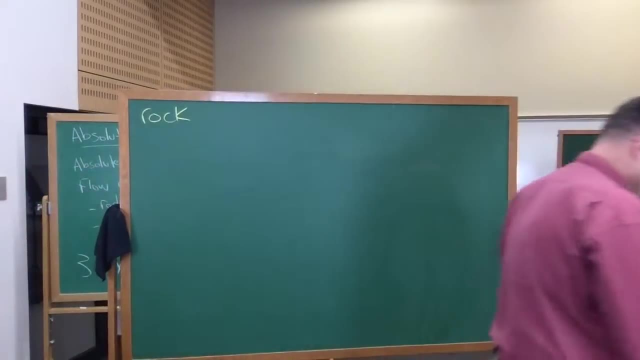 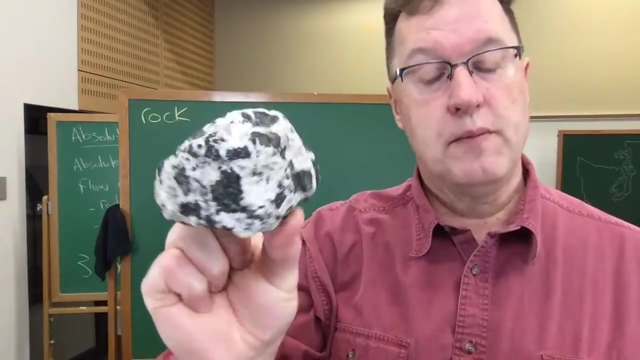 That's what I meant on the outline with flow chart. Okay, So we're going to start over here. We need a rock to get an absolute age from What is the absolute age of a rock. We could use this igneous rock that I shared with you a moment ago. 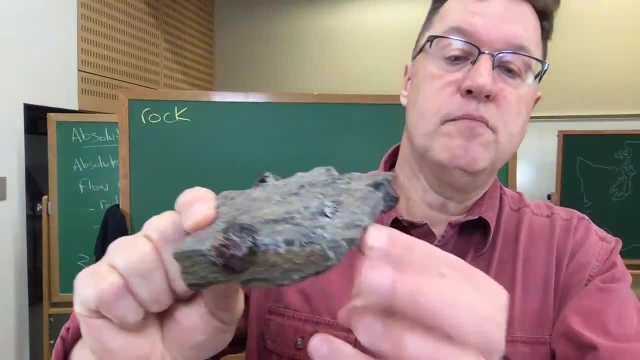 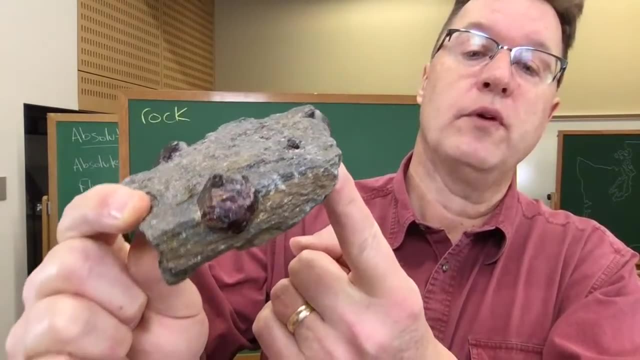 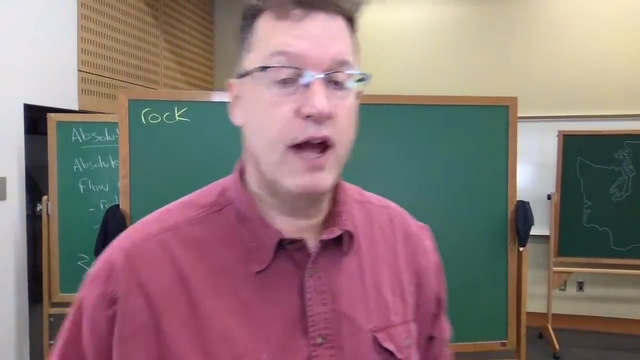 No, There are certain metamorphic rocks, like this favorite schist of mine that I've showed before in this live stream series, going back home with these beautiful garnets in them. So there are certain minerals in these rocks that we can use to absolute age date. 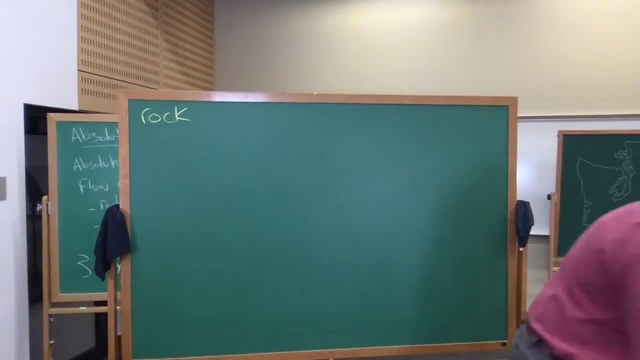 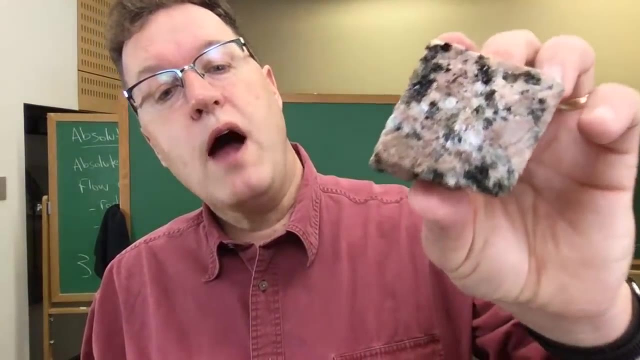 But that's the first major message. Okay, Rocks and minerals are not the same thing, young people. I'm holding a rock, but you can see that there are different colors. I don't even need the magnifying glass, You can see this pretty well. 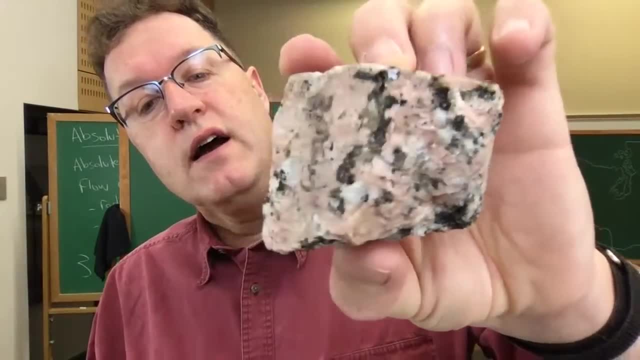 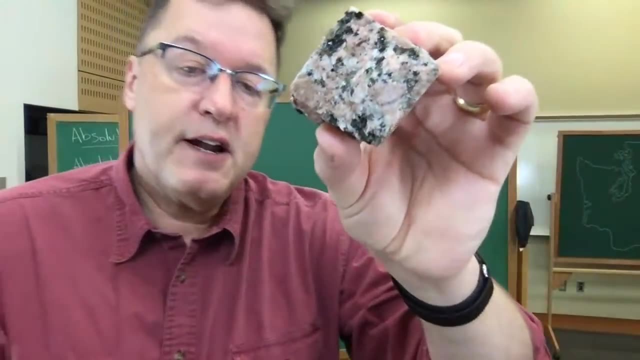 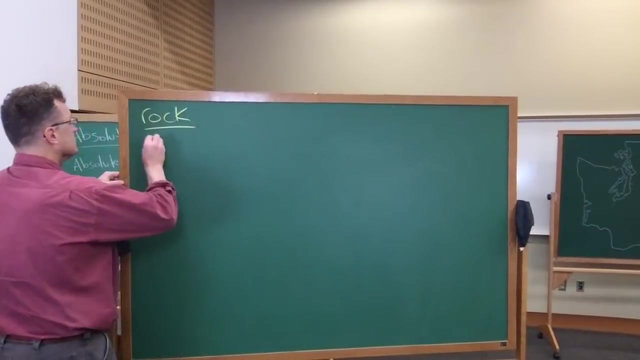 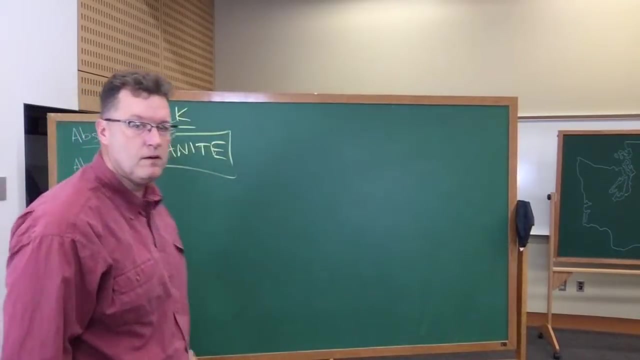 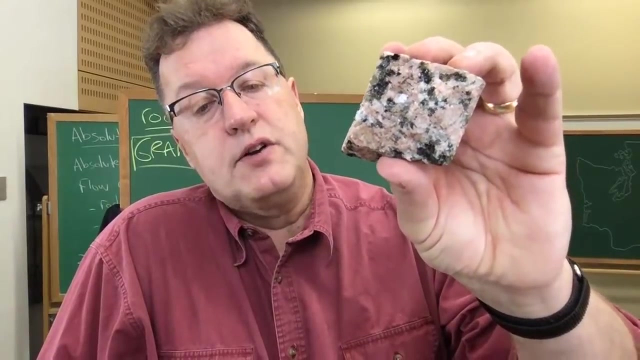 There are different colors inside of this rock And the different colors obviously this has been cut by a rock saw. the different colors are minerals. So let's get an absolute age for this igneous rock. This is called a granite, And I'm not saying this can only be done with granites, but I am going to use granite as our rock type to discuss with this process. 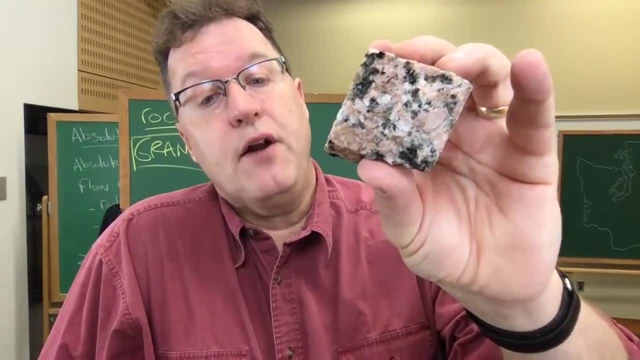 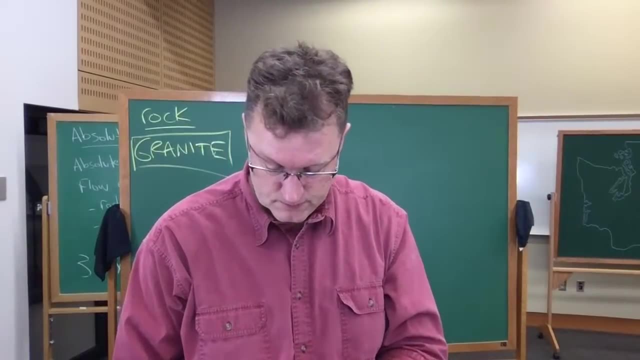 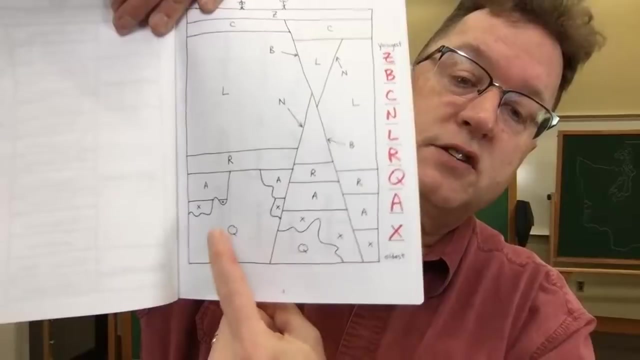 Good, Now the first step to get an absolute age from this granite. now, granite is just like Q, Do you remember Q? Huh, Yeah, Yeah, Yeah, Yeah, Yeah, Yeah. Q from yesterday was this liquid blob that cooled slowly underground. 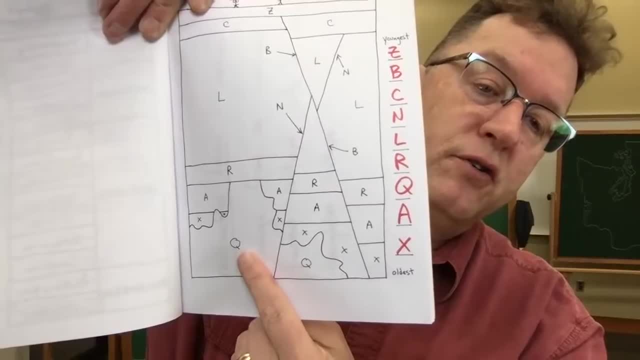 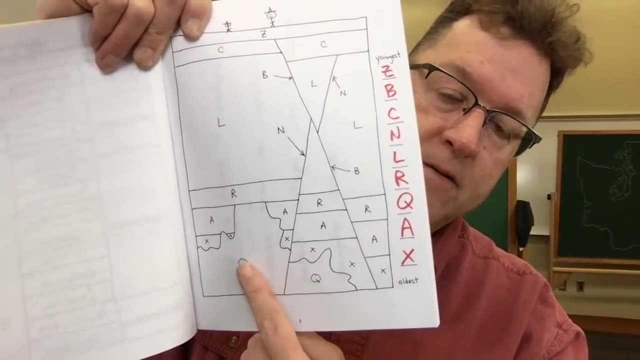 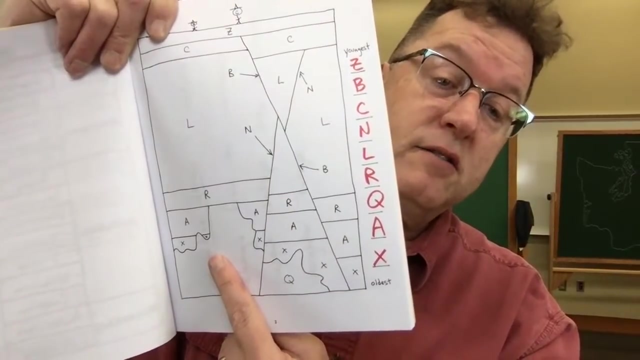 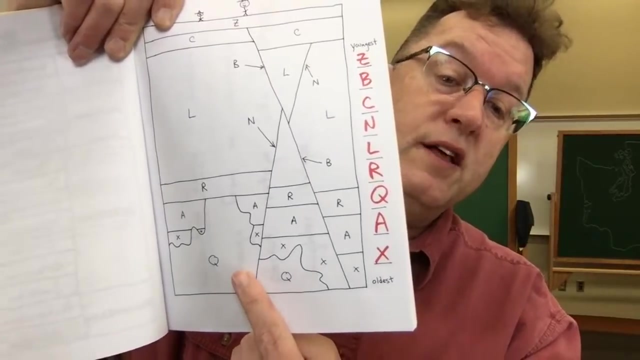 And that doesn't happen on a Tuesday afternoon, but it does happen within, you know, the same timeframe. So we can study the minerals in this cooling magma blob underground, do the absolute age date process that we're about to talk about and figure out exactly how many millions of years ago this Q liquid red hot blob cooled off and became a solid granite. 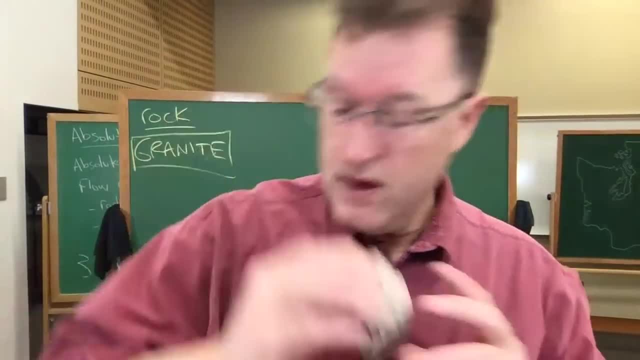 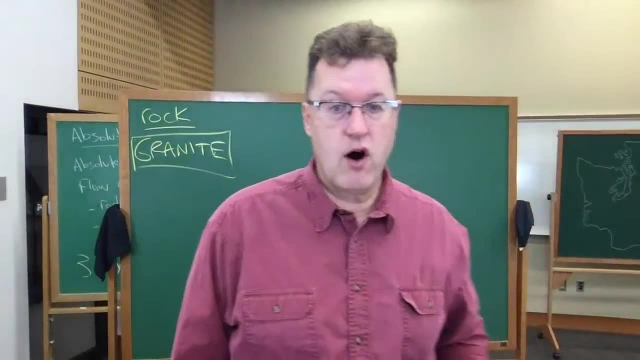 Okay, That's the context for this. Good, So to do this, we're actually going to take this rock and bust it up. We're going to go in a lab, down the hall, We're going to shut the door. We're going to put our earmuffs on. 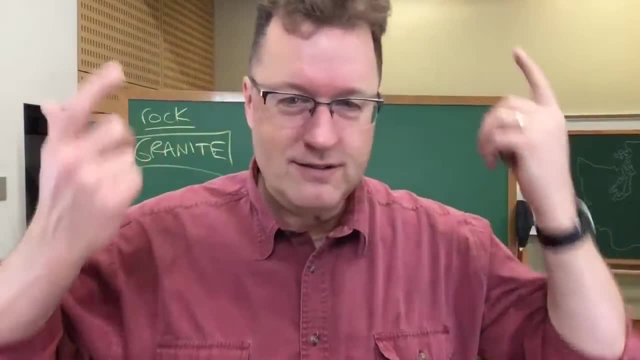 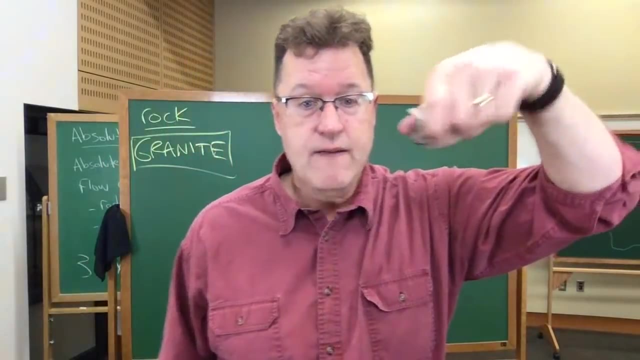 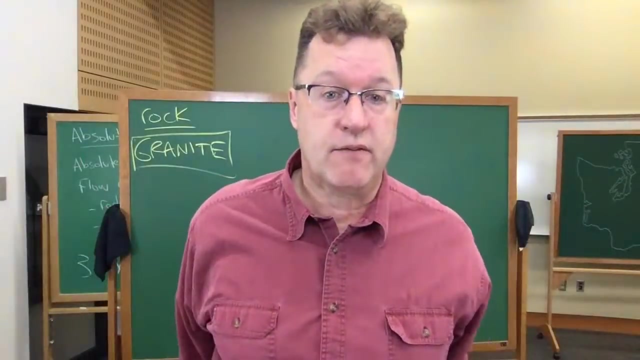 What do I call it Head Ear protection? I can't think of the phrase right now. We're going to physically put this thing in a chipmunk rock. chipmunk crusher- It's loud, man, It's loud. This is a fancy building. 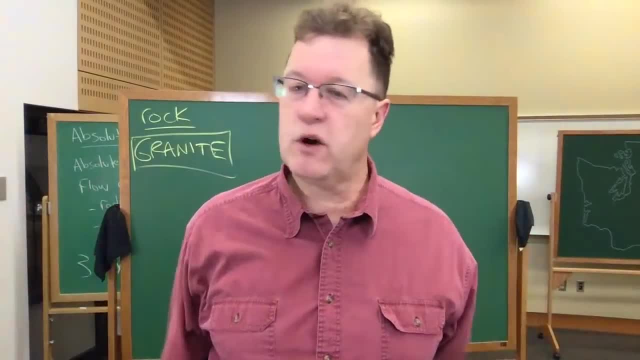 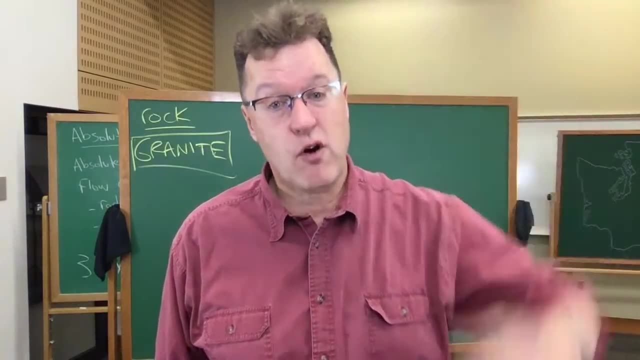 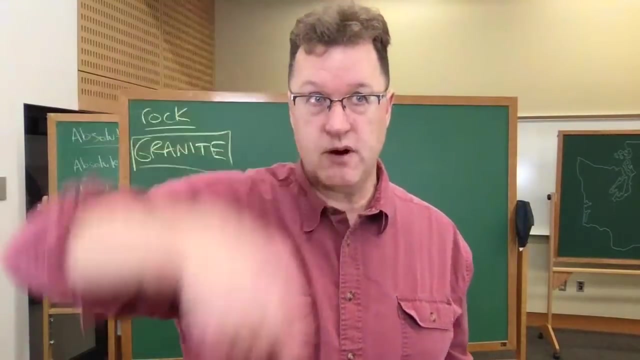 Taxpayers funded this beautiful building. We're grateful to everyone for funding this building And we have analytical equipment on all three floors in this building- Fancy equipment- And down the hall from my office right down here I'm pointing. behind you, on the first floor is a rock crushing lab. 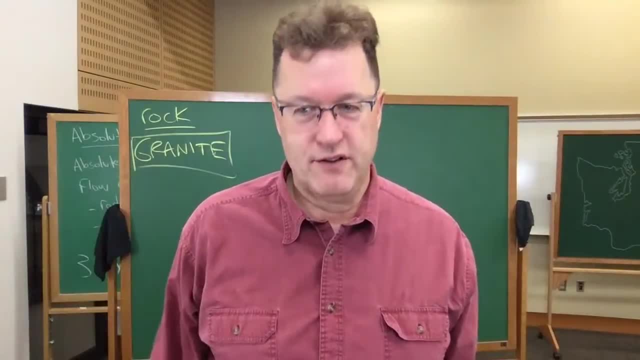 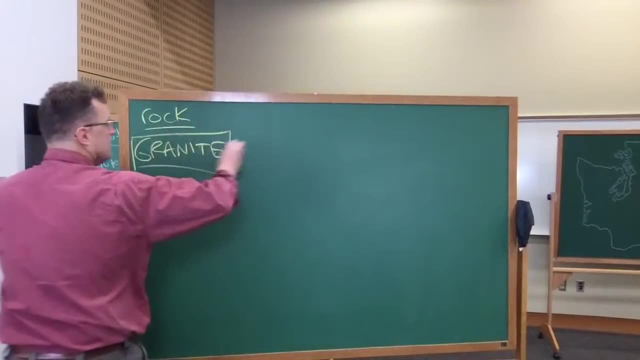 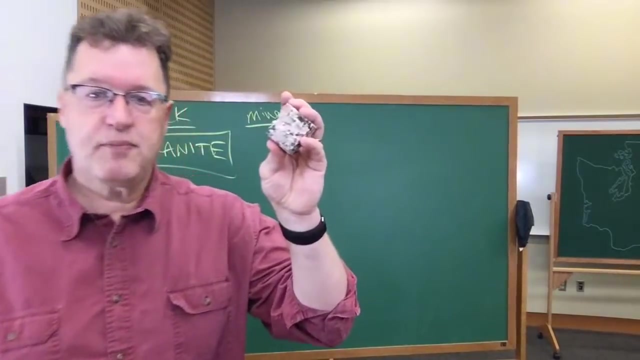 And it's so beautifully set up that I don't even hear them when they're in there crushing their samples. Chris Mattinson, Green Rocks guy. Okay, So we're going to separate, We're going to crush up the granite And free out. 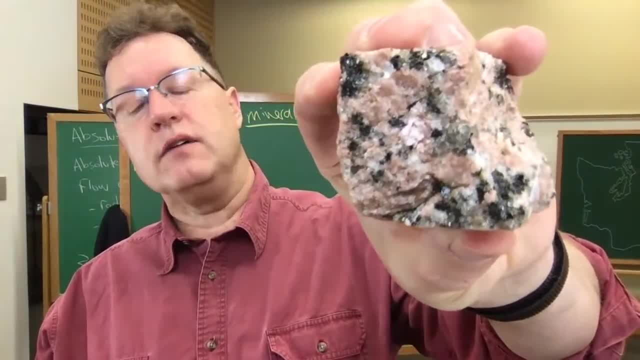 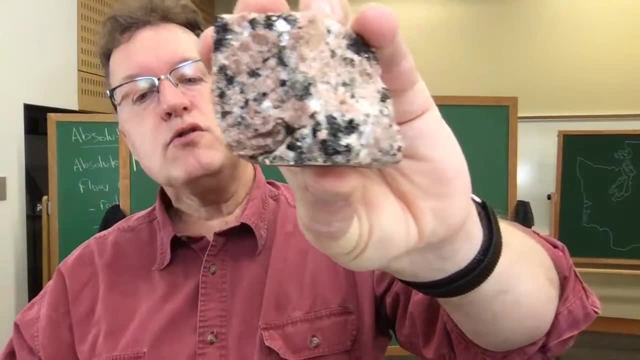 These individual magnets, Individual minerals that have been, you know, sitting next to each other. This is what they look like when they grew next to each other, When they crystallized in that cooling liquid blob in the dark, millions and millions of years ago. 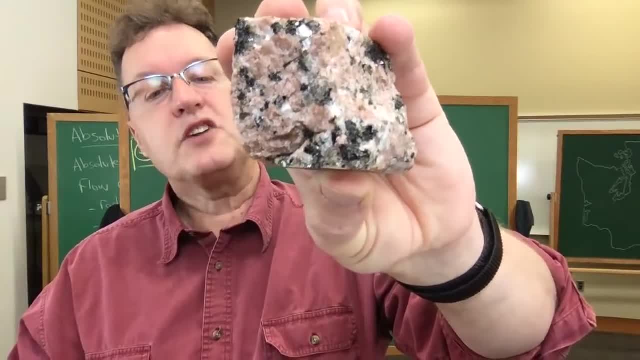 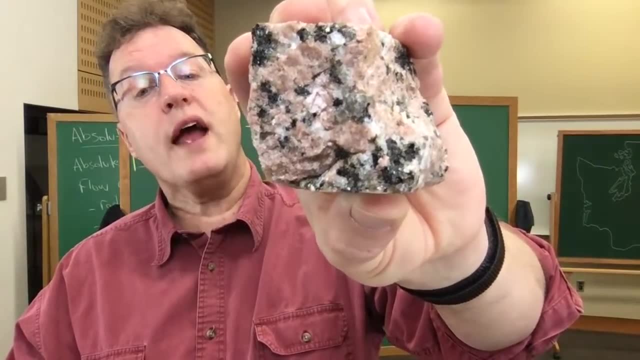 Well, we're going to free them up, We're going to separate the minerals. So there's some pink stuff in here, There's some black stuff in here And there's some gray stuff in here. There's a few other things. 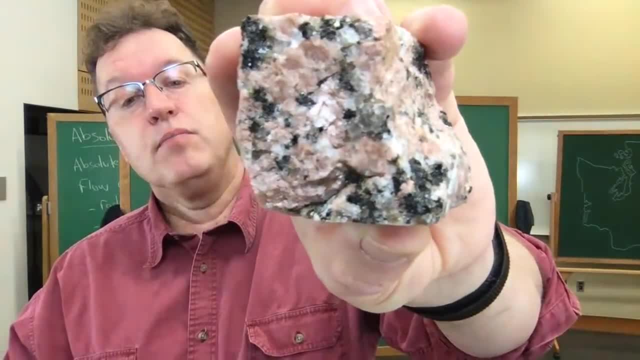 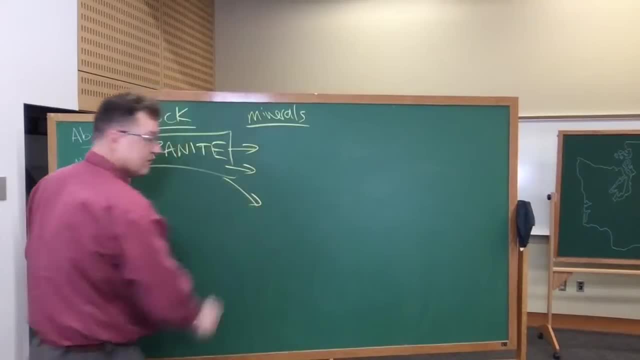 But let's just do that. Okay, Colored, You can see them: Black, Pink, Gray. Okay, So we're going to physically separate the granite into three piles of little pieces of things, Little minerals that are freed up from their neighbors. 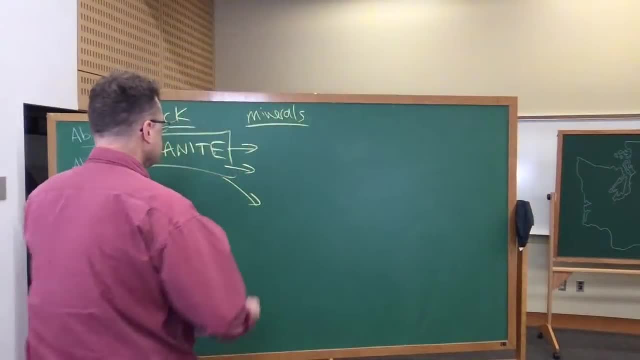 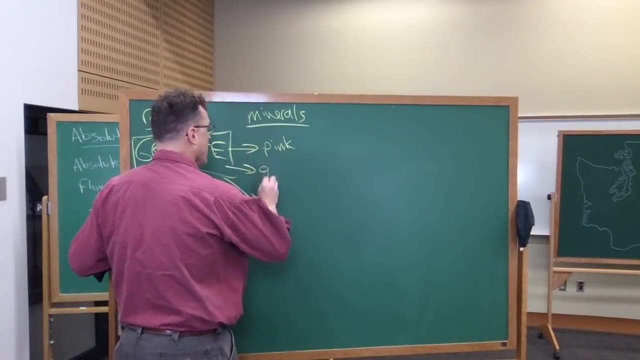 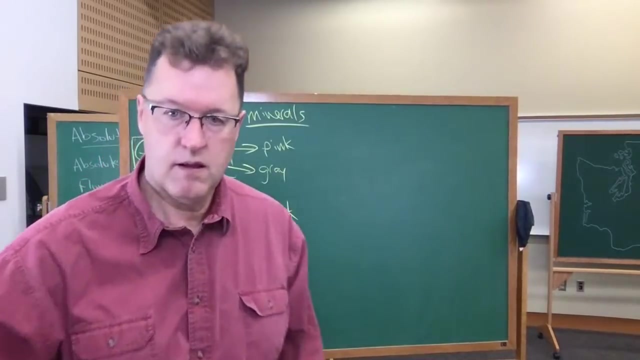 Mineral separation. We're going to separate the minerals, You got it. And we're going to have a pile of pink minerals, We're going to have a pile of gray minerals And we're going to have a pile of black minerals. They all crystallized at the same time, more or less. 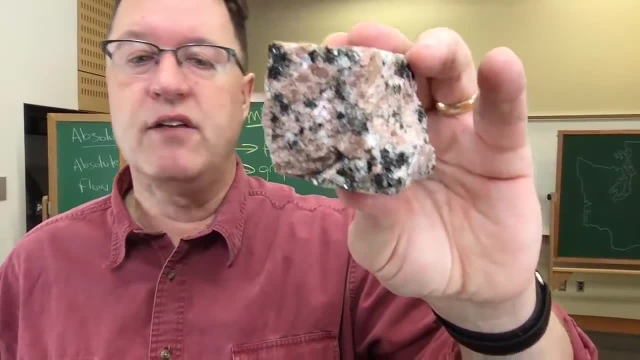 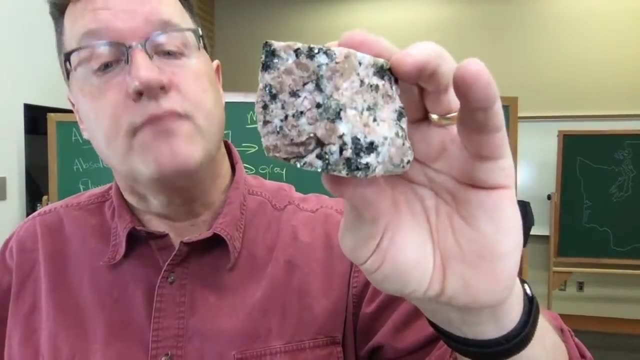 Within the error range that we're going to talk about today. they basically all formed at the same time. In the grand scheme of things, This is millions of years ago, So they essentially all solidified out of this magma at the same time. 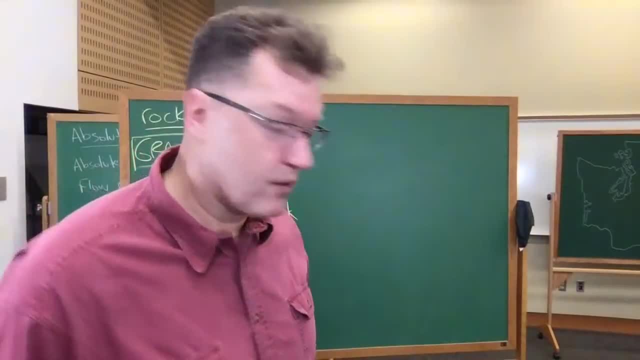 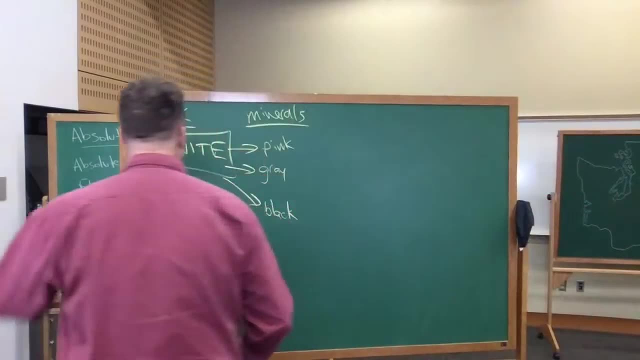 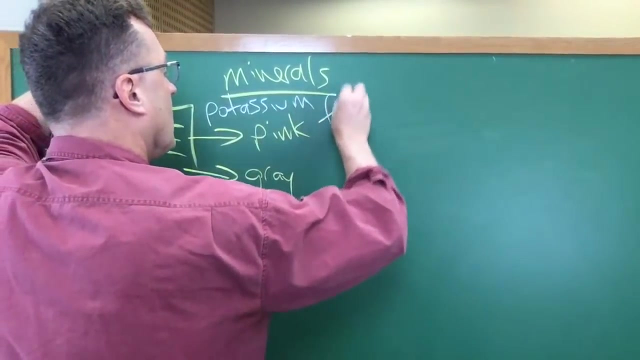 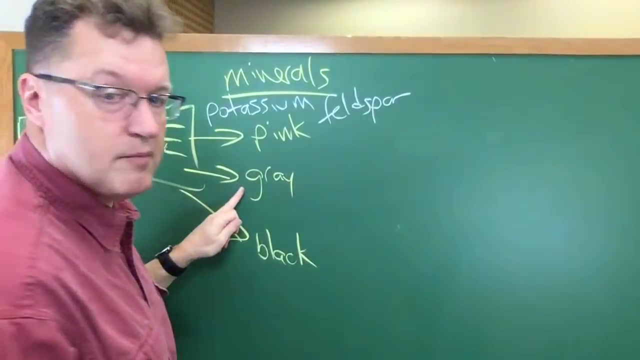 Okay, So we have names, of course, for these different minerals- The pink stuff. I'm going to write small for a little bit here. The pink minerals are called potassium feldspar. The gray minerals in that granite are called quartz. 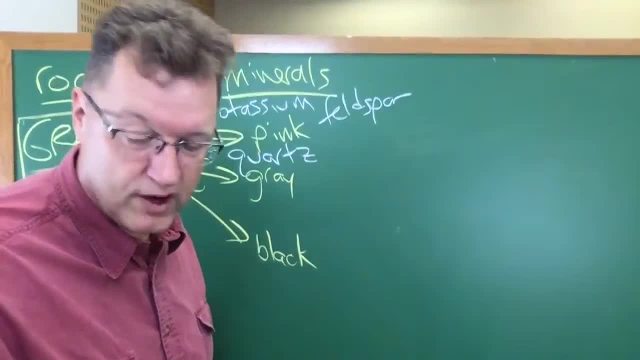 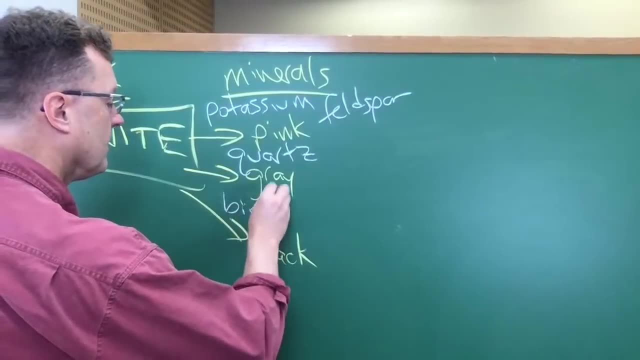 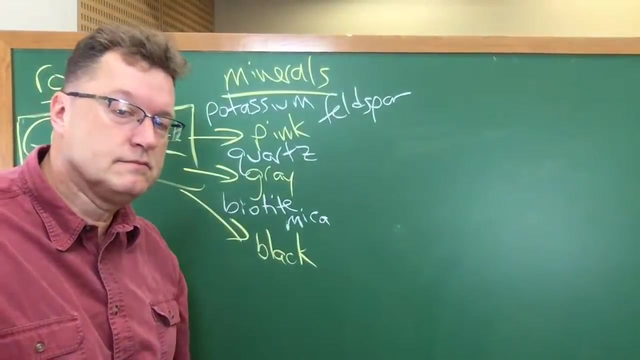 You're like: why don't you have the board this close the whole time? Because I'm pinned against the freaking bench right now, man, I can't even move. The black minerals are called biotite mica Drink. Okay. 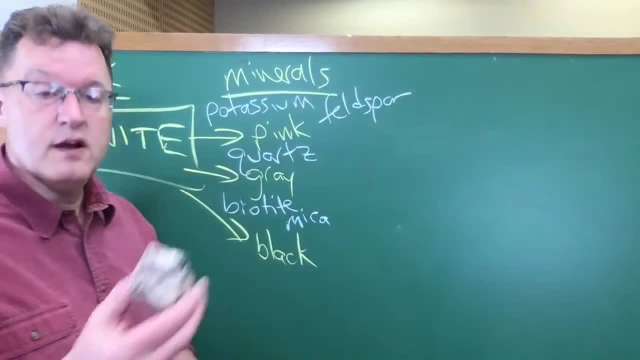 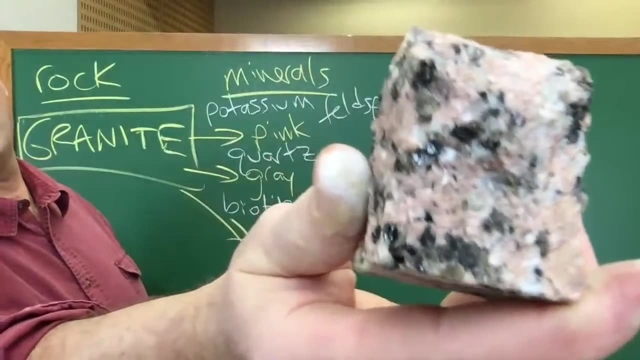 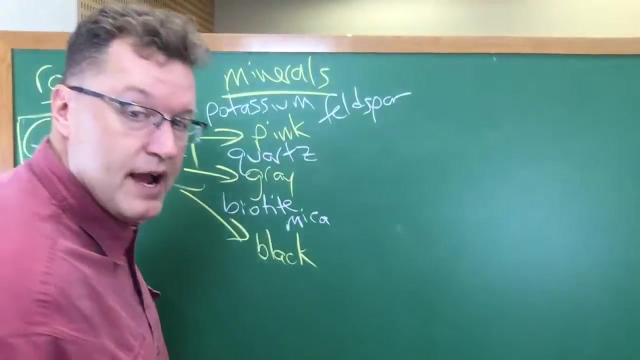 Pink minerals, gray minerals, black minerals: The pink ones are potassium feldspar, The black ones are biotite mica, The gray ones are smoky quartz. Okay, So we've got this granite broken out into essentially three piles of sawdust. 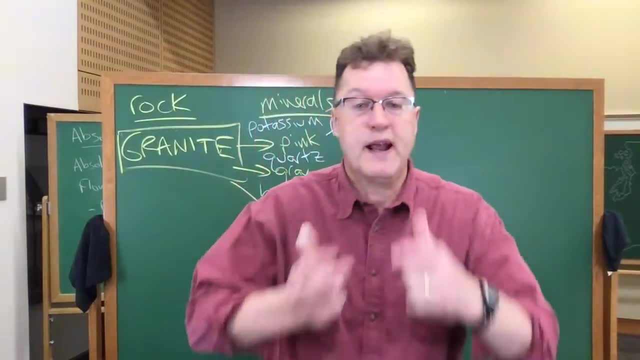 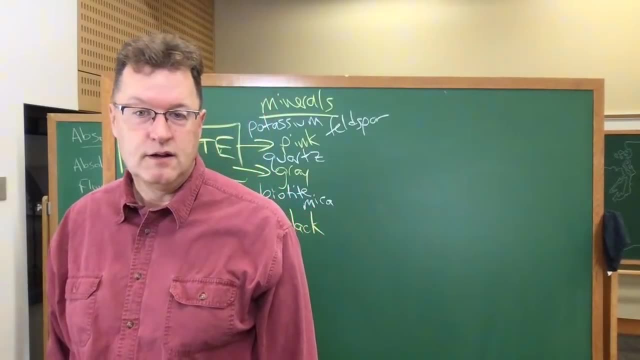 Pink sawdust, gray sawdust and black sawdust. We take all the pink sawdust, We bring it over to the waste paper basket. We throw it in the garbage. I always say that phrase and every student in the room looks up. 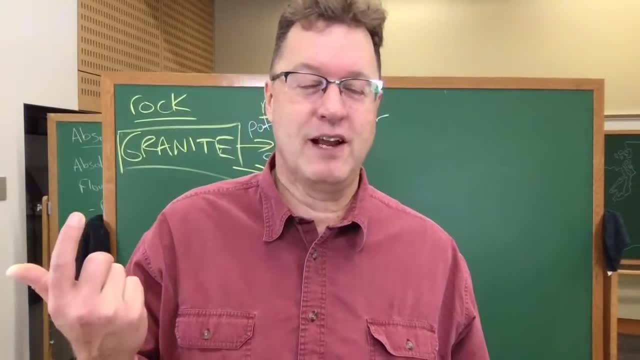 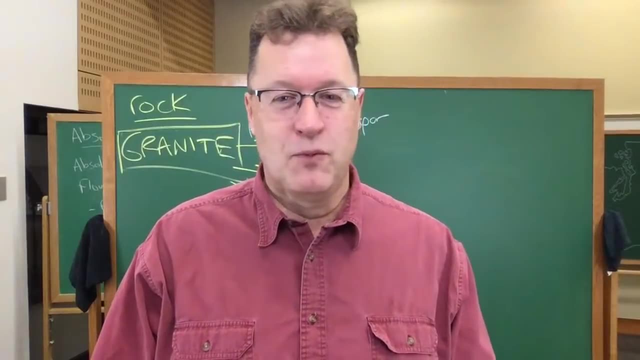 It's always fun You teach this. I've been giving this lecture for more than 30 years more or less, So it's fun that it doesn't matter who's in the room, what decade it is. There's just certain reactions to certain things that you say or do. 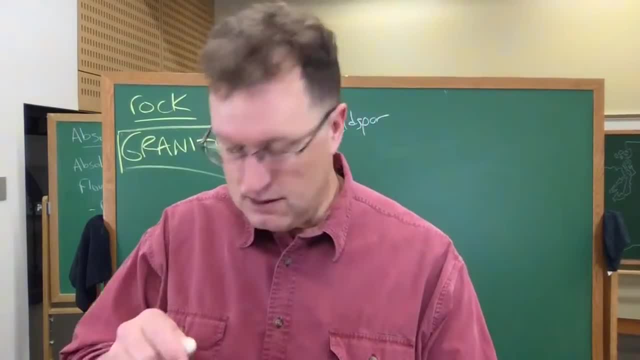 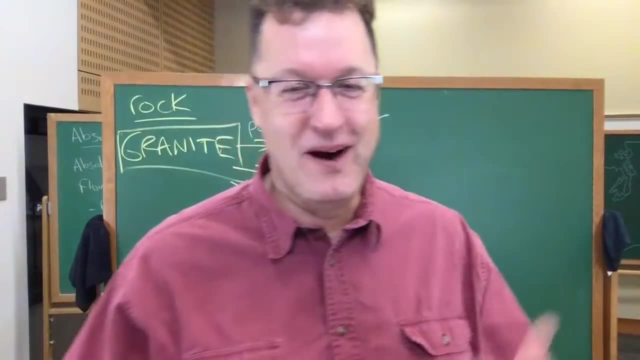 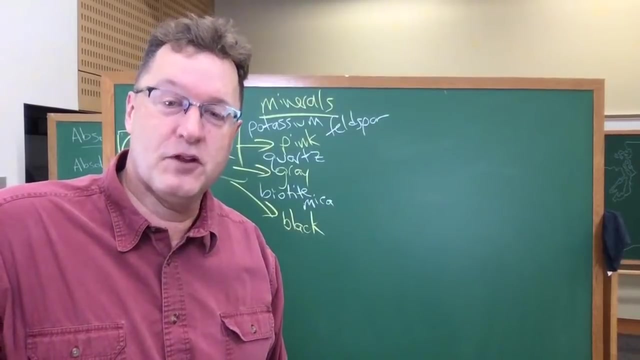 Throw it in the garbage. Huh, Back to writing. I don't know why I stopped and said that. All right, Wrong chemistry. We're not going to use the potassium feldspar. You'll see why. in a bit, The quartz, the mineral that you've heard of smoky quartz- not going to be helpful to us. 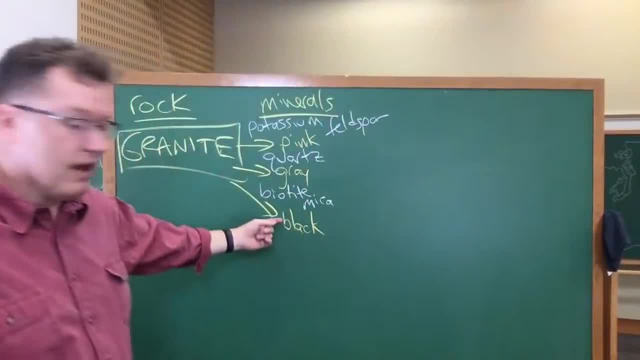 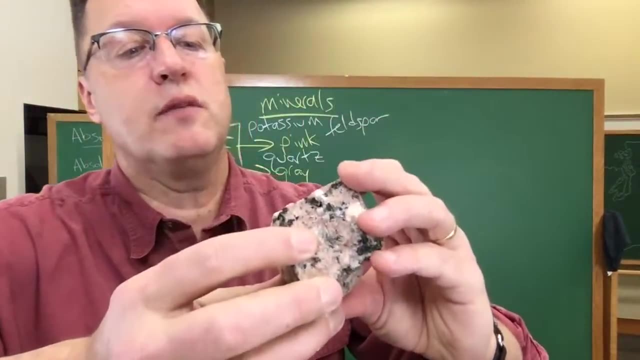 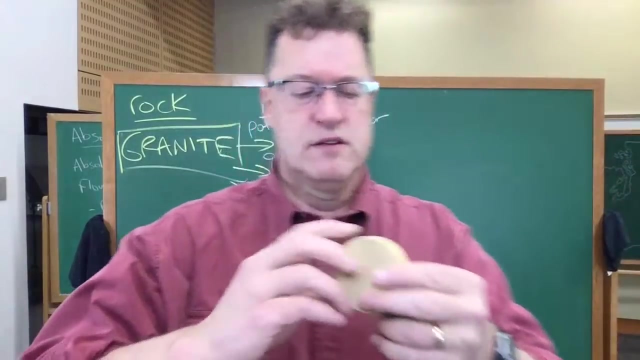 It's got the wrong chemistry Toss it. So now we're left with just the black biotite spars- And, by the way, can you see some of the black guys here? I don't know, Did that work? Somebody gave this to me and I kind of like it, but I always struggle opening it. 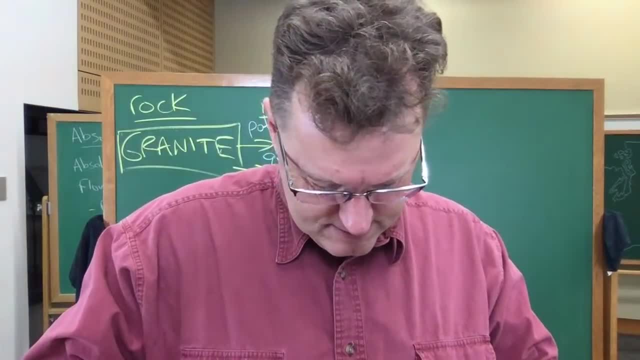 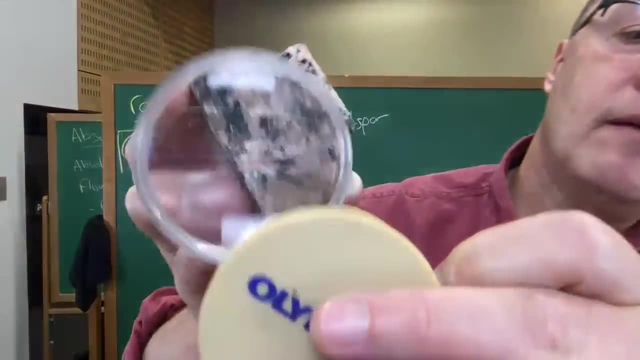 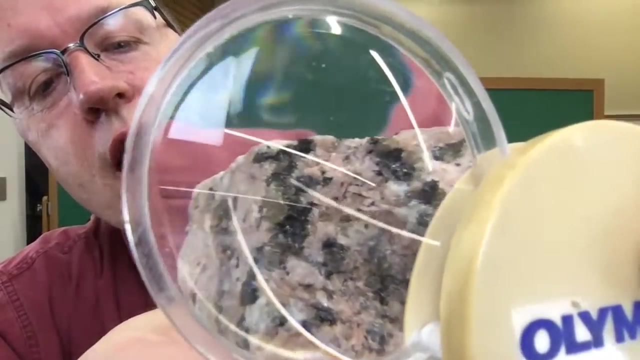 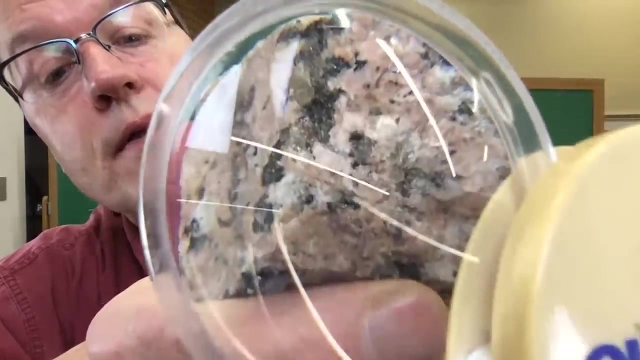 Oh, frick, Thank you. How much can I magnify here? There, That's pretty good. I want to show you these black guys. You see what I'm doing. I'm rotating the granite sample and I'm pointing out these. 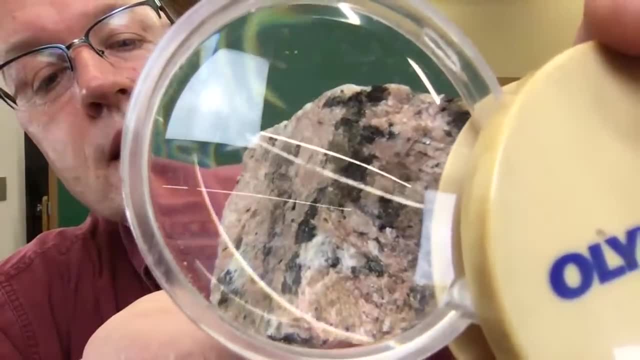 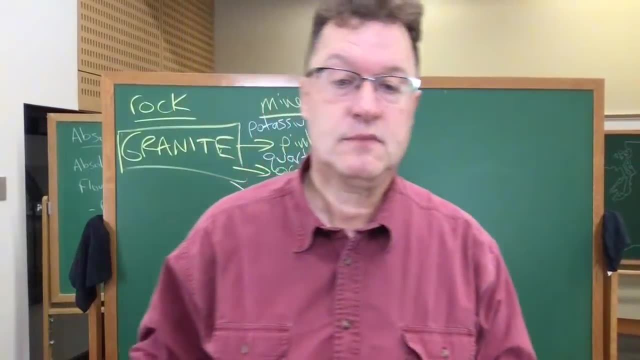 I'm looking at these black ones right here- Maybe you are too- And there's little flashes of light. Those are called cleavage planes on the minerals. Now you're taking geology 101 lab, so you'll see all this stuff in the flesh. 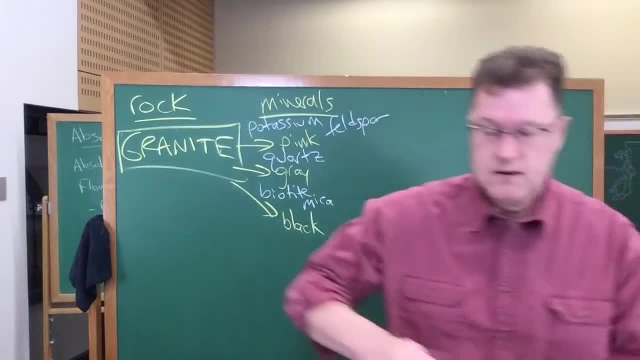 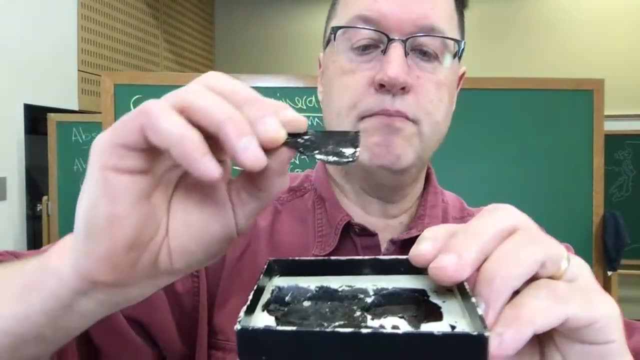 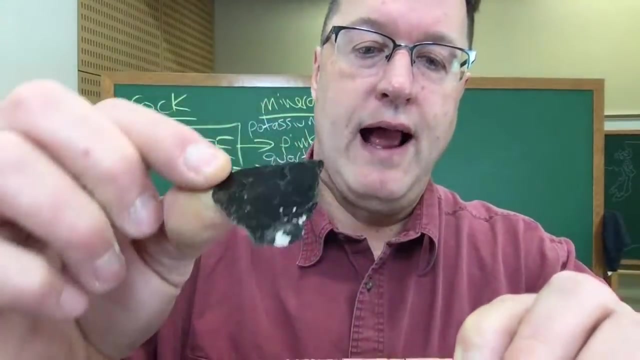 You'll see these biotite mica flakes. These are some minerals that have grown. Excuse me, These are some black biotite minerals that have grown bigger than these little guys And you're like: how does this happen? How do you make this in Mother Nature? 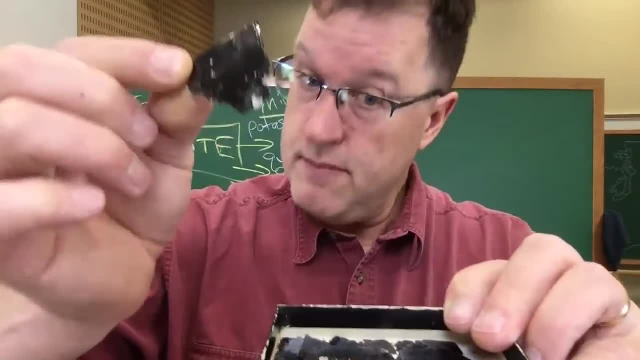 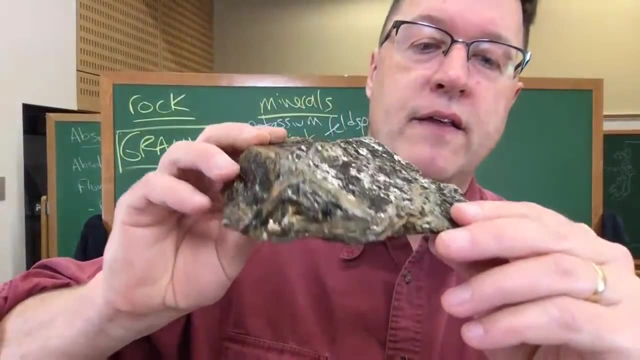 And you're like: well, we found these. These are minerals. now, It's not a rock, right, This is biotite mica Drink. We found that mica in these things called books. I've never found a place. 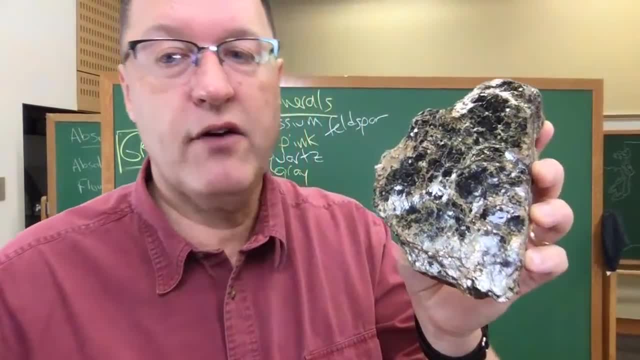 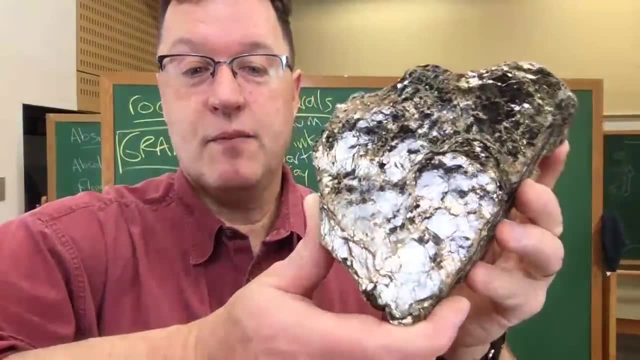 I've never been to a place. Has anybody here in the townie community, has anybody been to a place- in the mountains, let's say, where there are books of mica like this? This is not a rock. This is a bunch of biotite mica that has grown next to each other. 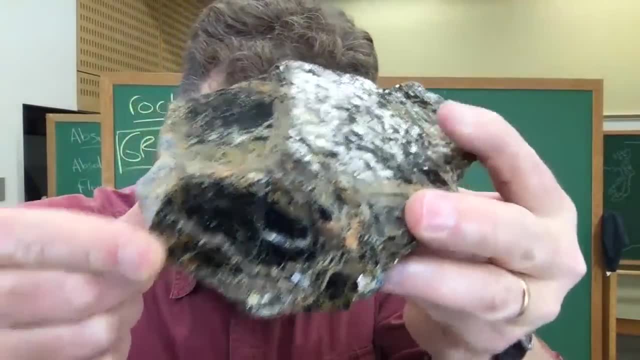 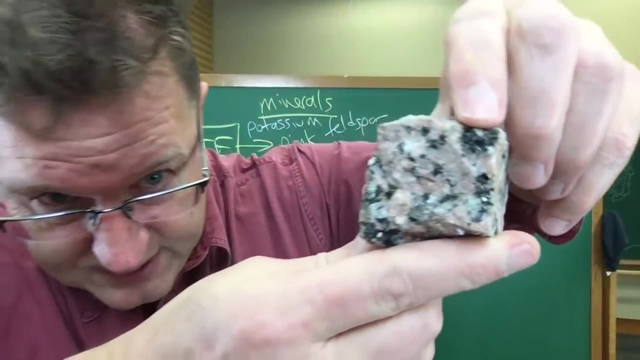 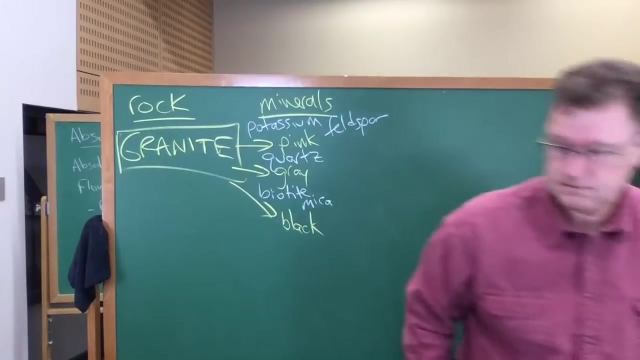 Isn't this cool. This is the stuff we're talking about, But we're talking about it right there. right, We're just talking about these little black biotite specks. Okay, I'm having too much fun. I got to move it along. 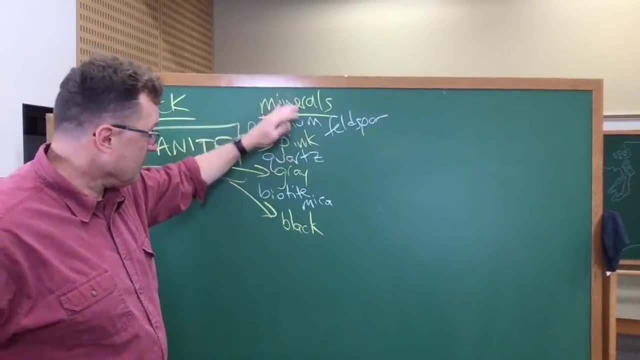 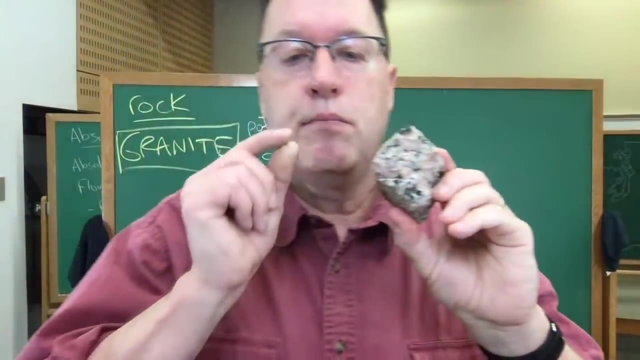 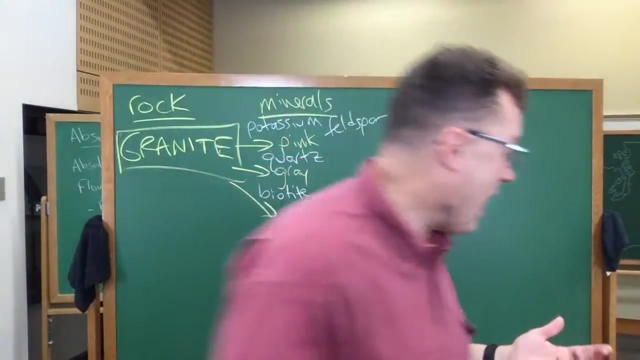 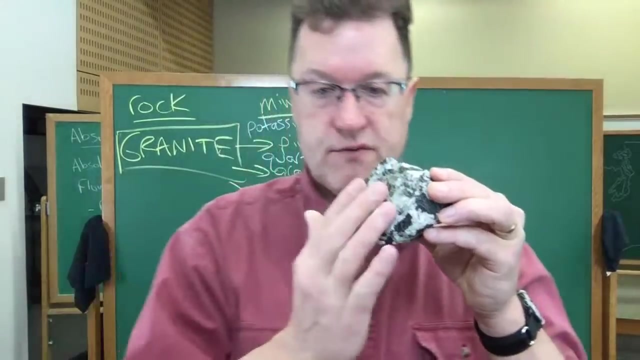 So out of this whole granite, which we've crushed up and separated all the minerals, we're going to toss most of the black biotite minerals. We're just going to get down to one black speck that looks particularly fresh. So when you're with a rock, oftentimes there's a weathered surface. 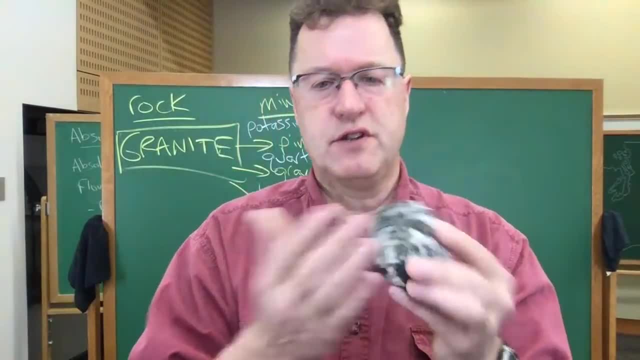 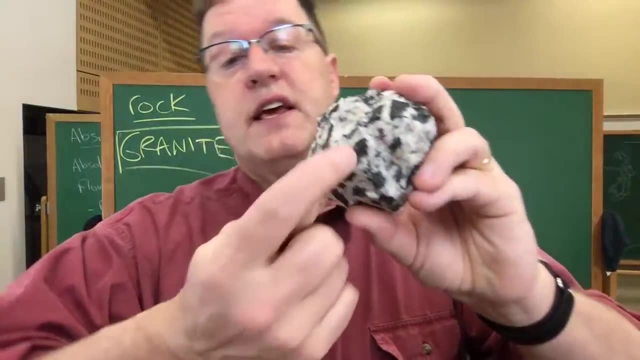 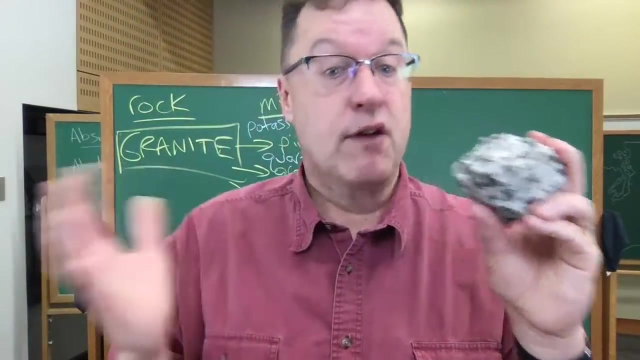 There's a corroded surface, There's a discolored surface. You're familiar with picking up rocks right Lots of times. it looks very different inside than it does on the outside. So it's the inside that we want. We want that kind of pristine, unaltered, unweathered portion of the granite. 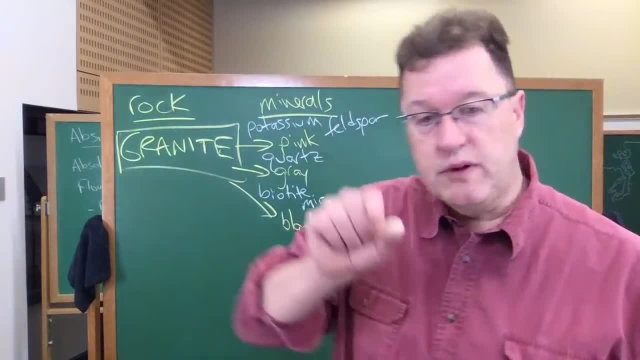 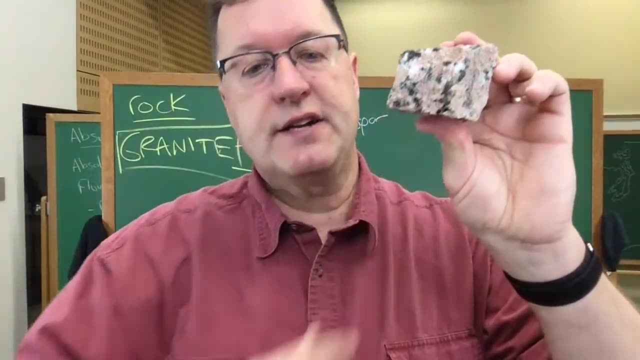 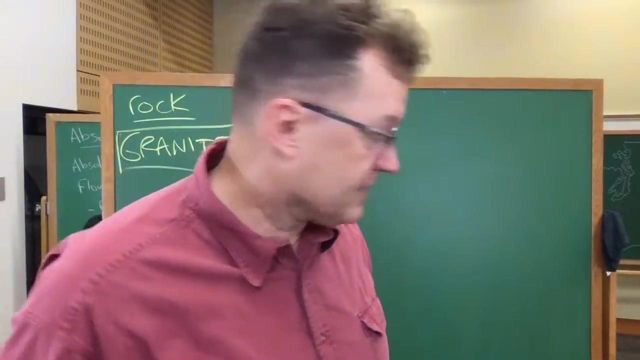 So we're going to select, with little tweezers, little forceps, the most fresh and kind of undisturbed biotite speck And we're going to toss the rest of the black specks as well. So now we're down truly to one black biotite speck using the Australian eraser. 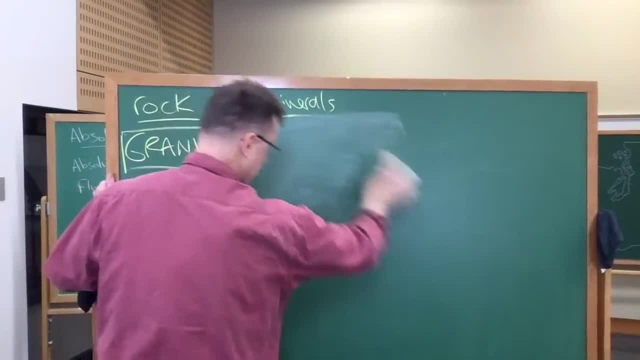 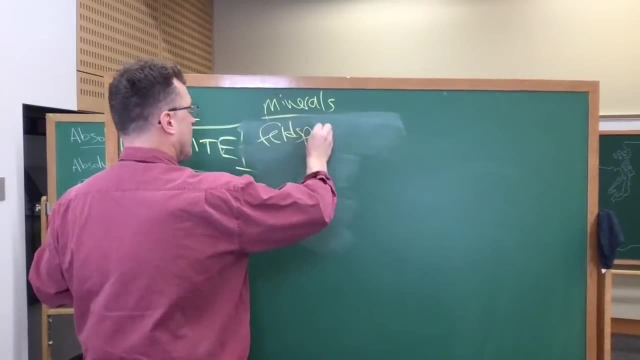 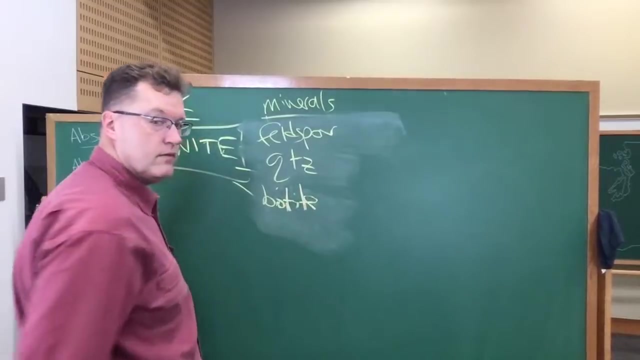 I think that's too busy. So let's just go back to that. Let's go back to feldspar, quartz and biotite. So we don't care about the feldspar or the quartz, They've been thrown away. 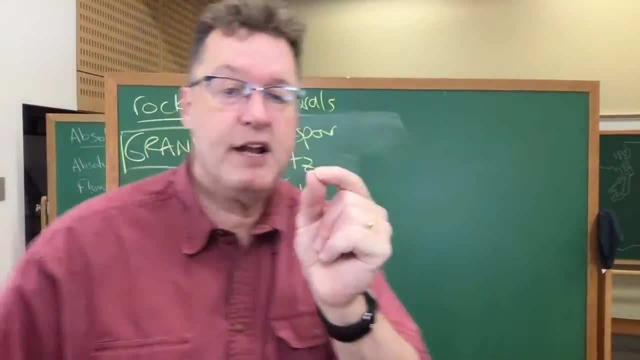 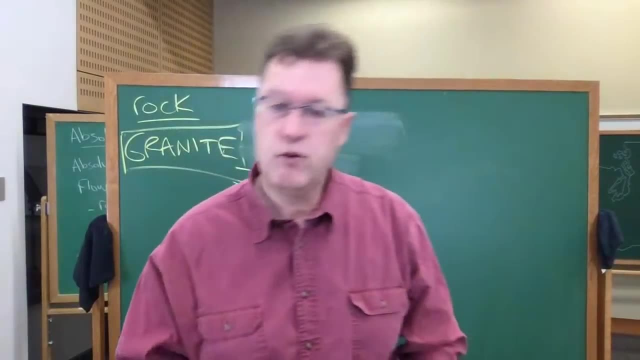 We don't care about the rest of the biotites. We're down to one tiny black biotite speck ideally from the middle of this sample, which this sample, hopefully, was in the middle of a huge pluton of granite like we were talking about yesterday. 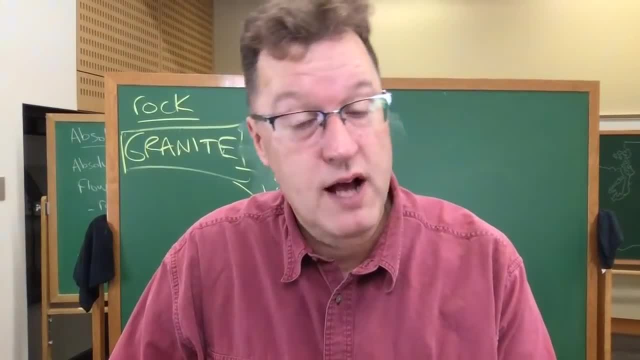 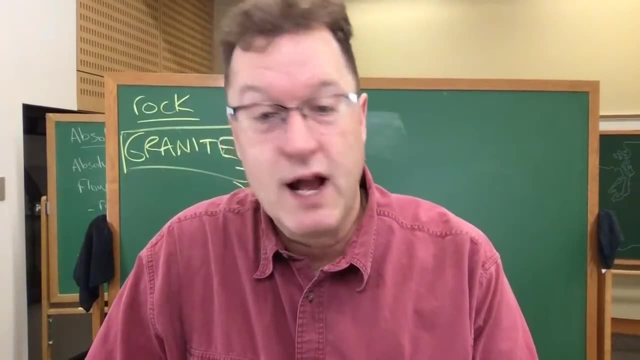 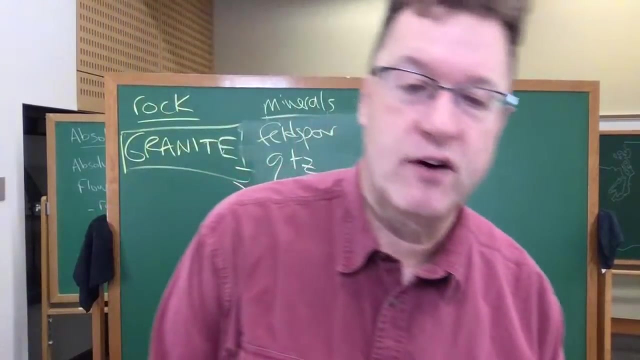 Okay, The process begins by sending our one black biotite speck to a laboratory who can actually do this work, And we wait weeks, and weeks, and weeks and weeks. I used to send my samples to Denver as a graduate student back when I was doing this kind of work. 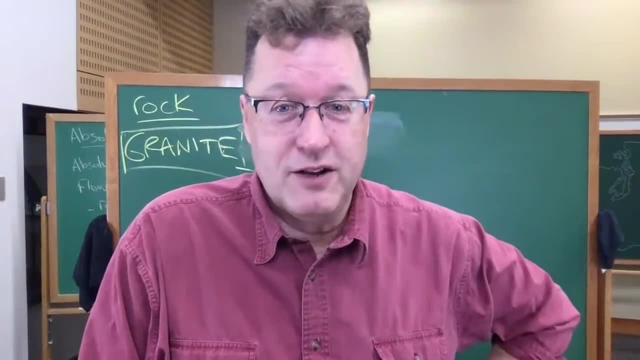 And you wait and you, literally, through the US mail, you send your black biotite speck to a lab and then months later they send it back to you. This is in the old days. I suppose it's all instant now. 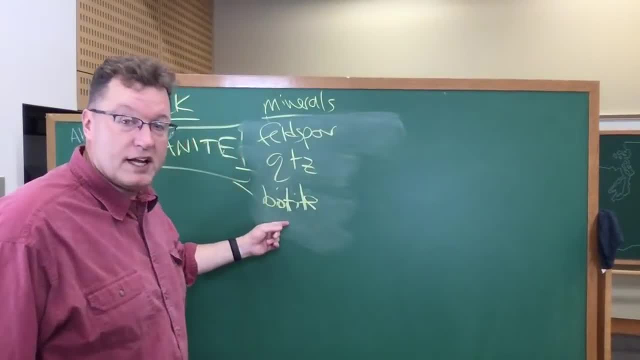 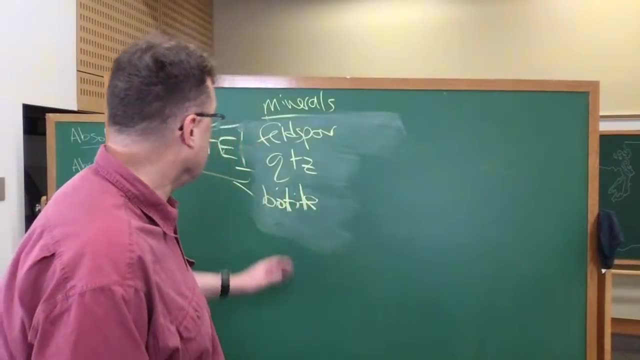 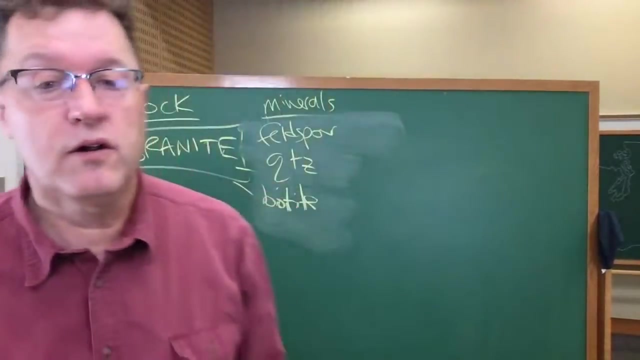 I don't know, And they're going to give us some information about what's inside of our black biotite speck. I'm going to use a different color now because we are leaving the world of macroscopic, we're leaving the world of visible. 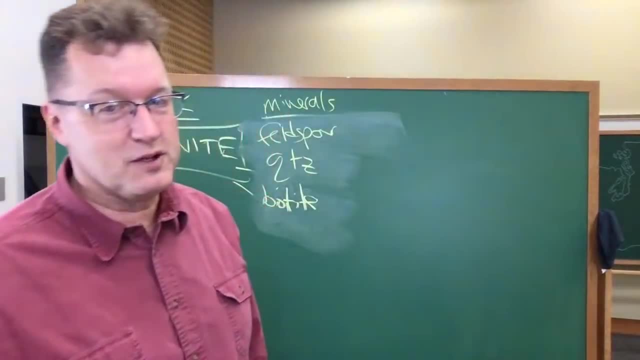 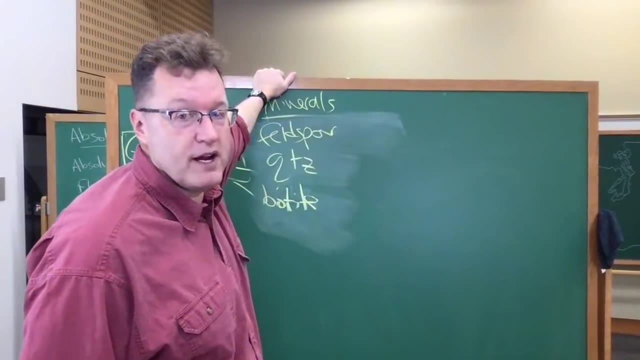 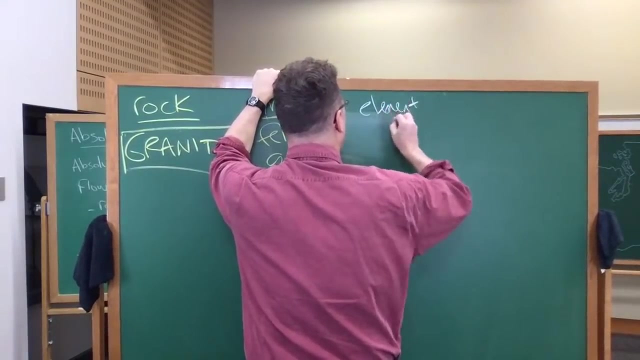 and we're going to the microscopic or invisible world, which becomes less tangible to us immediately, of course, Right. So the people in Denver- who charged us way too much money for this, by the way- are going to tell us the elements. 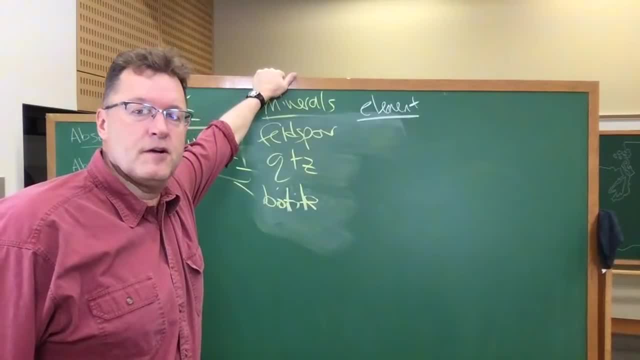 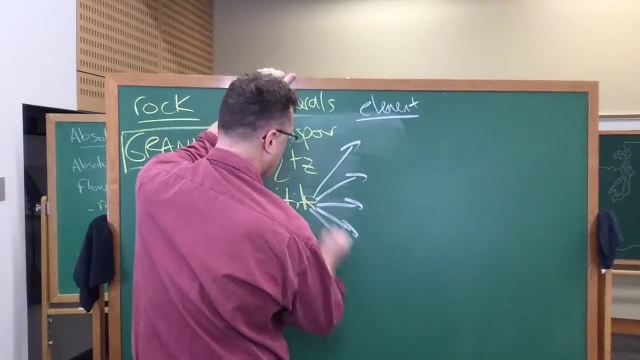 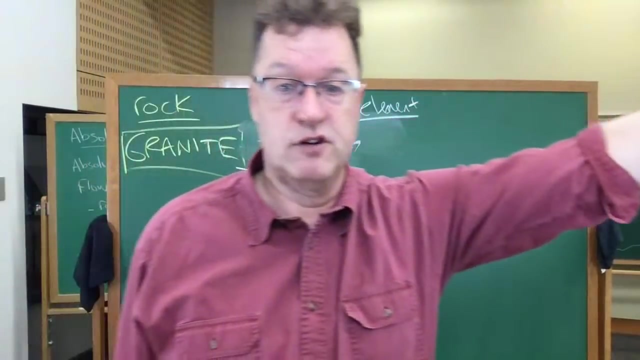 that are in the microscopic innards of that black biotite speck. So in this black biotite speck there are commonly five elements. You see on a periodic chart in a classroom, a chemistry classroom elements like in an ingredient, whatever, okay. 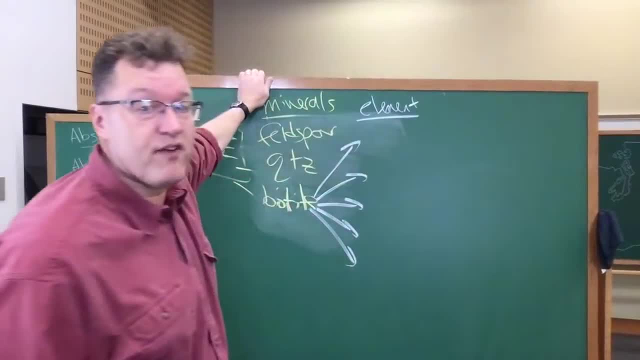 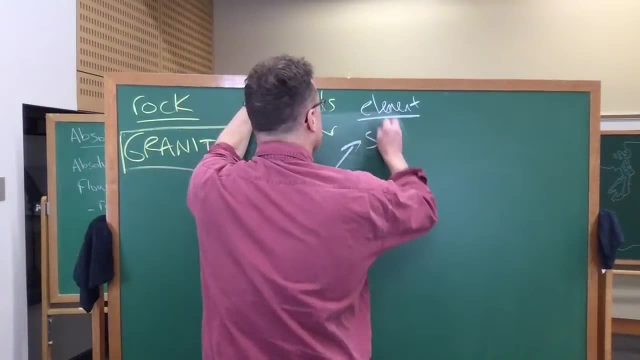 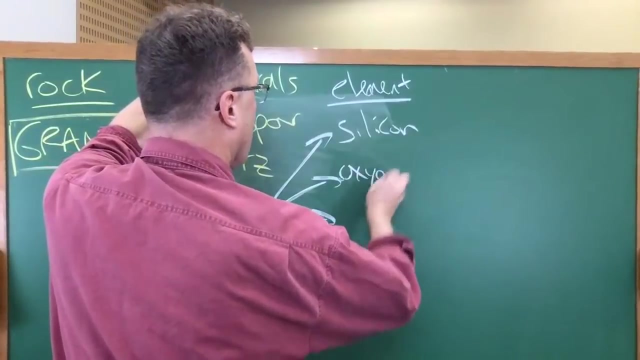 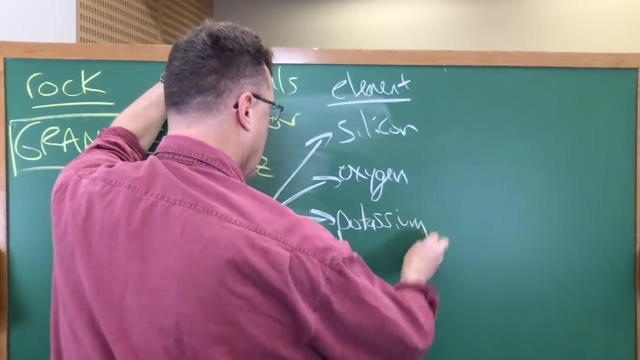 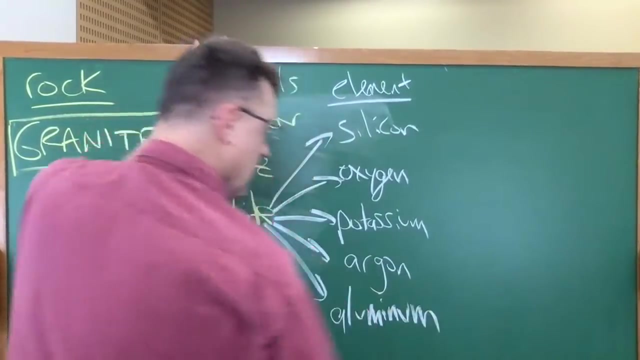 So these are the five common elements that you find in a biotite speck. We're talking about chemistry now. not much, but just a little bit Silicon. I'll come closer again: Oxygen, Potassium, Argon And aluminum. 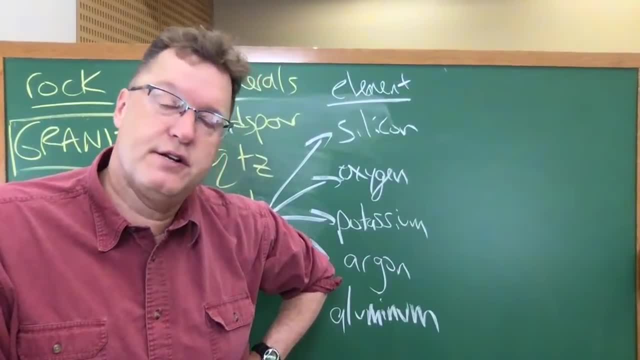 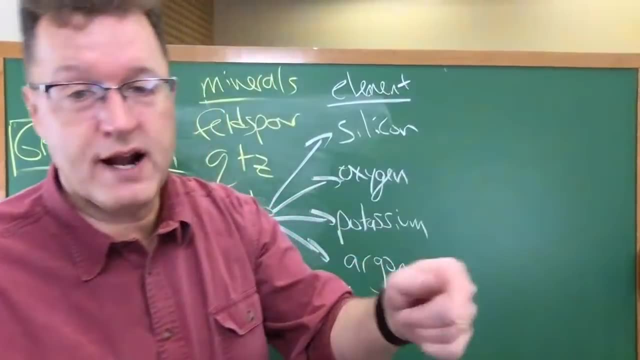 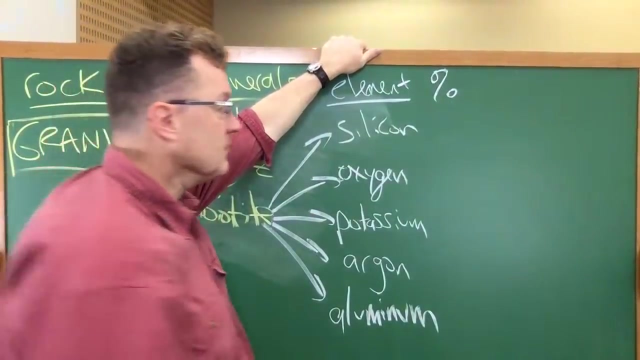 And they're going to tell us the relative percentage of each of those five common elements inside of the biotite that we sent them, The biotite that is from the granite that we're trying to get an absolute age data on. So let's make a column of percentages today. 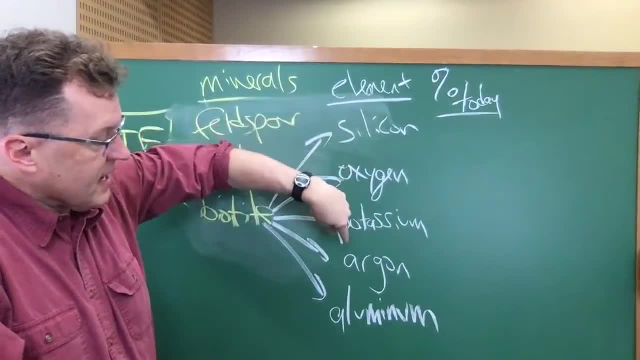 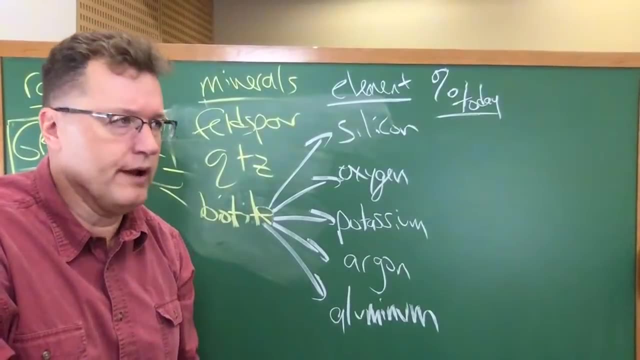 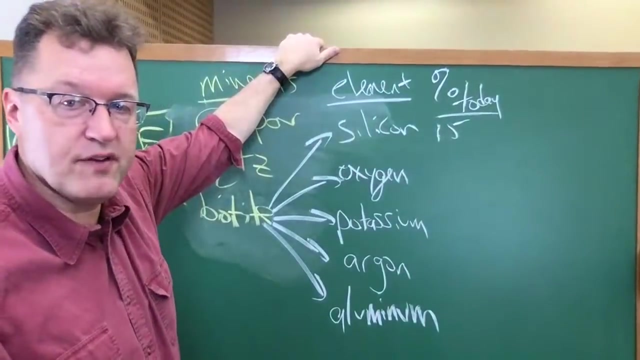 What is the percentage of silicon, oxygen, potassium, argon and aluminum in the black biotite speck today that we sent them in the year 2021?? Common number, Common numbers: 15,, 65,, 5,, 5,, 10.. 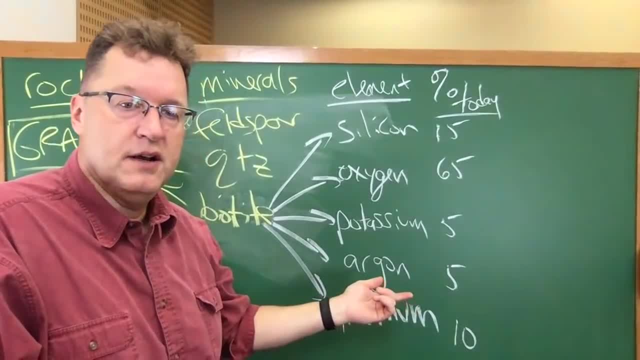 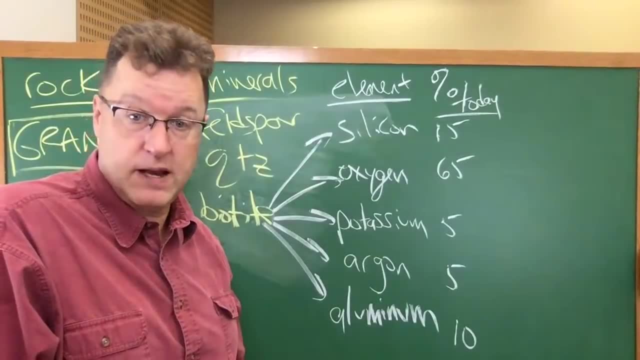 Uh-oh, what's happening. I'm just talking about percentage. In that black biotite speck, there's 65% oxygen, there's 15% silicon and so on. okay, And that's what they give us. 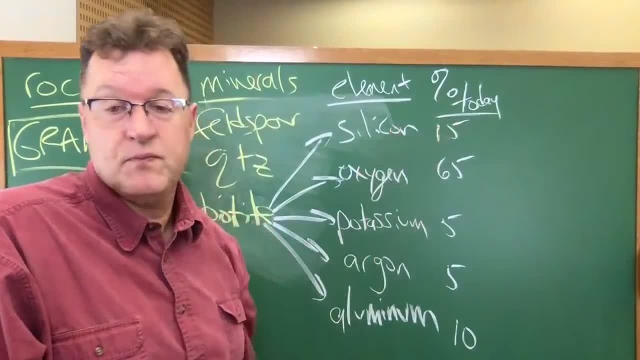 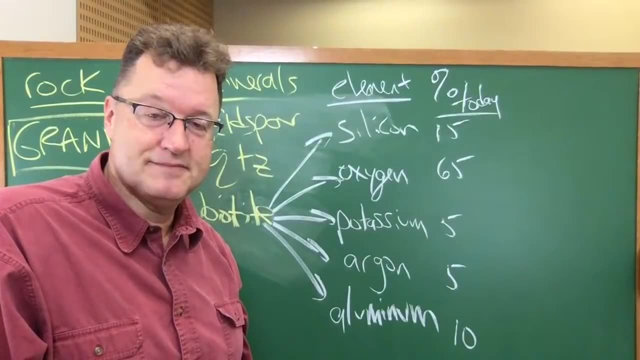 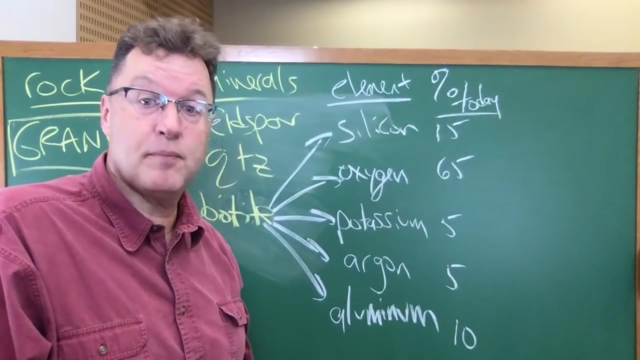 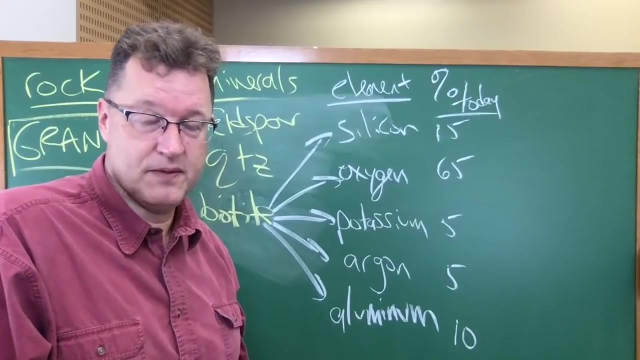 And somehow we're going to have to do some thinking to figure out the age of the granite. What's the age of the granite from this information? I'm pausing because we're about to take a break from the story. You still with us. 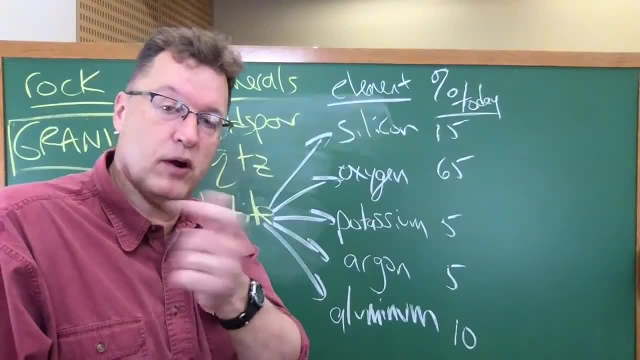 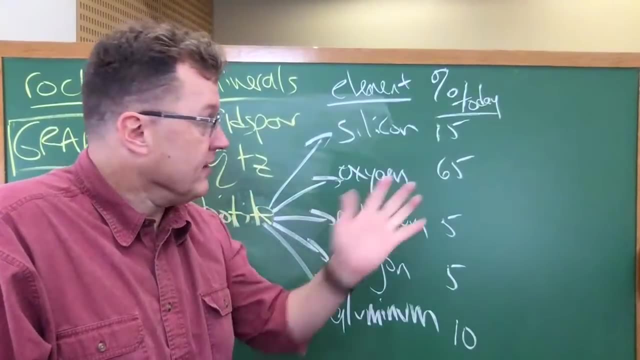 When we come back to the story. in other words, we're going to take a break and go to the yellow book and do a little bit of homework on concepts and terms. I'll try to make it fast-paced so we don't lose our momentum. 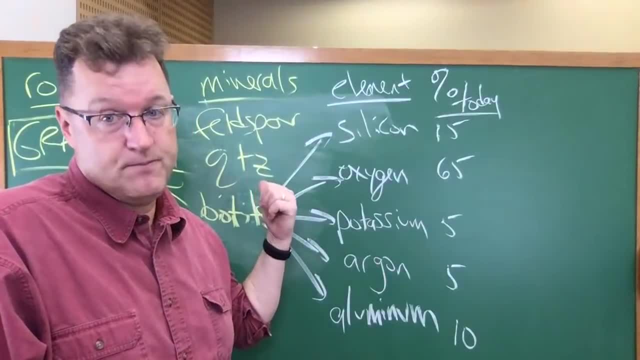 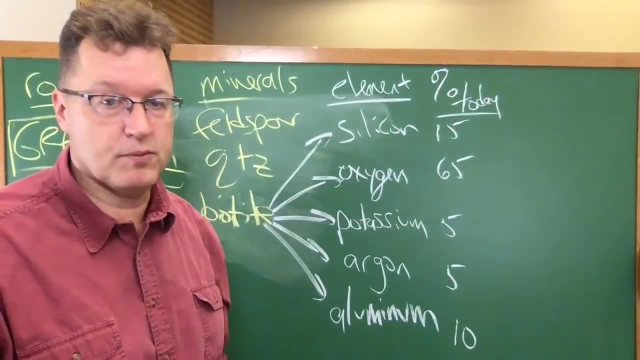 And we're going to come back here and we're going to figure out the age for this granite And to do that, we're going to make a second column of percentages and then we're going to compare parent isotopes. We don't know how to do that yet. 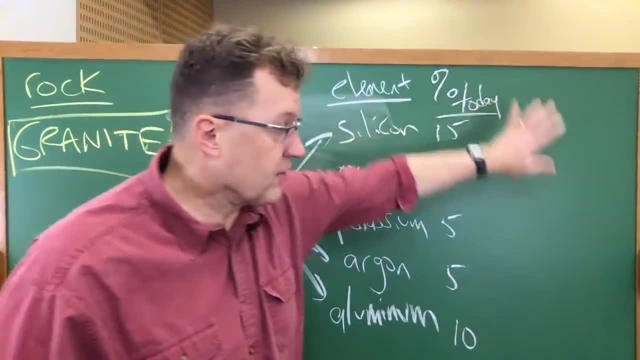 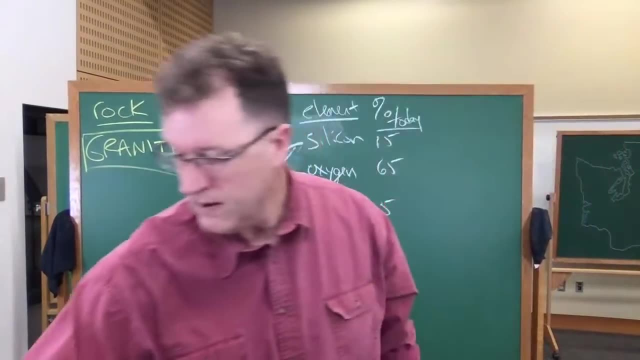 So give yourself some room, central student. You're going to make another column here in just a second, But I'm going to give myself some physical room And I'm not going to belabor this because, again, I think we've got something going. 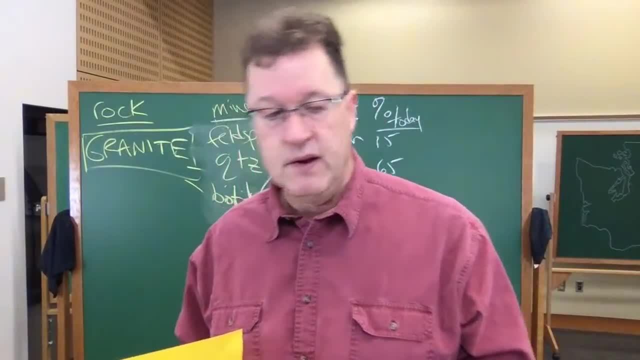 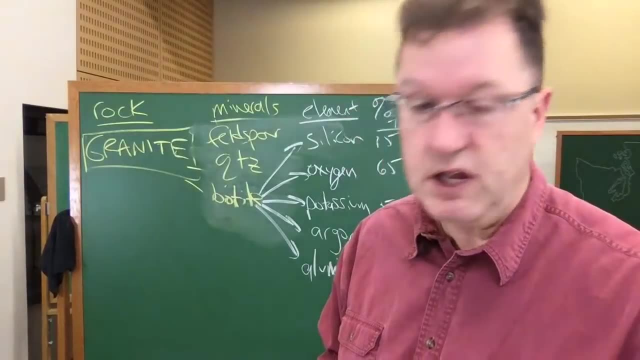 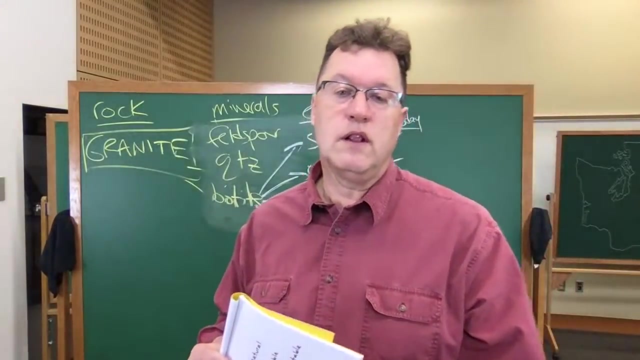 I can feel it. We've got something going right now, Except for those five no-shows. Not a fan at the moment. We'll see if they rally. So this was on the outline I gave you on the other chalkboard. Okay, so this is not particularly imaginative. 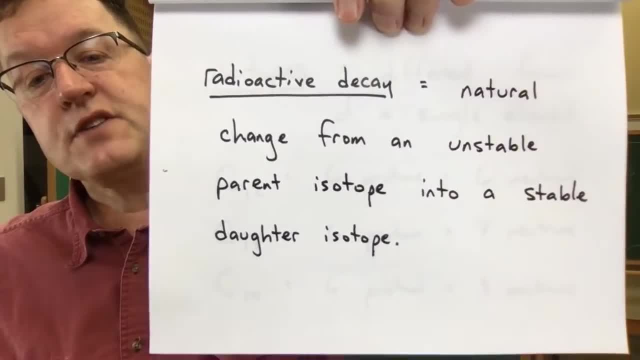 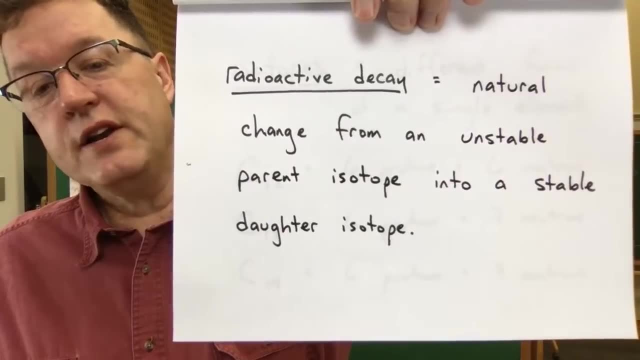 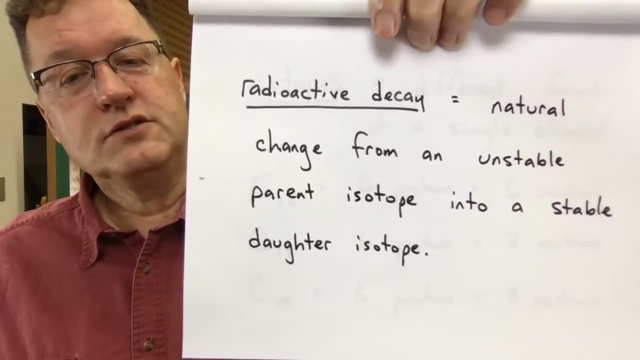 but it's the best way I know how to teach this. Let me just give you a very basic definition. first of all, We need to know about radioactive decay. You can read it as well as I. It's a natural process. This is not a human-started, human-determined 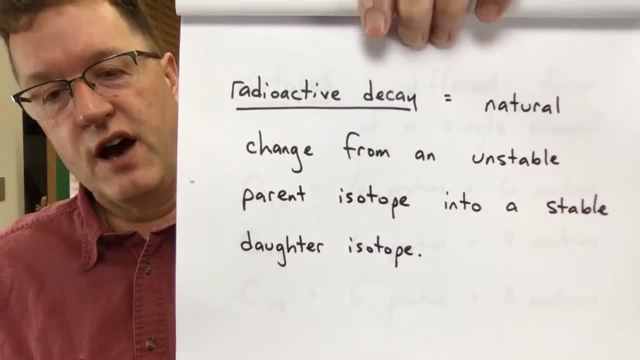 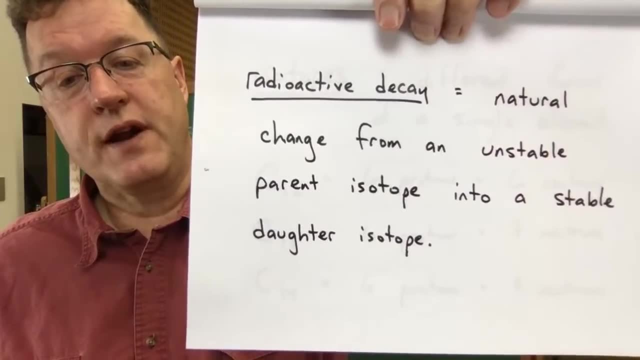 human-created process. This has been going on since the dawn of time. Radioactive decay: It's a natural change from one isotope to the next. Oh God, now we are talking about chemistry. Oh boy, I'm an oboe major. 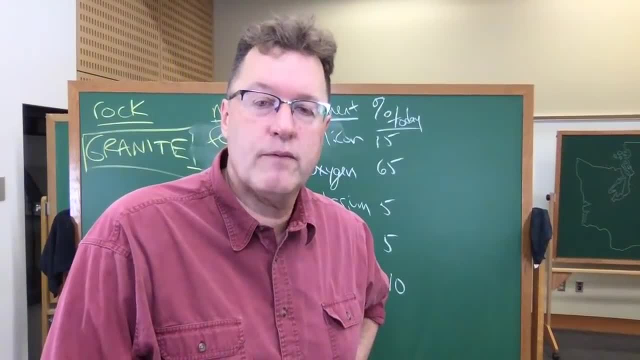 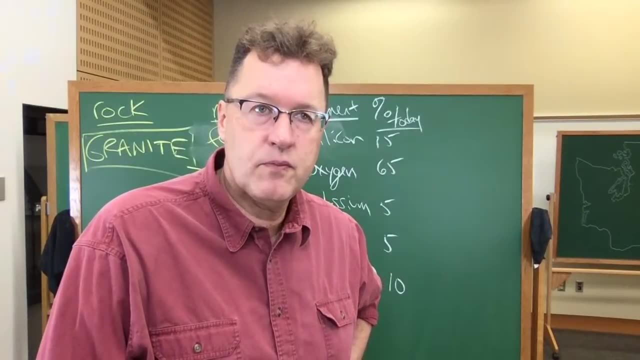 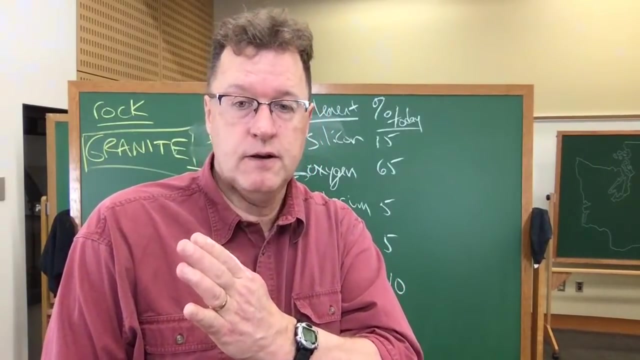 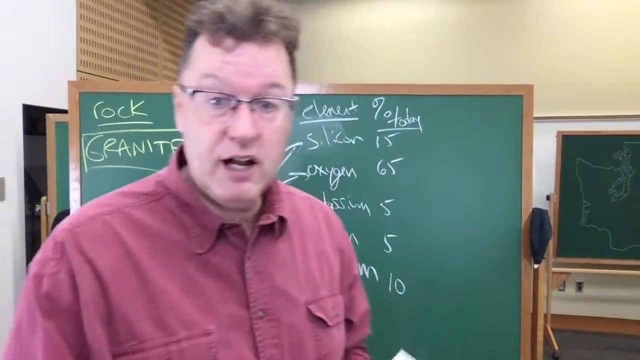 What are we doing here? Well, you know, I can maybe make this work for you. Do you believe in what we're doing? We can make it work. Radioactive decay: A natural change from one isotope to the next. Well, what's an isotope? 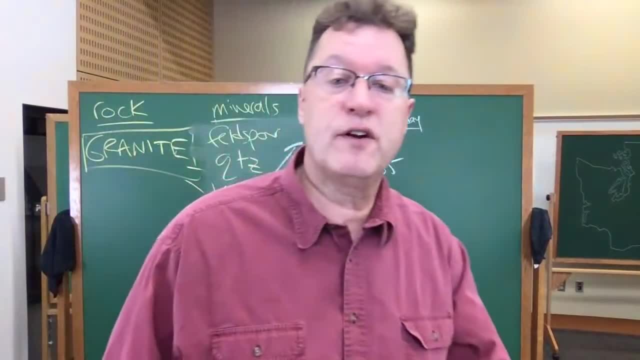 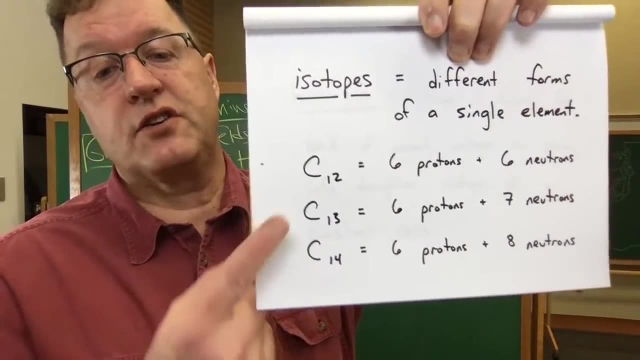 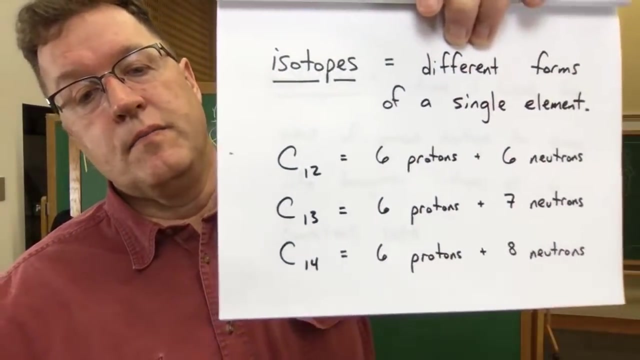 An isotope like these sometimes are found in different forms. So an isotope is just a different form of the same element, For instance carbon, which is not on our list. There is no carbon in a biotite mica flake. 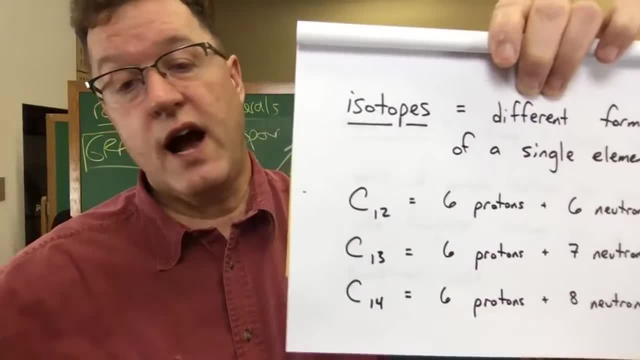 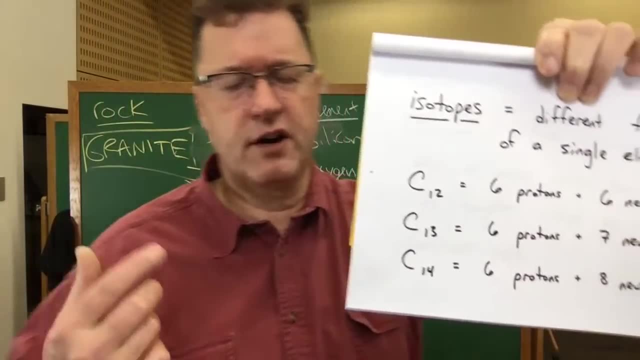 But just to help you see, if you've never had a chemistry class or forgotten long ago, isotopes are just different forms of the same element. So this is carbon, Carbon-12 or carbon-13 or carbon-14, probably because of carbon dating. 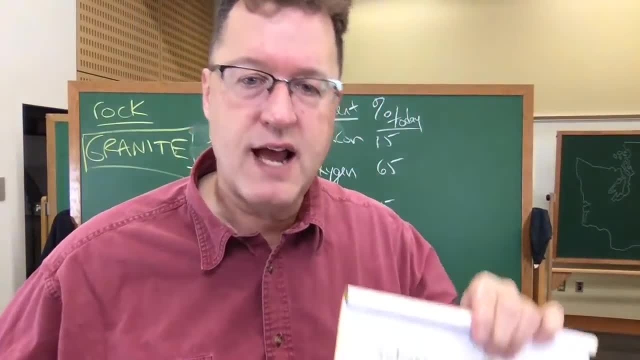 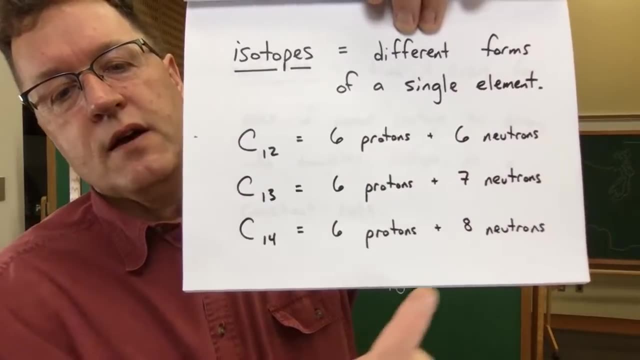 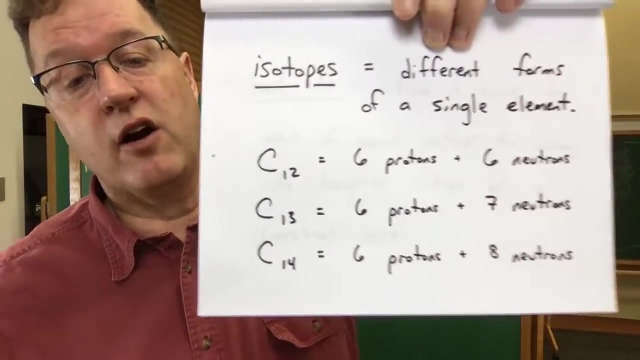 which is controversial among people who don't know anything about science. It's not controversial, But my point is: we have three different forms of carbon, based on different constituents inside of the nucleus. Let's not even care about any more than this When I say the word isotope. 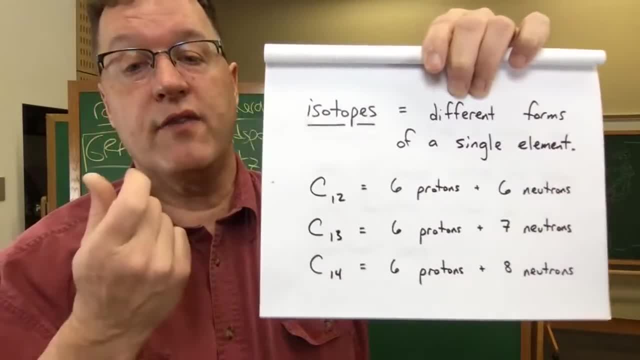 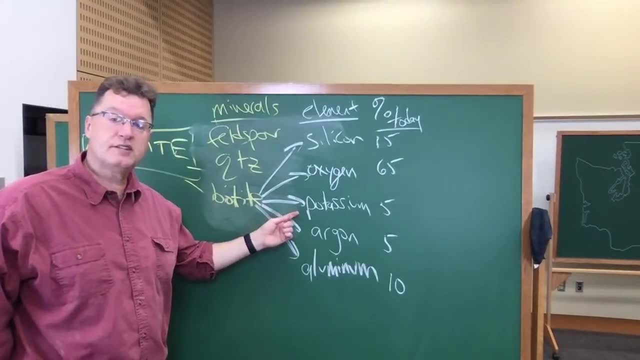 I'm just talking about a certain form of a common element. So there's more than one isotope of potassium and argon. We only care about one of them and we're not going to get hung up on which isotope it is. 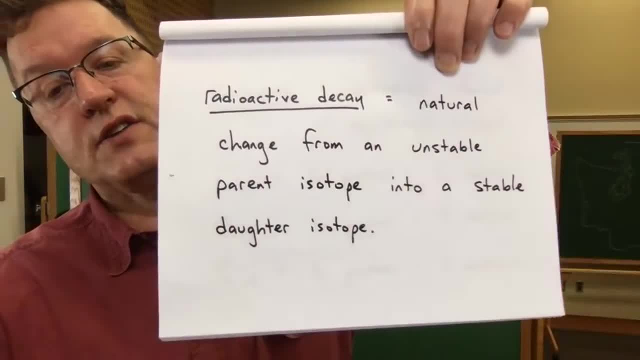 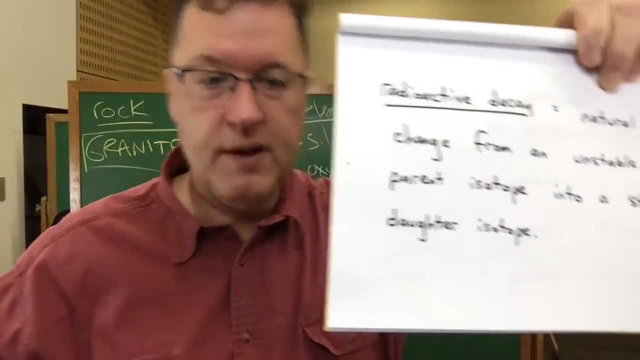 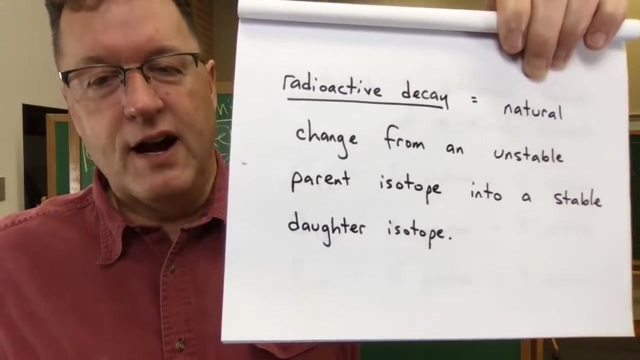 But we do care about that word isotope, because here we are back to this definition on page three. We have a natural change from one isotope, one form of an element, to a completely stable form of a different isotope. So right off the bat I got to say: 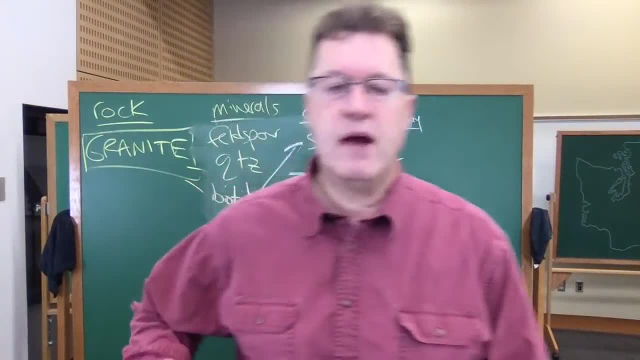 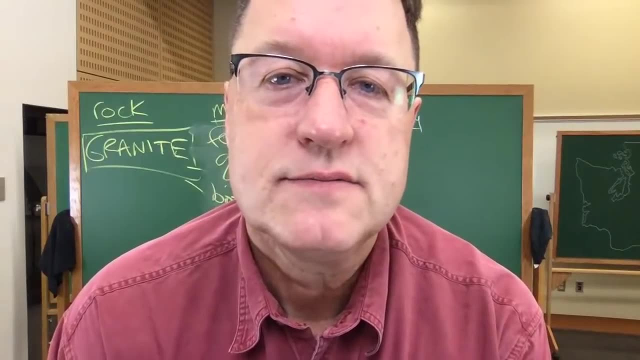 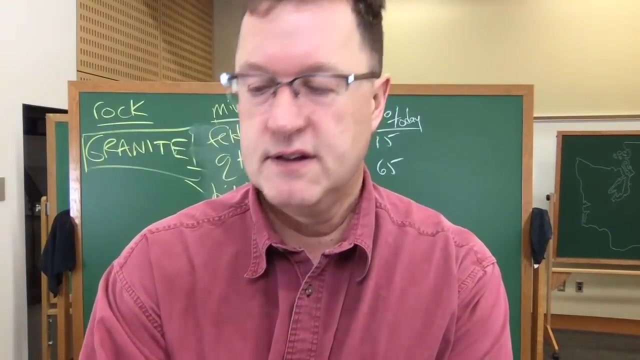 not right off the bat. I've been at it for half an hour. Let me emphasize to you: this is a magical process. I know we're talking about science and a little bit of chemistry and a little bit of math, But if we just step back and think about this, 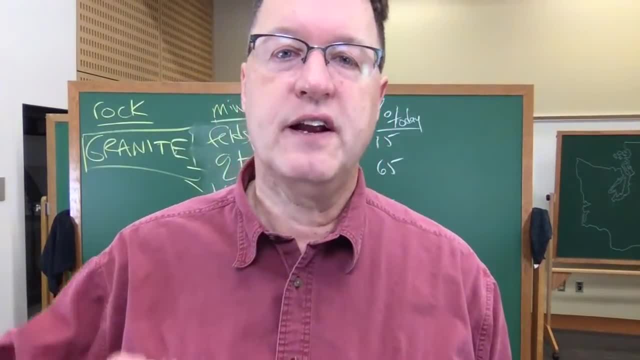 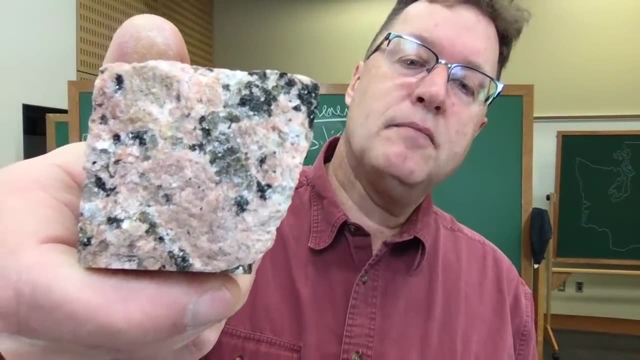 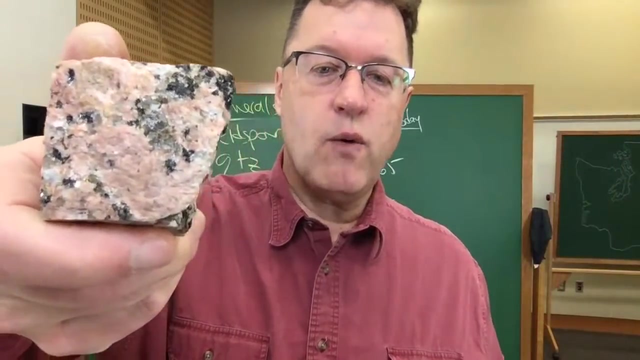 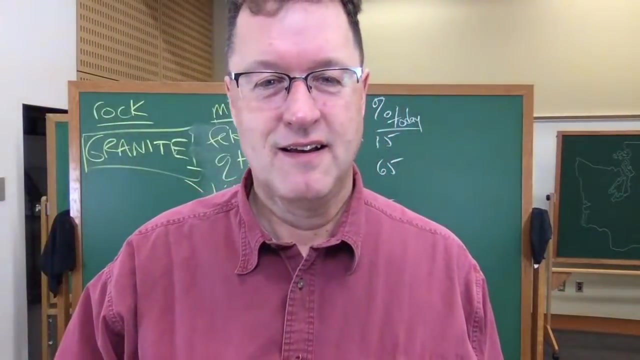 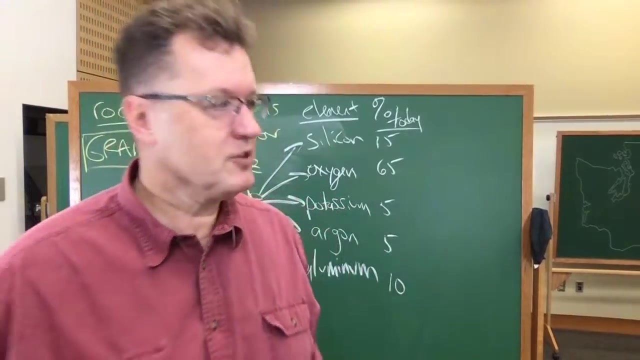 there have been discoveries in the last 150 years to realize that in this black mineral there is a natural change that's been going on for millions of years at the microscopic level. Nobody started it. There are certain elements that are radioactive, which simply means 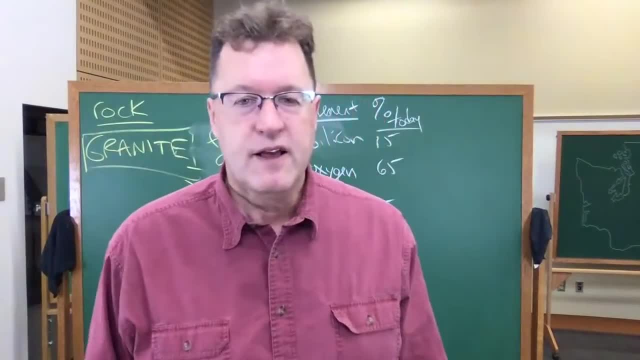 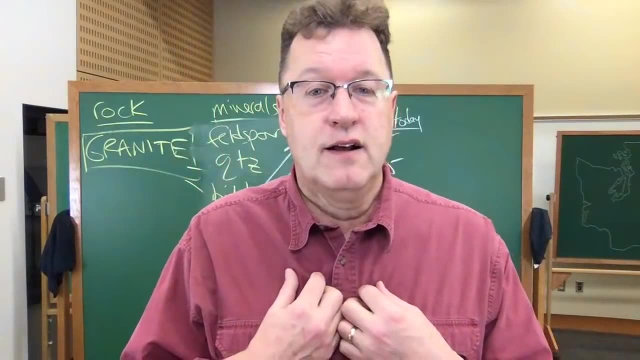 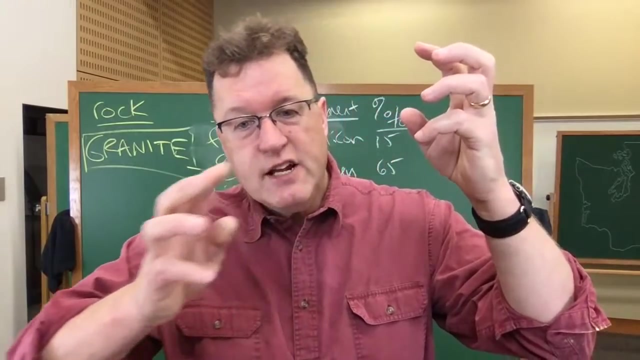 again. I'm just stepping back and thinking about this and trying to help you see it, If you are a radioactive element- and a few of these will be radioactive- if you're a radioactive element, that means an isotope of you naturally wants to change. 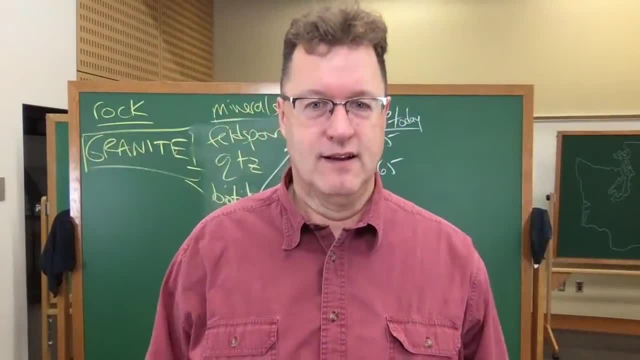 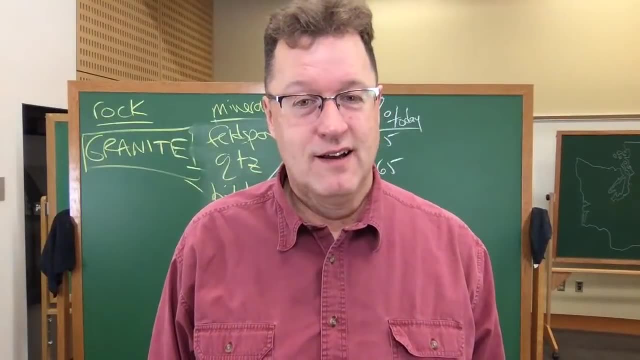 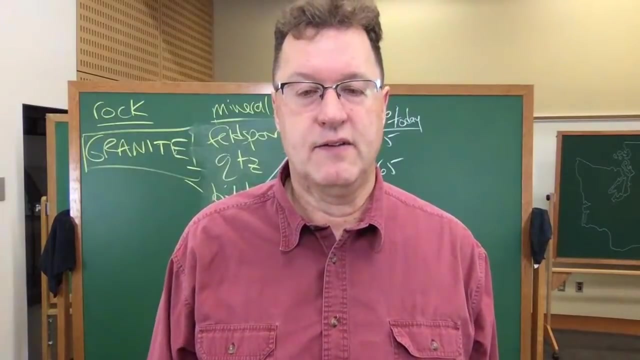 into a completely different fricking element Right before your very eyes, in the middle of this rock, And I'll cut right to it, because this is the whole concept to talk about today: That change from one isotope into a completely different isotope. 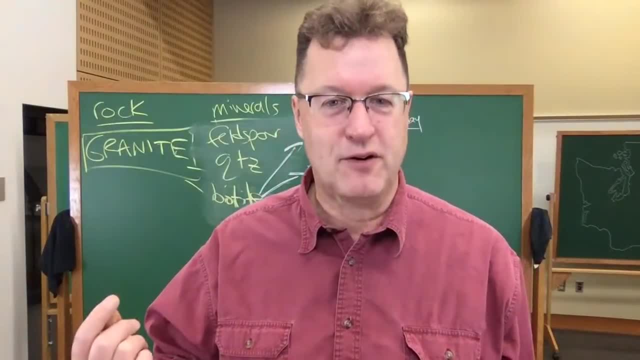 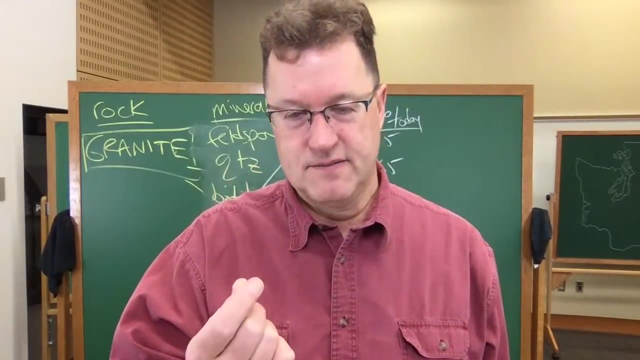 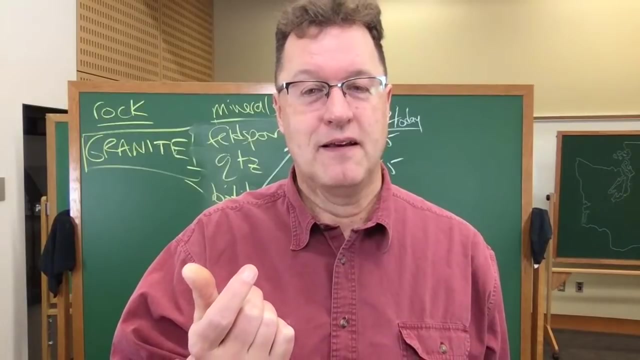 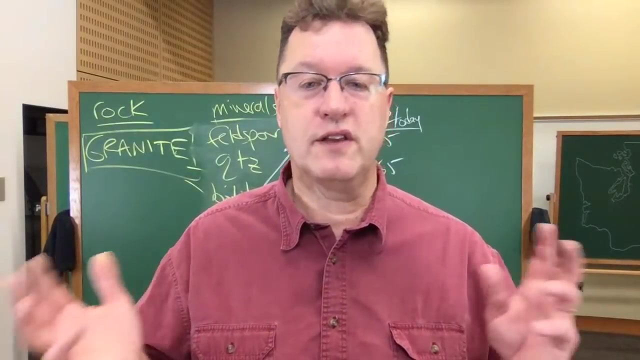 at a microscopic level inside of a black mineral, in a granite. that elemental change happens at a constant rate And therefore we can keep track of time. And I don't know who we have in the townies here. We might have some who are violently opposed to this concept. 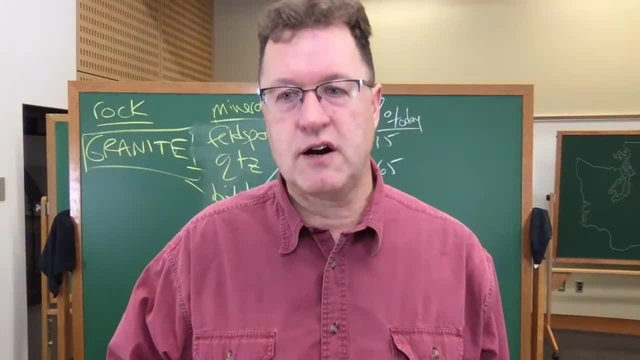 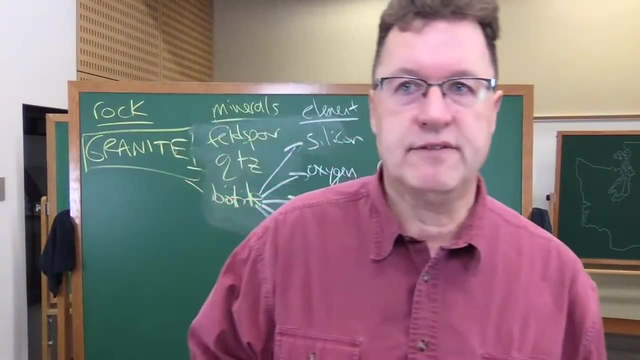 And one of these days I'll come up with a lecture for the public. I've been thinking about doing this for a long time. I never have In a vacuum. I guess it's hard to understand this or hard to believe it. 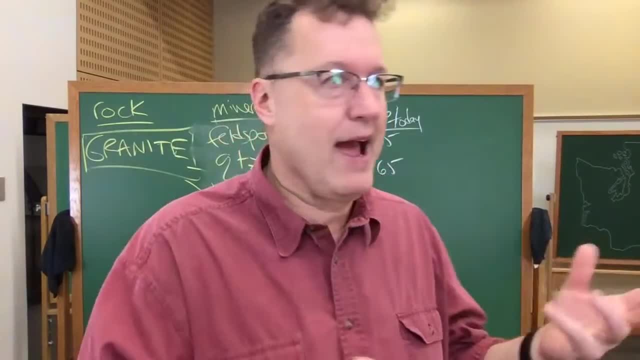 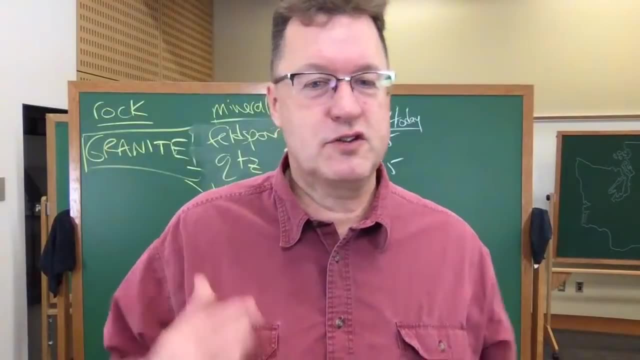 Because it's microscopic and it's in a lab, and I haven't even been in these labs to see this measurement of parent and daughter isotopes. So there's a certain element of faith with me too, I must admit, But in a vacuum. 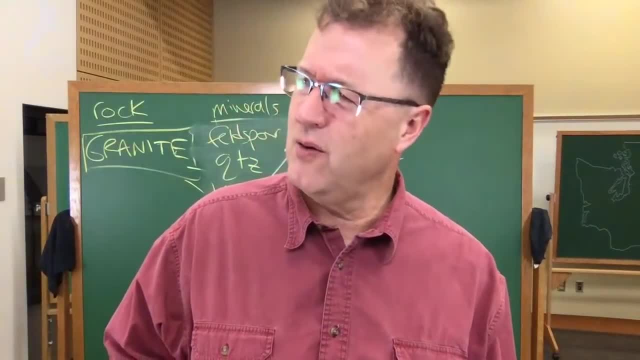 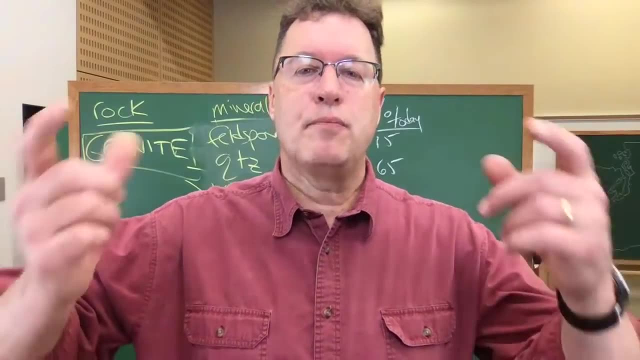 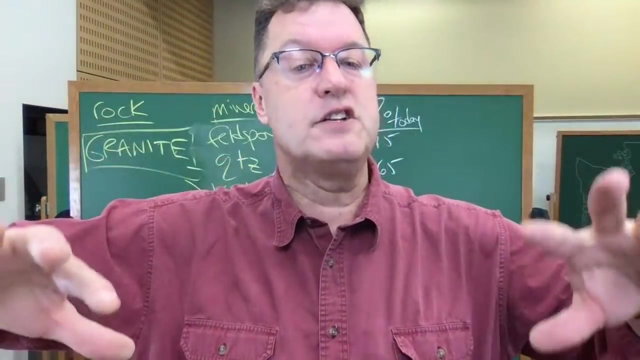 it feels like what I remember. my dad used to kind of go that way. Really, They're getting the ages from that, But the point that is lost on almost everybody, it seems, is that there is amazing amounts of field checks and relative age date rules. 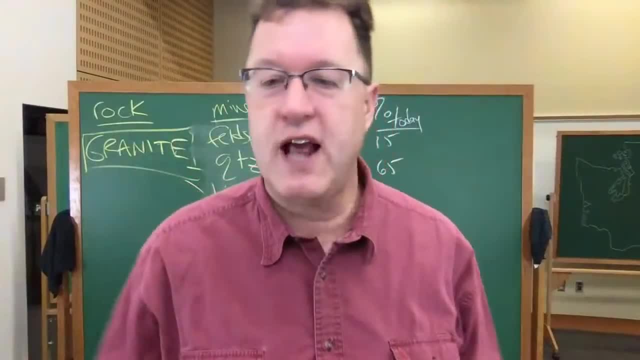 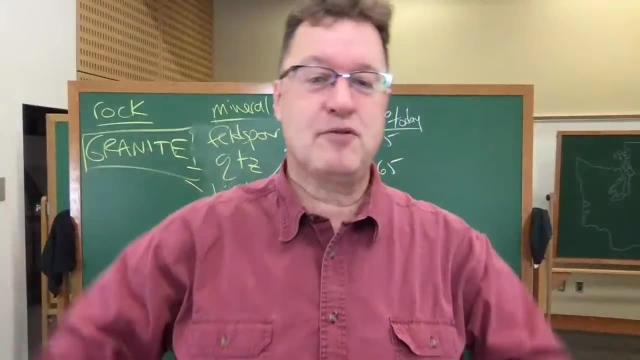 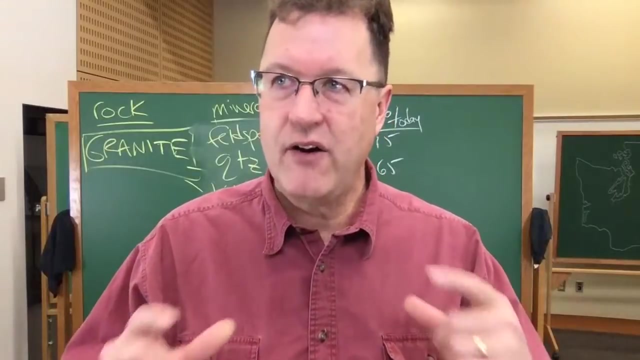 that are common, basic, common knowledge to everybody, And it all works beautifully. The relative ages work with the absolute age. The absolute ages confirm the relative laws. That's what I need to think how to present, Because I think it could really work. 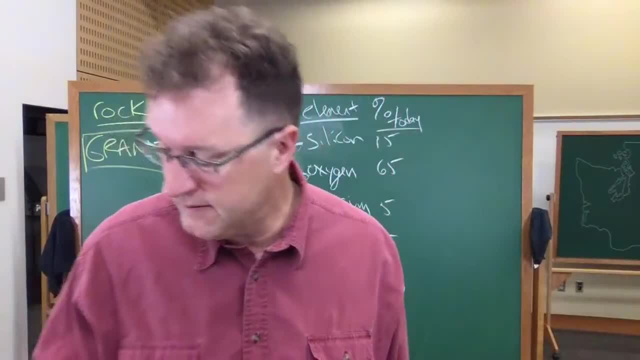 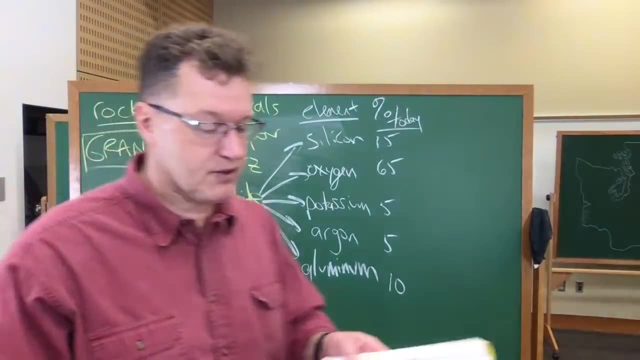 For those that were interested in watching that, But I don't have that for you today. Okay, We really took a break, A longer break than I wanted, Okay. So we're about to come back to this story, But I want to put a little asterisk. 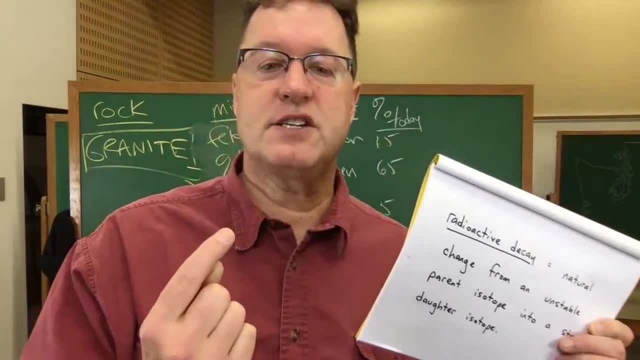 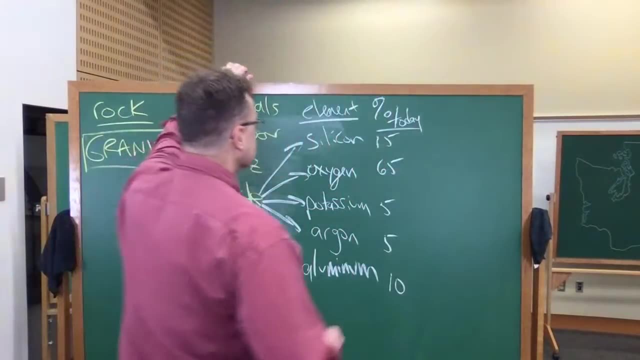 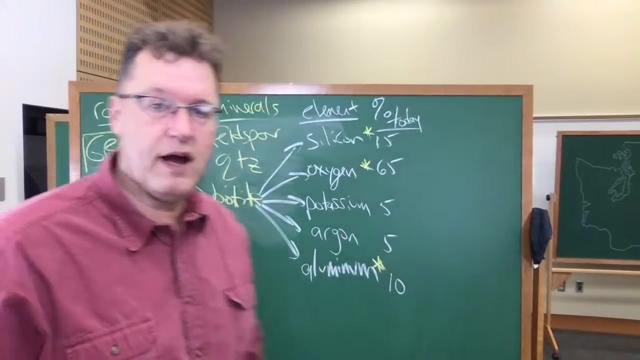 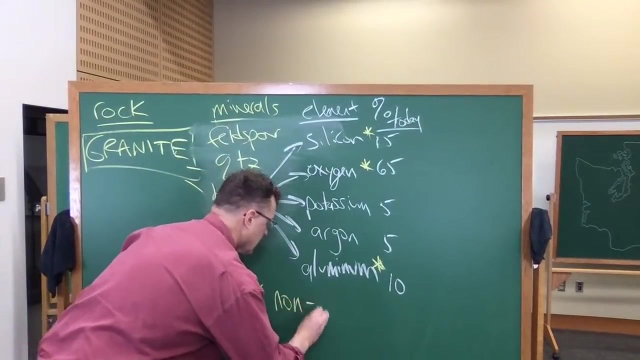 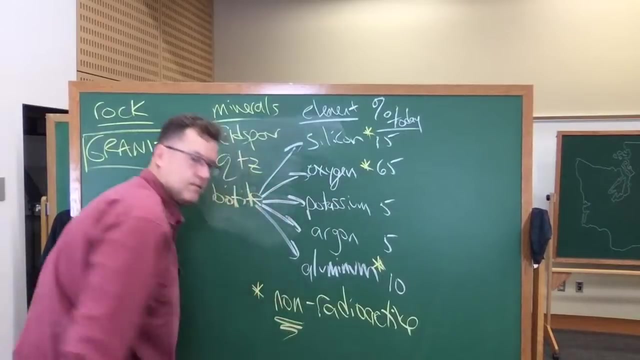 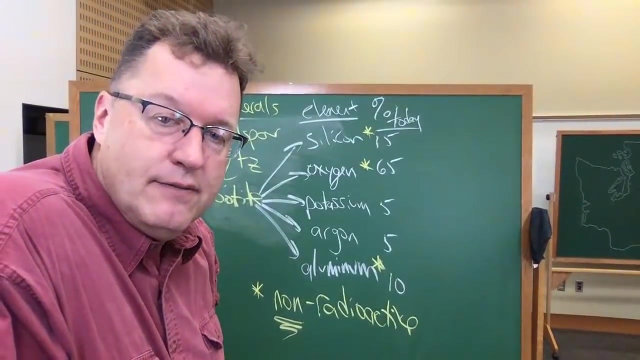 I always struggle with that word. Asterisk, I'll just say ask for short, I'm going to put an asterisk. A star means the element is non-radioactive, Which means it doesn't do this changing business. We haven't even talked about the change yet. 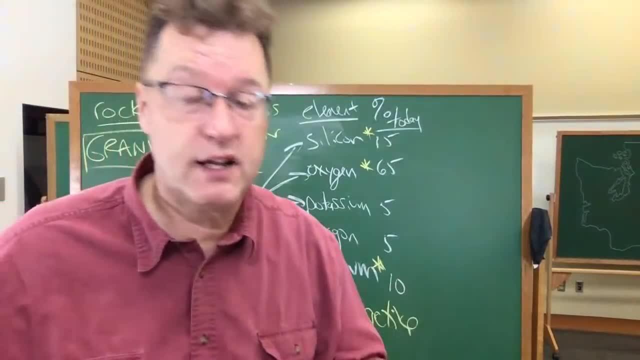 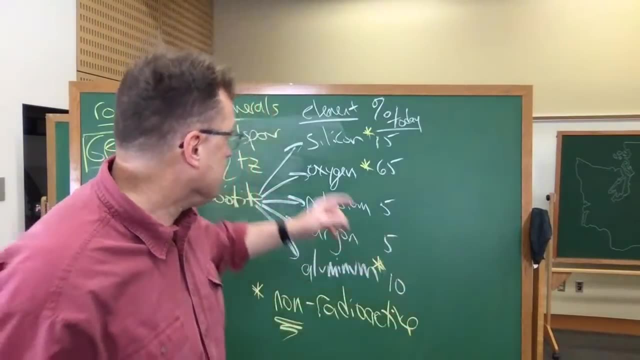 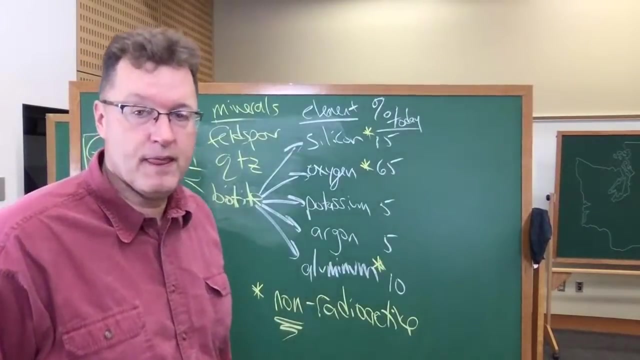 But I've given you the concept that if you are an element that's radioactive, that means you're naturally changing to a completely different element. But silicon, oxygen and aluminum were not selected for this problem today, Because they're non-radioactive. 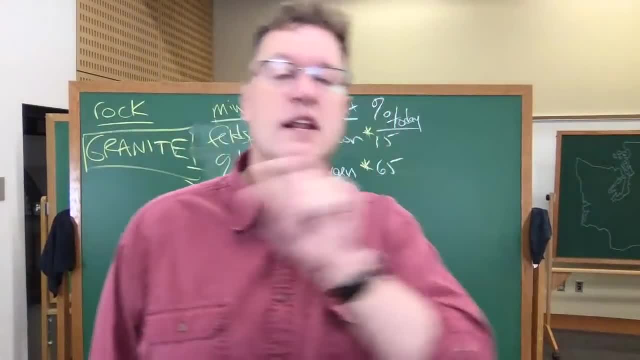 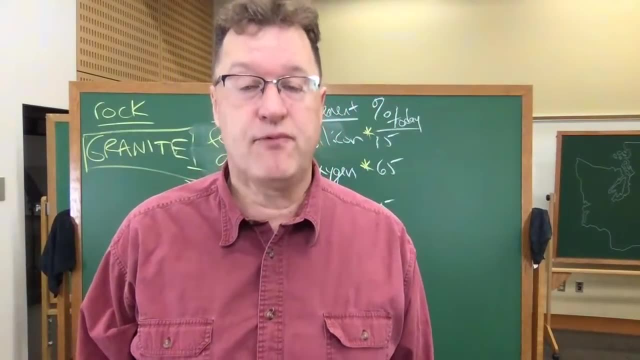 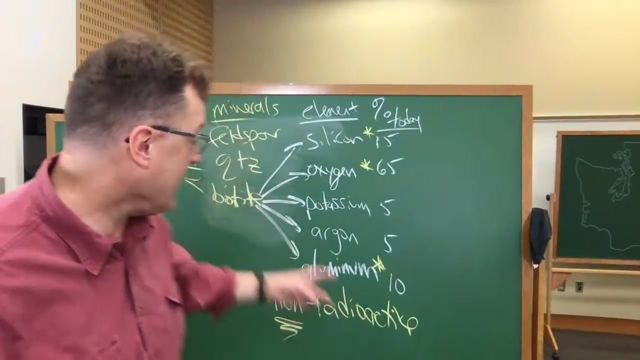 They're not going to be helpful to us. We need the decay, We need the change, The slow, steady change of one element into another to keep track of time for us. And potassium and argon is radioactive, Potassium and argon. 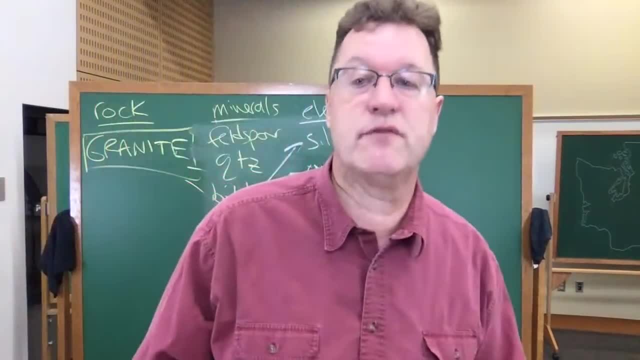 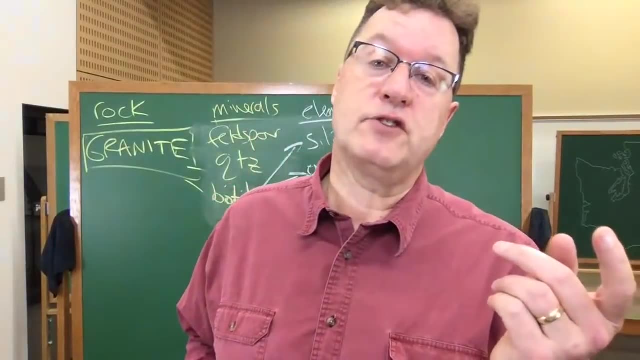 are going to be carefully looked at for the rest of our period. today We have 15 minutes left. That's about right. Okay, So if you feel like things are dragging and whatever, it's going to get intense here for the next 15 minutes. 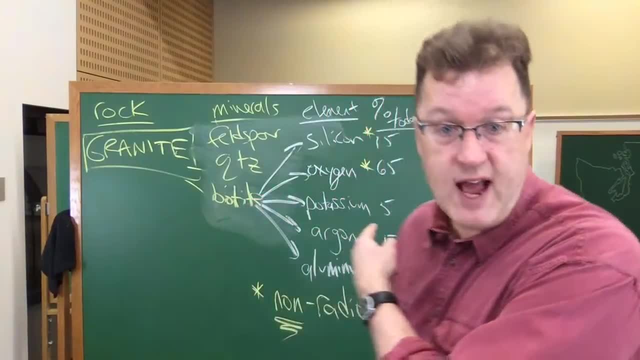 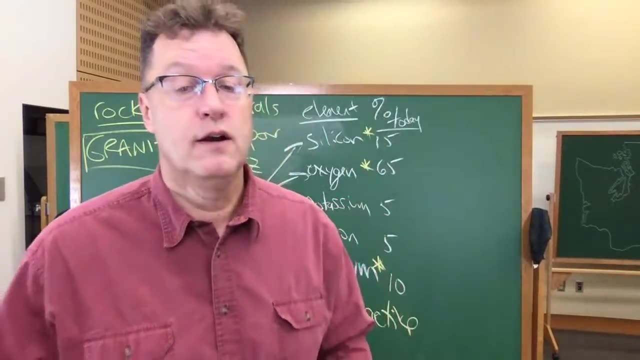 You ready? We're going to do three examples. This is just granite number one. By 15 minutes from now, we're going to have three answers to three different problems of three different granites that have three different ages. One more page. 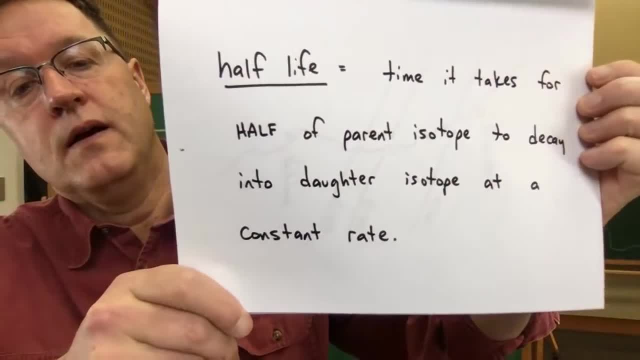 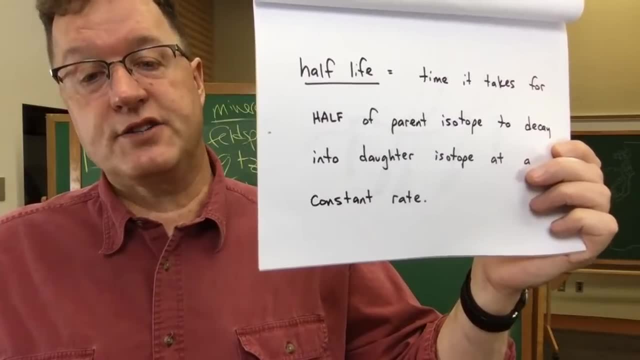 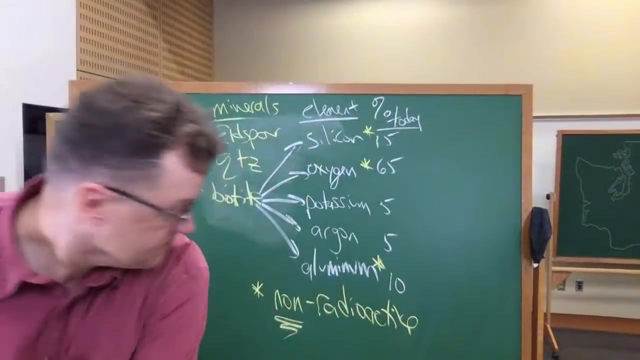 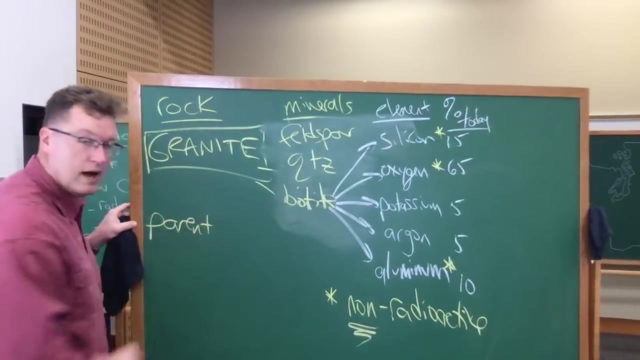 Page five: half-life- You've heard that phrase perhaps. Half-life is the time that it takes for half of a parent isotope to decay into the daughter isotope at a constant rate. Okay, so I need to go back. Parent isotope, daughter. 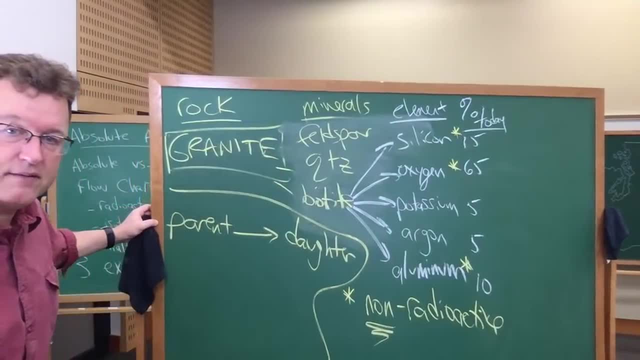 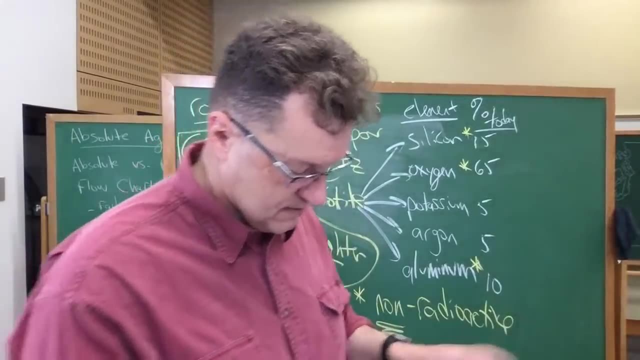 So this is in a little bubble all by itself here. okay, I'm just giving you more background on what parent and daughter is. I'm going back to page three and being a little bit more careful now. This radioactive decay is a natural thing. 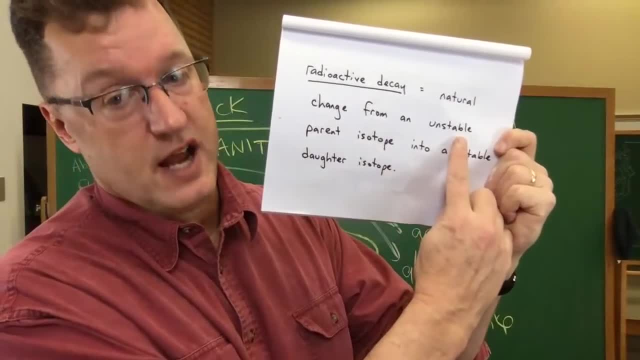 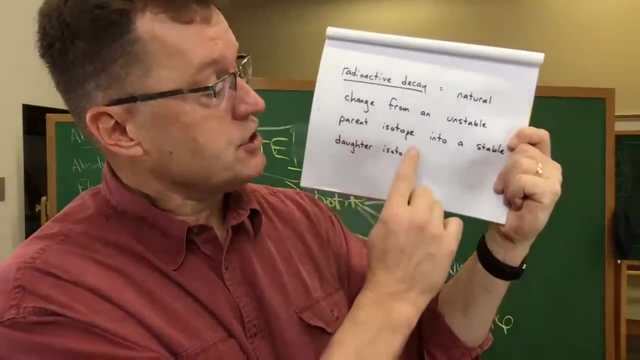 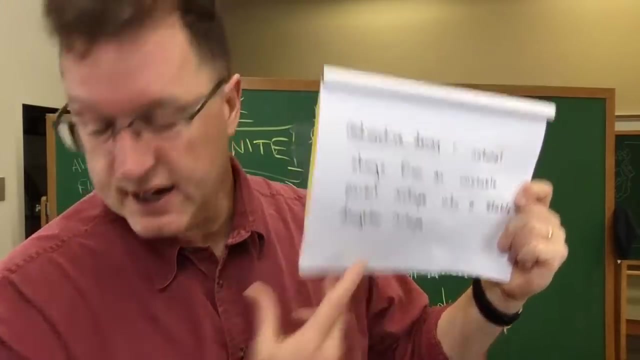 and we take an element that is unstable, We call that unstable isotope a parent and it changes into a different element that we call a stable daughter. Let's not get hung up on. why do they call it parent and daughter? I don't even know, okay. 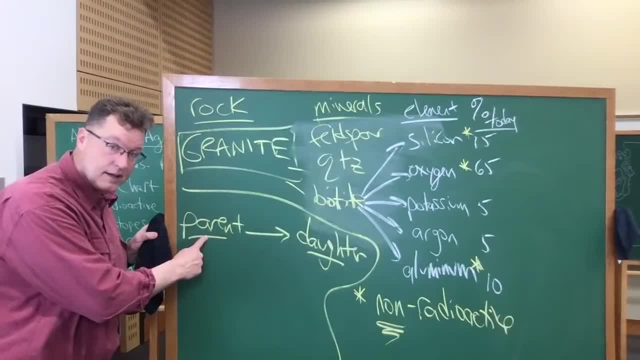 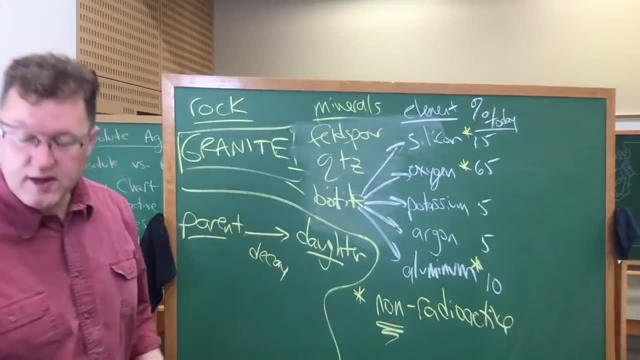 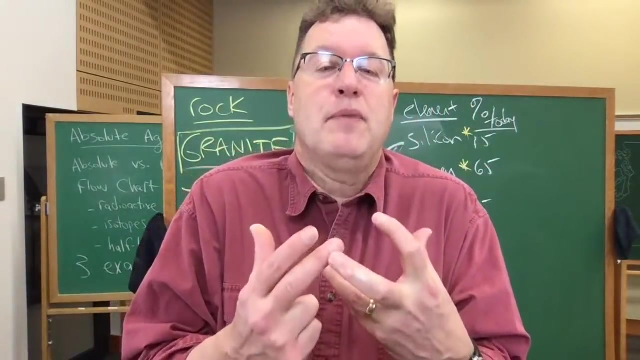 But the parent isotope is the original element. The decay happens, The arrow says decay, And then we end up with the more stable configuration. It's like you are born to a body but you don't feel like it's the right body for you. 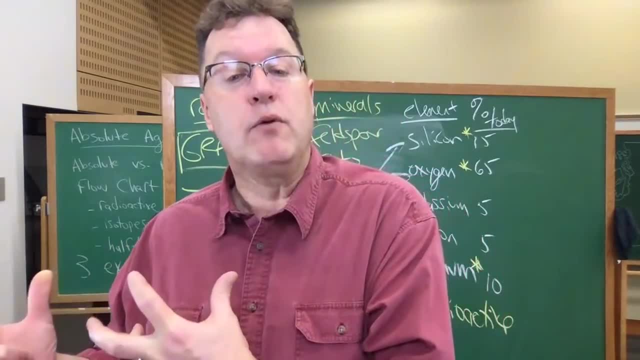 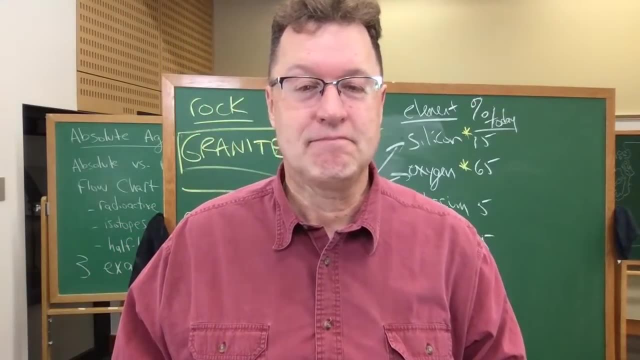 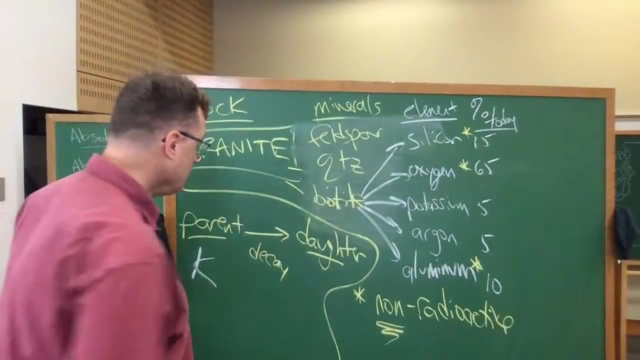 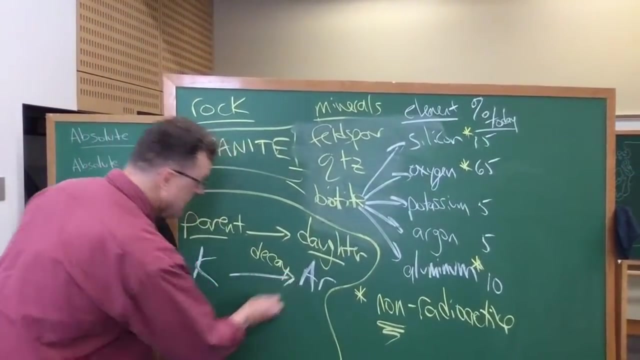 And you are not going to be totally happy with yourself unless you change into that other body. What's the chemical abbreviation for potassium K? What's the chemical abbreviation for argon Capital A lowercase r? There's an isotope of potassium that decays. 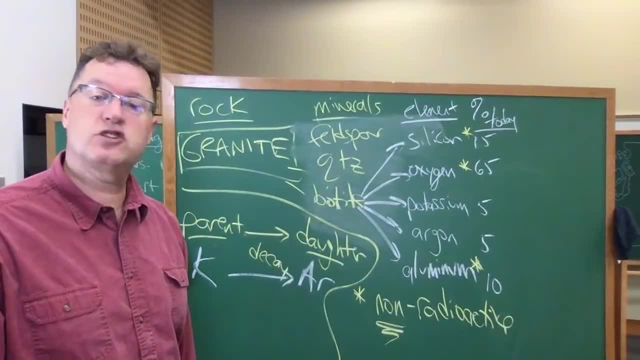 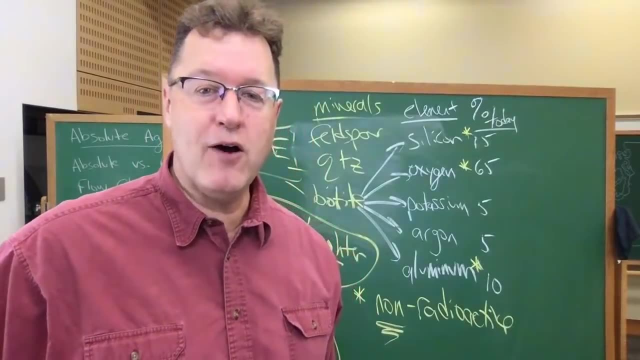 into an isotope of argon. It even gets stranger because potassium is solid and argon is a gas. Why is this happening? Nobody knows, But it happens at a constant rate And it's been measured in laboratories around the world for a long time. 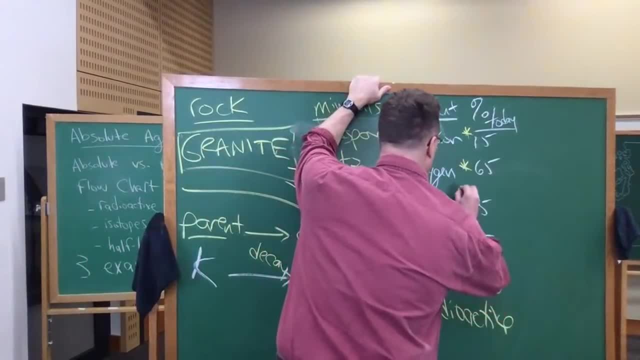 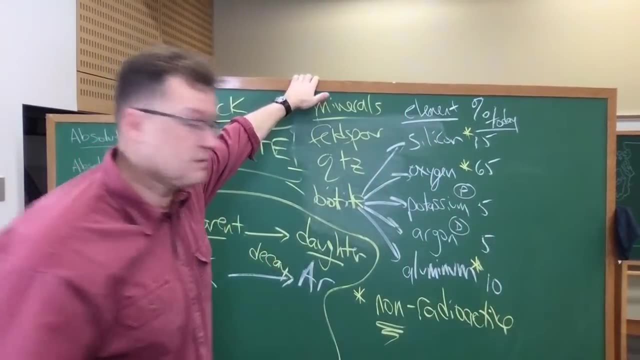 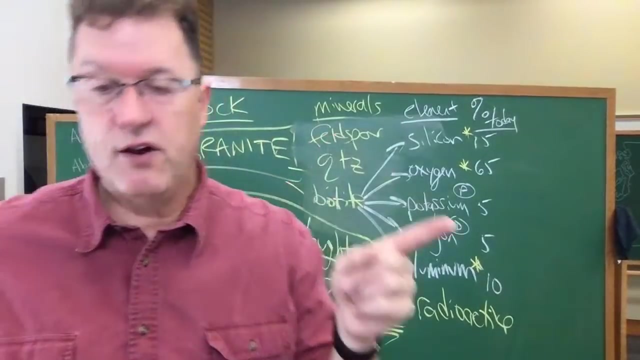 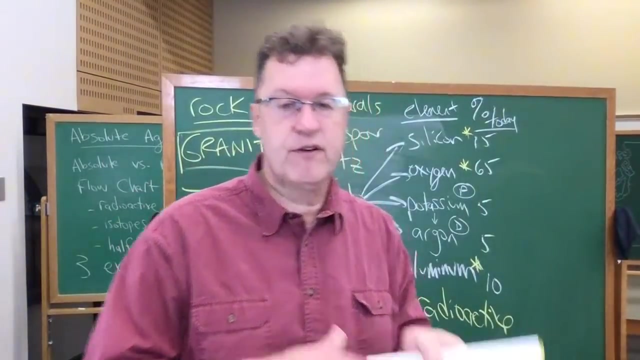 So we do have a parent and a daughter in the same black speck, And we know that it's the parent potassium that's decaying into the daughter argon at a constant rate. Now we circle back to half-life, And half-life is talking. 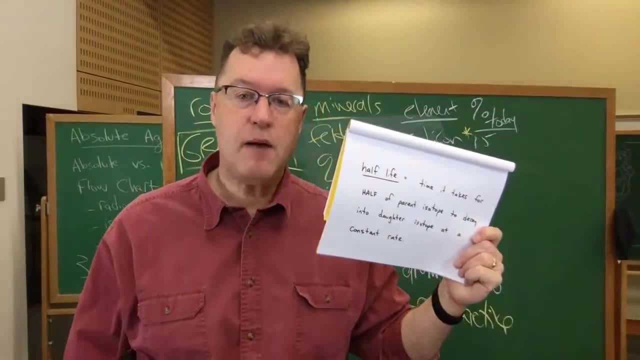 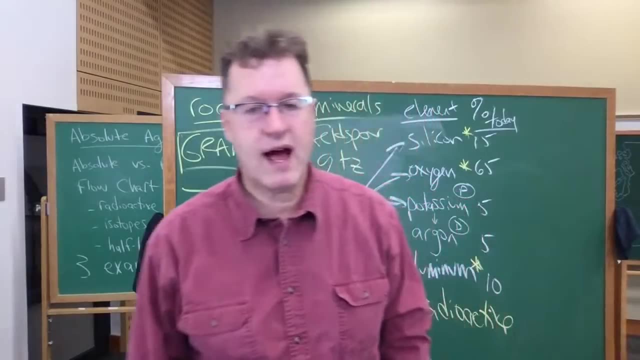 about the time that it takes for that decay to happen. There is this analogy of an old-fashioned- what do they call them- hourglass sand, going from the upper half of the hourglass and going down to the lower, like olden days. 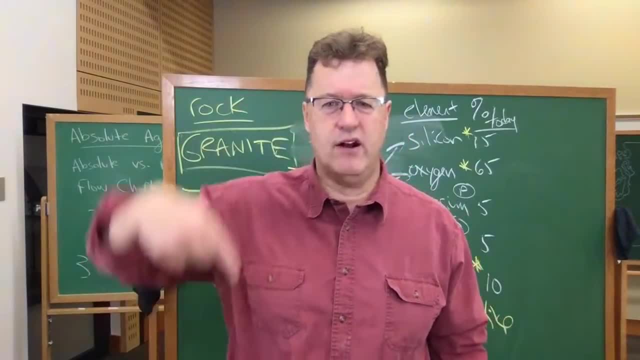 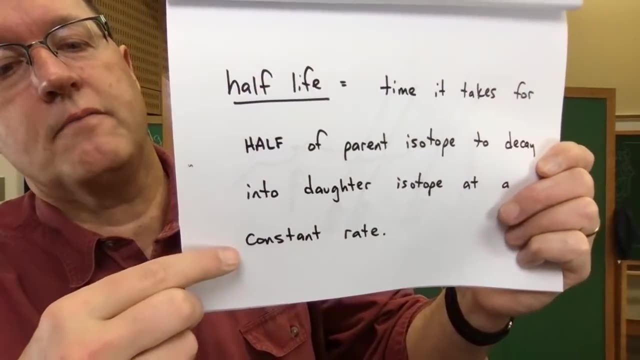 keeping track of time, what as the world turns, I don't know, But the idea is that there's this steady forget it. I don't even know how to describe the thing if you don't know what I'm talking about. 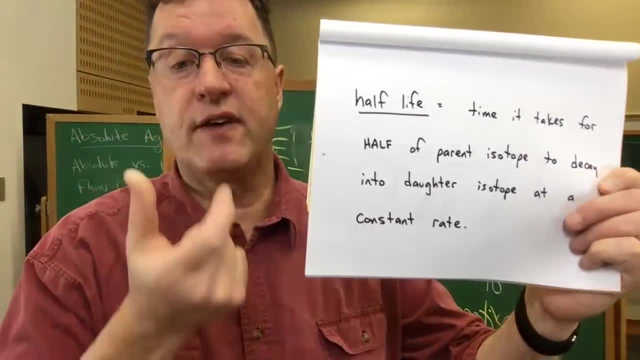 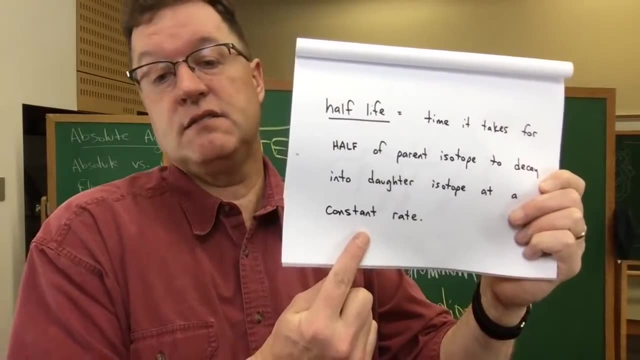 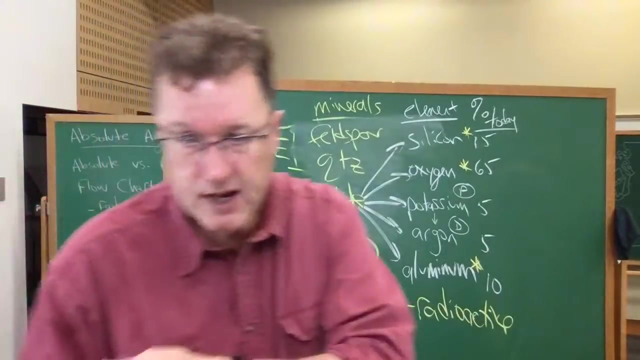 Half-life is the time it takes for half of a given amount of parent to decay into the daughter, And by measuring these processes for the last hundred years in laboratories around the world. and it's not just potassium and argon, there's rubidium decaying into strontium. 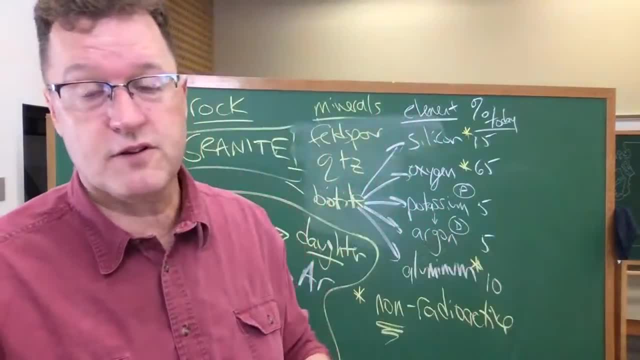 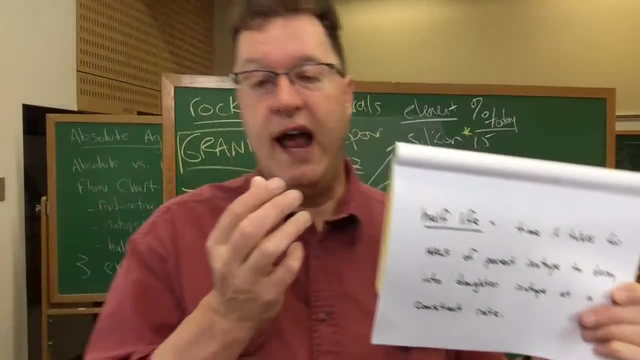 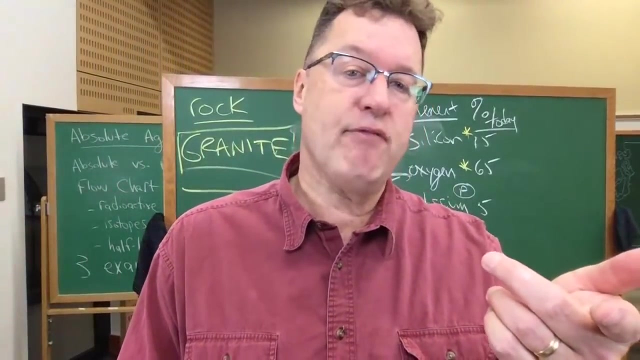 there's uranium decaying into lead. certain isotopes of those elements do the same thing. The half-life is the time that it takes for half of a given amount of parent to decay into the daughter. You are not expected to calculate the half-life. 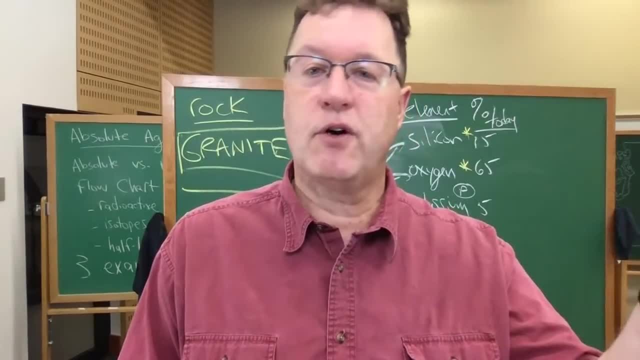 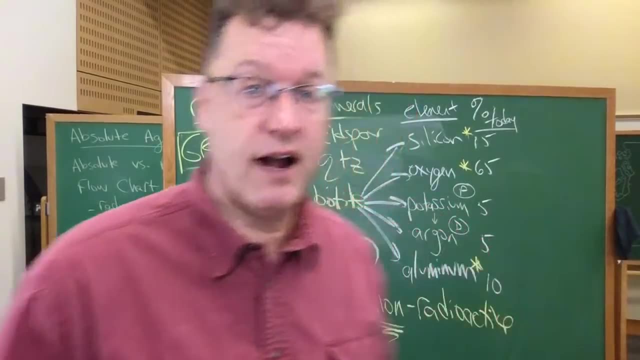 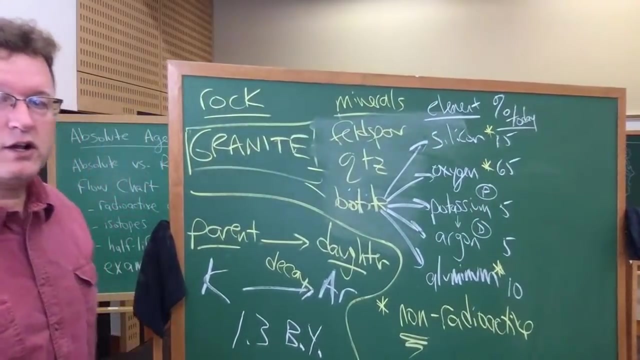 That's been done for you. That's the careful work of laboratory people around the world for more than a century. Here's the half-life of potassium decaying into argon for our problem, Good Lord. 1.3 billion years with a B. 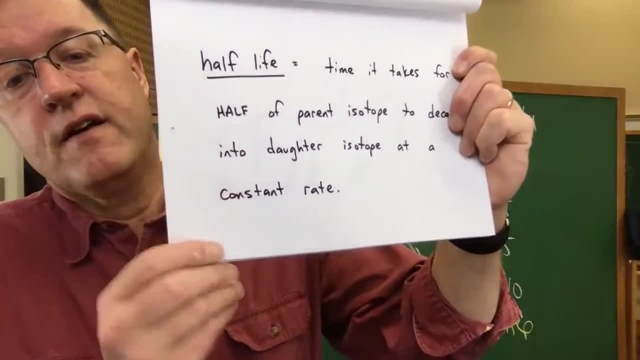 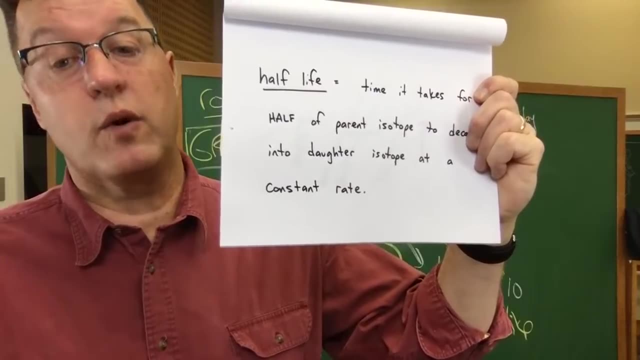 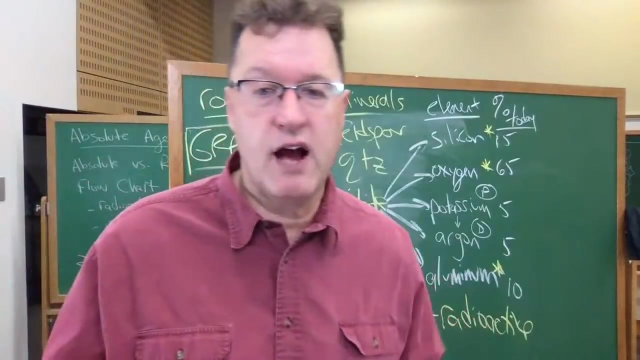 Billion years is the half-life for potassium to decay into daughter, For potassium to decay into argon, In other words, the parent decaying into the daughter And the half-life uranium going into lead, etc. You can Google half-life. 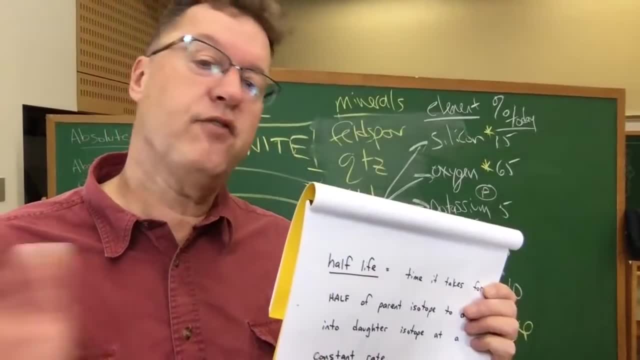 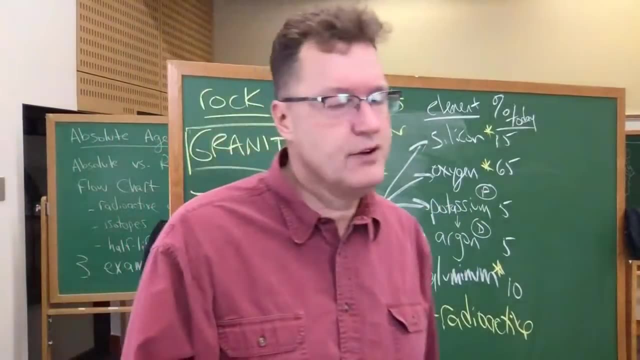 You can find all these different parent-daughter pairs and the half-lifes that's been calculated for them. And we're deep in the weeds now, aren't we? How are we ever going to solve this problem? Don't give up on me. 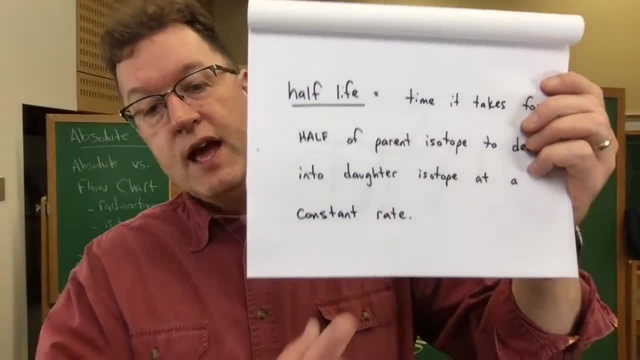 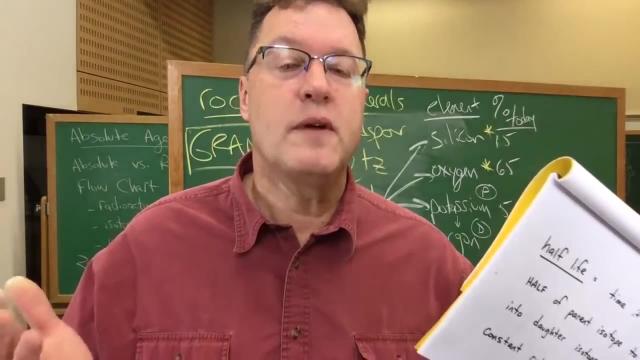 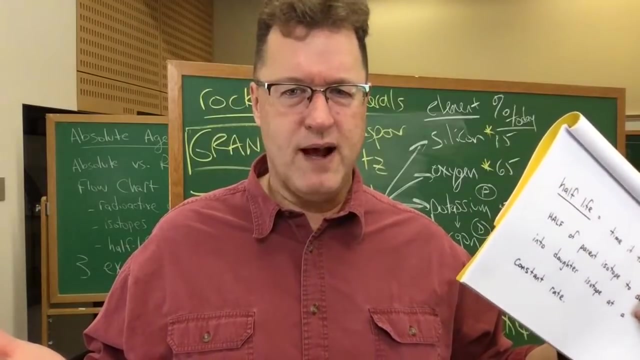 We're going to do it quickly. right now, Half-life constant rate. We use uniformitarianism, by the way, to you might go. how do you know? it takes a billion years. We've only known about this radioactivity. 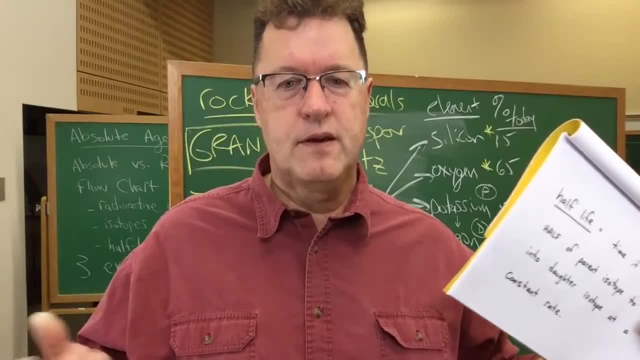 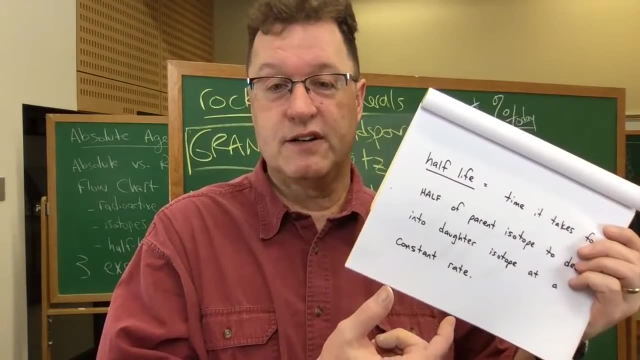 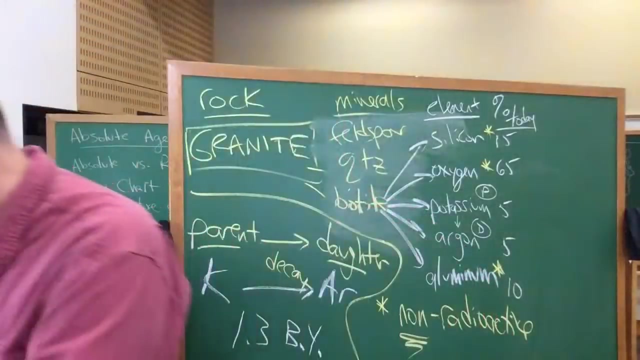 for a little more than a century. You take the steady decay rates measured today for the last hundred plus years, you assume that's a uniform decay rate and therefore you come up with these numbers. Okay, That was the heady part of today. 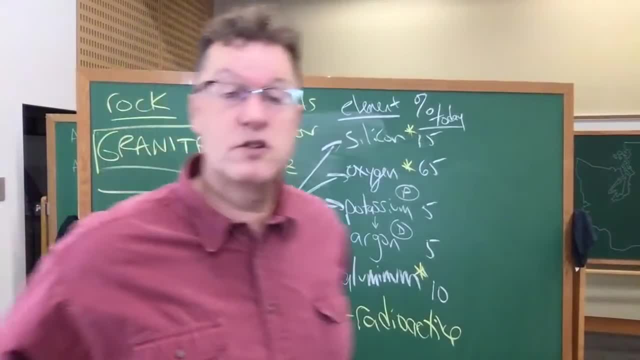 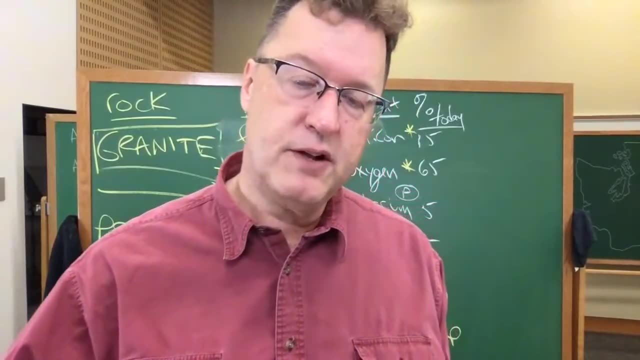 Let's get back to practical stuff And students. this is what you will be doing on our first quiz and our first midterm exam. We'll start talking seriously about those midterms and evaluation of your performance next week. Too early for that, Okay. 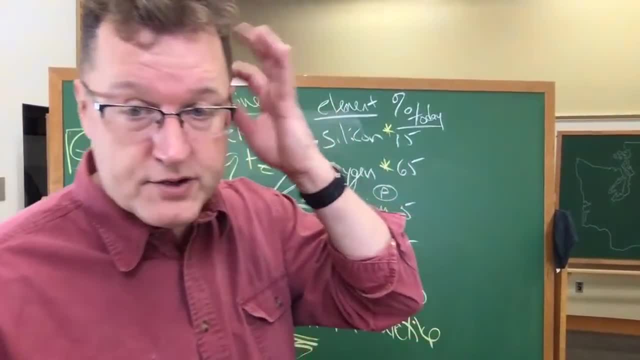 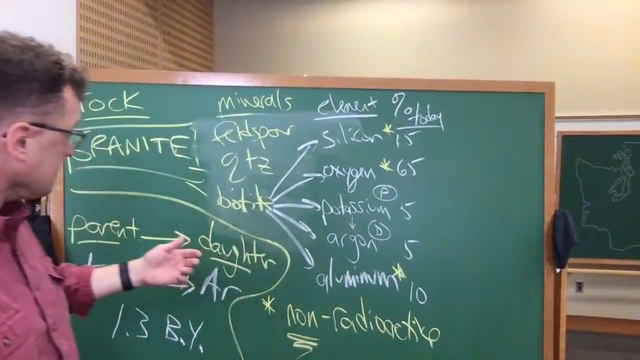 But this obviously is a big day and it'll be a big part of our midterm. Okay, So I have, so let me coach you up now. Okay, So on an exam, I will tell you the elements, I will tell you the parent. 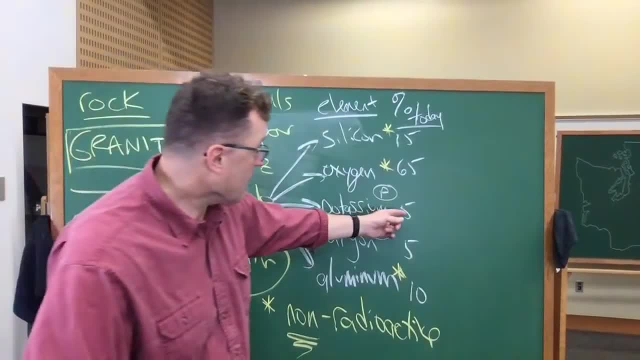 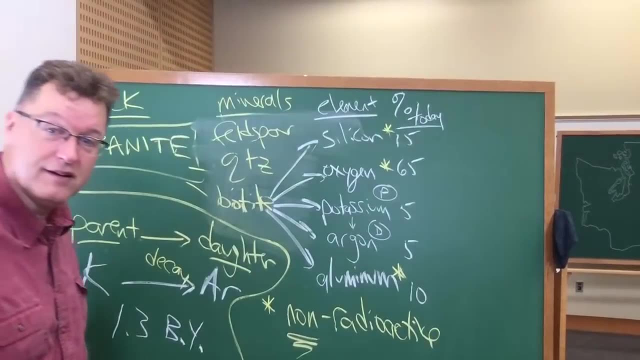 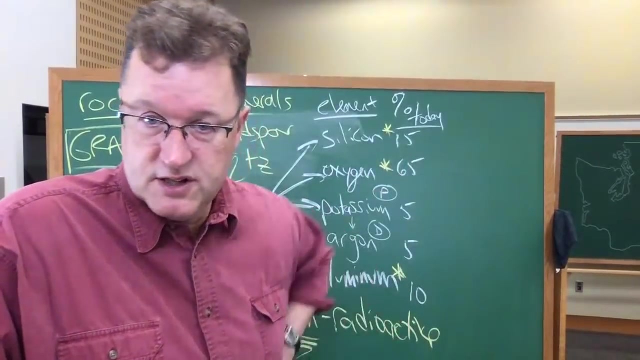 I will tell you the daughter, I will tell you how much parent and how much daughter in that sample And I'll tell you the half-life. I probably won't use potassium and argon, I'll use something else, But the process is what you want. 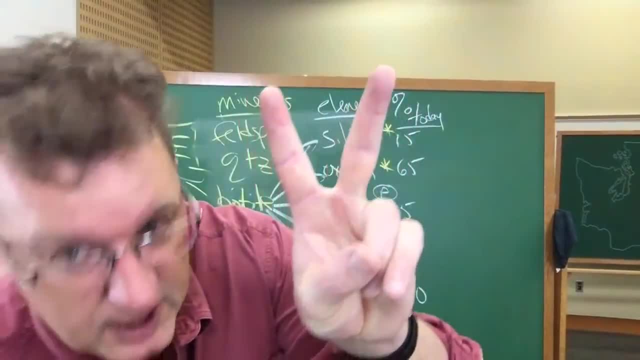 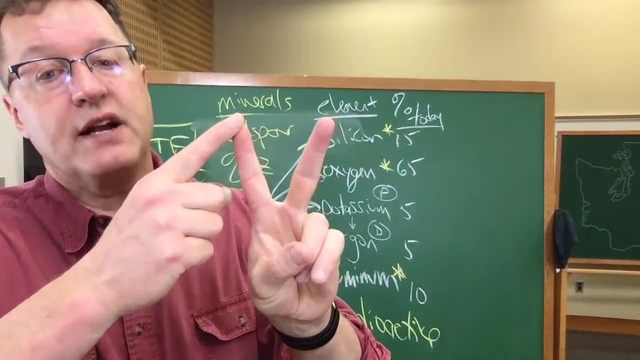 So here are two steps to success. I'll give them to you verbally and then I'm going to do it quickly in the last eight minutes. Step one: make a second column of percentages. I'll do it right now. Make a second column of percentages. 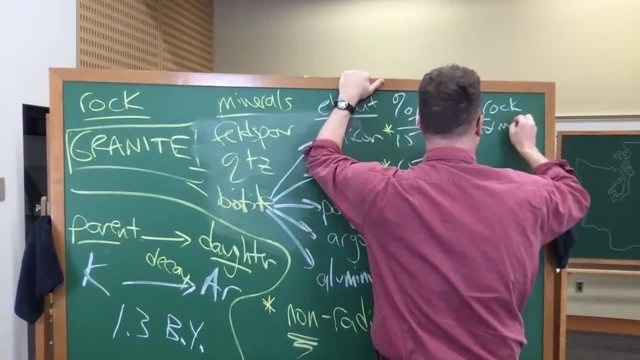 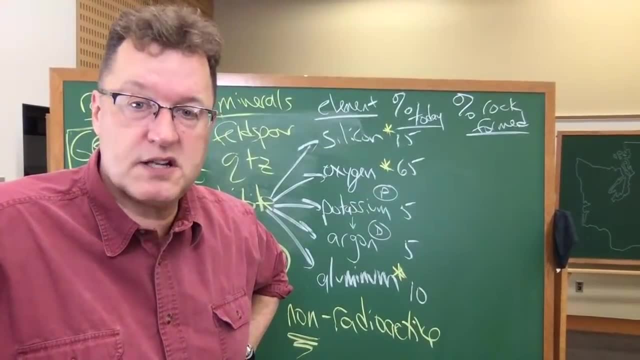 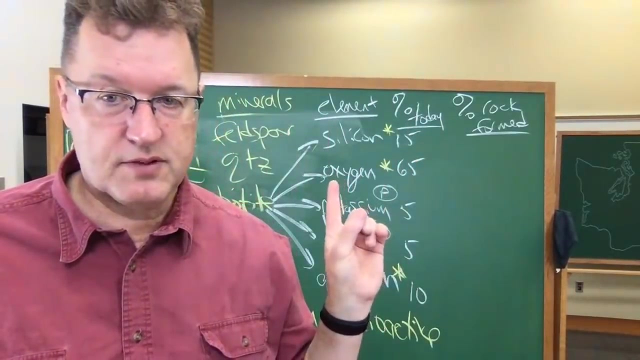 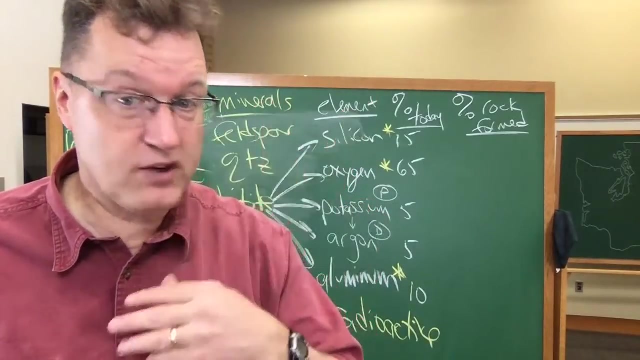 for when the rock formed. The numbers are going to be slightly different. I'll do it in a second. Second and final step. compare the parents in both columns and calculate the age of the rock. Two-step process. I have to give you a bunch of this on the quiz. 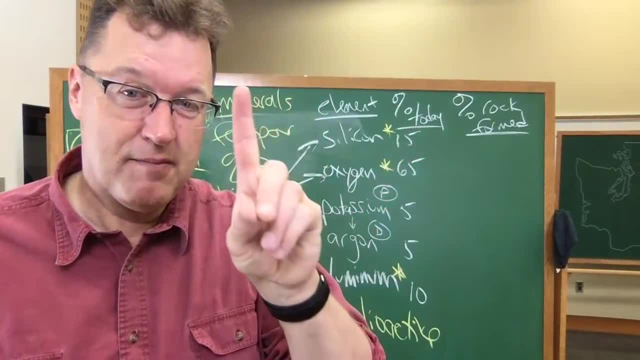 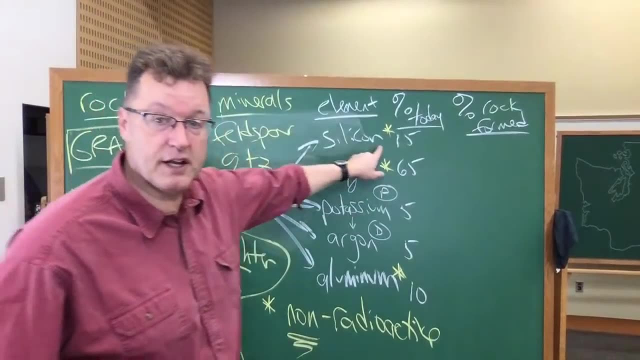 but you have to do the two steps. Make a second column of percentages, Compare the parents in both columns. Let's do it. How much silicon in the original rock Fifteen? Why Silicon is non-radioactive. It doesn't change. 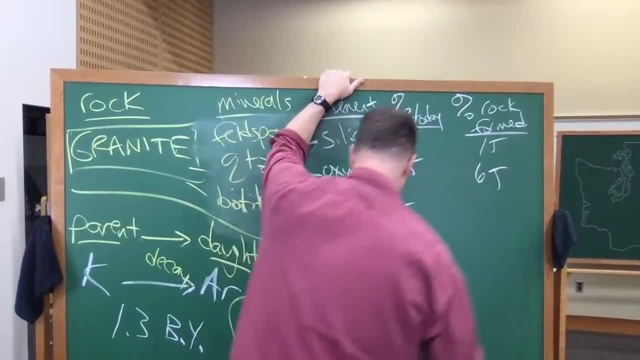 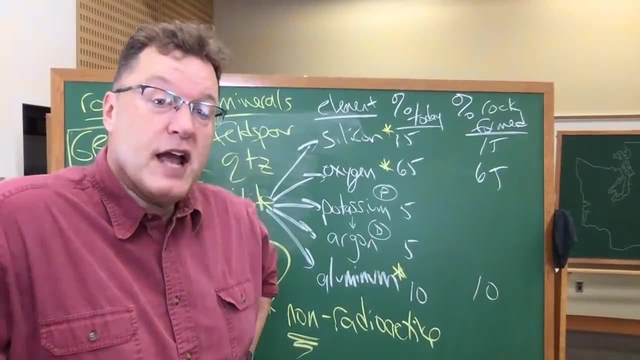 It doesn't decay. Oxygen 65.. Aluminum 10.. Those are non-radioactive elements. They do not decay. They're not going to change their percentage in the black biotite spec, Unhelpful to us. We move on. 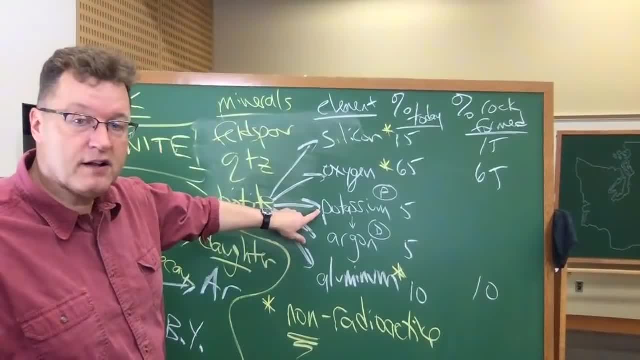 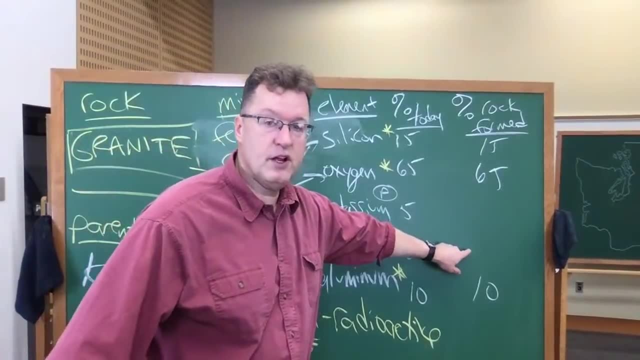 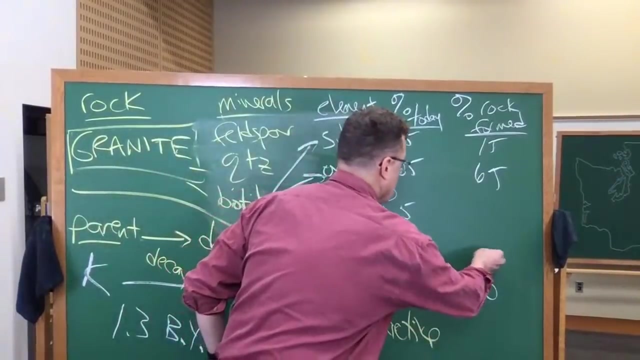 Harder question: This is parent, This is daughter. Potassium decaying into argon: How much daughter in the original black biotite spec Correct Zero For our purposes? this is kind of a fudge. now This is geology 101,. 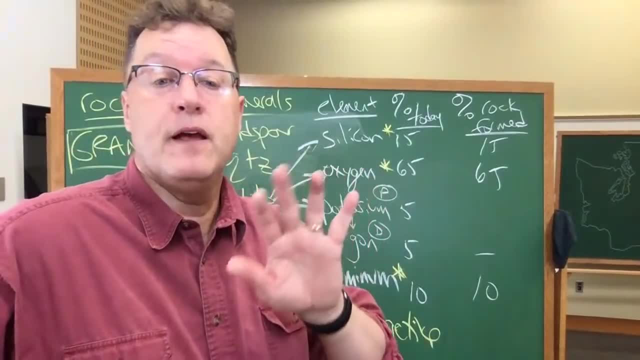 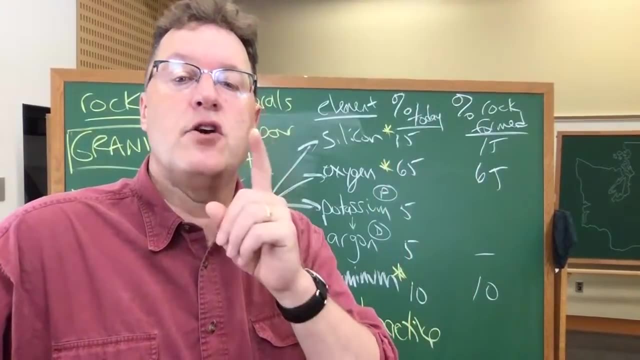 and this doesn't technically work the whole all the time. But for us we're going to have to round a few corners here to make this work. for us non-science people, Here's the rule: There's never any daughter in the original rock. 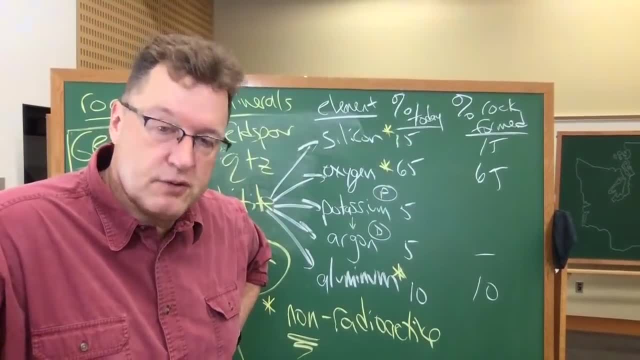 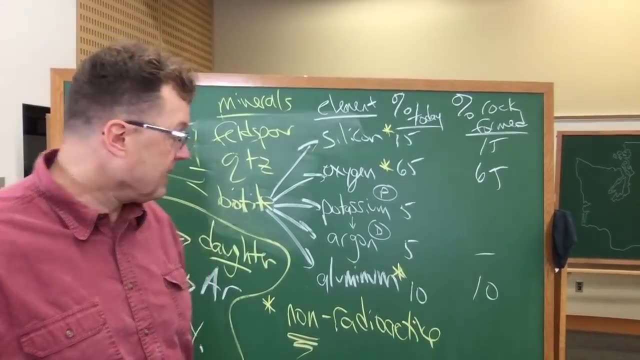 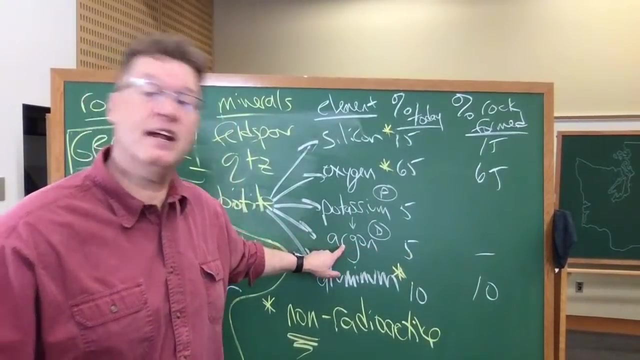 There's never any daughter in the original rock. Please write that down. There's never any daughter in the original rock for our purposes in this 101 class. Because what is this 5% argon? It's 5% potassium that has decayed into argon. 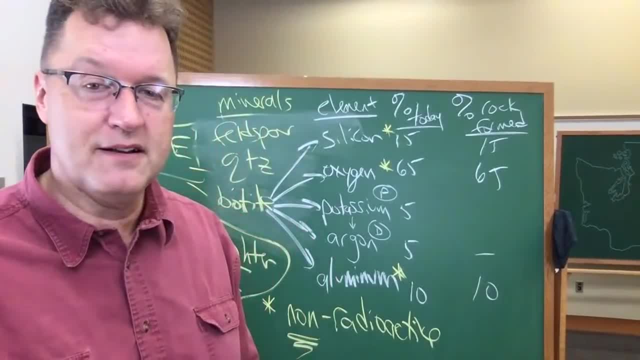 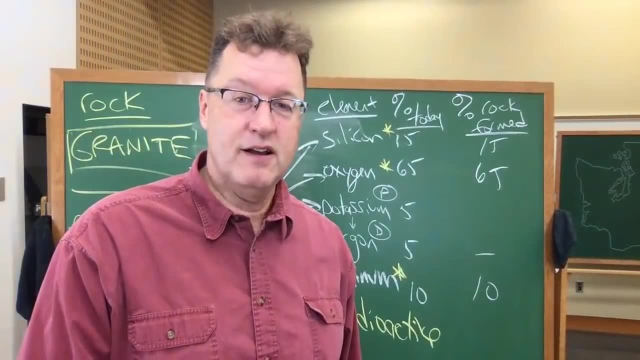 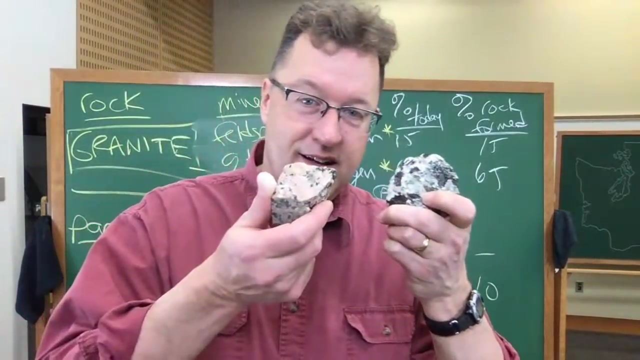 since the granite was created. So if we view this daughter as the result of radioactive decay- which we should- and if radioactive decay is only happening when the granite exists, then it's the decay itself that's keeping track of time for us. So there's never any daughter. 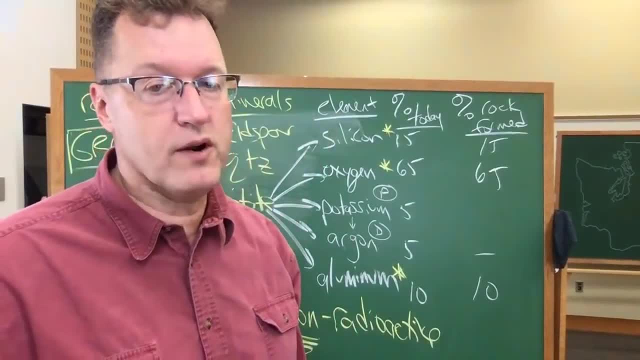 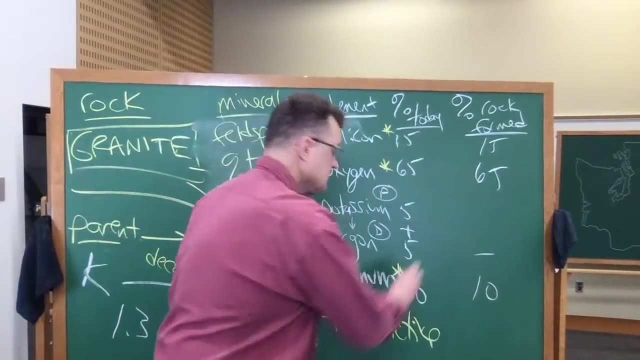 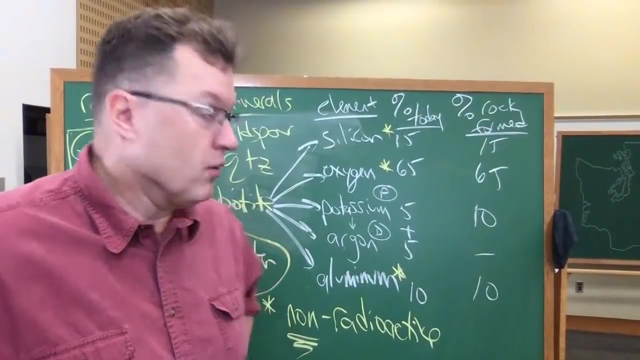 zero daughter in the original rock, And that's an important step, because then what is the last number? here We're going to add the parent and the daughter together to get the original amount of parent. We have completed step one. We have made a second columnary column. 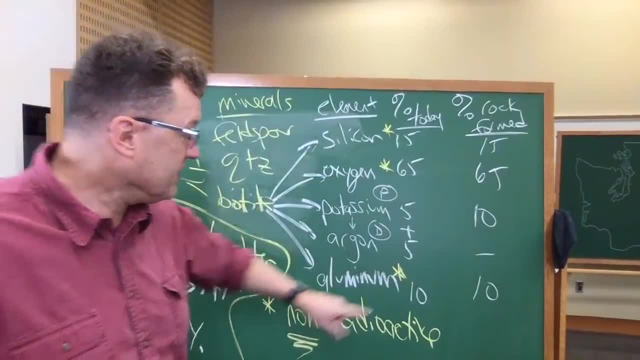 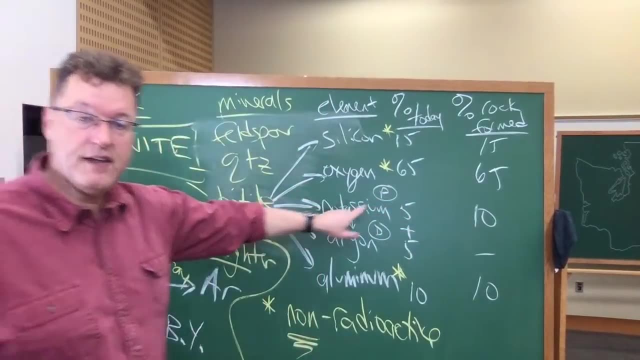 of percentages for when the rock formed. And, of course, the only difference is we never have any daughter in the original rock and we get the original amount of parent, the original amount of parent in this granite number one, by simply adding parent and daughter together. 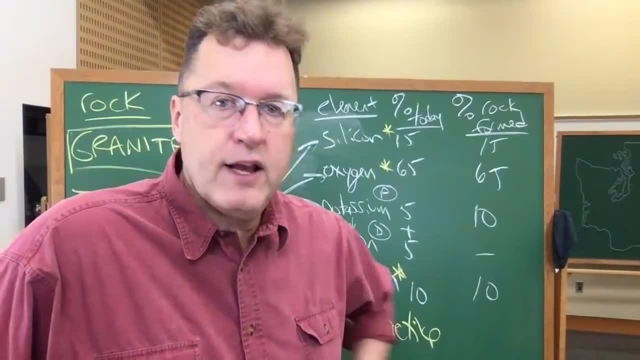 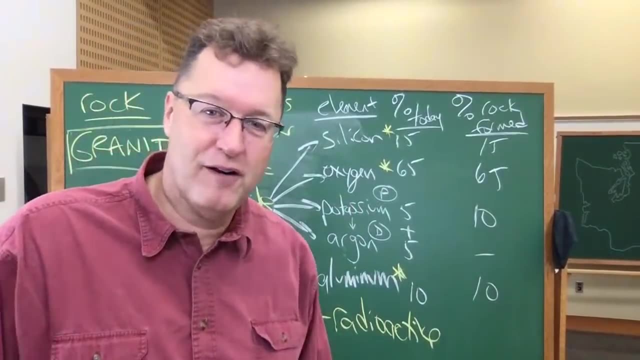 You want a pro tip, I'll give you half the credit for the problem on the midterm. if you simply add the parent and daughter together, You can screw up the rest of it. I don't care, I'll give you half the credit just by saying. 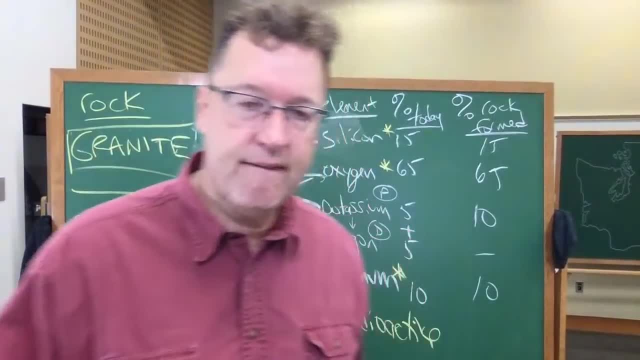 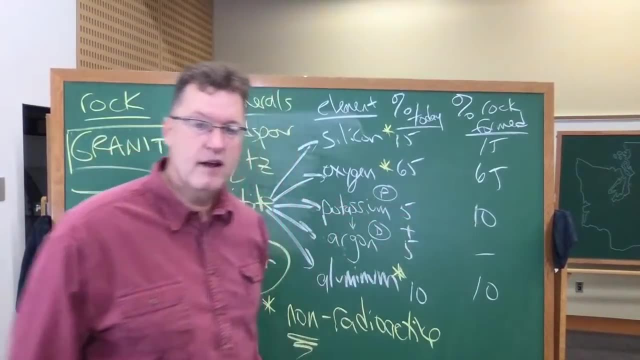 that's the first step. I'm just going to find the parent and the daughter and add them together. Whether you even understand why you're doing it or not doesn't matter. I'll give you half the credit. Add these two guys together and get the original parent. 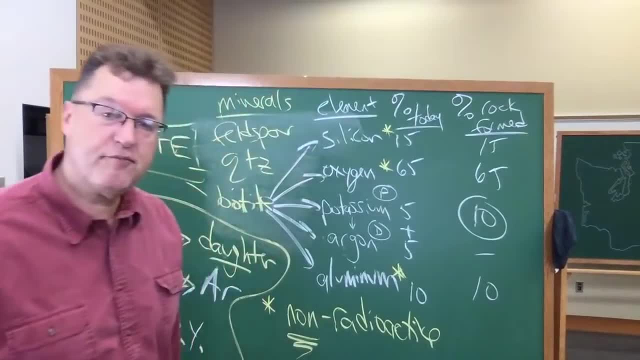 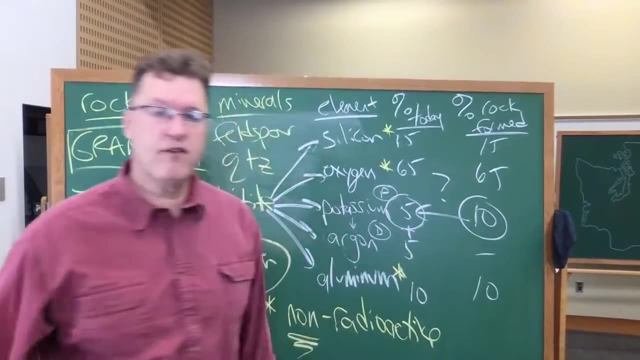 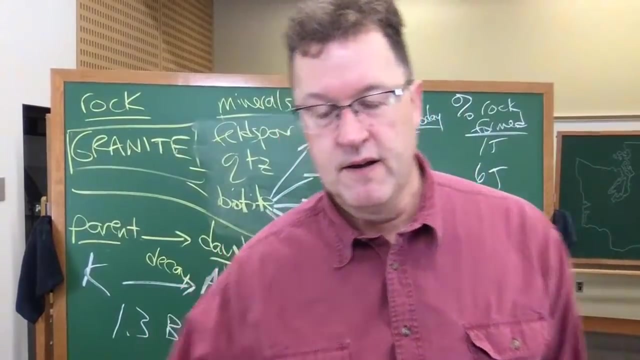 What's the second and final step? Look at the original amount of parent. Look at the current amount of parent. Ask yourself how long did it take to go from originally 10% parent down to 5% parent? I made the first example. 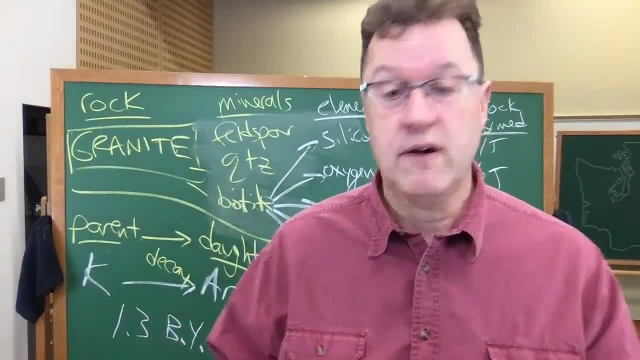 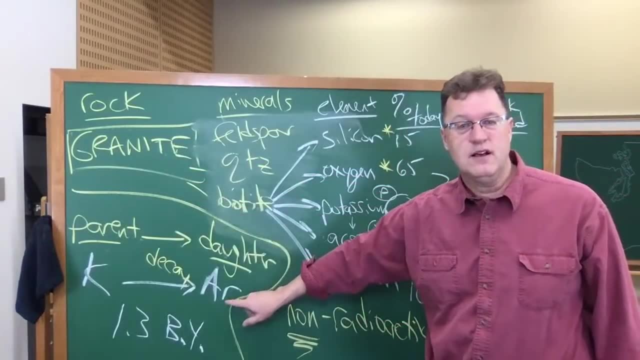 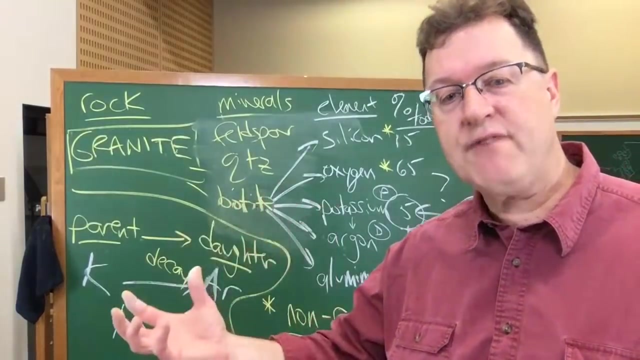 as easy as I possibly could Correct. What did I do? I selected a granite that has an age that is precisely the same as one half-life, Because what's the definition of a half-life? The time that it takes for half of the given amount of parent. 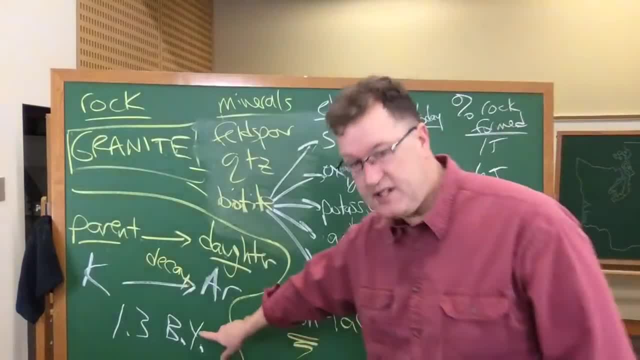 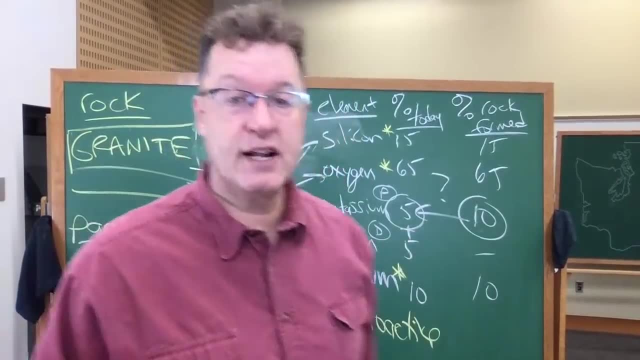 to decay into the daughter. This is the half-life of potassium-globulin. a potassium going into argon Five is half of ten. So what is the answer? We're at the answer. What is the answer for granite number one? 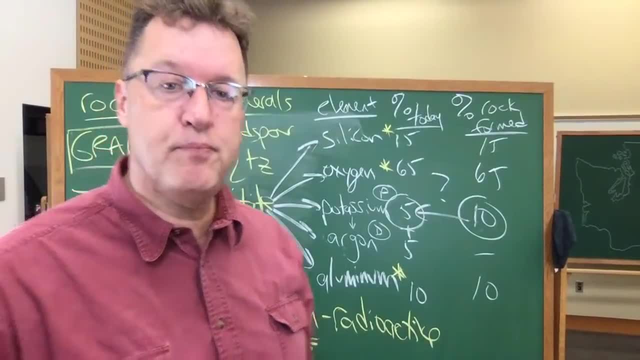 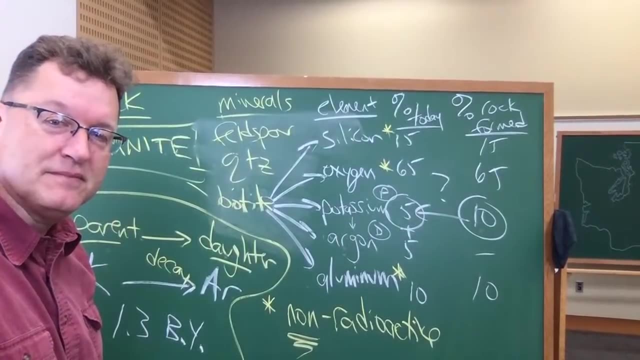 1.3 billion years. It's a granite that's 1.3 billion years old because of five being half of ten And it takes 1.3 billion years to go from ten down to five. I don't have time. 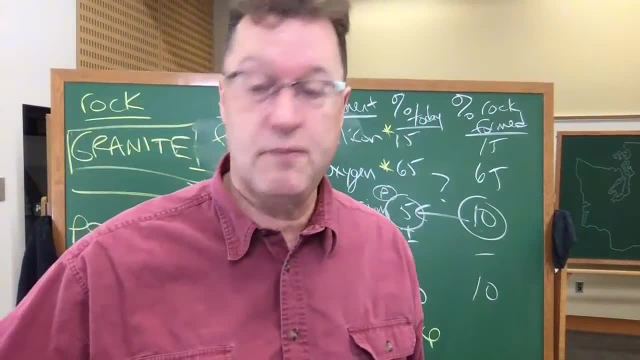 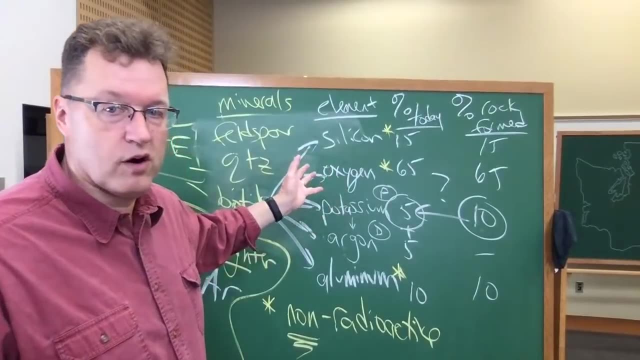 I'm going to go over, by the way. I apologize for that, but I apologize for that. We're going to do two more examples. I'm not going to start over, but the other two examples of the granites. I'm just going to erase this portion. 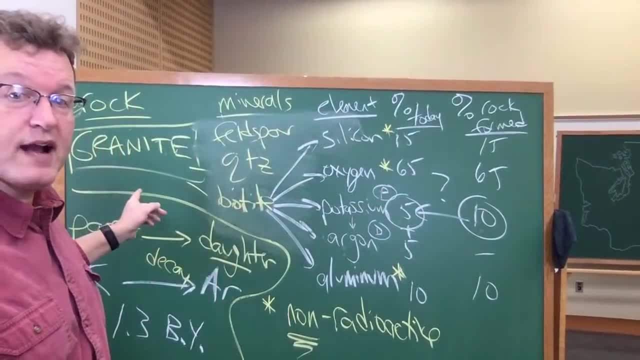 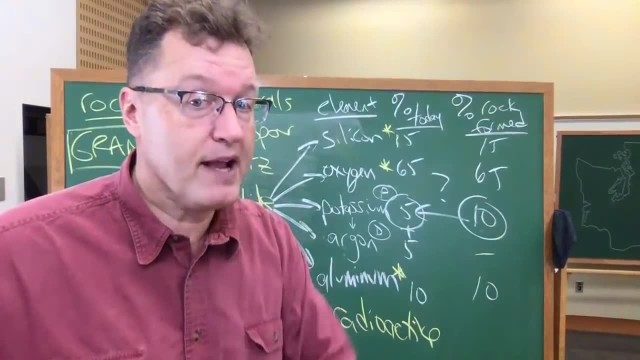 So we're going to have for your notes. we're now moving on to granite number two and granite number three. I got a couple twists on this story, but we have the basics right now for how we come up with absolute age dating. 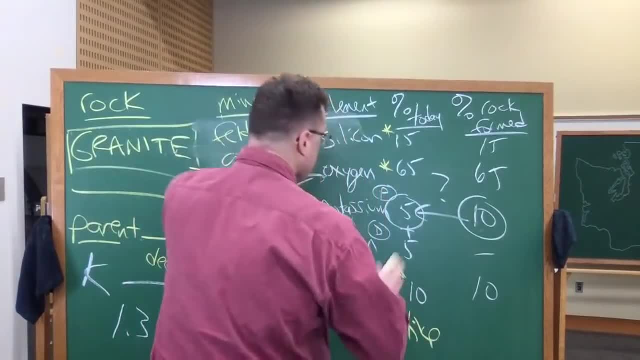 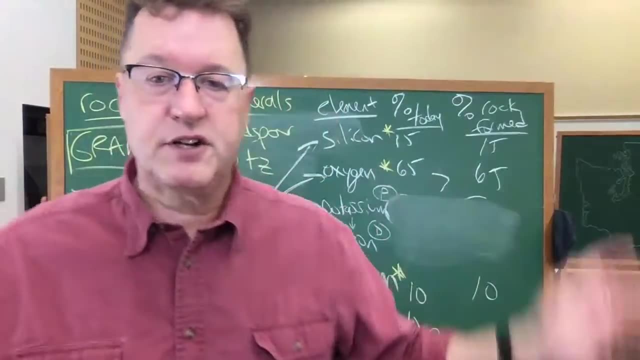 You ready? Okay, Australian eraser, Let's get it. You are now given granite number two. You bust it up, You separate the minerals, You send the black speck to Denver. You get the stuff back. This is a different granite. 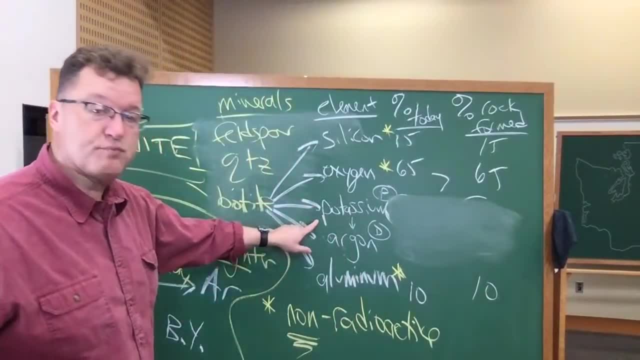 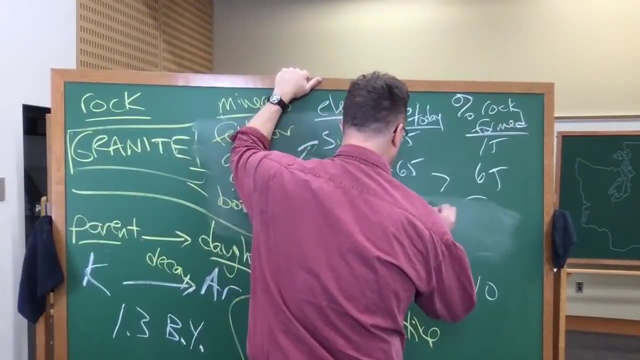 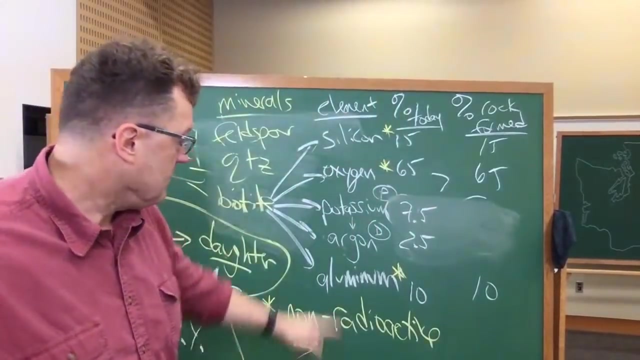 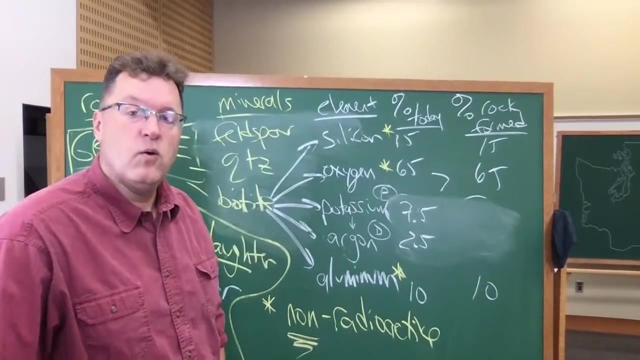 with a different age. right, Let's play with these numbers. In granite number two, there is 7.5% potassium and only 2.5% argon. What's the age of granite number two? I'll give you a second. 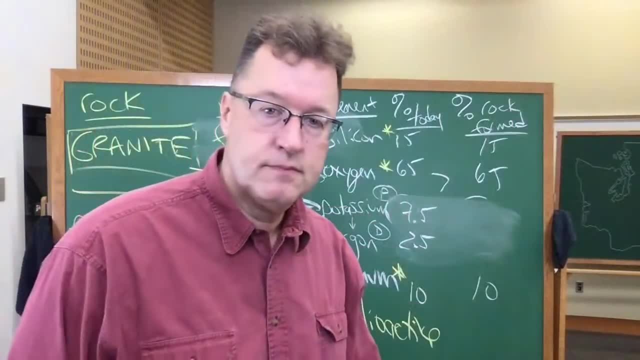 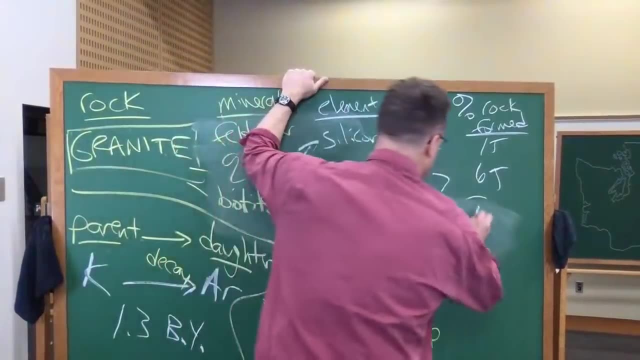 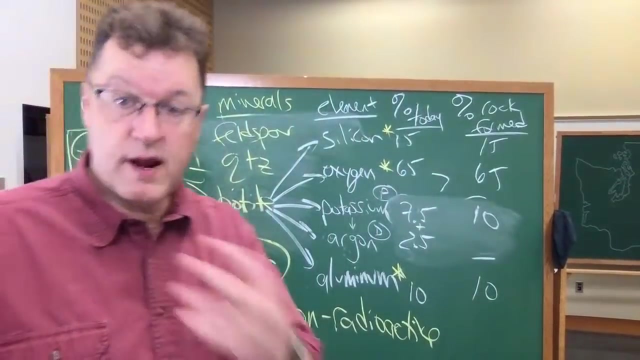 What's the first step? Add the parent and daughter together: 7.5 plus 2.5 equals 10.. How much daughter in the original rock Zero? That's our rule. This granite is going to be, you tell me. 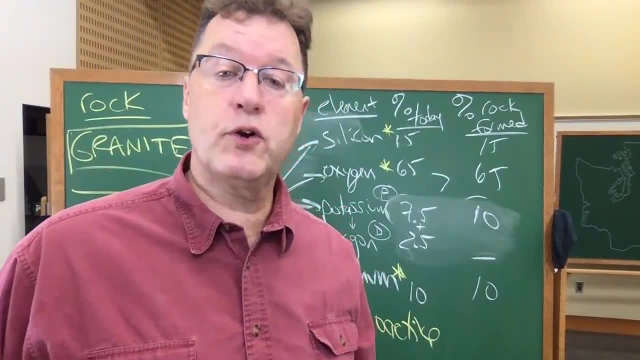 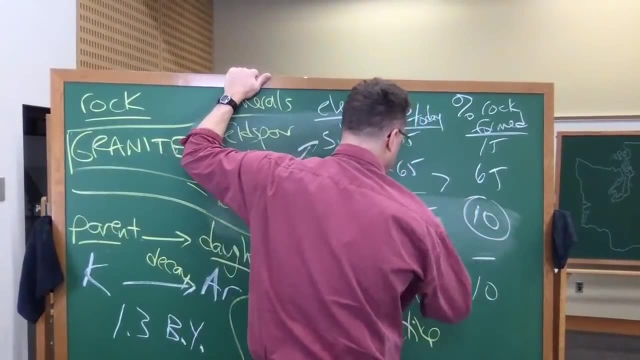 I'm not going to wait, though You tell me, is this granite going to be older or younger than the first example? Because this second step is to compare the parents, And this time we're going 10 down to 7.5% potassium. 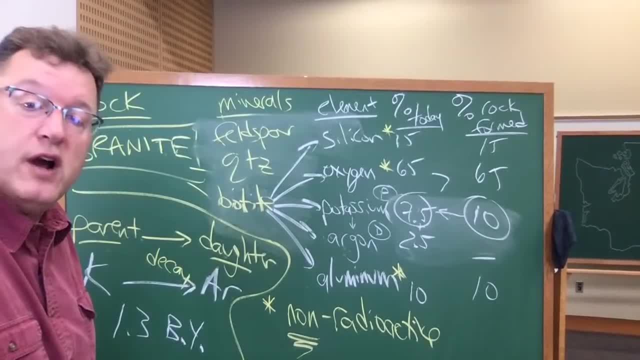 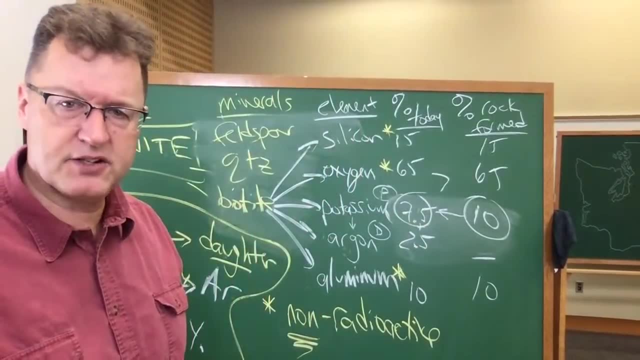 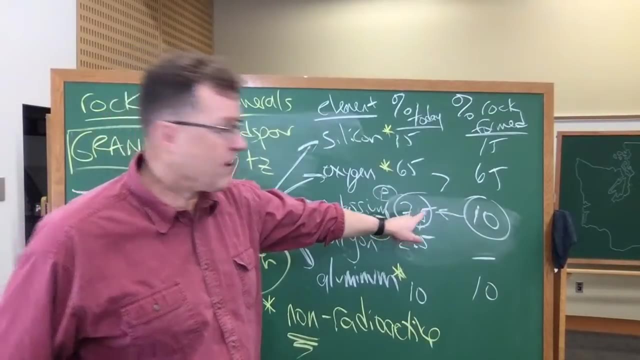 Is our granite going to be older or younger than 1.3?? The answer is younger. Why? Because we're not doing as much decay. Does this make sense to you? We start with 10.. We just start decaying. We start changing the parent. 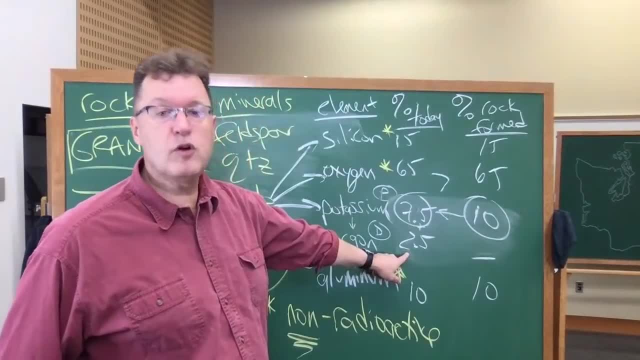 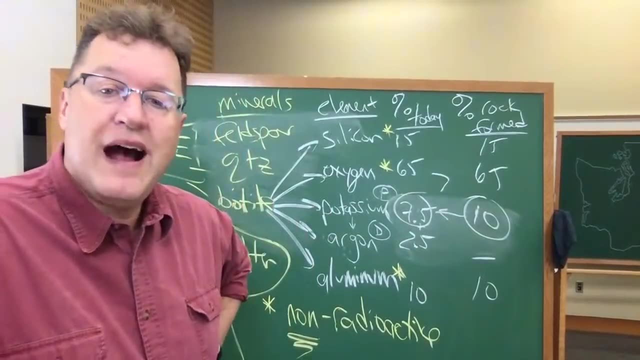 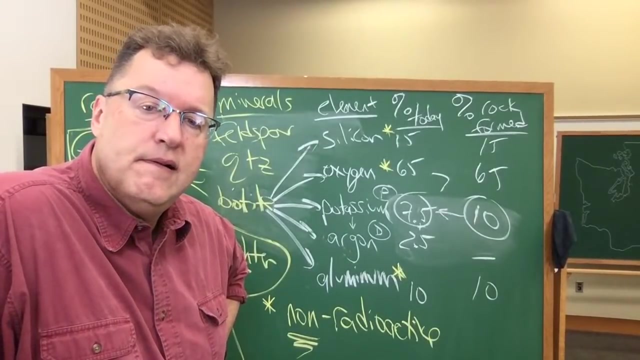 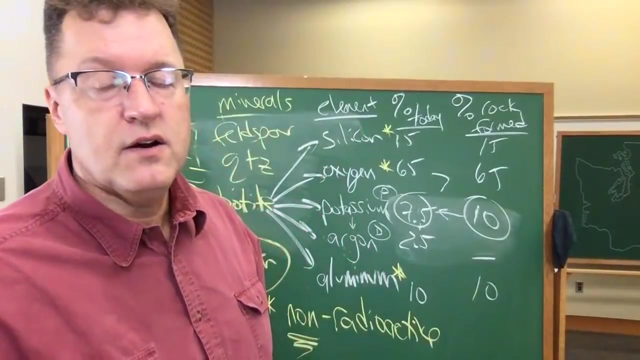 But we only end up with 2.5% daughter. We still have a full 7.5% parent. So how old is granite number 2?? The answer is 0.65 billion or 650 million. And you're like: 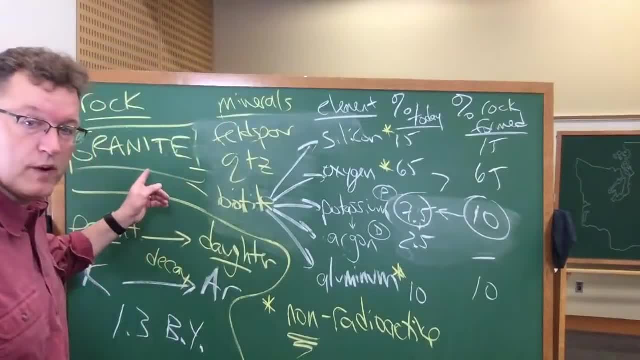 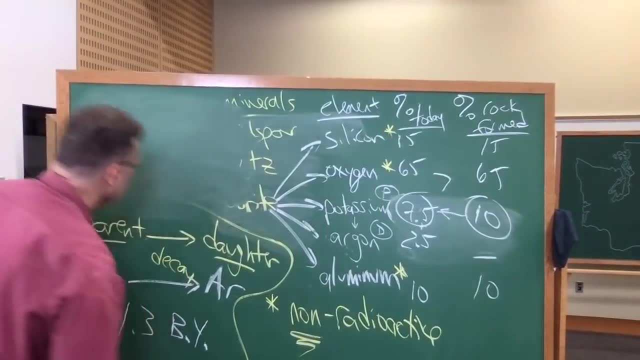 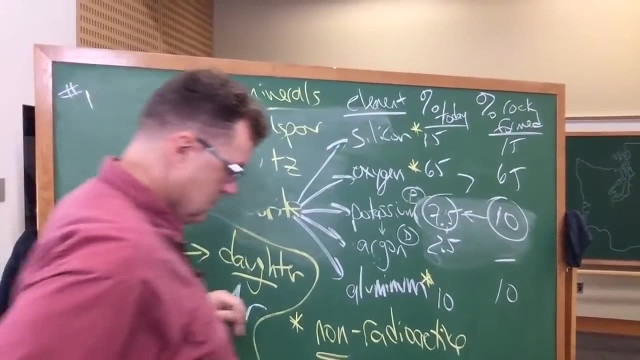 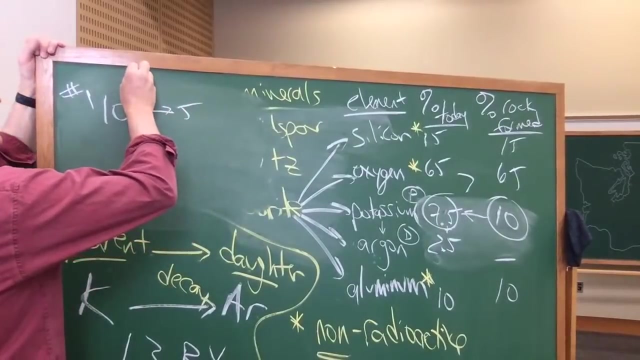 what? How'd you do that? I'm going to erase part of this. I'm going to erase part of this. Example number 1. We went from 10 down to 5. That took 1.3 billion years, Correct? 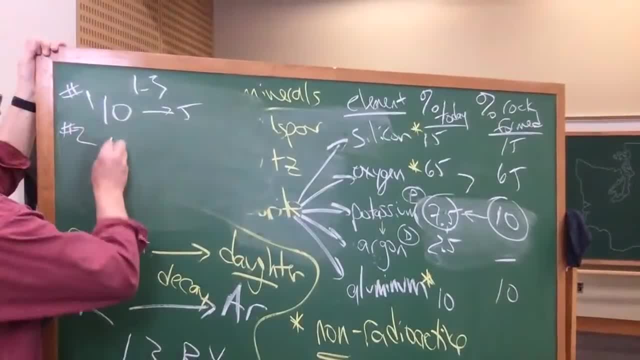 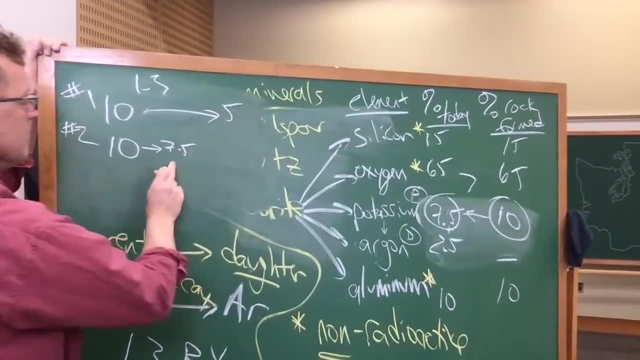 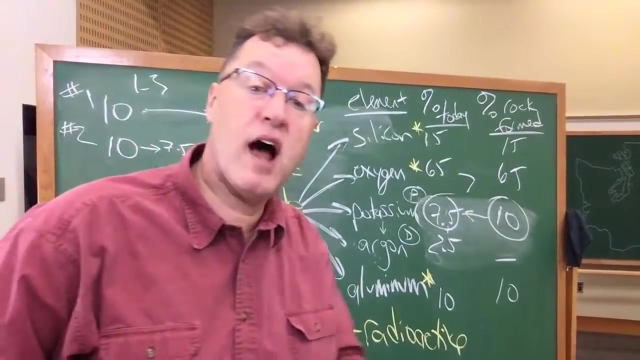 Example number 2. Which we just did together: We start with 10 And we're only going- let me make this bigger- we're only going to 7.5, 10 down to 7.5.. That's not as much decay, therefore. that's not as much time that has transpired. 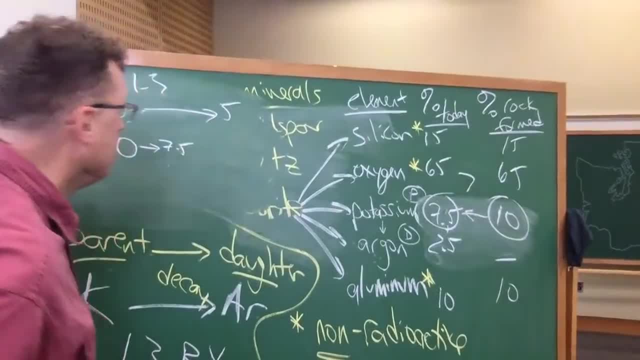 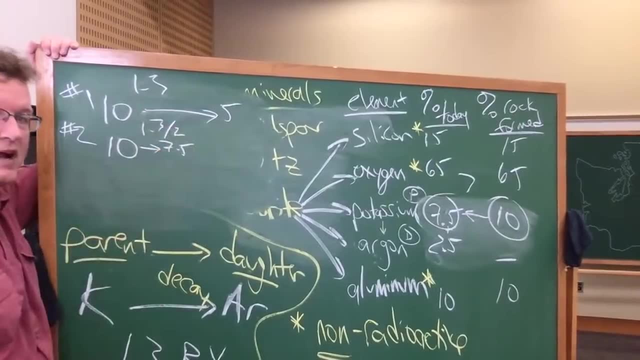 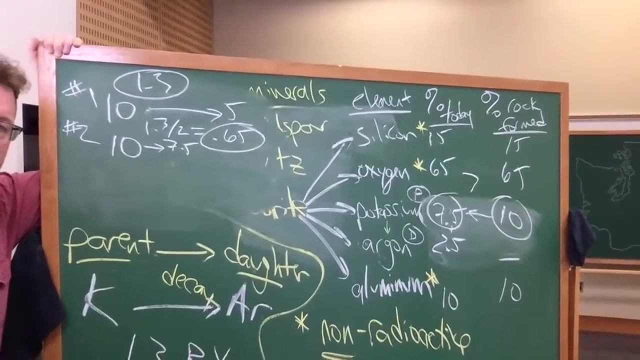 That means this granite is younger than granite 1.. But where did I come up with 0.65?? I took the 1.3 and I divided it by 2. To get an answer of 0.65 billion, which is the same number as 650 million. 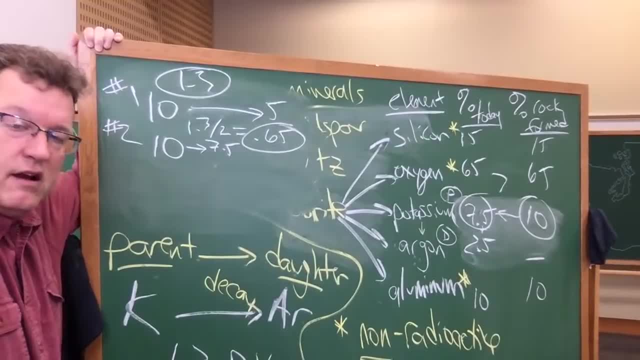 Granite number 2 is 0.65 billion And you're like: okay, I guess I wrote it down, but I don't get what you mean. I'll try an analogy. I don't know if it's going to work. 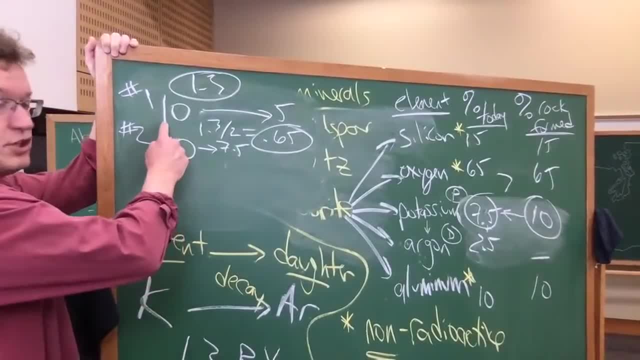 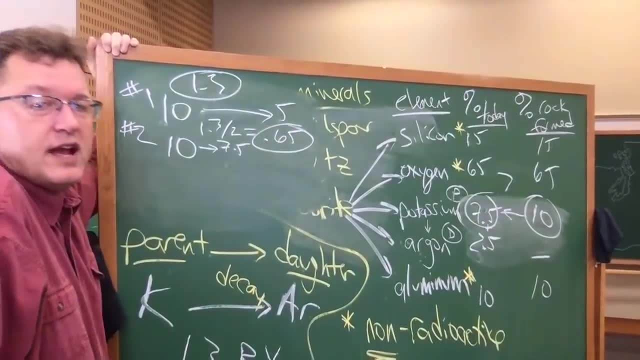 This is for Washington people only. It takes two hours for you to drive from your house in Seattle and come over to Ellen. It takes you two hours. Well, it takes us older people two hours. It takes you two hours to travel from Seattle to Ellensburg. 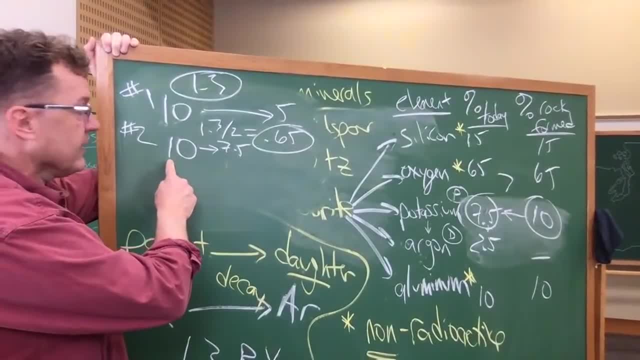 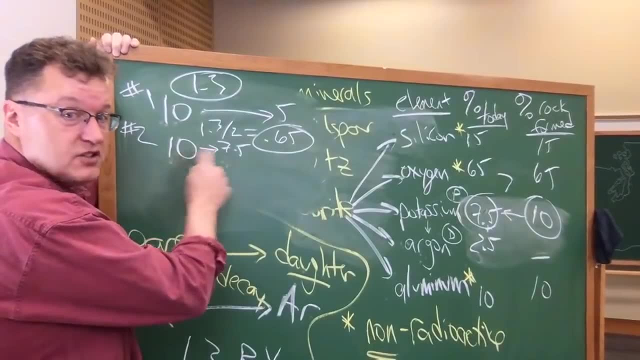 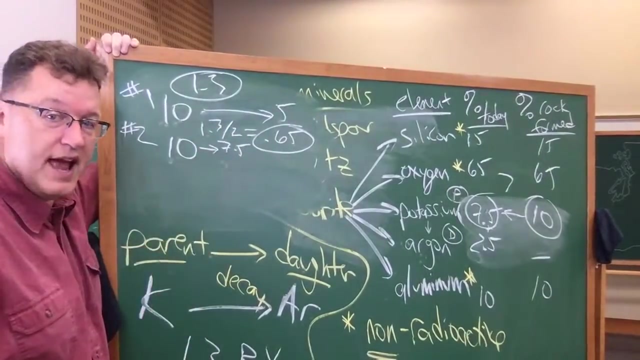 But what if you're not going to Ellensburg? What if you're leaving your house in Seattle and you're going to go skiing at Snoqualmie Pass, which is half the distance? Half the distance means it's half the travel time. That's why we're cutting this 1.3 and a half. 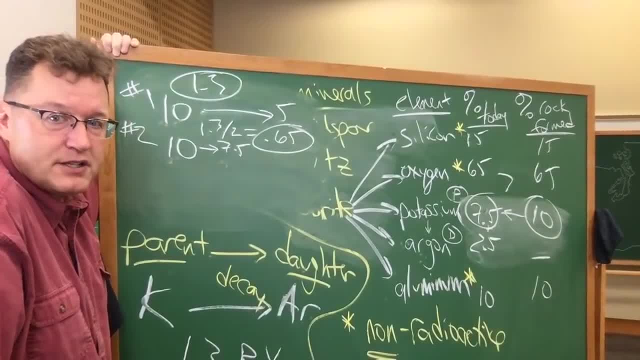 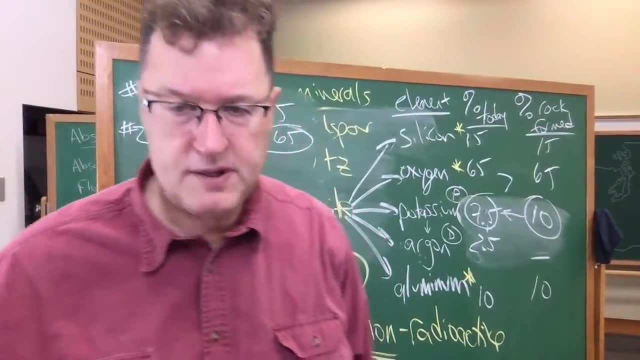 We're going half the distance, We're decaying half as much. That's the best I can do, And some of you are advanced thinkers and you go. well, I think you probably need calculus for this, don't you? This is like a differential thing. 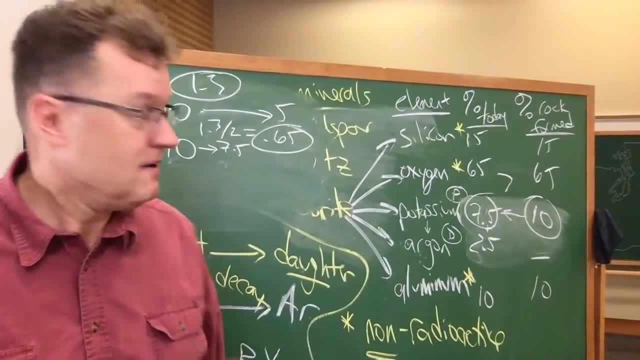 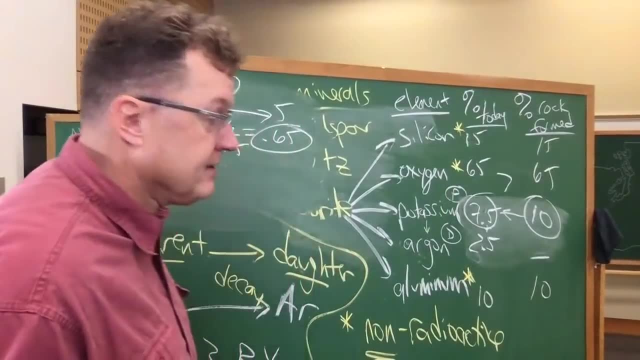 It is. It's a differential equation. We don't have calculus behind us, So we're going to make it like this and hopefully feel like we have the concept anyway. One more example and then I'm done. I did not budget my time this morning. 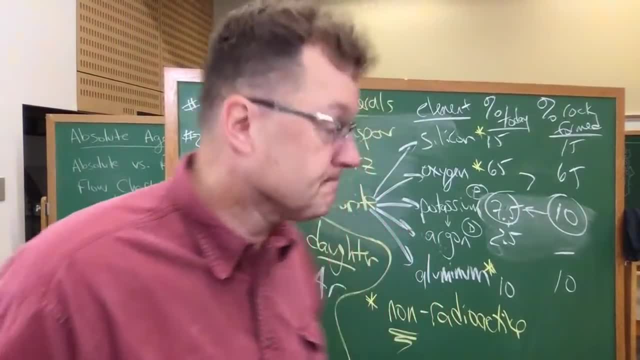 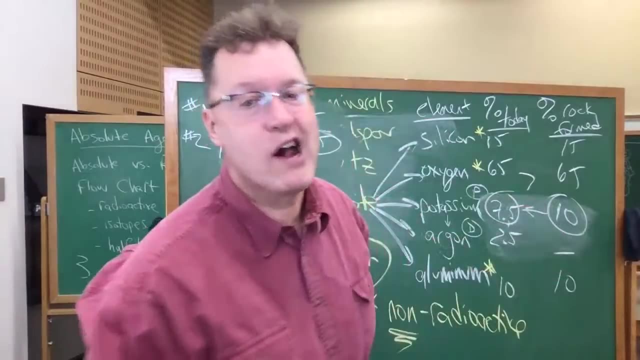 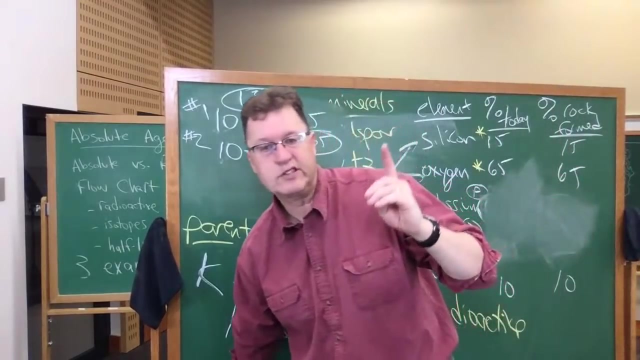 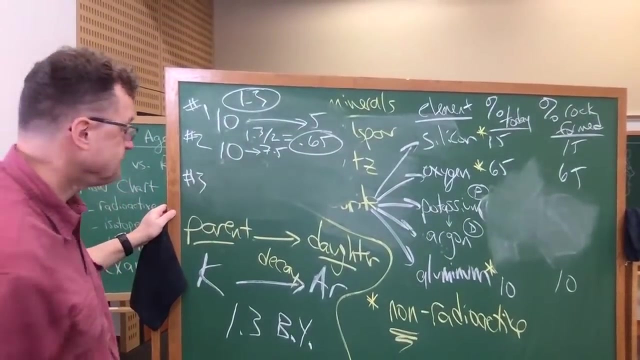 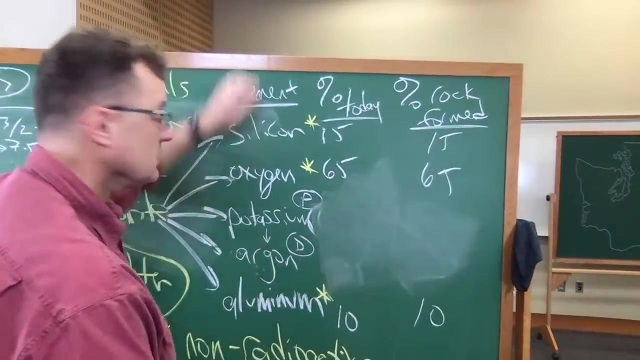 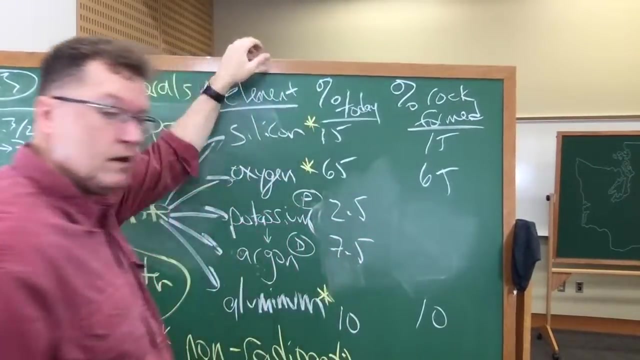 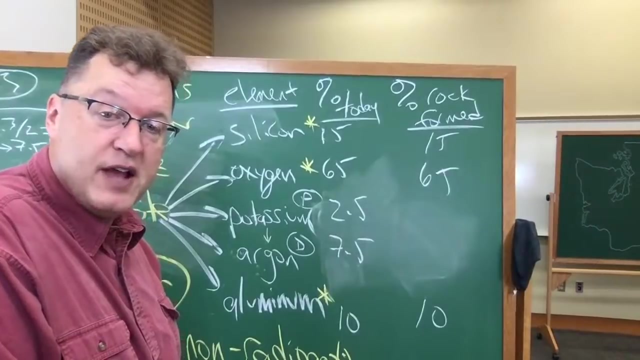 I truly apologize. You're going to have to give me another five minutes. It shouldn't be easy Eating the frickin' rock. One more example and we're done. Flip them For. example three: our last granite to analyze has 2.5% potassium and 7.5% argon. 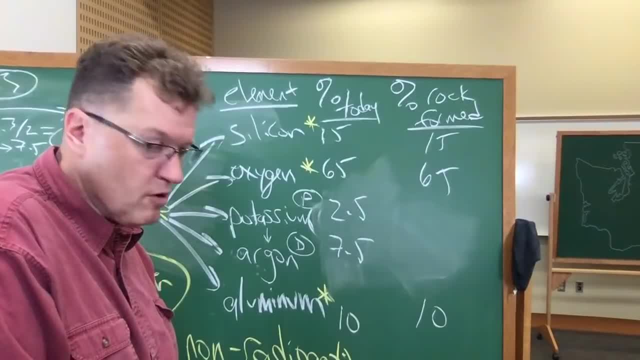 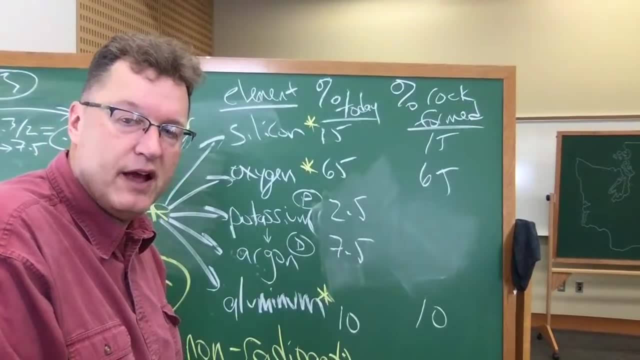 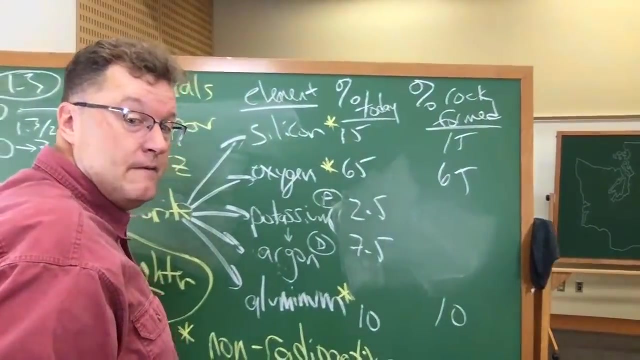 Yes, I'm removing some math here. I'm removing calculus. There's a logarithmic curve. We don't have the background for that And I forgot that math from 40 years ago. anyway, Using our process, can we get an age for this last granite? 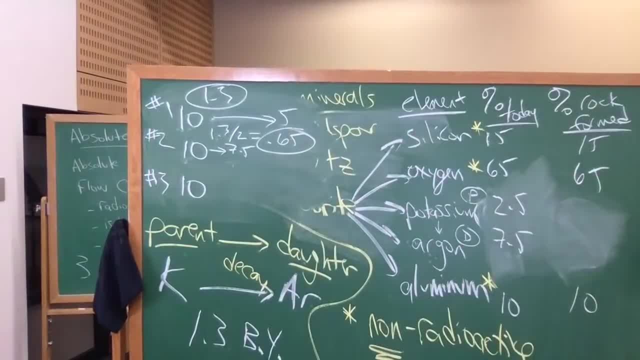 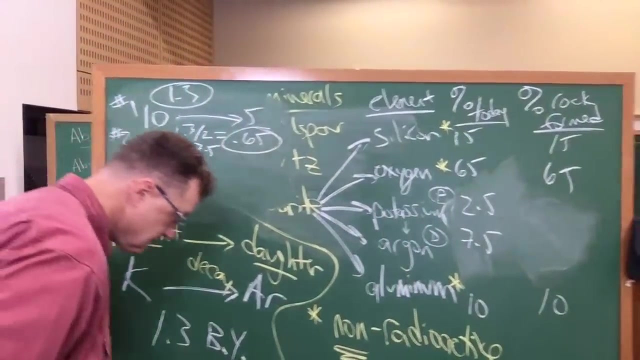 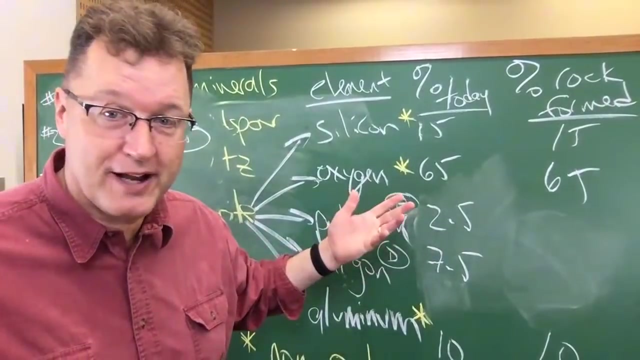 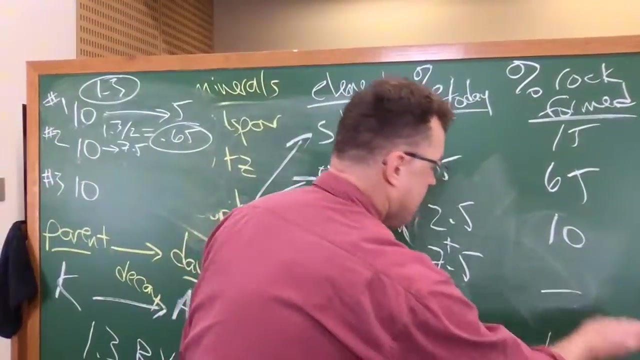 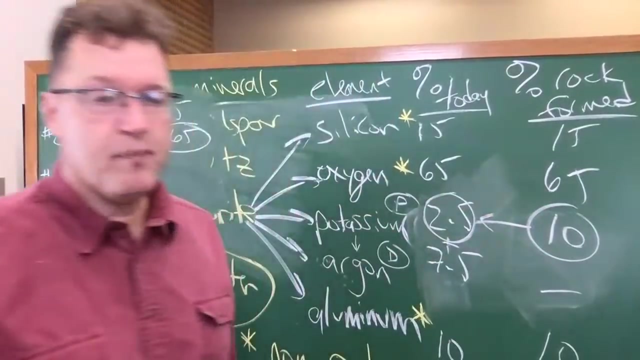 I'll wait. Here we go. What a clown. What's the first step? Add the parent and daughter together. How much daughter in the original rock Zero. This is example three. Second step: compare the parents. I hope you can see that granite three has to be far older than anybody else, right? 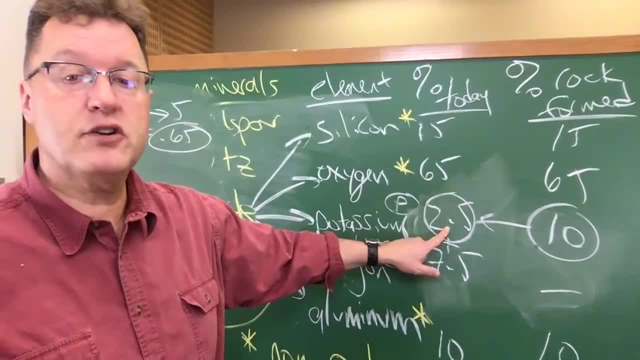 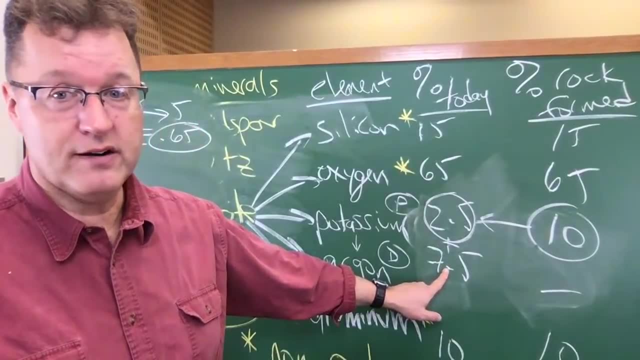 We started with 10%, 10% parent, and we go all the way down to 2.5.. That means a lot of decay has happened. Look it, we got a lot of daughter in the rock. If we have a lot of decay, 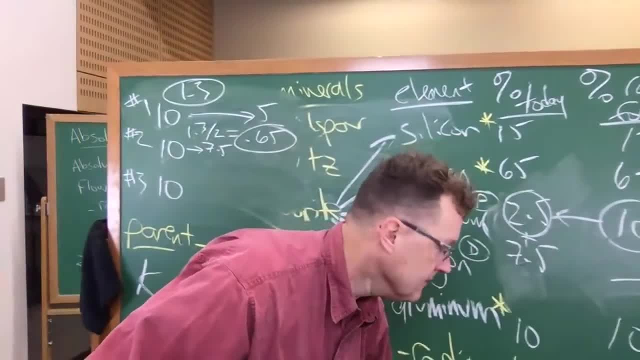 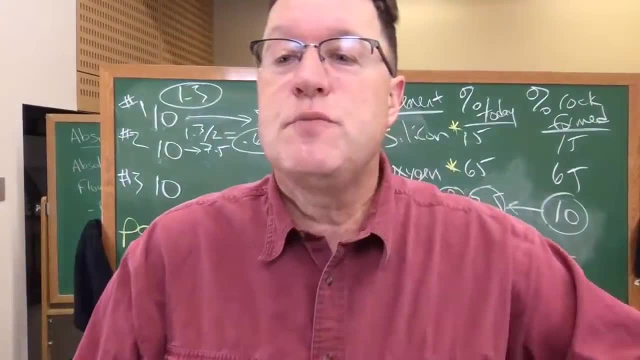 that means a lot of sand has gone through the hourglass. What, And do you have an age? I will wait, since I'm already late. I see 2.6,, 2.6, 2.6.. I see 1.95, 1.95.. 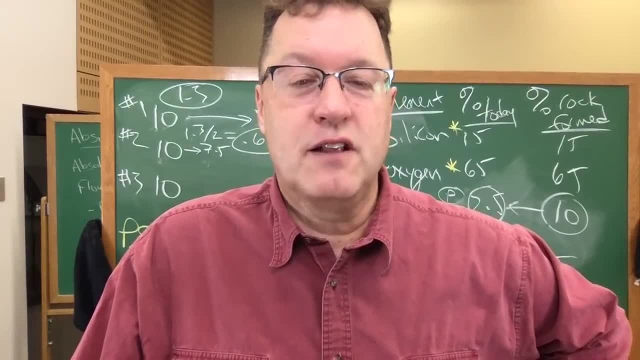 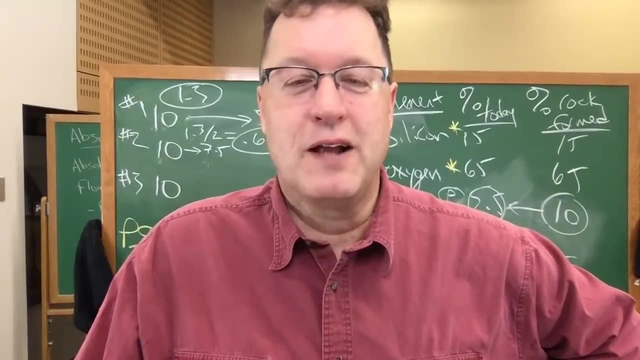 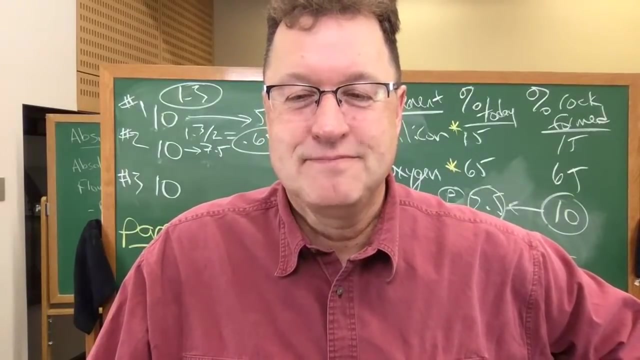 This is beautiful. And it's beautiful because I've given this lecture every quarter since 1987 and I always have those two answers Somehow comforting. But only one of the answers is right And the correct answer is 2.6.. Don't feel bad: 1.95 people. 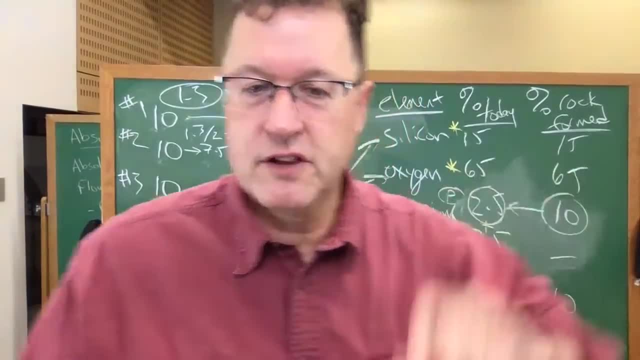 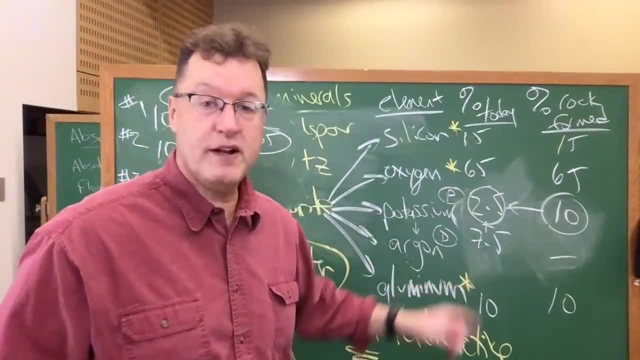 Let me give you the answer first of all again. Let me give you the answer first of all again. 2.6 billion is the answer for granite number three with these numbers. 2.6 billion is the answer for granite number three with these numbers. 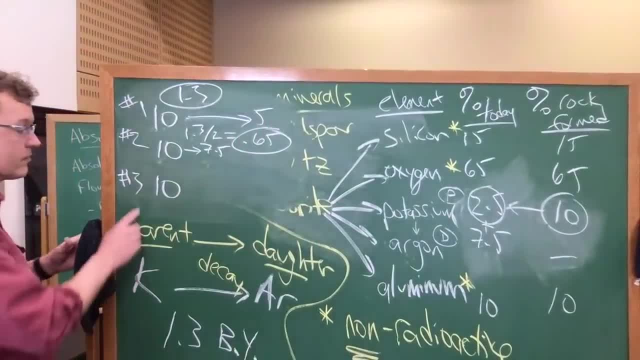 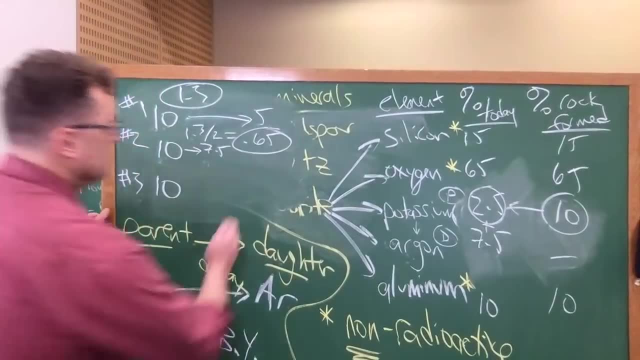 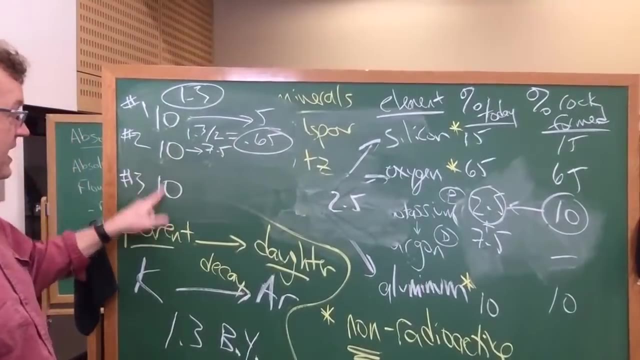 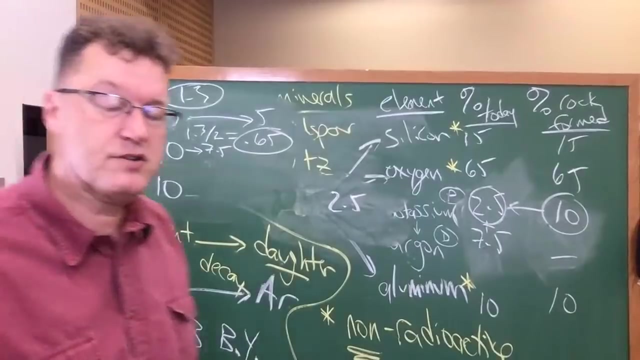 Let me try to explain why We started with 10 and what are we going to with this last example: 2.5.. We're going from 10, where we started before, all the way down to 2.5.. all the way down to 2.5. we're going all the way to 2.5. but here's the thing we need to realize. 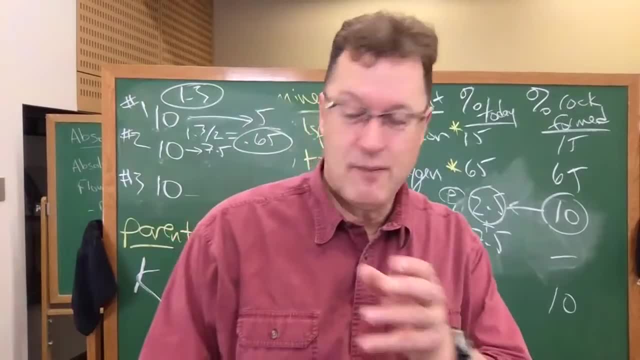 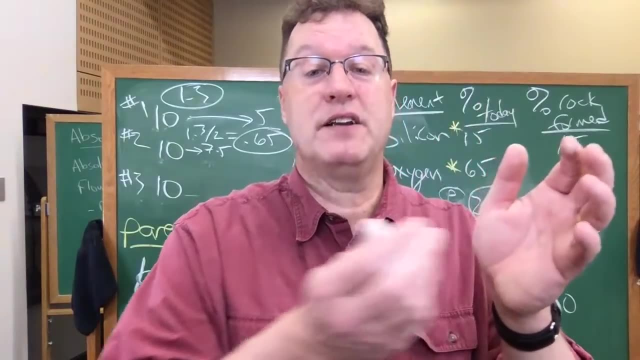 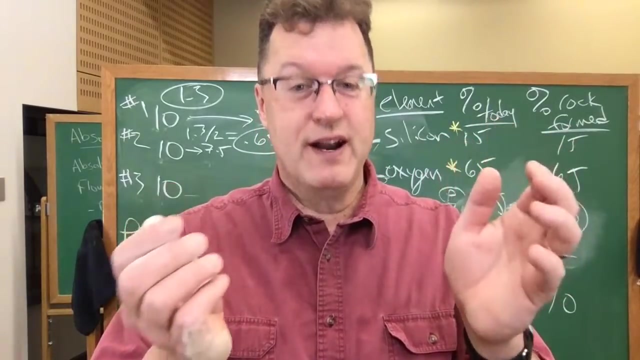 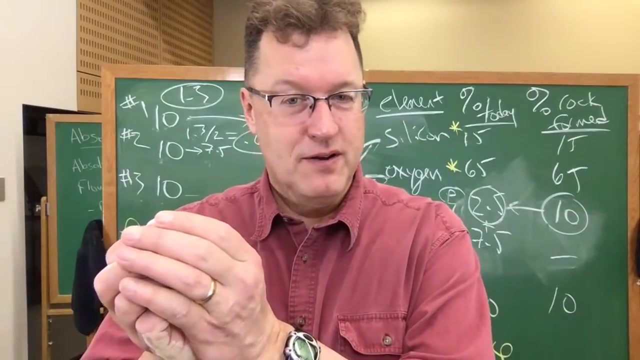 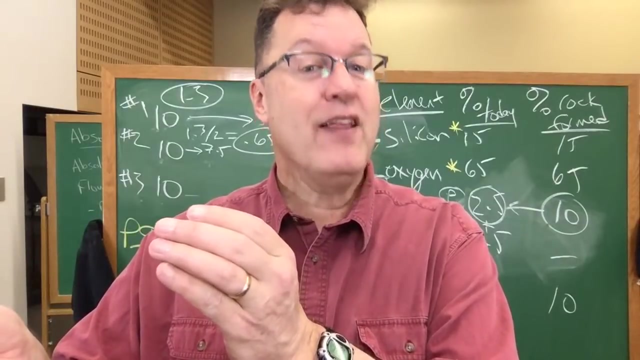 half-life on page five of the yellow book is the time it takes for half of the parent to decay. take a given amount of parent, cut it in half. that's one half-life. but what do you do with the remaining amount of the parent? you cut the remaining amount of parent in half and that's going to take another full half-life. 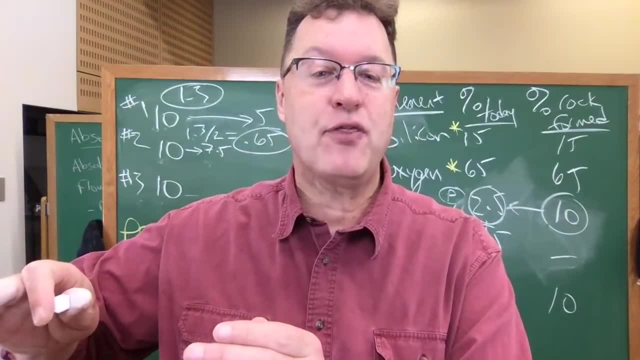 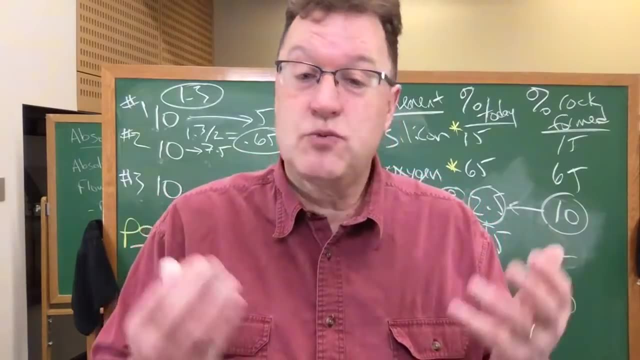 this is a logarithmic decay curve. if that means nothing to you, don't feel bad. it barely means something to me. but what the concept is is we never get to zero. we keep cutting the remaining amount of parent in half and that's going to take another full half-life. this is a logarithmic decay. 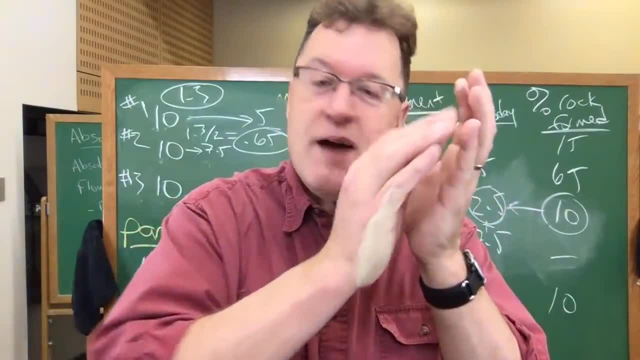 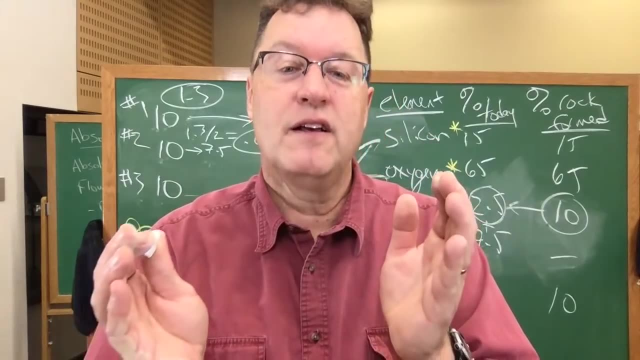 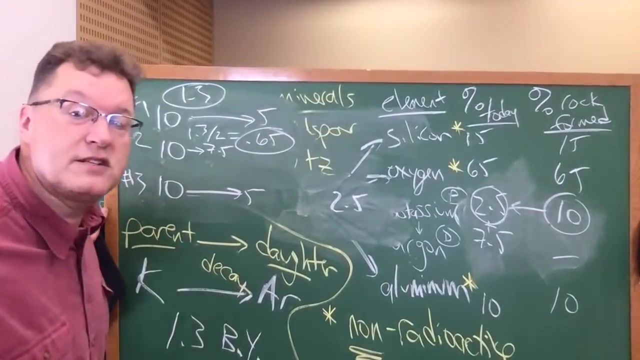 of parent in half and each time we cut the remaining amount of parent in half after a half-life process, it takes a full half-life. so 10 down to 5. how long does that take? how long does it take to go from 10 down to 5? half of 5, half of 10 is 5. 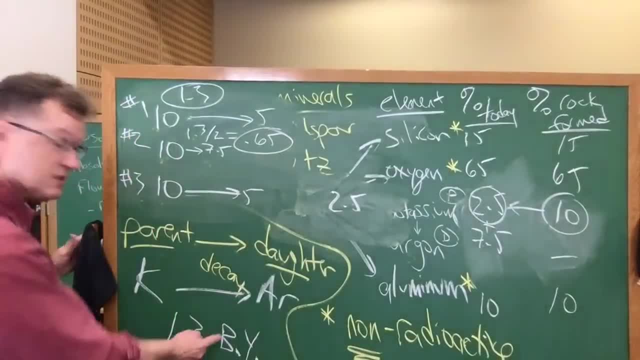 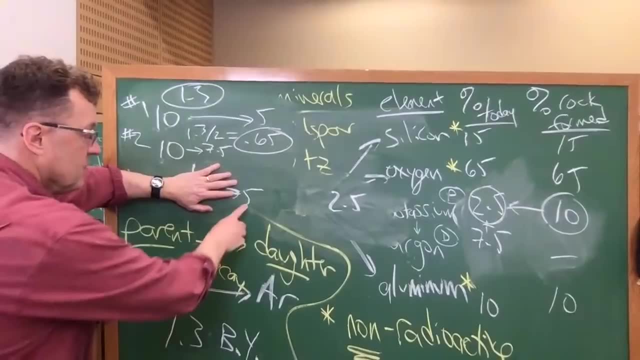 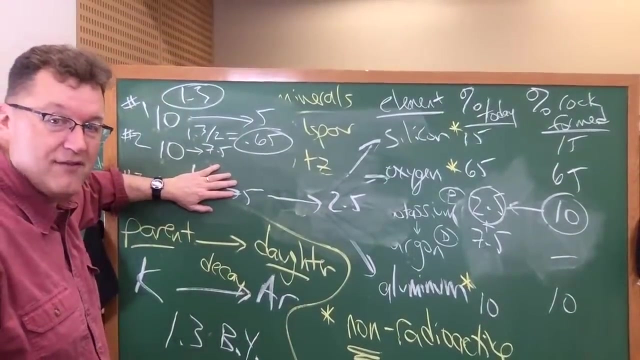 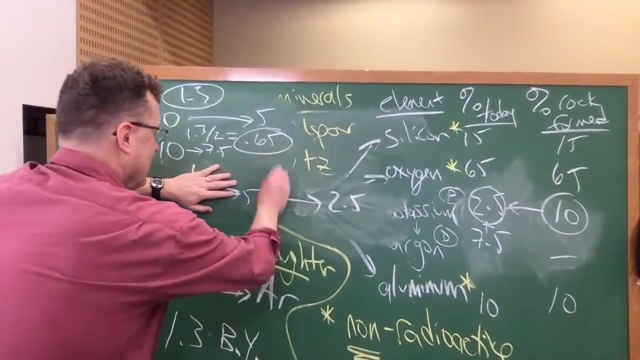 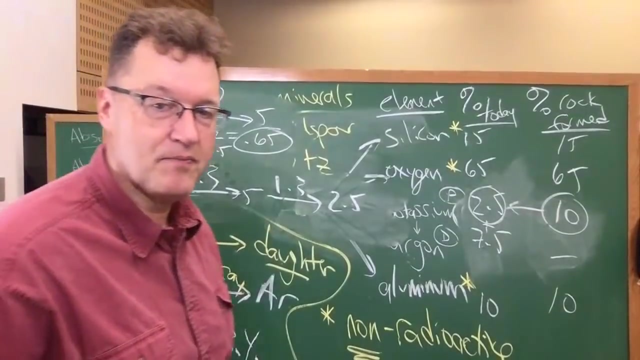 cut the parent in half, that's a full half-life. what's the half-life? 1.3? forget about it. now we've got five percent parent. what's half a five, 2.5. how long does that take? 1.3, 1.3 plus 1.3 is 2.6 and that's the answer. 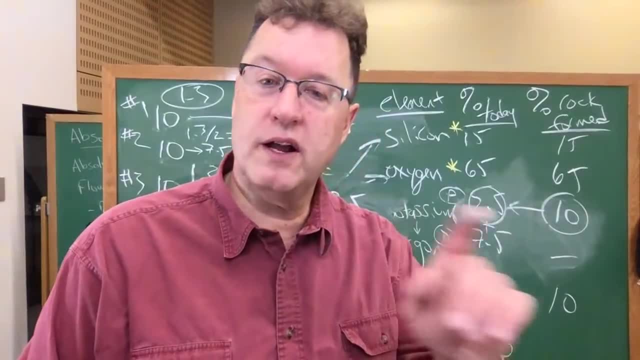 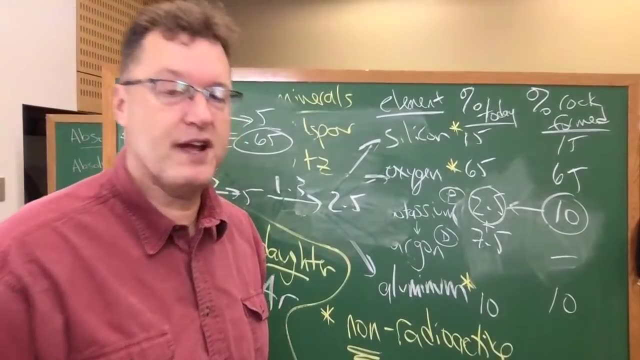 1.95 people. you were incorrect, but i said you were wrong. i see what you were doing. you were taking our work in the previous two examples and kind of combining them makes perfect sense, except for this fact that this half-life is on a logarithmic decay. 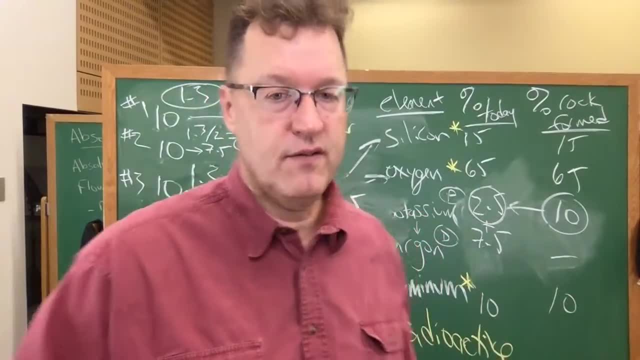 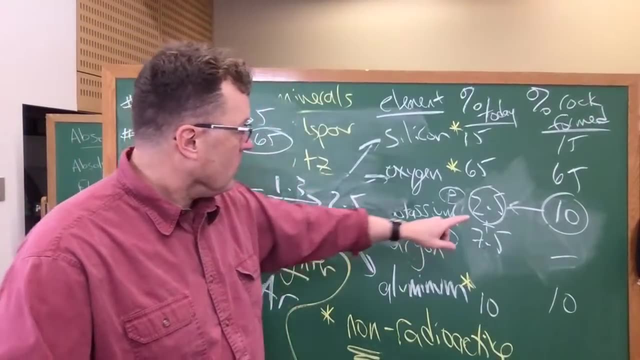 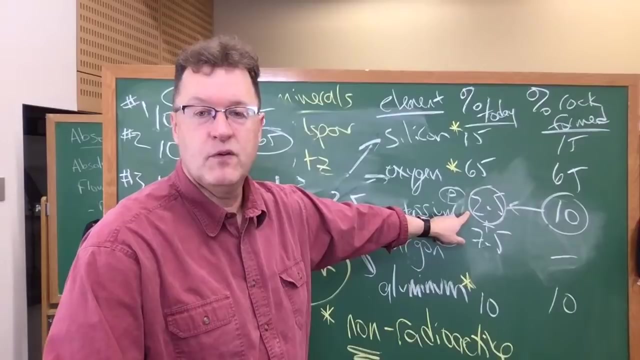 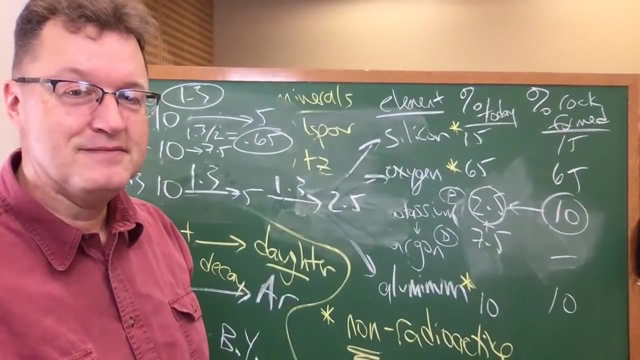 scale, a logarithmic decay curve. so just verbally, what if our um, what if our parent back from denver was 1.25? what would be the age of granite? number four, if our parent was 1.25, 3.9, north new mexico hockey fan. that is correct. 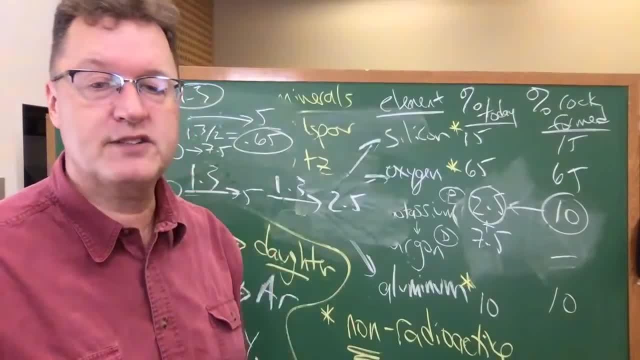 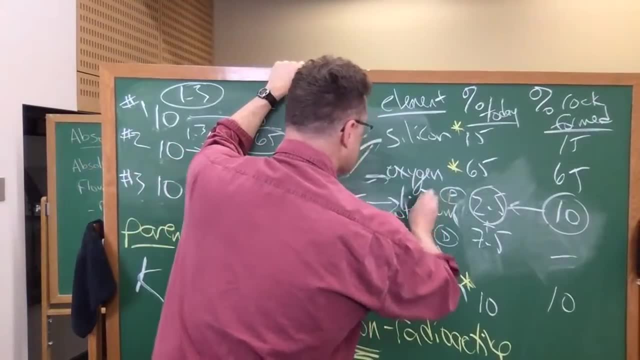 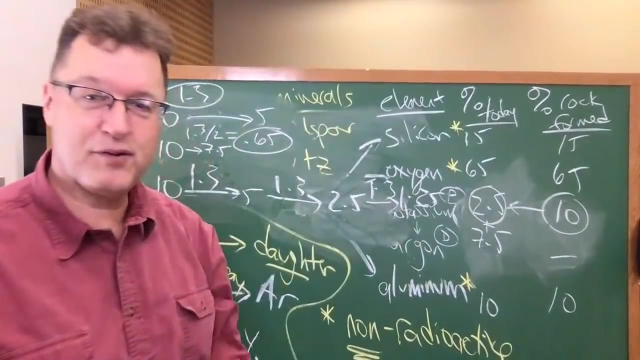 the answer for my verbal example number four is to go from 2.5 to 1.25. 1.25 is half a 2.5. that's going to take another 1.3. you see why we never get to zero: 1.3 is half a 2.5. 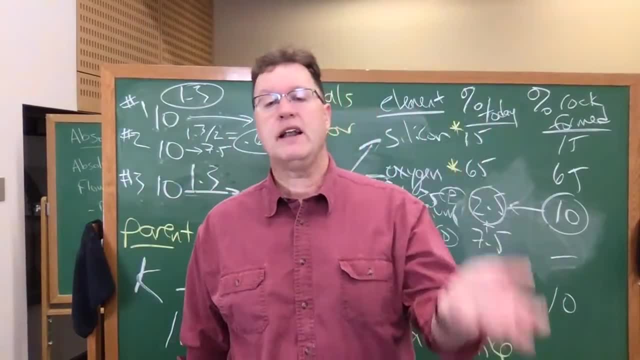 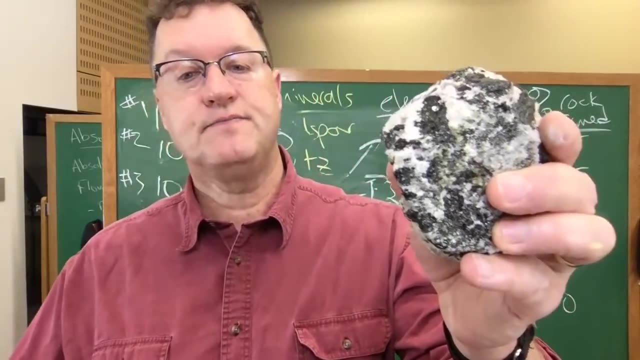 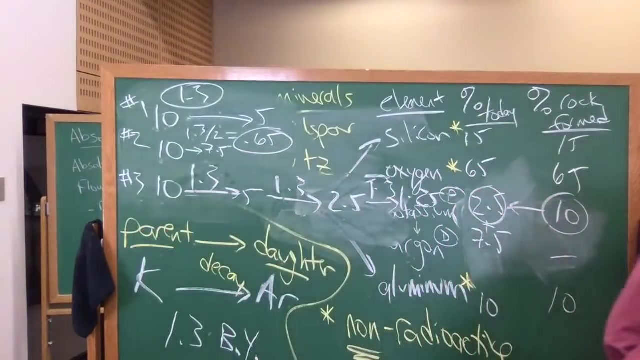 we keep cutting the remaining amount of parent in half. that is the process behind determining absolute ages of this diorite, which is an igneous rock, this granite, which is an igneous rock, this schist, which is a metamorphic rock, and this fossiliferous limestone, which is a 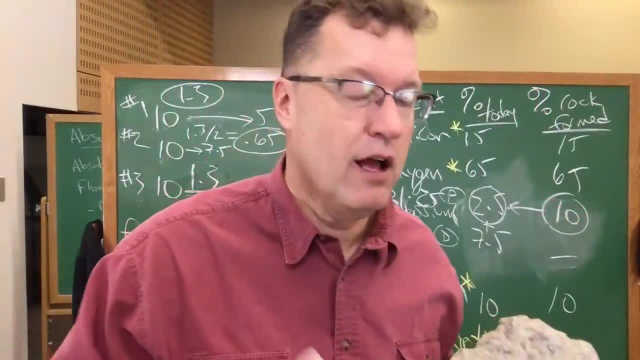 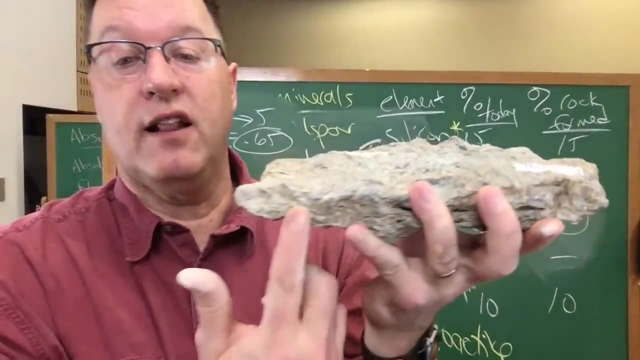 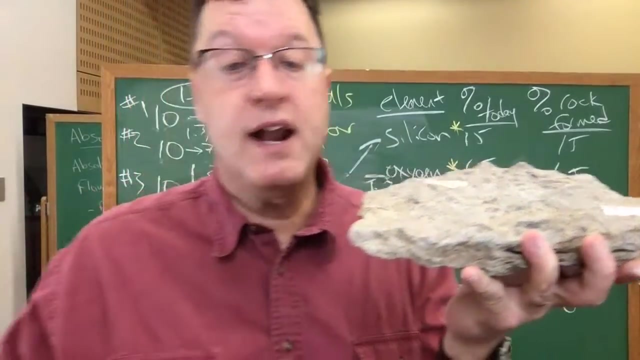 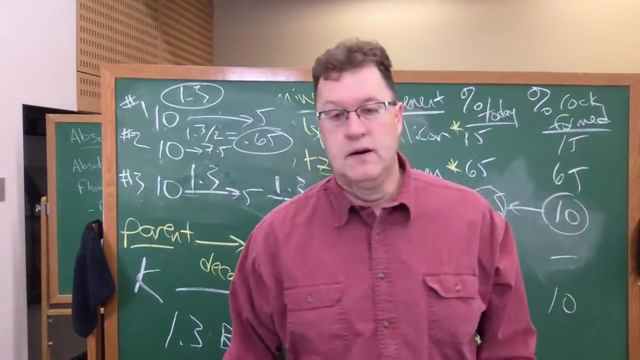 sediment, wait, no. sedimentary rocks, sedimentary rocks. this process does not work. so beautiful marine fossils in a limestone collected at cincinnati, ohio, on the off ramp of i-71- whatever it's called. we cannot use this process for that. now i have violated my solemn vow that i would keep these lectures to 50.5. 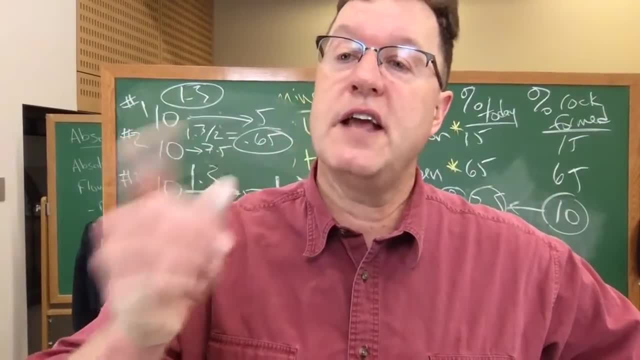 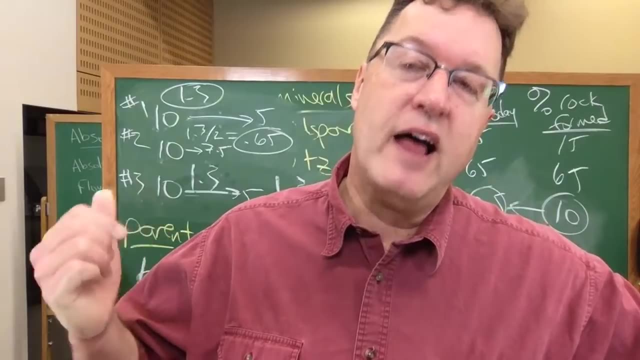 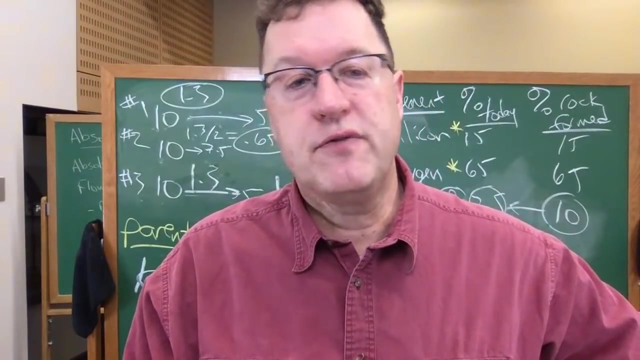 minutes and I apologize one more time because I've gone 10 minutes over. That will not be a habit, I promise, but this one is valuable enough information and it took a while for me to get rolling, so I hope that you feel like it was worth the extra 10 minutes. Central students, thank you. 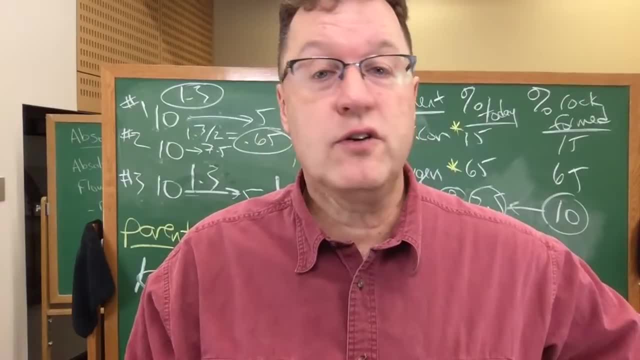 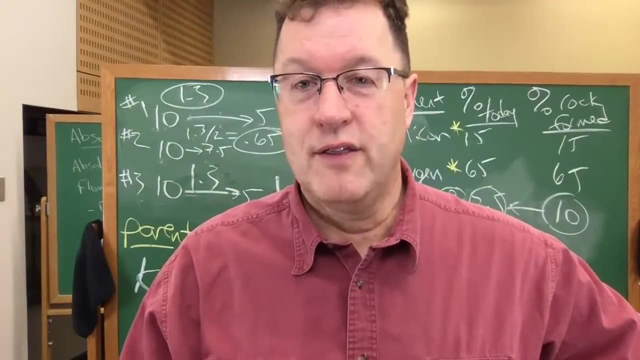 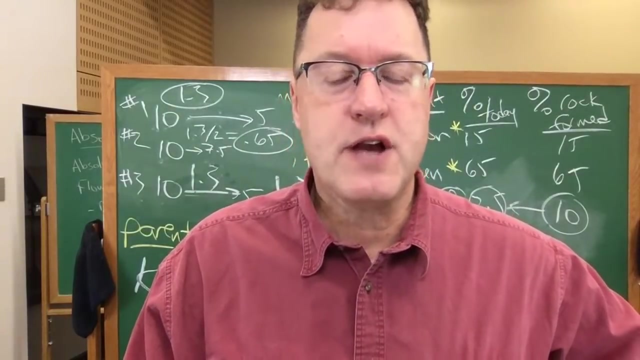 for joining us today. Have a good weekend, I love you. Goodbye, and we'll see you Monday morning at 10 am, right back here in our virtual world. The following week is when I will see you face to face and I will be hugging you. No, I won't. I'll be shaking your hand. No, I won't, but I'll be. 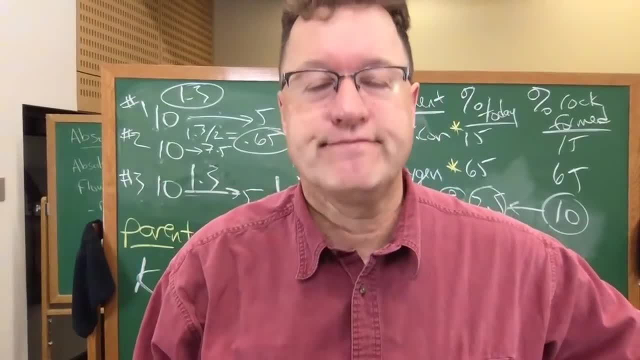 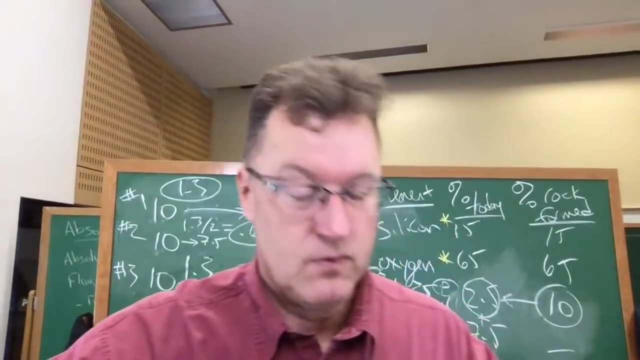 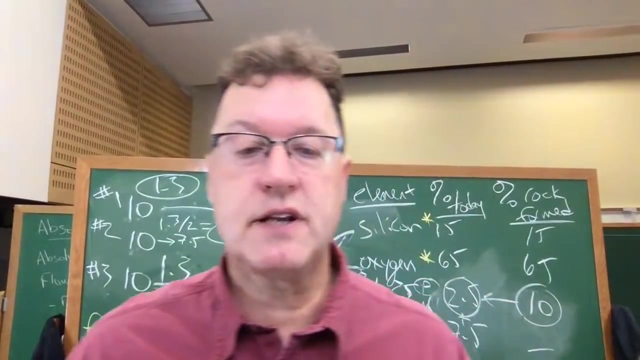 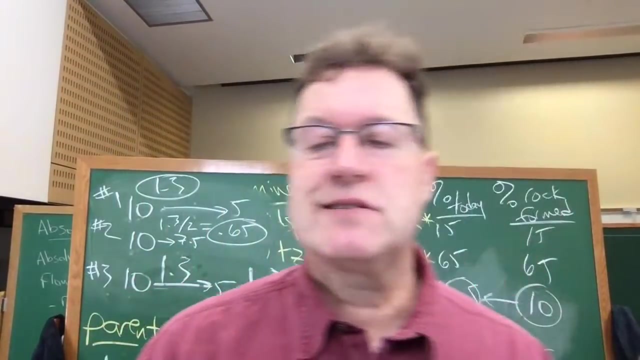 doing that, Thanks, Goodbye. Okay, townies, You want to talk for a few minutes here? Okay, Uppercase in the live chat, and if you want to ask a question or two, this is one that needs a sprucing up. It's a lecture I've given a long time and I need to. 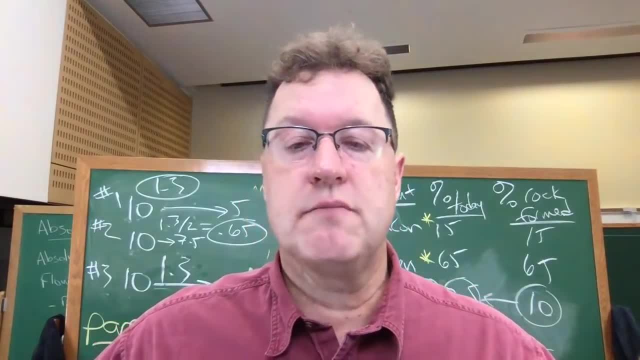 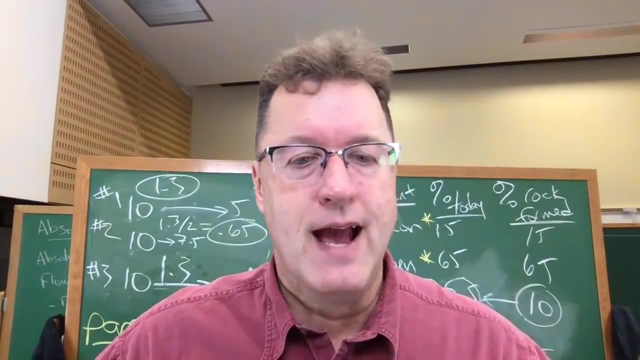 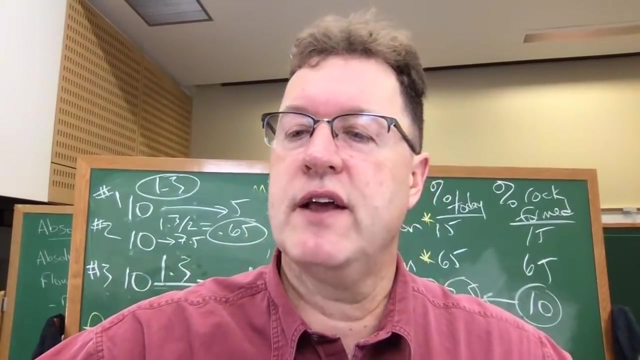 work with geochronology professors like Chris Mattinson and get a little bit more accurate or something. I always feel like I need to improve this lecture, but the concept, I think, is there. I saw, Joseph, Can you get to? 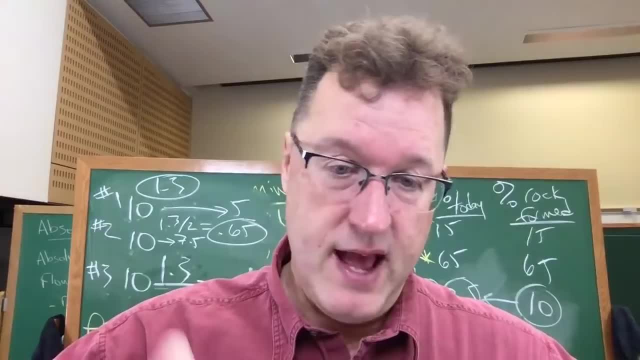 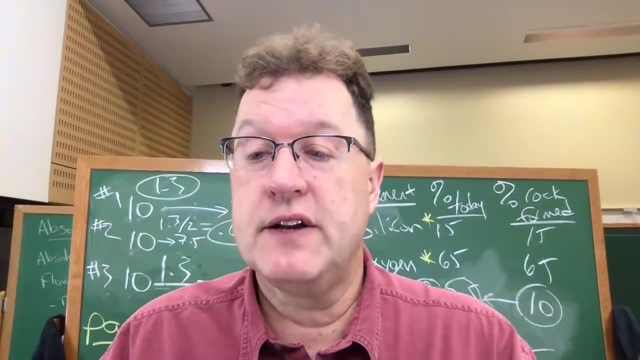 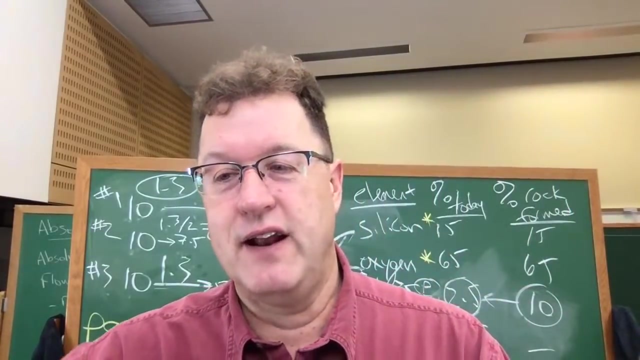 zero percent parent in an igneous rock? No, Because of that. the way that half-life decay curves work, Joseph, as I understand it, you never get to zero. Remember, the age of the earth is 4.6 billion years and if we've got rocks that are approaching that, then we're not even going to 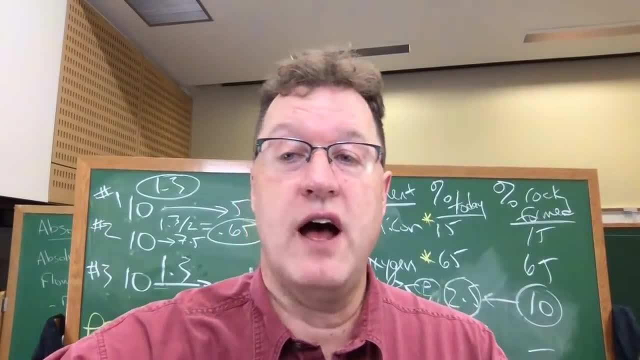 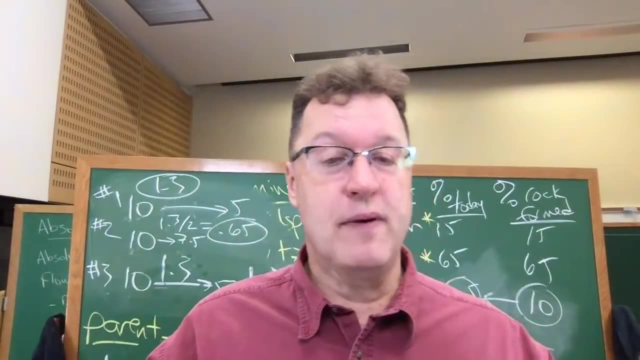 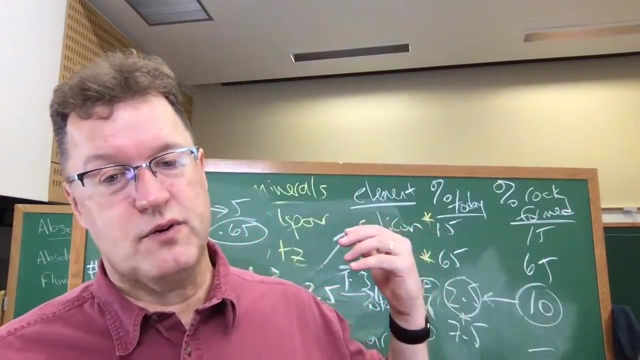 see that, but there are some. That's why carbon dating, by the way, is the same process of half-life, but the half-lives for carbon are in the thousands of years, not billions of years, and so the carbon dating is not done with these rocks. 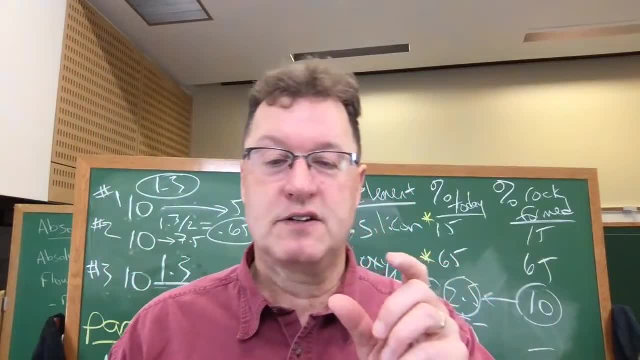 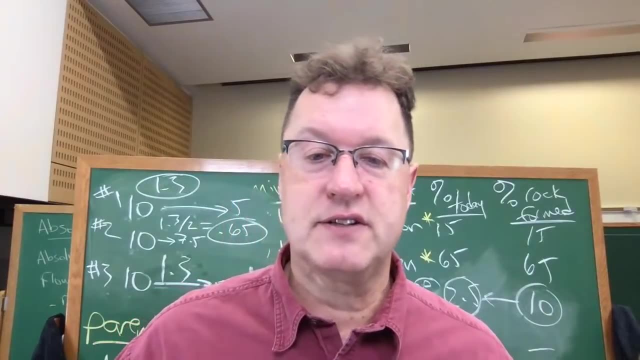 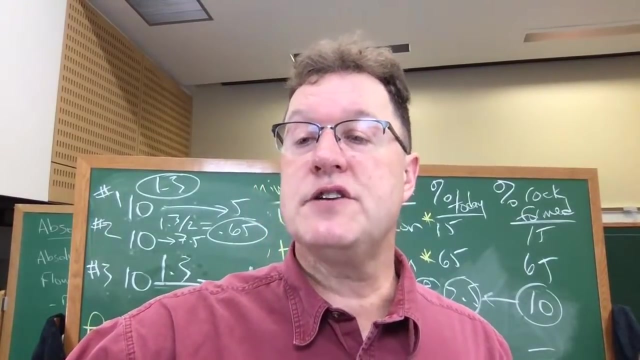 because the half-life is way too short. Instead, the carbon dating is used on organic matter primarily. that is used with archaeological sites and very recent, let's say, neotectonics Technology suggestions about the lighting. Thank you, I'll read those later. Do igneous Steve Do? 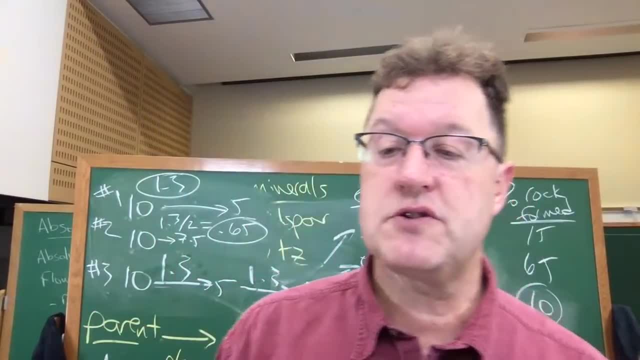 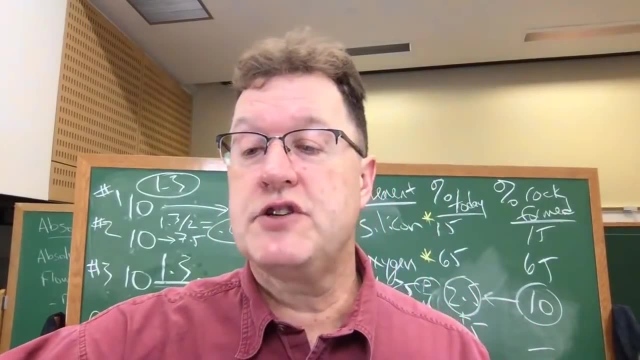 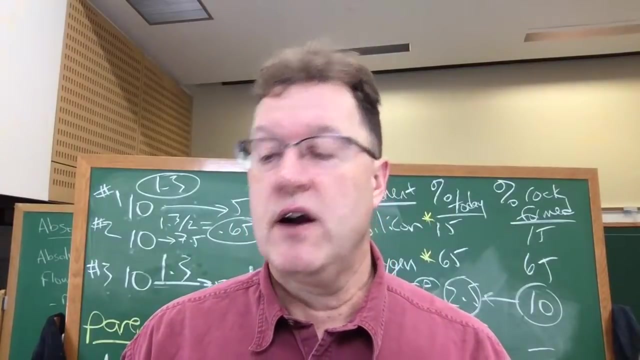 igneous rocks on other planets have the same properties? I assume so, Steve, but I'm very weak on. I know essentially nothing about planetary geology. Does the geology department have No? How does biotite mica differ from biotite gneiss, Eric? biotite mica. 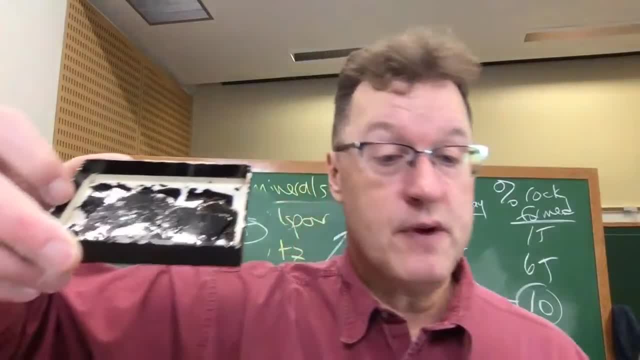 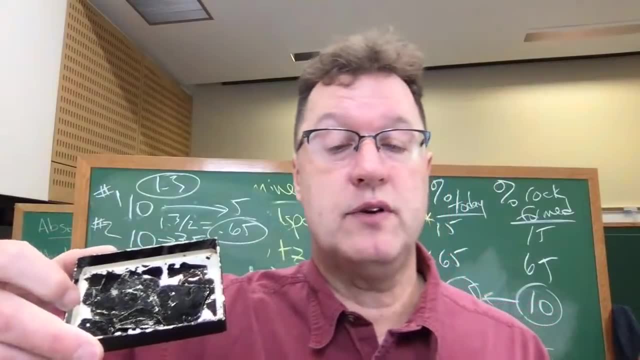 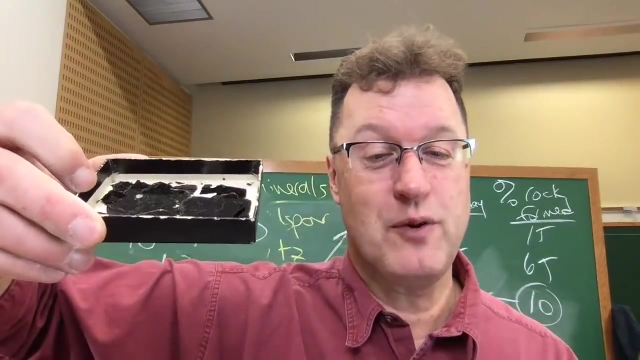 Is a mineral and the swakane biotite gneiss, for instance, which I was talking about with the exotic terrain series, is a metamorphic gneiss. that's a rock that has a lot of biotite, mica- within it, So it's called a biotite gneiss just because it's a metamorphic rock. that. 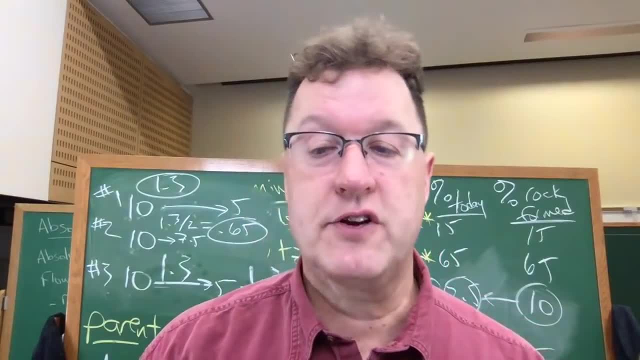 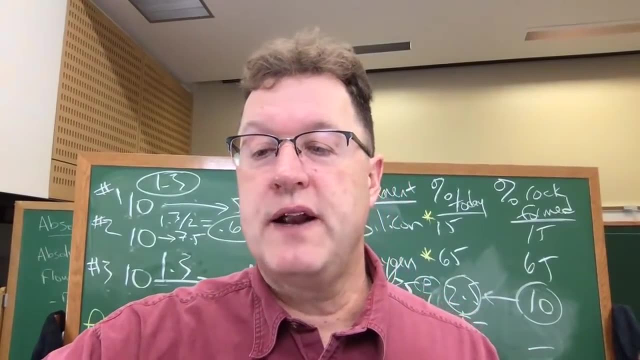 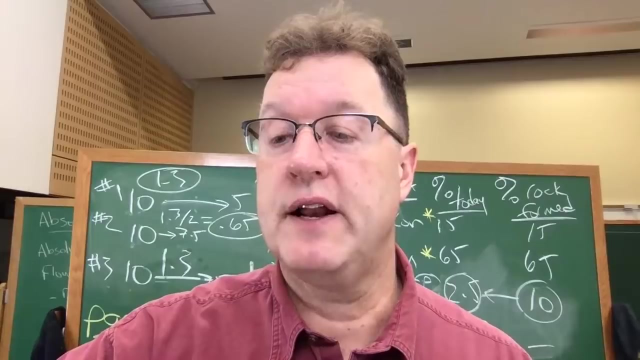 has a large amount of our star of the show here today, the biotite gneiss. Okay, Is logarithmic reverse exponential. I can't remember. I'm sorry. I'm embarrassed to say that I don't know. Somebody here probably can help us there. 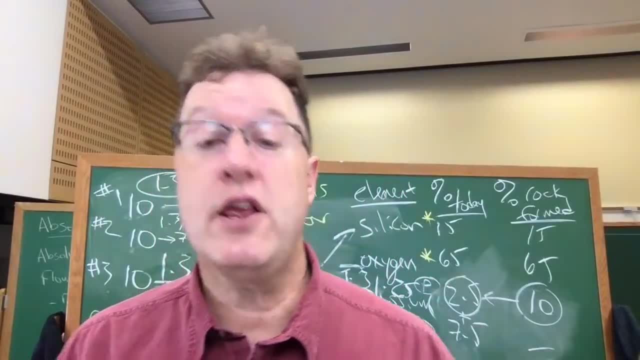 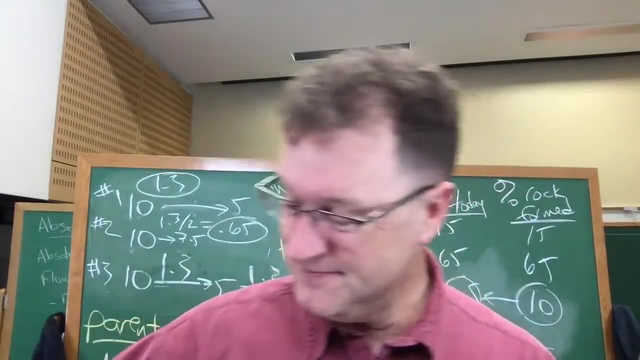 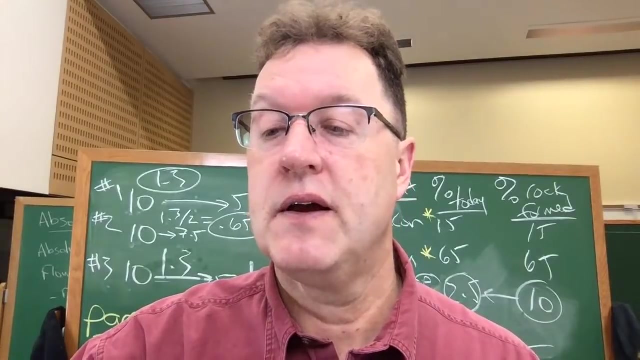 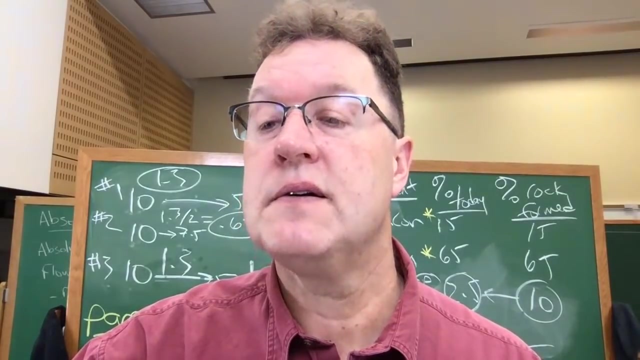 Why not use potassium? Why not use the potassium feldspar? Why not use the pink stuff here? Wrong isotope of potassium. It's just a certain isotope of potassium that we can do this. Oh, I see many of you are asking that. 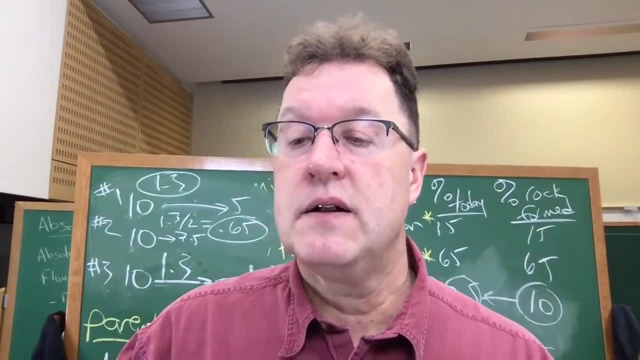 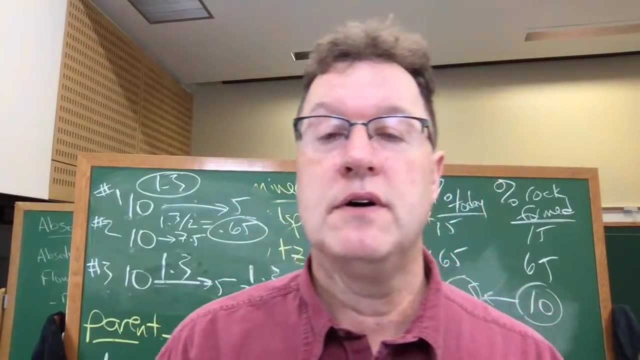 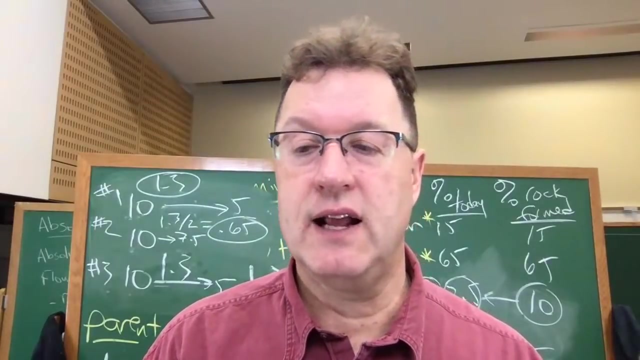 Todd Geologically Speaking, who is on fire? Have you been to Geologically Speaking's YouTube channel or Instagram? Are you an Instagram user? Todd's been on fire lately. Todd, I'm glad you could break out time from your time. 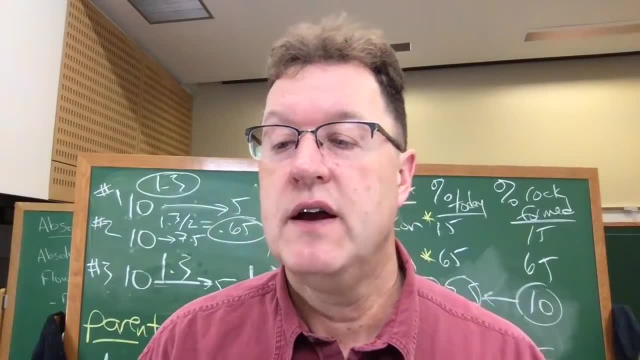 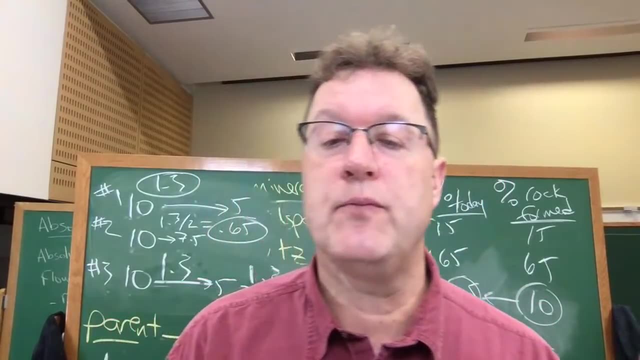 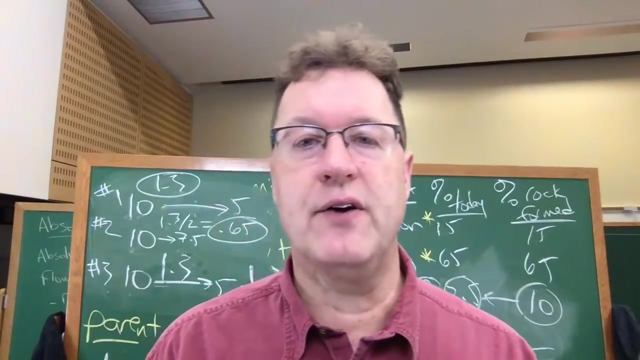 Thank you. Thank you for taking your busy work schedule to join us. This is how the age of the Earth, even the Moon, was determined, correct? Yes, I'm fuzzy on that too, but we've never found a rock on planet Earth. that is 4.6 billion. but we have found rocks that. 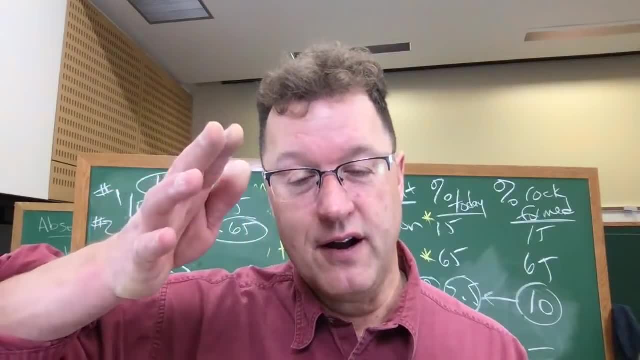 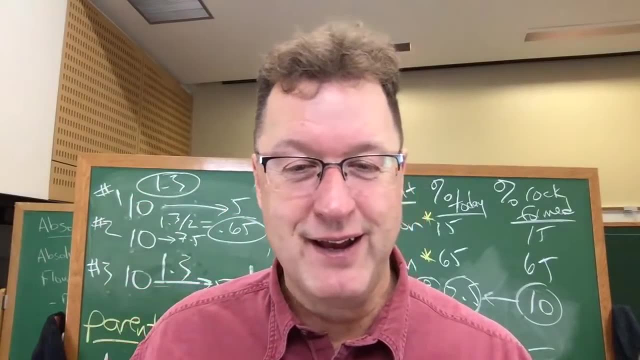 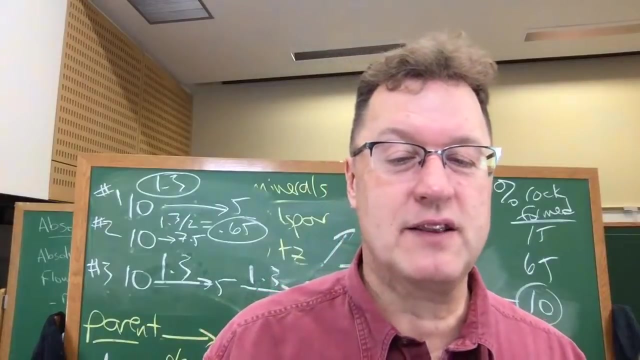 are over 4 billion and there are minerals in that little bit more than 4 billion-year-old rock that has radioactive decay recorded with gneiss. So we can back calculate to the origin of the Earth, but there is no rock that's been. 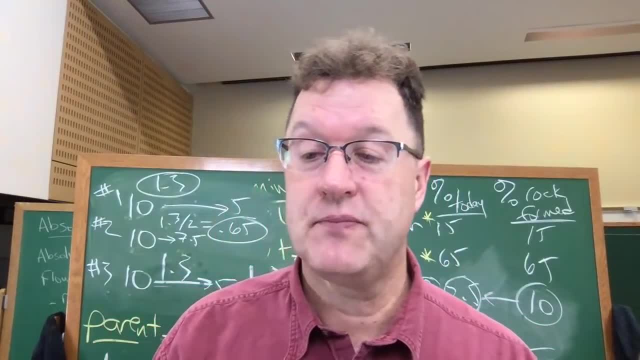 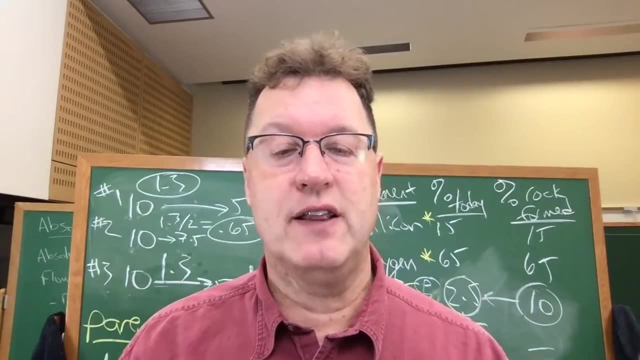 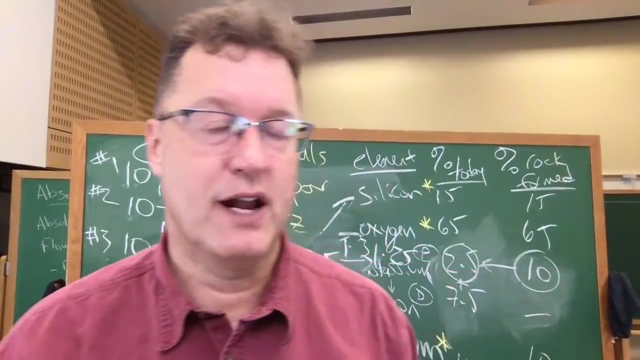 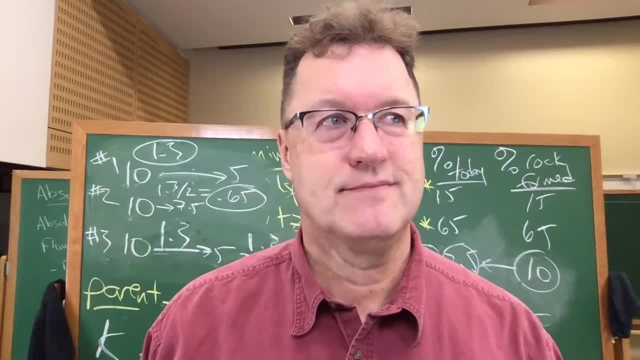 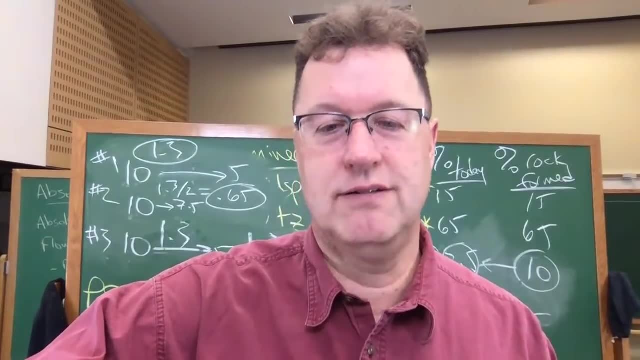 But one of these days I'm going to. I think some of you know how I like to work. I kind of work off of guilt, So I told myself one of these days I'm going to do the exotic terrain thing. 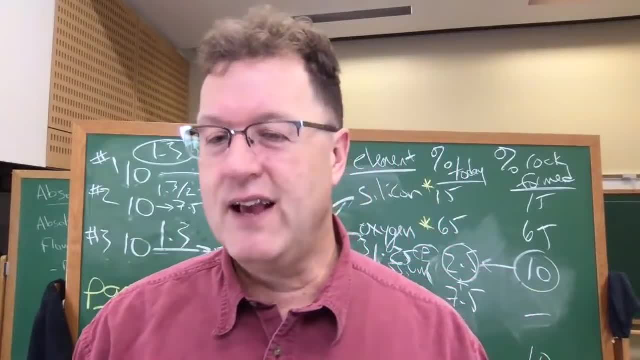 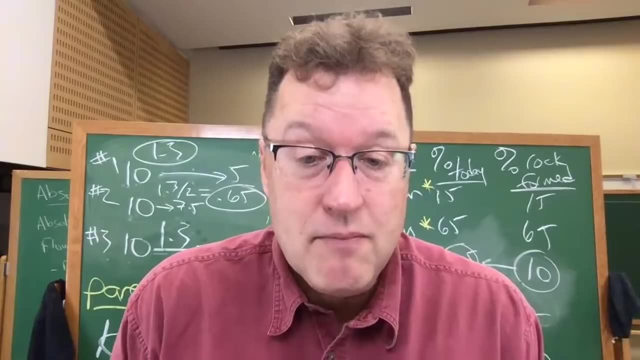 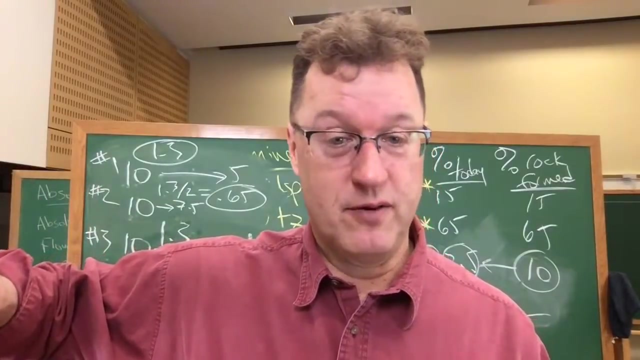 And I did. I feel great about it. One of these days, maybe soon, I'll figure out how to really get into this, Because it's obviously a major topic and it is a topic that is a deal breaker for many who maybe have interest in geology. 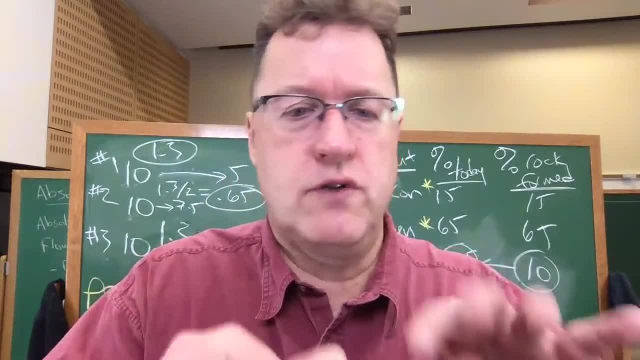 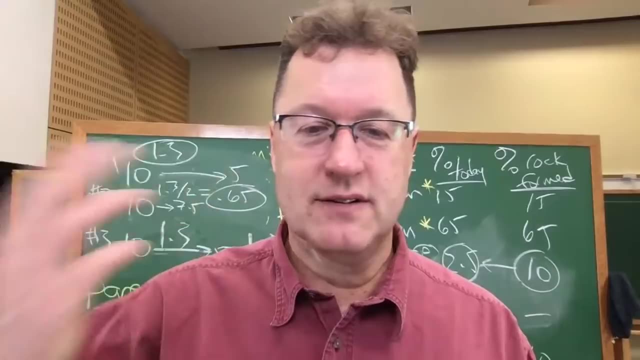 But as soon as he started talking about millions of years, that's where he lost me and I'm out. You know, it's like I realize I'm not going to be able to convert many, but maybe a few that are willing to honestly see what we're doing. 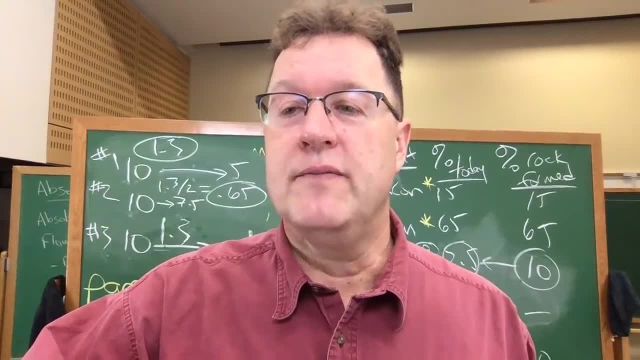 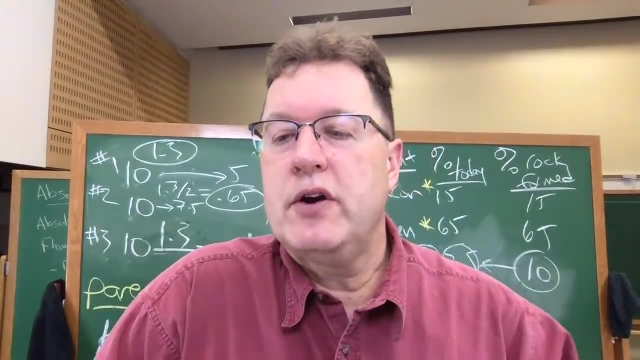 And a couple more and I think we're done. Yeah, I feel bad about going long there, but it's kind of had a little bit of a roll going. What would be a good resource to refer to as I practice this at home? 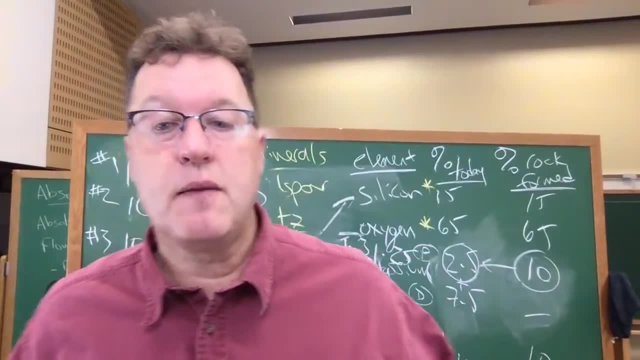 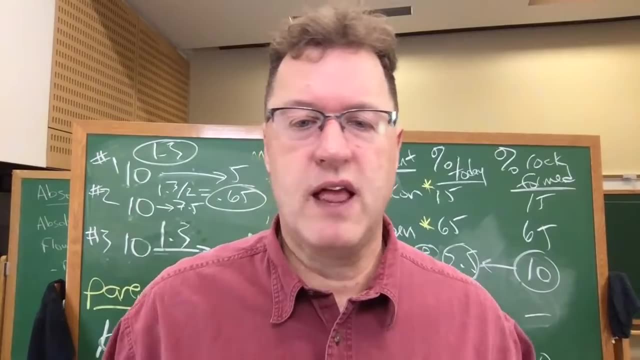 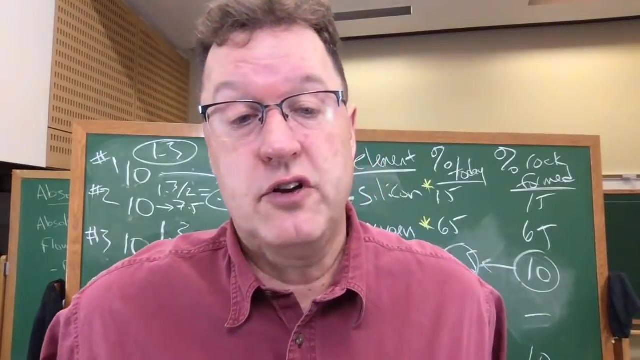 There's some good. I don't have one specific. Maybe somebody here can help. There's some good YouTube videos on this, using like M&M And other kinds of statistical things And just some little short geology, So you can just go to YouTube and type in absolute age dating. 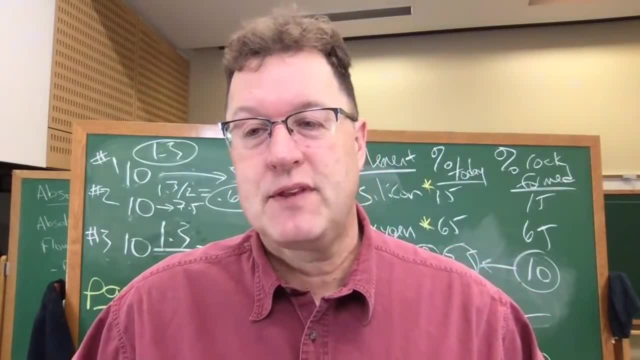 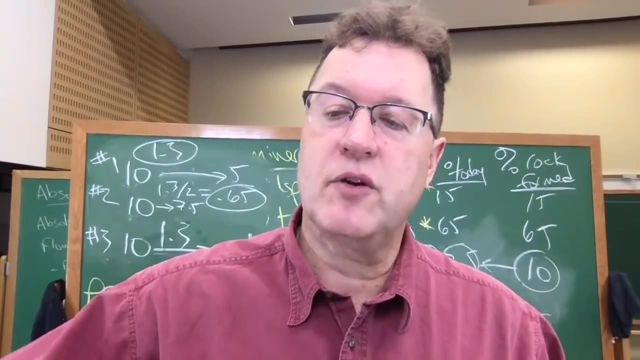 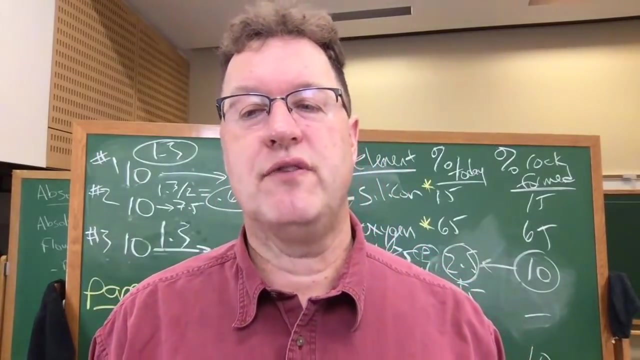 or radiometric dating or something like that That brings up. can somebody help here? Ivana Ivana, Ivana, I believe, is the name, And he's in Brooklyn, New York, And those that were with us in the fall with the live stream series. 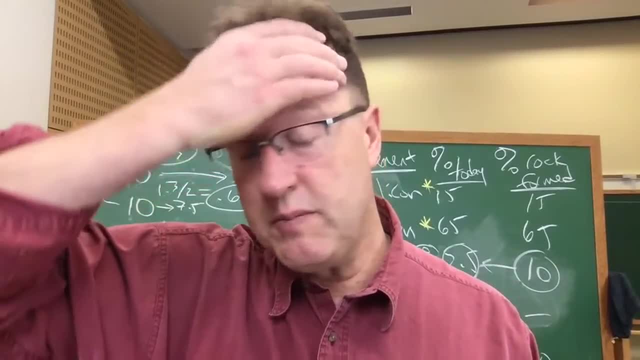 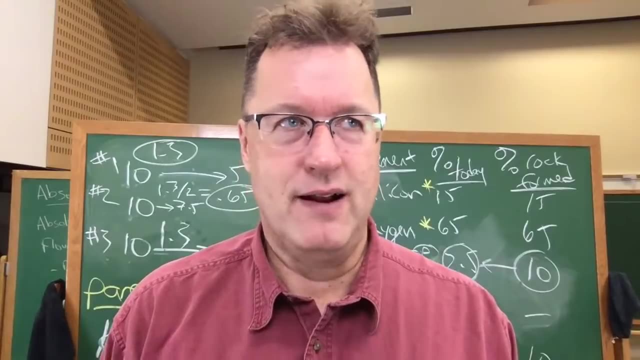 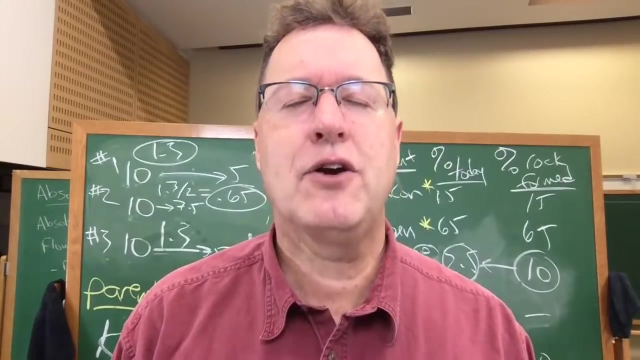 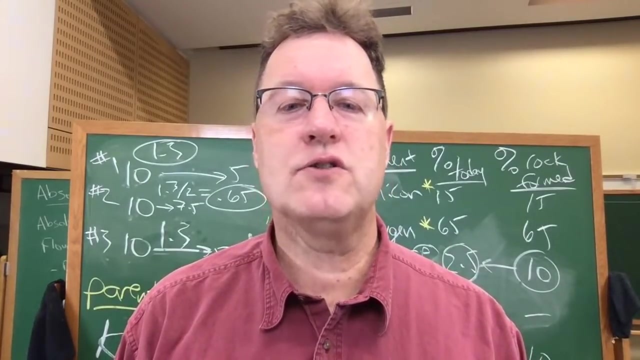 know that Ivana was a major contributor to what we were doing. I think a self-taught guy, But in his spare time- I don't know how many hours- he's compiled an incredible, an incredible database where you can see. you could lose months looking at all the videos. 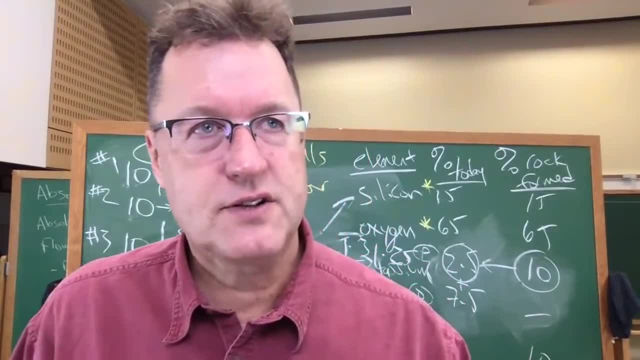 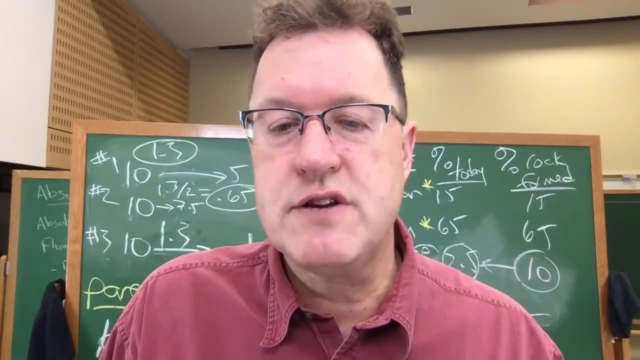 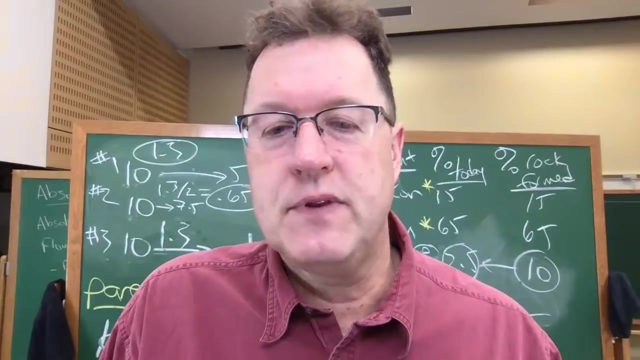 he has put into this Earth science online. somebody have it. What's the name of Ivana's geology video? I'll bet you, if you go to Ivana's video warehouse, essentially you could type in absolute ages or something. 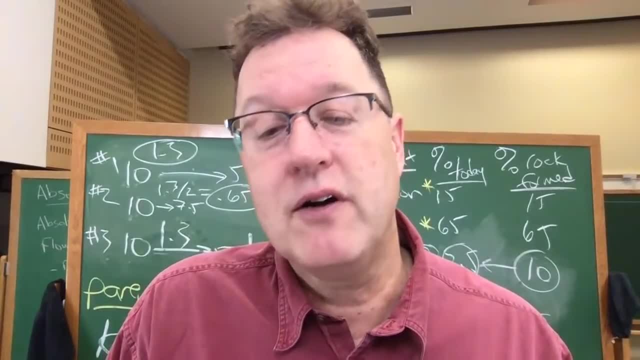 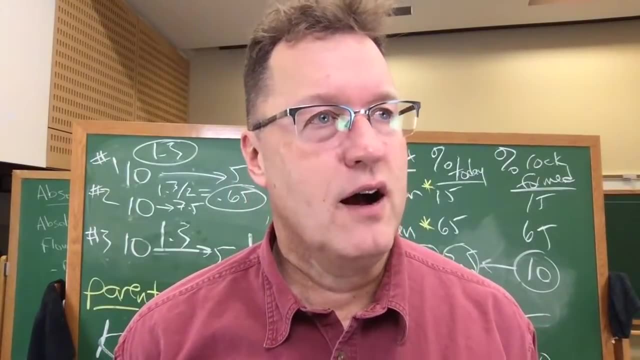 You could. you could probably. I'll probably do that. after we're done, I'll probably go and see a couple of videos that's out there. I haven't done that, Nobody's got it. Earth, Earth science online Video database or something like that. 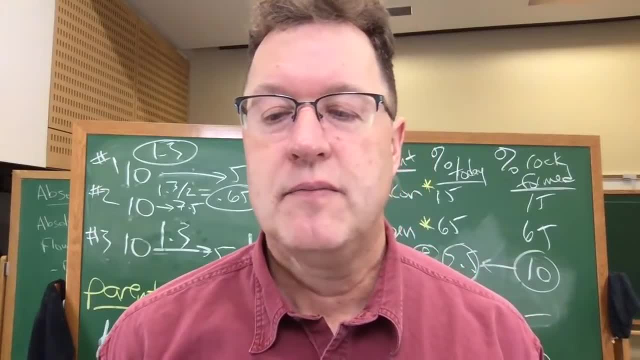 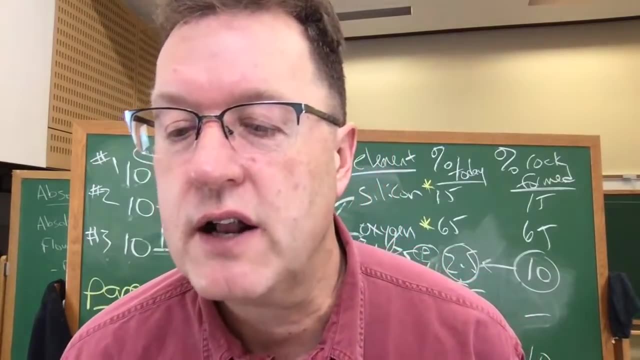 I'll wait a couple more minutes See if anybody somebody can find it, But it'd be nice to have that in the live chat comments for people. I think Ivana- I don't know if he's with us in these. Thank you, Charlie. 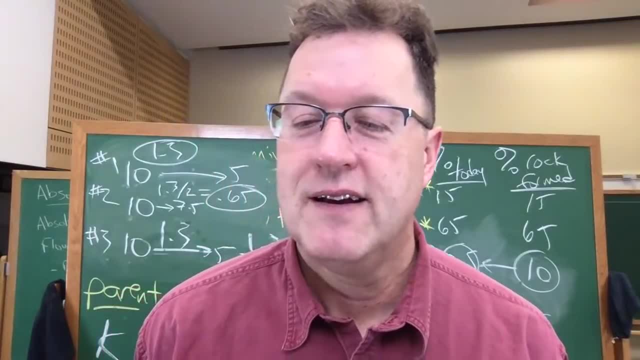 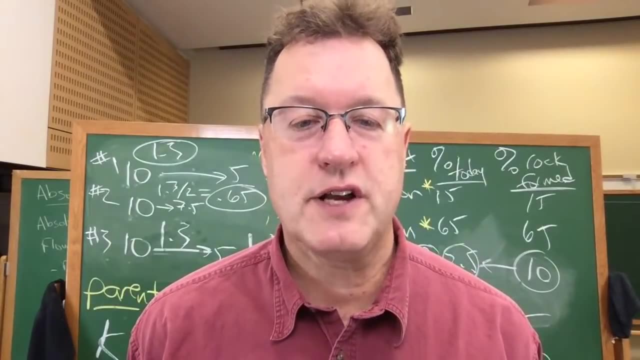 Earth science online video database. Yeah, Earth science online video database. Go there You will be, if you love geology. and I've only gone a few times and then I get like overwhelmed, Like there's just so much there. 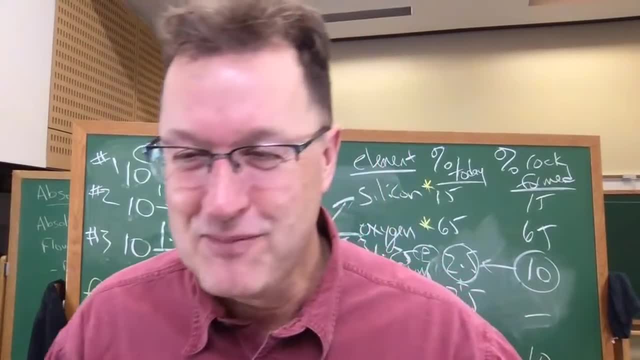 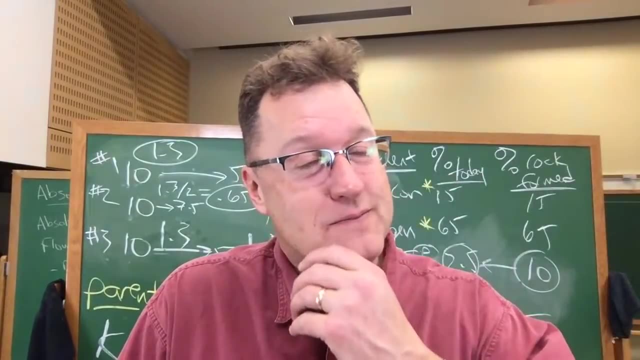 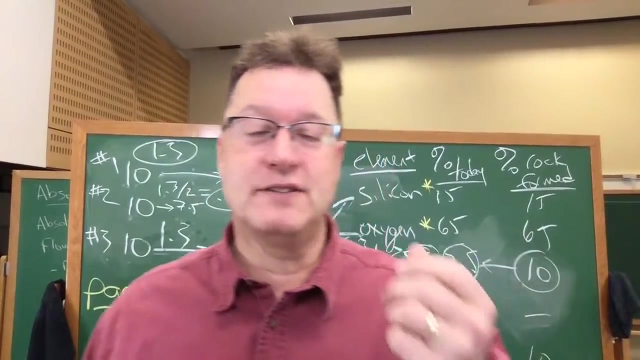 I don't even know where to start. I don't even know where to start. I just like leave. Probably not a good recommendation, But he's got. he's got everything typed in by subject and author and other things, And so you can. there's a lot video wise that I'm still old enough. 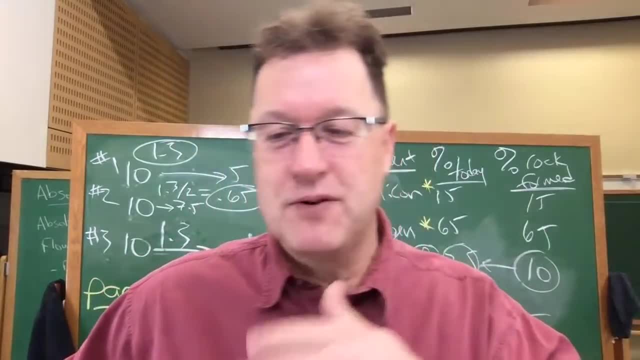 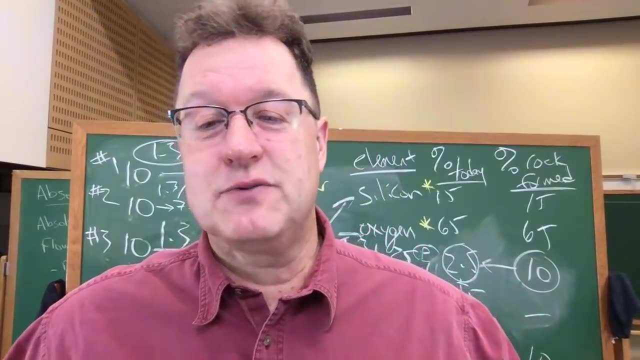 I don't think about going to YouTube to learn stuff. I go to scientific papers or other things, but there's enough now. You know there's junk, but there's also really good stuff And I don't know how much Ivana has really gone through. 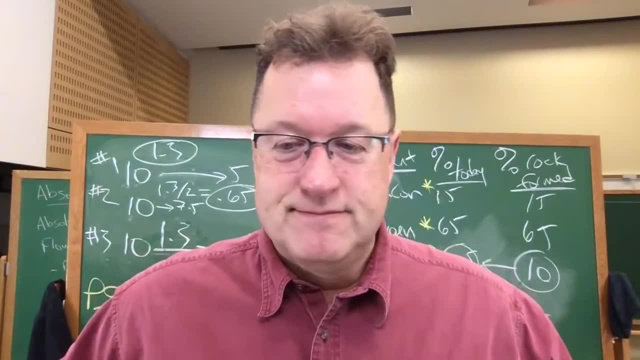 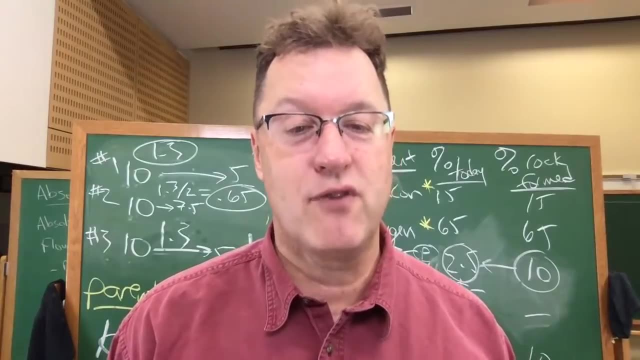 And kind of I don't know whatever. It's all there And you know the BBC has done a lot with this sort of thing over the years- the Men of Rock series, But there's others that are. there's actually you know what. 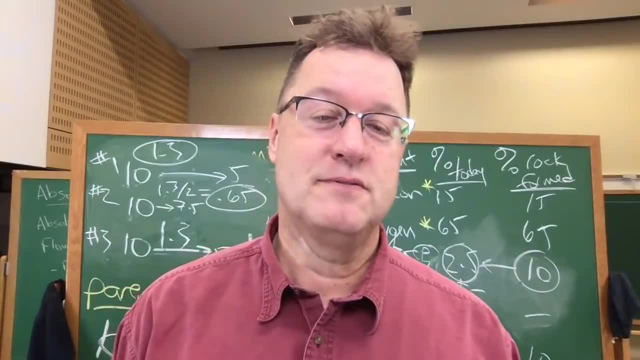 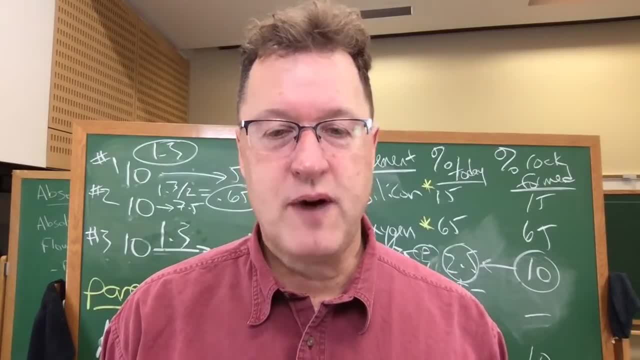 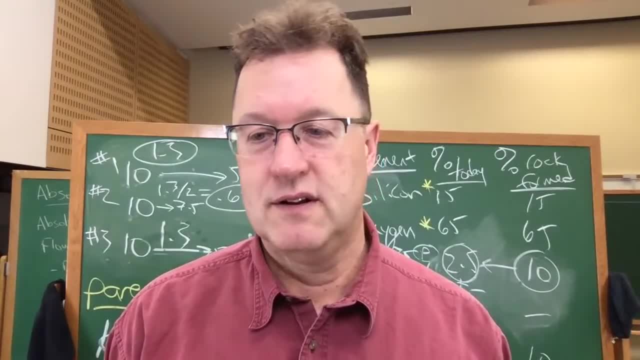 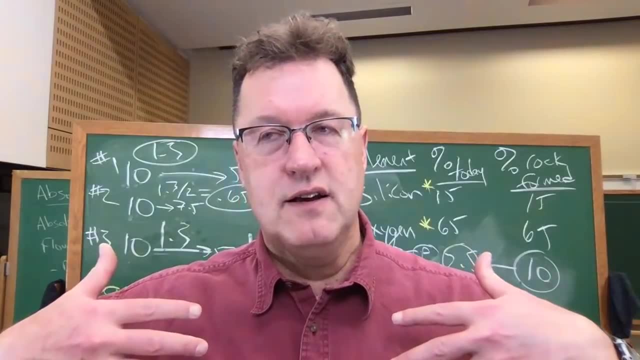 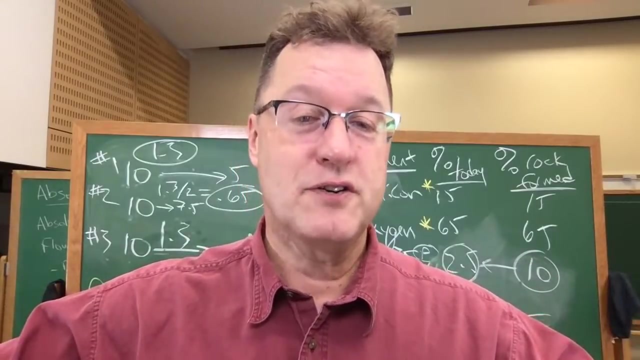 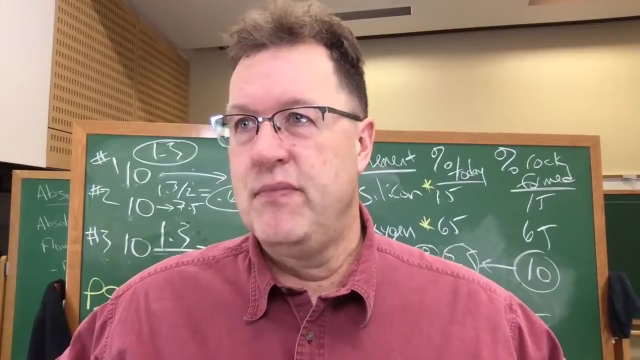 But one really positive thing of this whole: nine months of virtual, isn't it likely there's going to be a just a explosion, a proliferation of great online resources? Like even when we go back to normal lives, won't there be way more stuff from? I don't know? 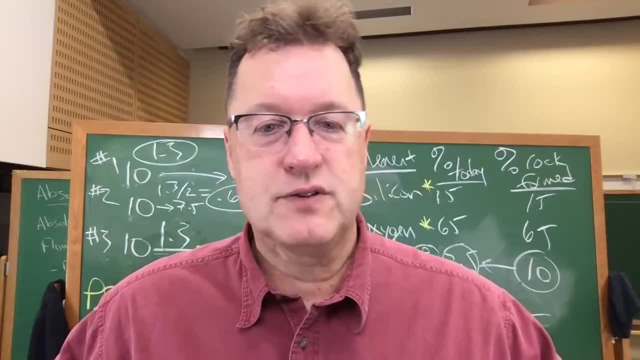 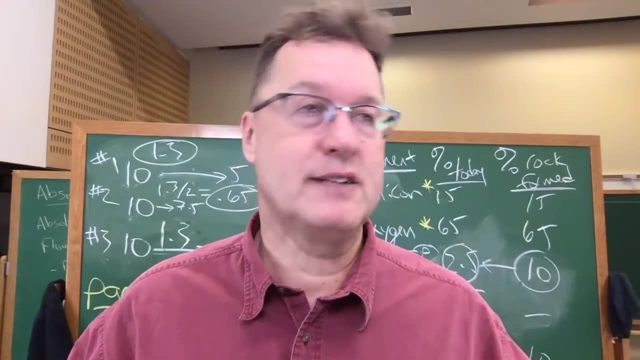 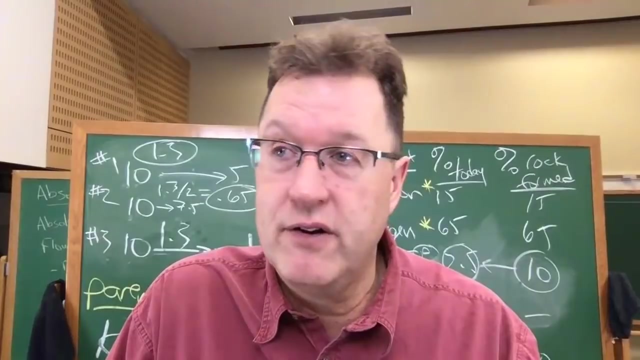 the field of your interest and People making videos. obviously I'm doing these things and making them available. I guess, as I say, that I guess most university people will not be making their stuff available for free to everybody. They should, but they don't. 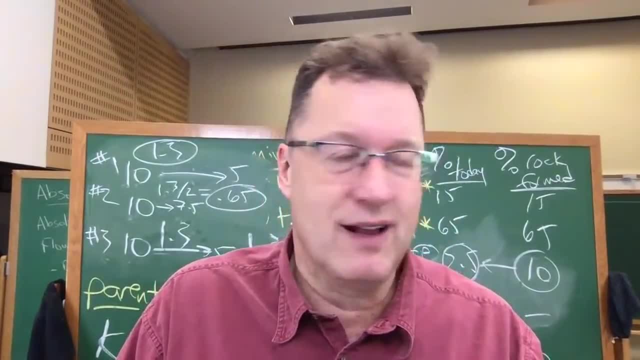 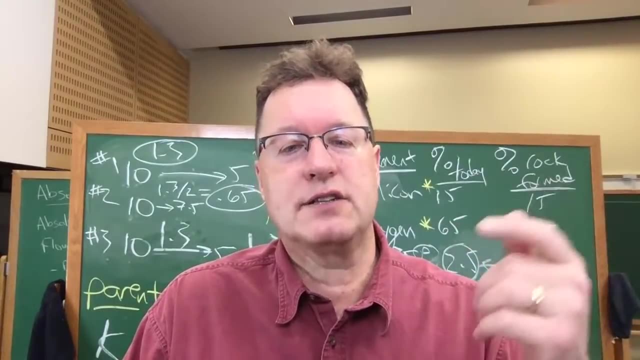 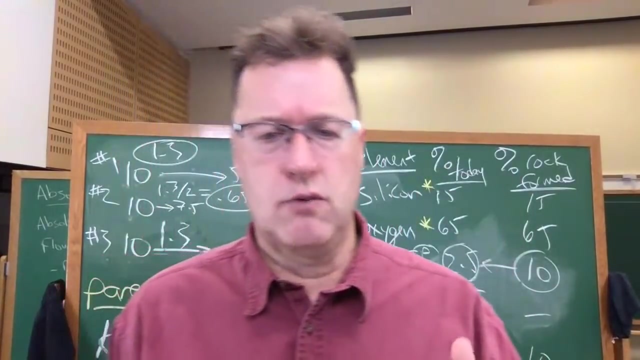 Of course you've got to pay for the great courses and whatever. Make it all free. I saw Ian Stewart and Alice Roberts both on Twitter asking- I'm sure I'm guessing their BBC bosses or whatever were saying we should probably make a few of these programs free to everyone.